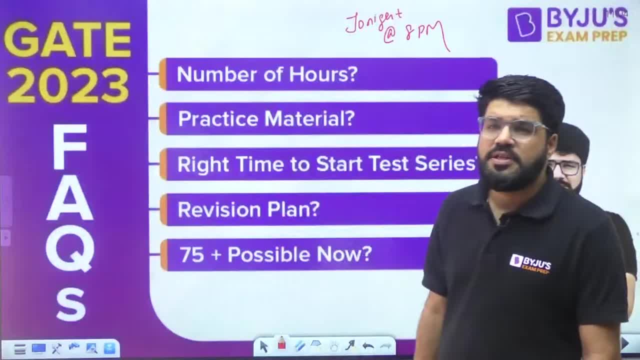 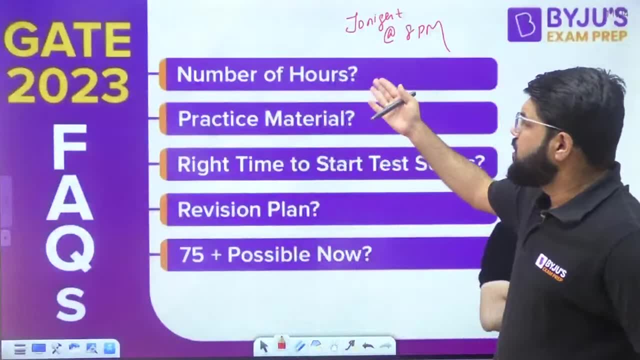 Last on a 100 odd. around 100 odd days are left for the examination. Okay, so what are your regular queries in the last moment, last 3-, 3 and a half months, how you should increase of the number of hours Now, how many number of ours should be the 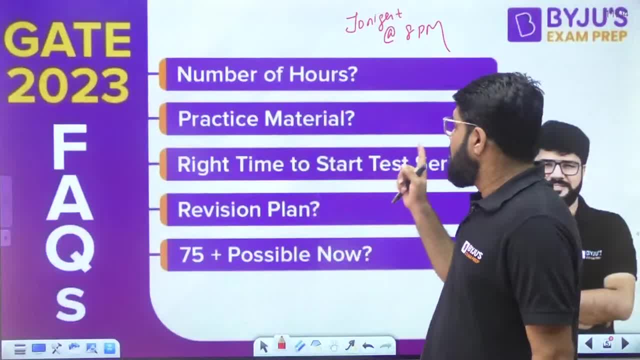 target Now from where you should position yourself. what are your interests in this? What is your one expected progress? Any questions regarding this? Luke Dean is the one who has to the target now from where you should practice, now especially right. what is the right time to? 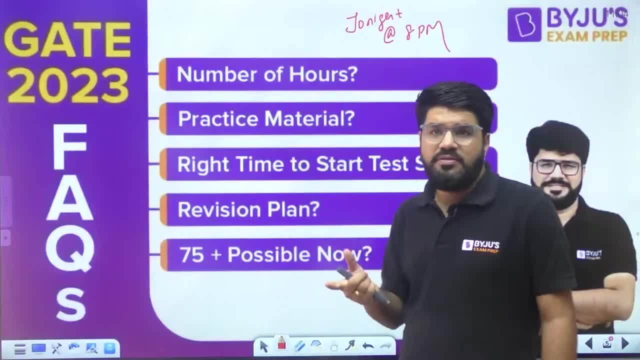 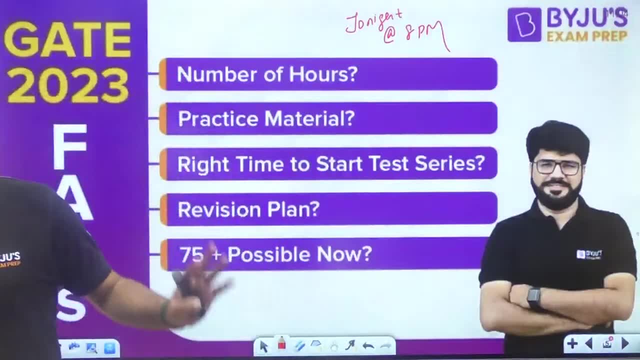 start our series, especially the mock test. what is your revision plan? there's a very time- see high time- you think about a solid revision plan and is 75 plus possible. now we're going to conduct, we're going to discuss all of this right gate. 24- 90 percent sethupati will be conducted by iac. 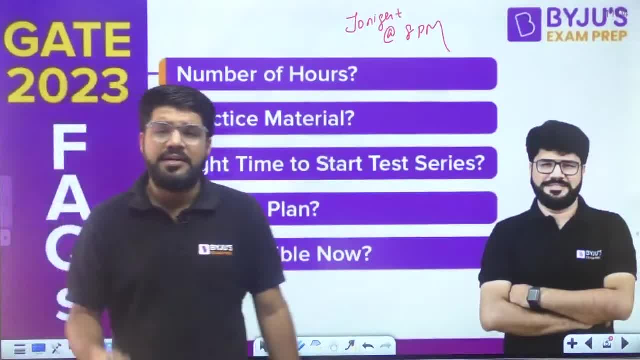 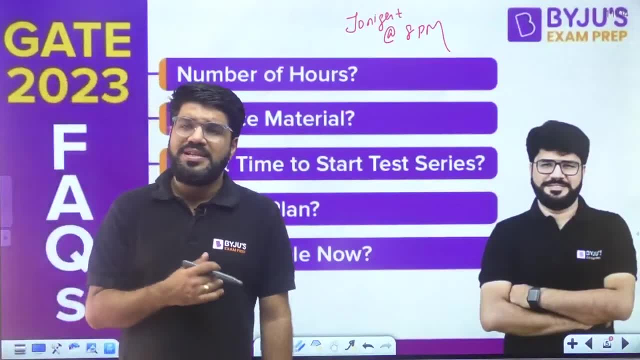 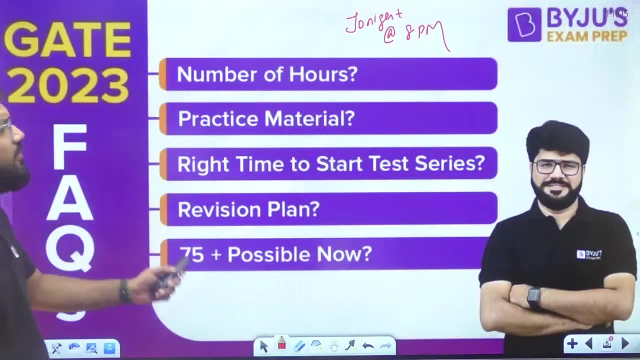 as per the cycle, it is 100 percent iac unless and until they change. they add some organization that is a different thing, or else it is iac turn only if the same bodies remain. so 2016 and 2008 was conducted by iac. after eight years, 2024 will be iac, right, so join me live tonight at the 8 pm. 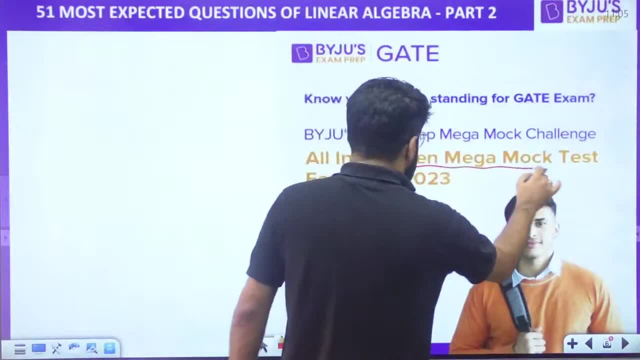 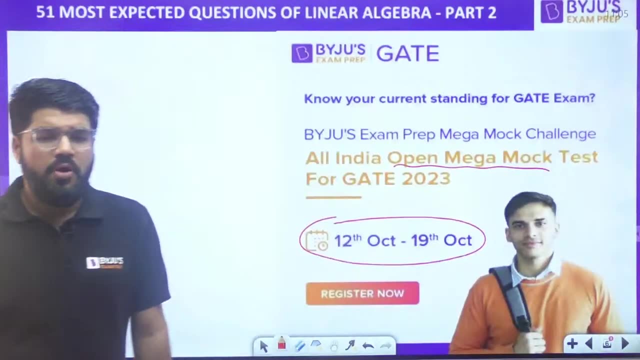 right also guys. all india open mock test is still live. the dates are 20, 12 october to the 19th october. you can register now and appear in the all india open mock test, compete among thousands of students for gate 23 and see your performance. 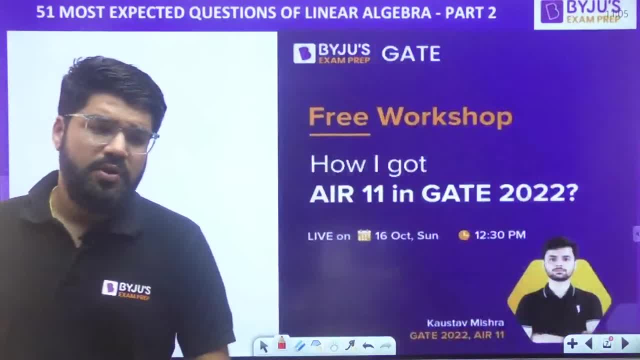 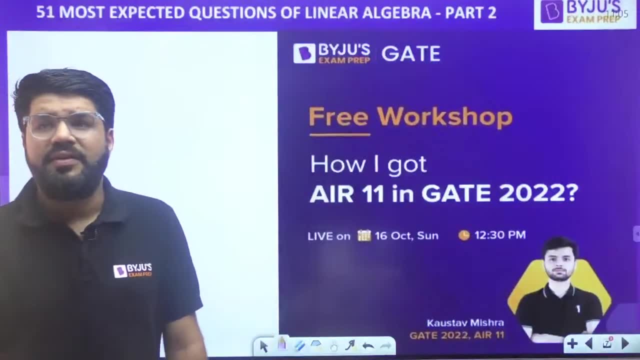 and this is on the byju's exam prep app. download the app from the google play store if you don't have that right. also, we have a free workshop that is today only, by kostaf misra. yes, kostaf secured all india- rank 11 in 2022- and he is going to talk about his journey, how he secured all india. 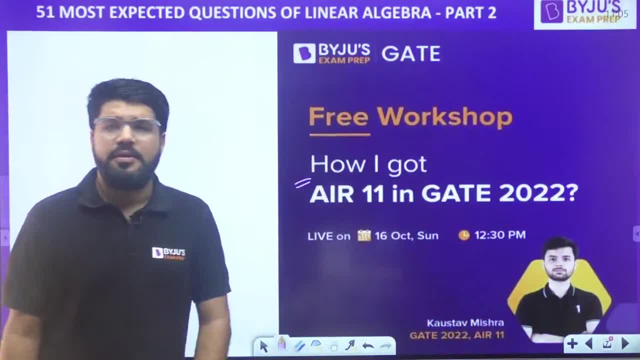 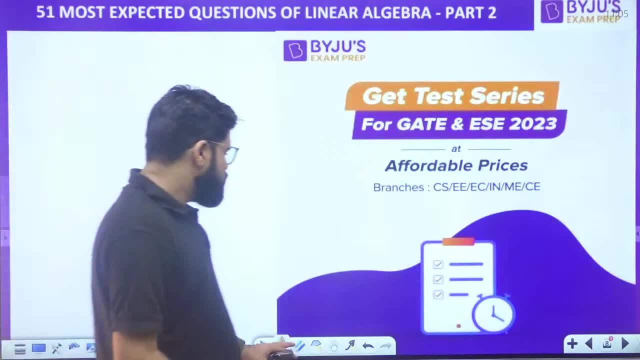 rank 11 in the gate 2022. today at 12: 30 pm. that is again on the byju's exam prep app. keep downloading, keep you know, have the byju's exam prep downloaded with you and also right, if you want the test series for gate, eac and even other pse. 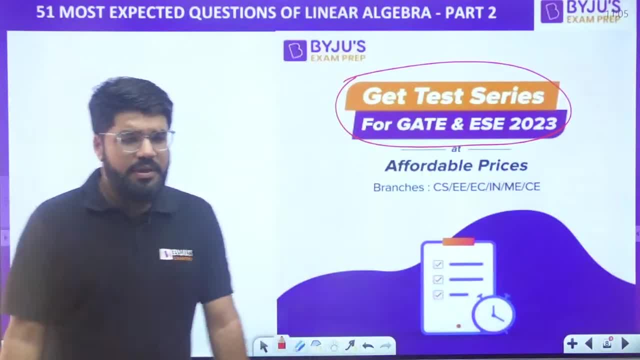 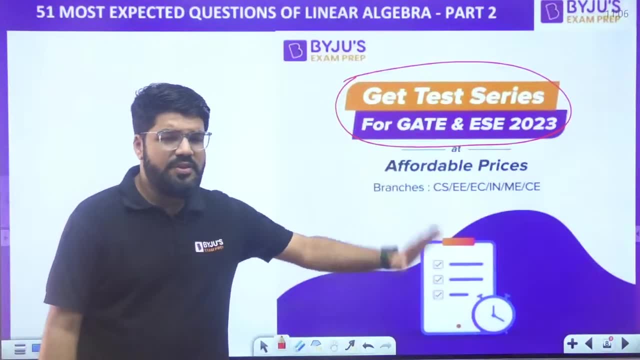 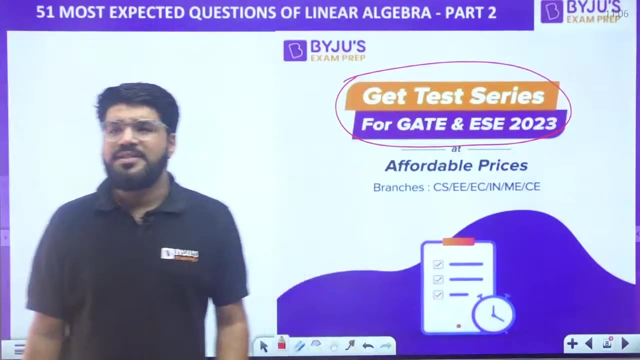 user examination at the very affordable prices. okay, byju's exam path has brought you the test series. you can purchase that also, and it's affordable price. what is the price? what are the timings of the exams? everything is mentioned on the app, right? uh, exact timings, honey. you can check on the app only. so, guys starting. so guys, yesterday. 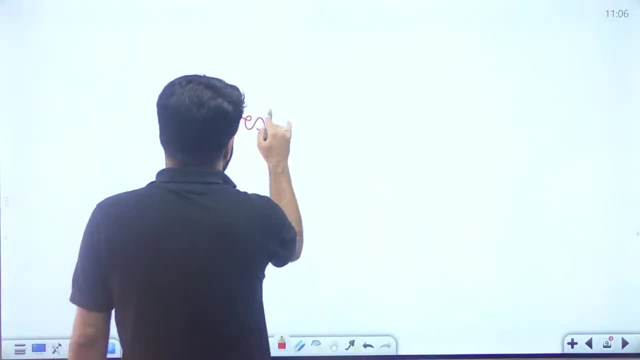 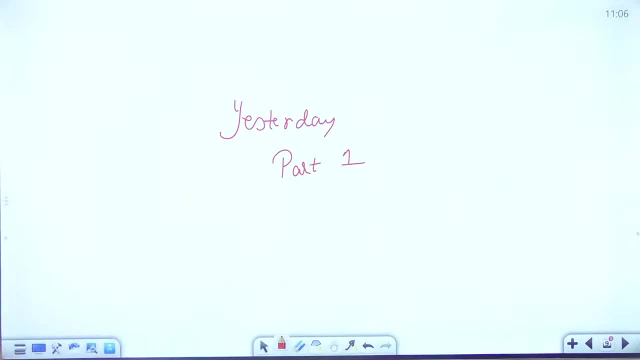 if we have a quick review. yesterday we had discussed a part number one of GUE6 one session which is scratched up by oakland um. so if you want to download that, we have a link available in the description of this 51 question series and in that part number one. and in that part number one we completed the. 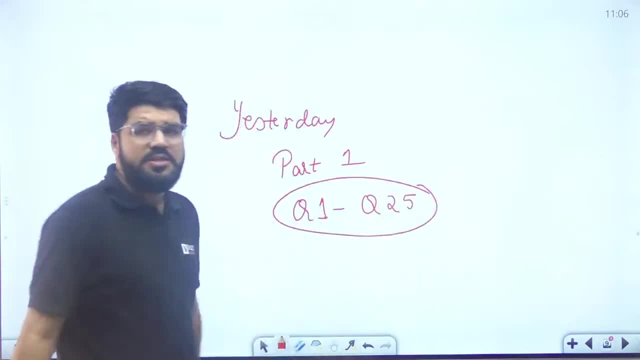 question number one up to the question number 25, and we discussed the questions based on the concept of rank. non-homogeneous system of equation. homogeneous system of equation, all those things? yes, gajendra, planning for it. let me find some bandwidth. busy with many classes, but yeah, i have. 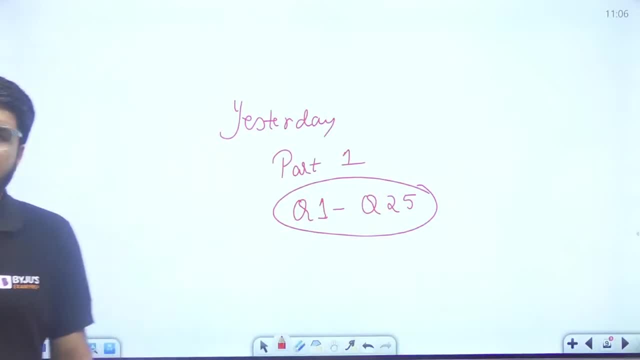 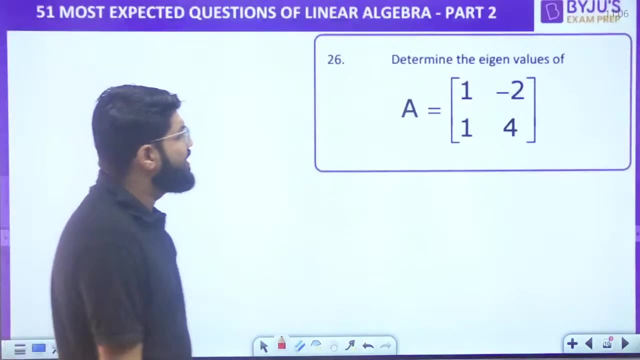 that in the mind. as soon as i find bandwidth, i am going to conduct that also, gajendra. okay. so question number one to question number 25 was done yesterday, and now let us continue with the question number 26. determine the eigenvalues of this two cross two matrix. okay for two cross two. 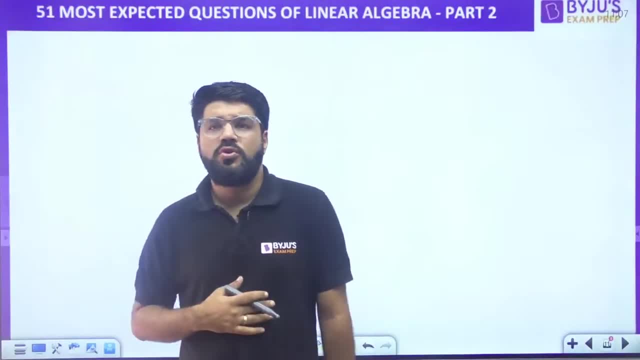 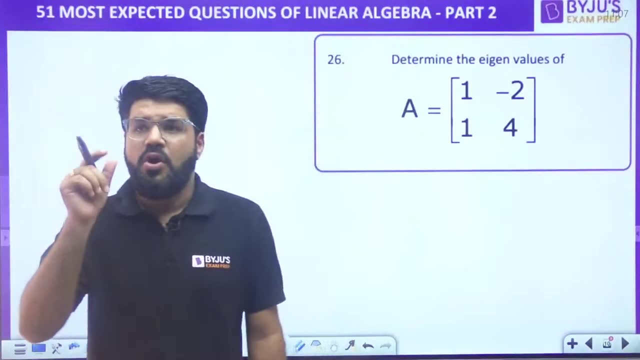 three cross three. i'll tell you the direct methods, direct formula, although we all should know that let's have a quick revision. you know, like yesterday, we have taken the question and, relevant with the question, whatever is the revision, concept, property, technique, whatever is required, i am supporting. 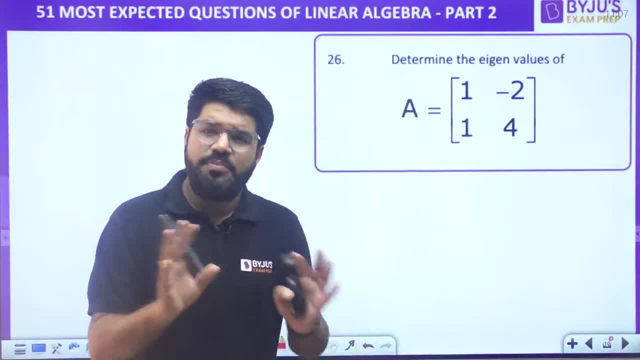 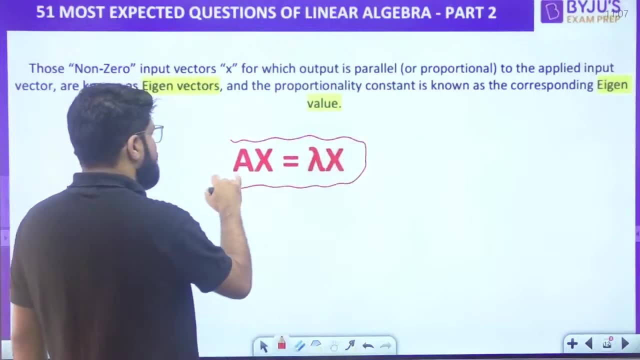 that, so that you know, even if you are studying algebra for the first time. this session, in brief, gives you a quick, good summary of the algebra and you become comfortable, right. so this is how, primarily, eigenvalues and eigenvectors are defined: the non-zero input vectors, those non-zero input vectors x for which output is proportional to. 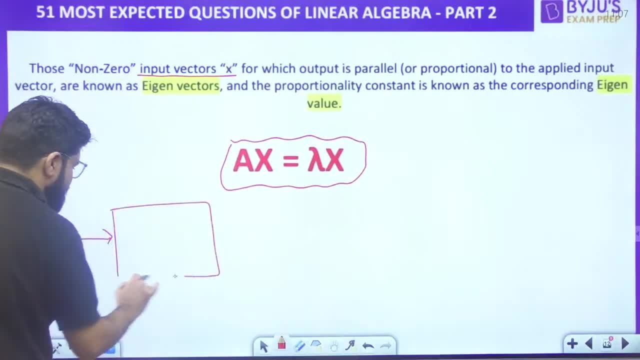 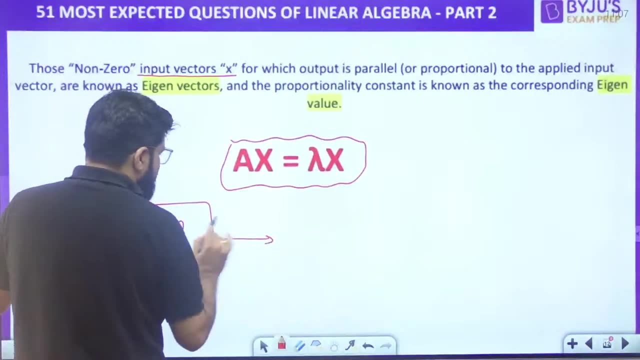 the applied input, right. so in short, let's say you have a system, matrix a, you have a system defined by the matrix a, you apply some input x and you get the output. you get the output like what you were getting in the homogeneous system of equation- right in homogeneous. or let's say: 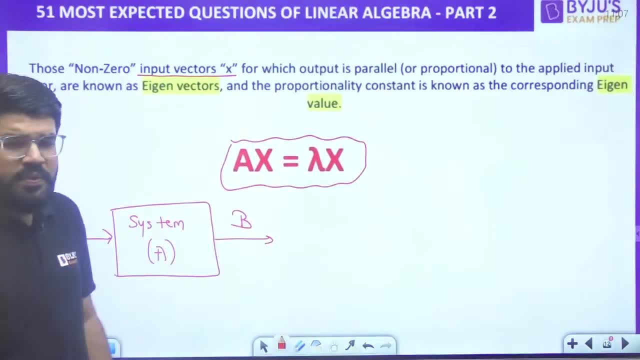 system of equation a into x is equal to some constant b right. a. x applied to the system, it produces some constant b in homogeneous. that becomes the null right. but now those special vectors for which the output, those special vectors x, for which the output is proportional to x. now, 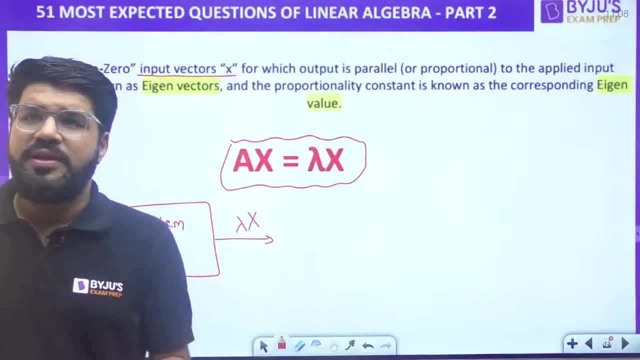 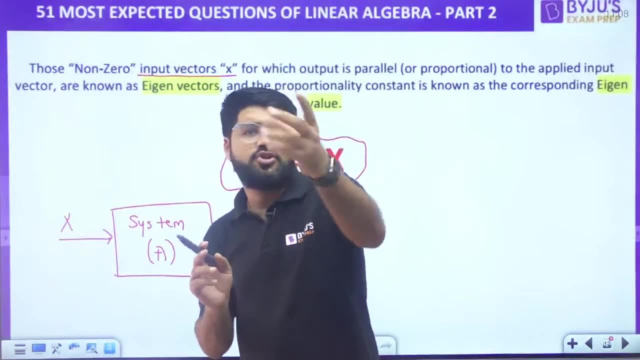 proportionality means lambda into x or alpha into x, anything. so let's say lambda is the proportionality constant. those input vectors: very brief theory in the brief, more focus on questions and techniques. right so those input vectors x, for which output is lambda, x that is proportional to the input. 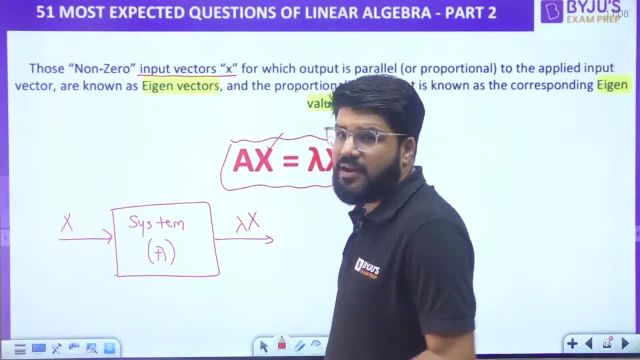 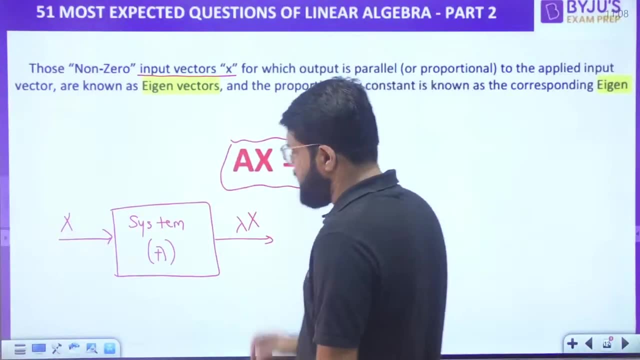 parallel to the input, are known as the eigenvector. so x will be the eigenvector. the proportionality constant, the number that is multiplied by x that appears with the out x in the output, is known as the eigenvalue. that is known as the eigenvalue right. so we call x as the eigenvector. 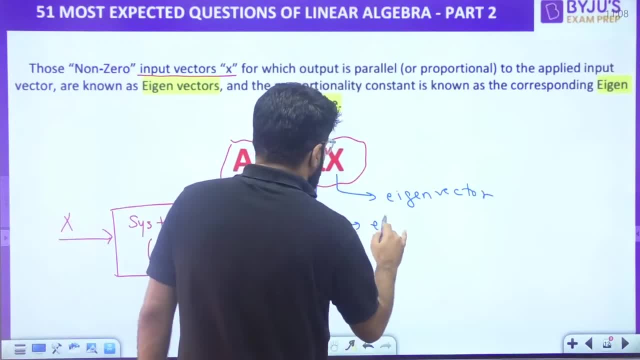 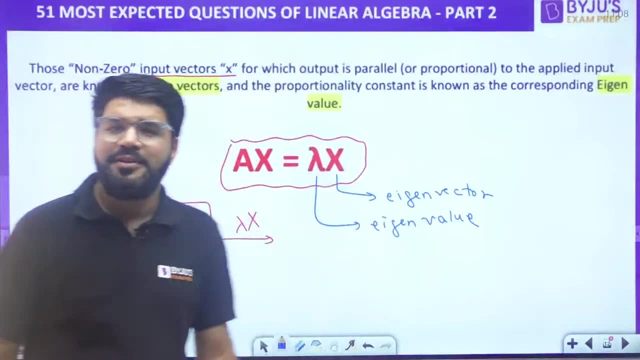 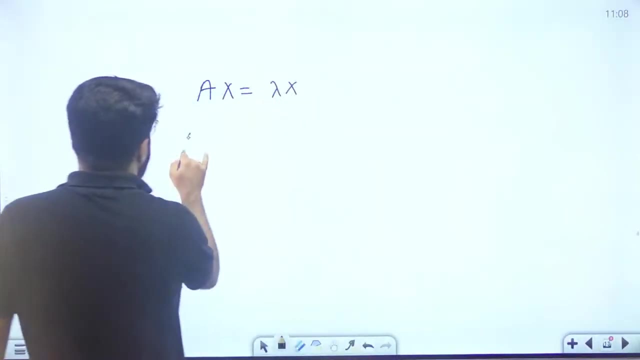 and lambda as the eigenvalue. now, how do you solve this eigenvalue then? how do you solve for this eigenvalue? thank you, jeet. right, how do you solve for this eigenvalue? so let's have a quick review. we have a x equal to lambda x. bring the x on the left hand side, so a x. 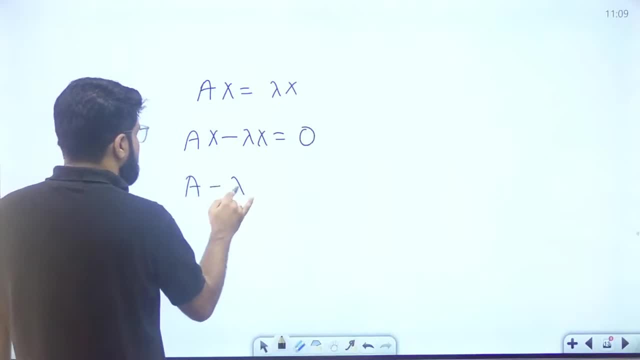 minus lambda x is equal to 0. taking the x common, you have a minus lambda i whole multiplied by x equal to the 0. a minus lambda i whole multiplied by x. a is a matrix, lambda is a number. so you can't subtract matrix a number. that is why we multiply by i equal to 0. 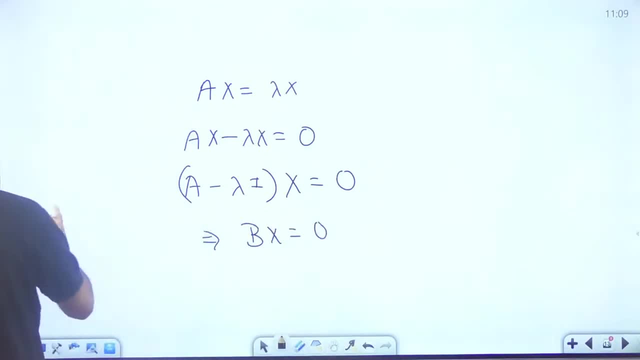 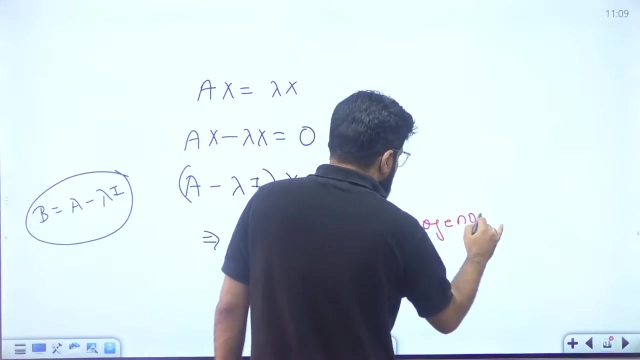 right. this is of the form bx equal to 0 right, where b is equal to a minus lambda i. let's say b is equal to a minus lambda i. so this is like bx equal to 0 right. bx equal to 0. yesterday we have studied bx equal to 0 is known as. what type of system? bx equal to 0 is known as homogeneous. 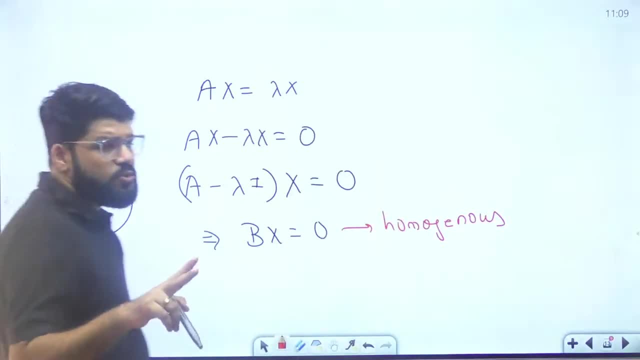 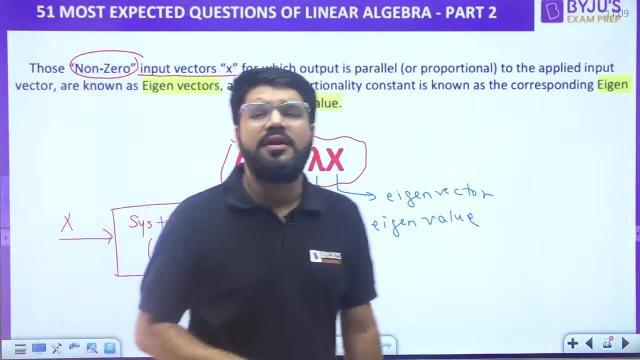 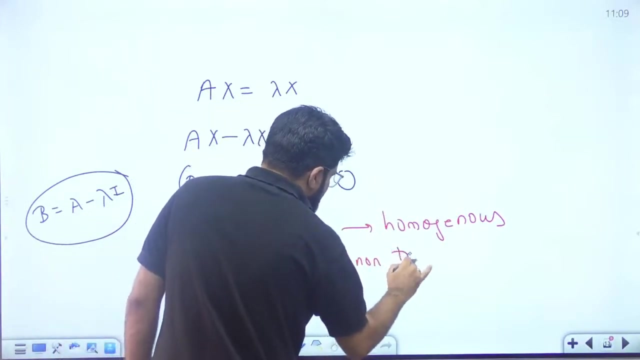 type of system, right. what type of solution you want now? homogeneous has two types of solution: trivial and non-trivial- right? you want the non-zero input vectors and non-zero vectors in the non-trivial case, right? okay, what we need is the non-trivial solution now, everybody. 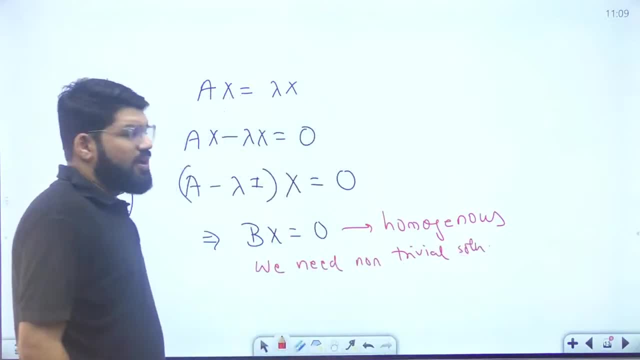 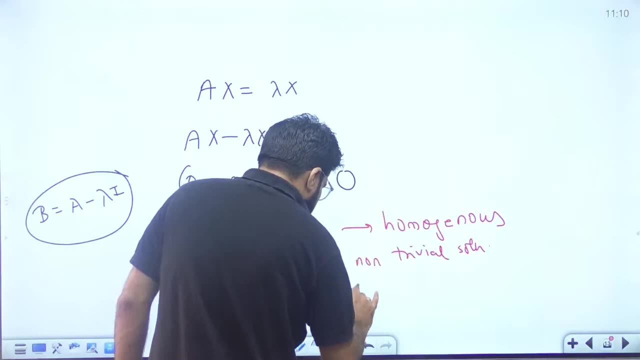 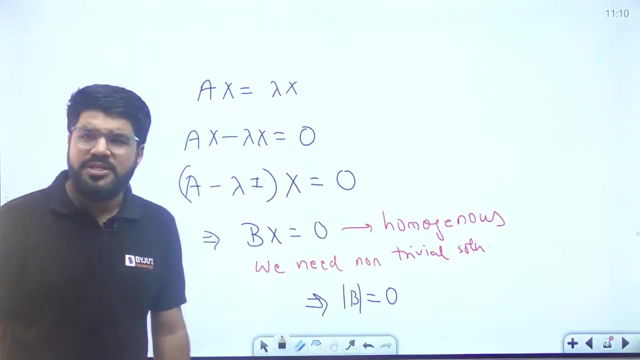 we have taken several questions yesterday. what is the condition for non-trivial solution? what is the condition for non-trivial solution? the determinant of the matrix, which matrix? here the matrix is b. it is not a right. yeah, direct equation, that's what. okay, so modulus of b equal to 0. here the matrix is: 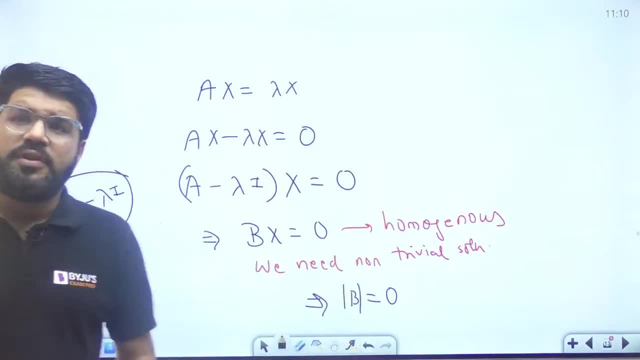 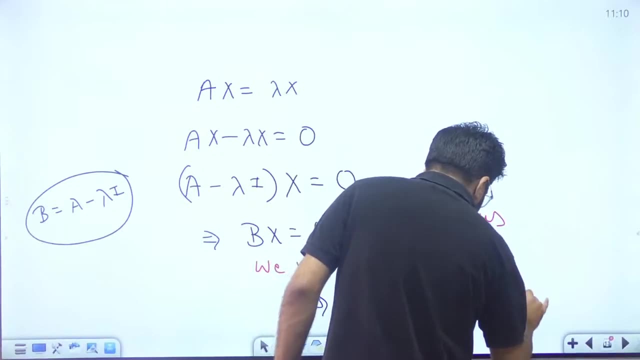 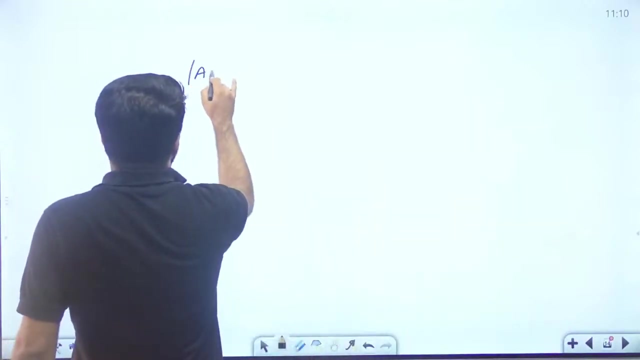 b. so determinant of the b is equal to 0. that is the condition for trivial solution. now, determinant of b, what is b? a minus lambda i? determinant of a minus lambda i, equal to 0. this is the very famous, known as what everybody can recall. what is this equation known as for any matrix? a modulus of a minus lambda. 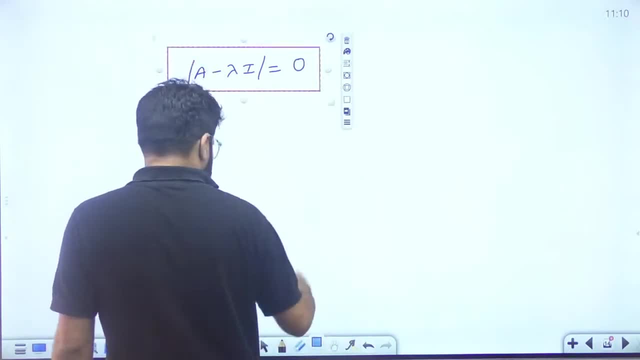 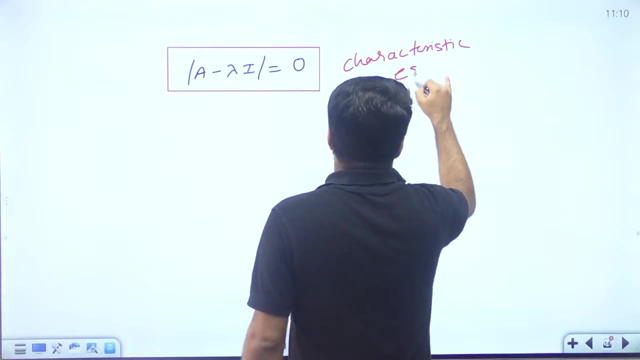 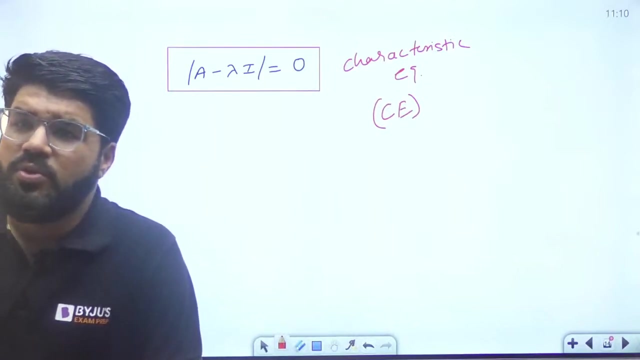 i equal to 0. modulus of a minus lambda i equal to 0 is primarily known as the non-trivial characteristic equation. in short, we will keep calling it as ce. modulus of a minus lambda i is equal to 0 is known as the characteristic equation right. so to find out eigenvalues. 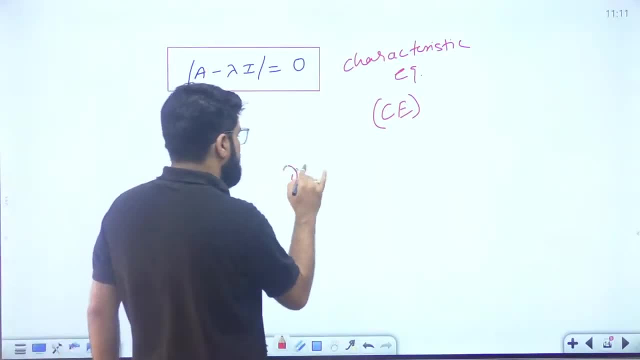 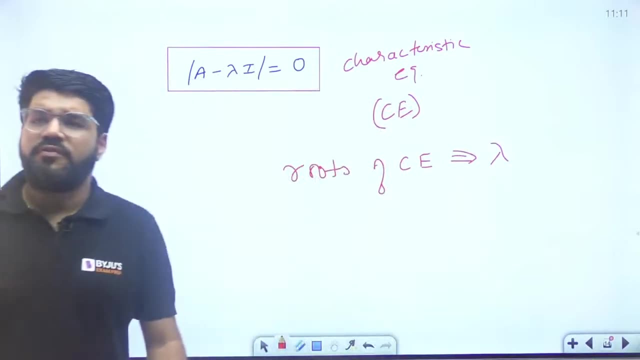 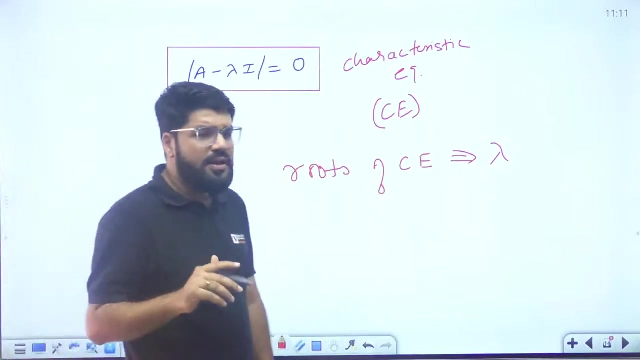 you need to solve the characteristic equation so that you get the lambda. the roots of this characteristic equation will be lambda will be the eigenvalue. so one more way of defining eigenvalue. eigenvalues are the roots of characteristic equation. now they go commonly. the question of eigenvalue is a question if it is direct calculation. question 90: 2 cross 2, 3 cross 3. 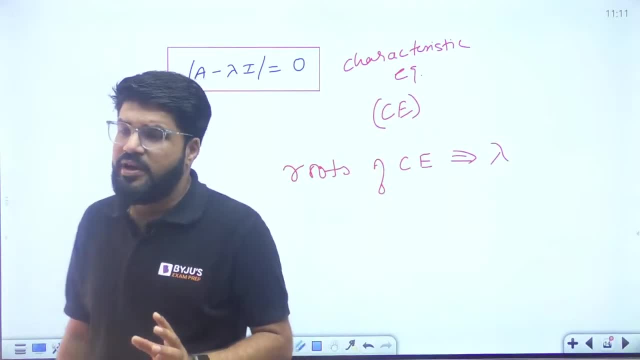 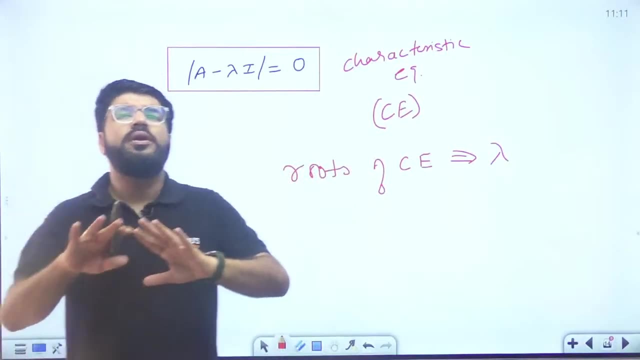 90, 2 cross 2, 3 cross 3. so i will separate out the method for 2 cross 2, 3 cross 3, for higher order. if there is a question, it is mostly property based. so there are set of properties, 16 properties, i'm going to tell you. that is going to cover all types of questions of eigenvalue. 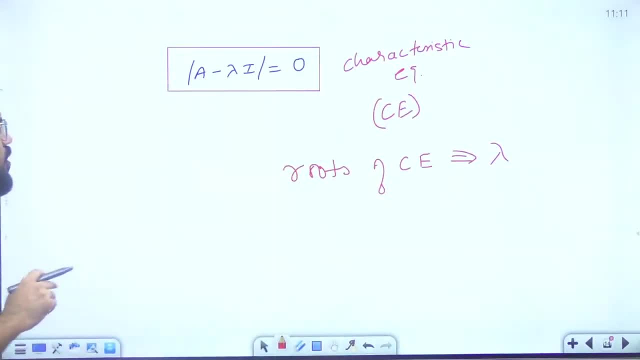 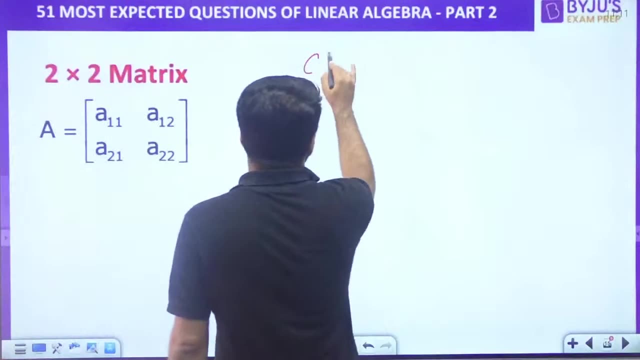 that is going to cover all types of questions of eigenvalue. okay, so roots of characteristic equation are eigenvalue. so if i take a 2 cross 2 matrix, right, if i take a 2 cross 2 matrix, two matrix- characteristic equation is simplified as no need to derive. okay, let us write down. 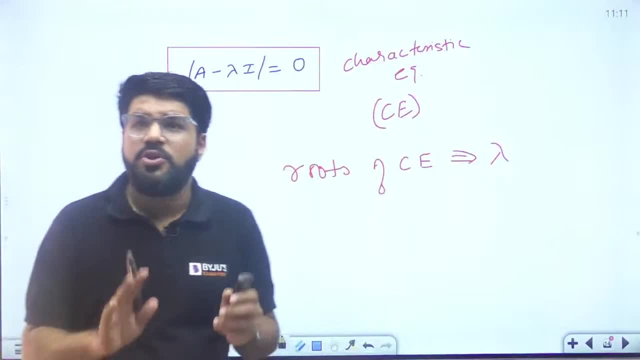 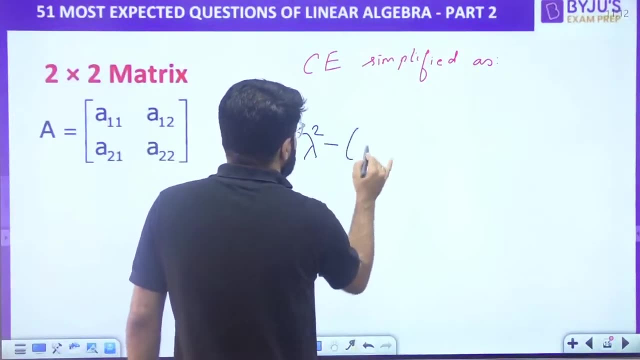 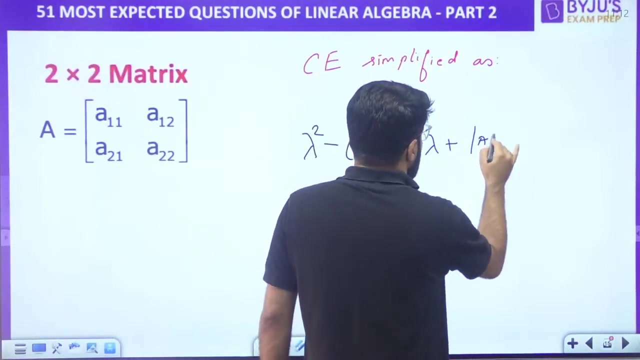 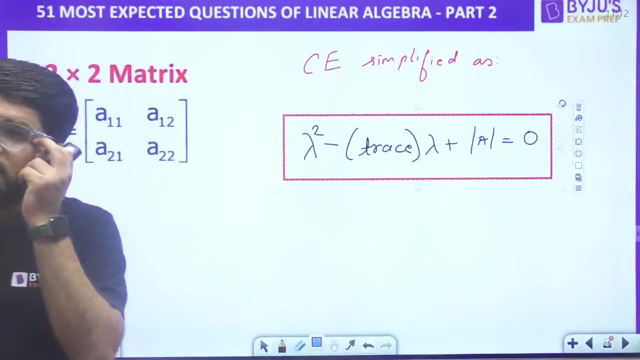 directly. when i apply the formula a minus lambda i determinant equal to zero for a two cross, two matrix, what is the simplified result? direct. note: no time for derivation, although it's two line, but still lambda square minus trace. lambda plus determinant of a equal to zero. lambda square minus trace. lambda plus determinant equal to zero directly. you have to use this if it. 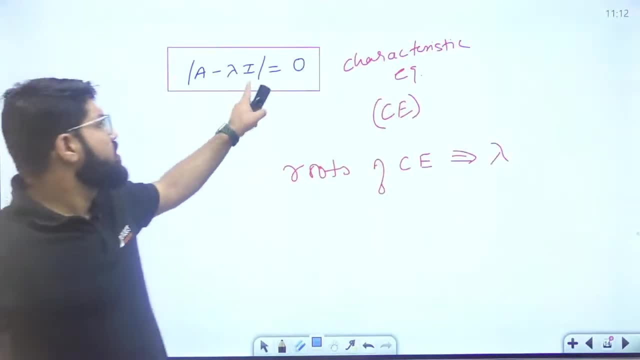 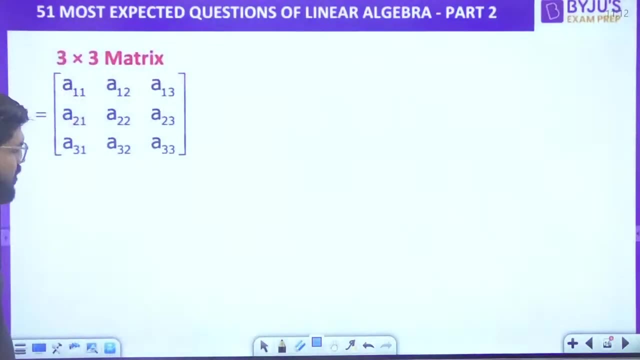 is a two cross two. many students i have seen they start always using this equation, whether it is two cross two, three cross three. two cross two, three cross three is the most common type of question, so please use this for two cross two, sir. what about three cross three? i'll write down the result. 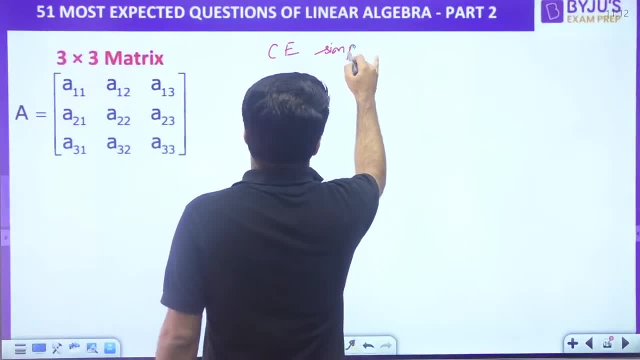 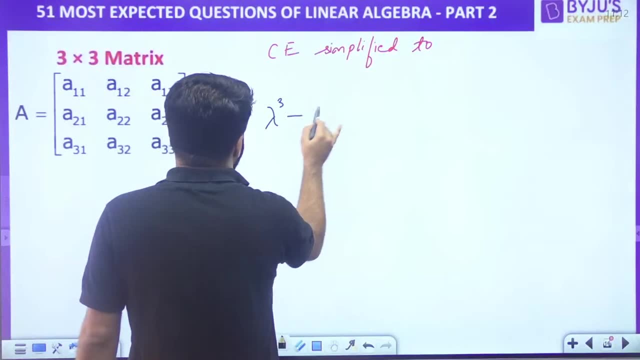 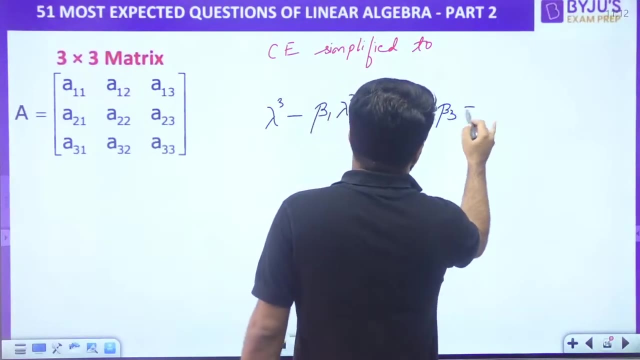 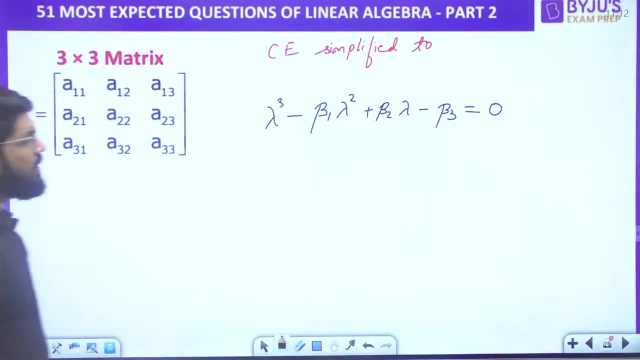 for three cross three. also for three cross three, characteristic equation is simplified. as characteristic equation is simplified to you: lambda cube, cubic here, minus beta one lambda square plus beta two. lambda minus beta three, equal to zero. lambda cube minus beta one. lambda square plus beta two. lambda minus beta three. 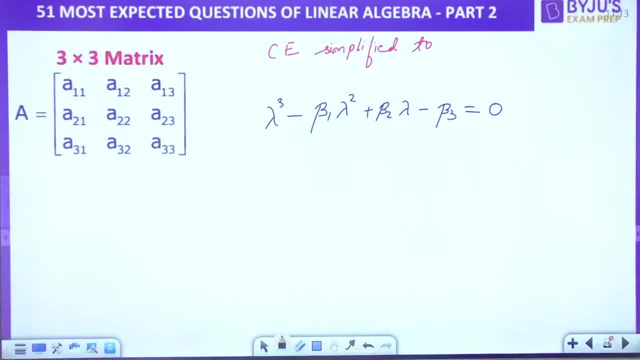 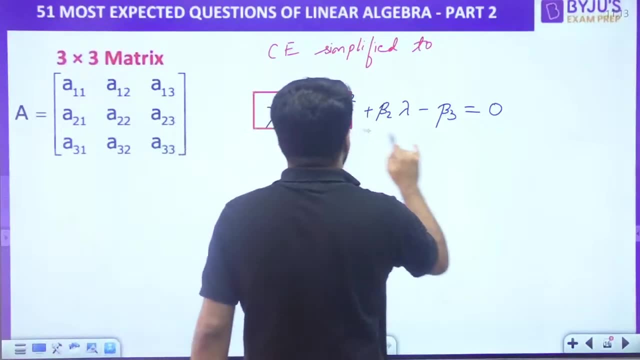 equal to the zero lambda cube minus beta one lambda square plus beta two lambda minus beta three, equal to zero. now what is the point? beta one, beta two, beta three. i'm there to explain, you don't worry, gotcha, i know how to estimate that this matrix system. 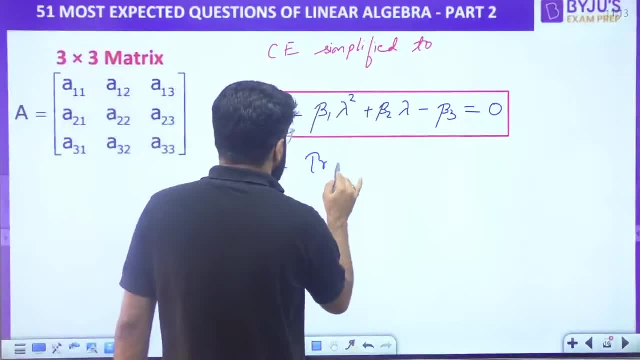 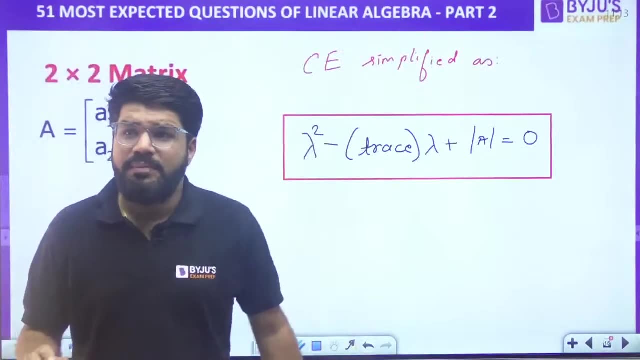 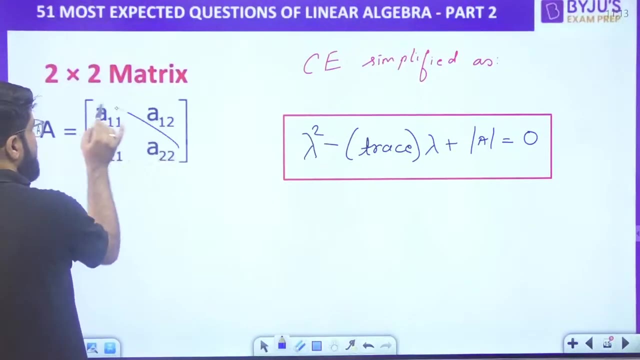 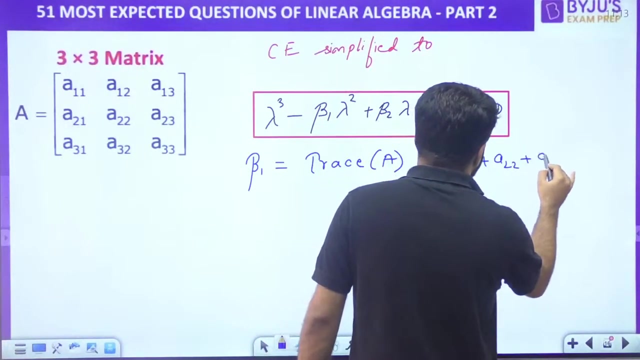 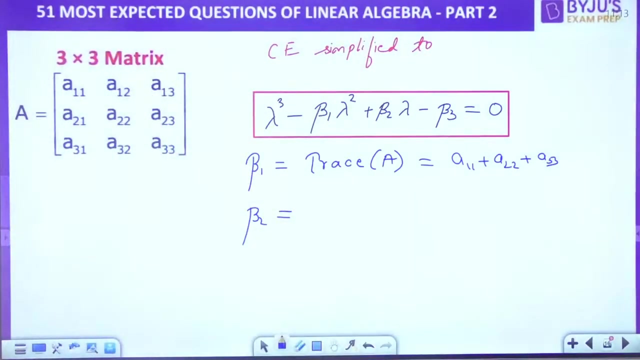 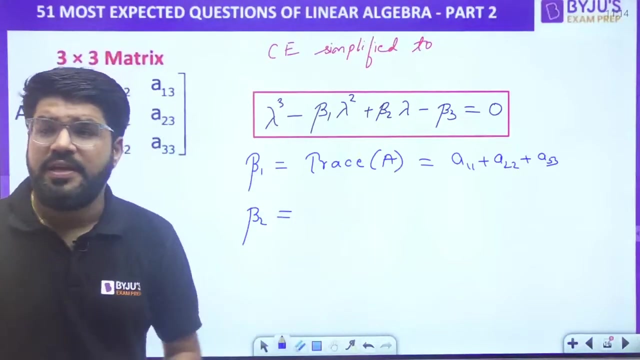 but it too long. are you just kidding? what is the "-frame"? then beta 2, right? good morning pioush. right, right say, to put the real-life: Fourier series is a very Fourier series is a very important tool related with this eigenvalue and eigen signal concept. okay, not only Fourier, even Laplace Z. 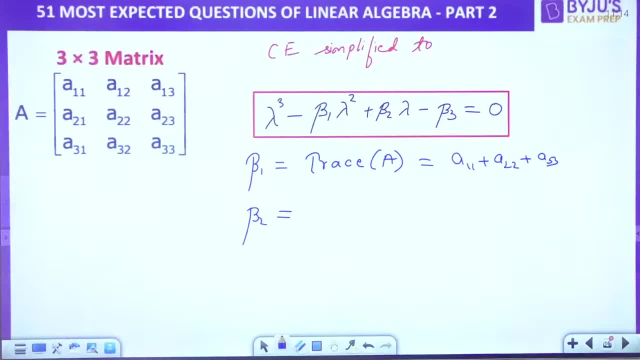 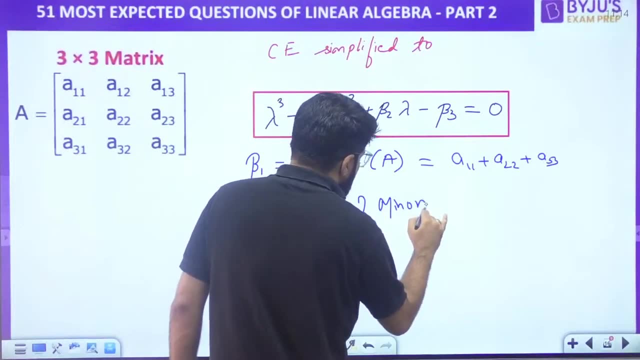 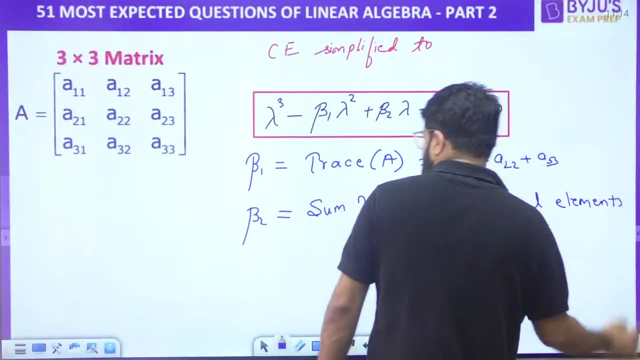 discrete. maybe dying is a very related concepts we use. okay, so what is beta 2 now? beta 1 is sum of diagonal elements. beta 2 is known as sum of sum of the minors of the diagonal elements. we will apply on question, don't worry, beta 2 is. 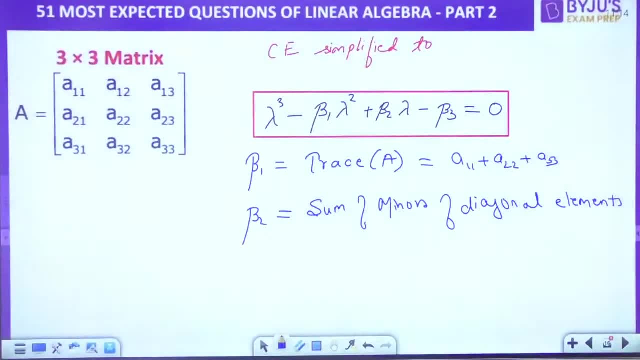 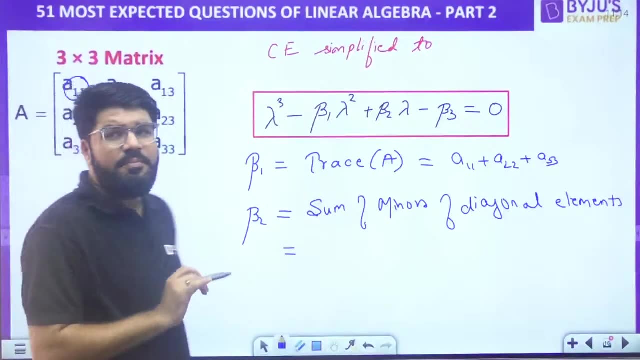 known as the sum of the minors of diagonal elements. okay, what does this mean? what is the meaning of this sum of the minors of diagonal elements? this is equal to everybody. see, this is the first diagonal element. how do you calculate the minor of any many element? delete its row and 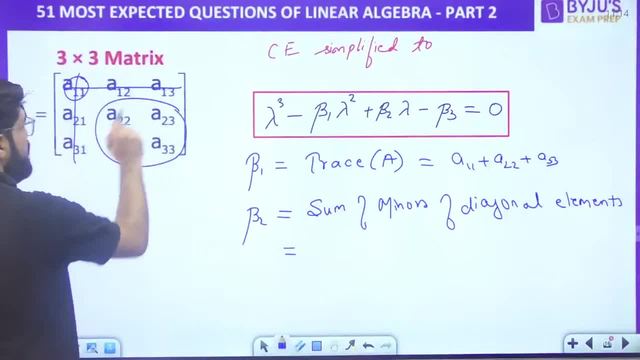 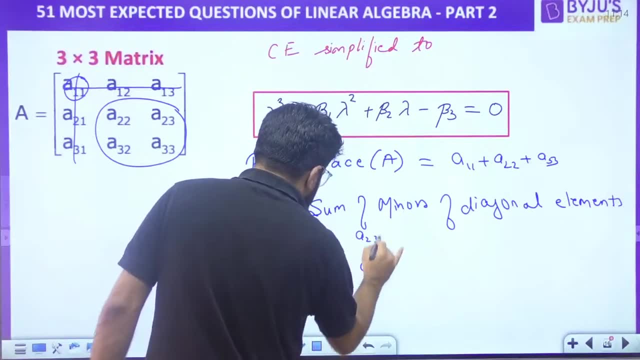 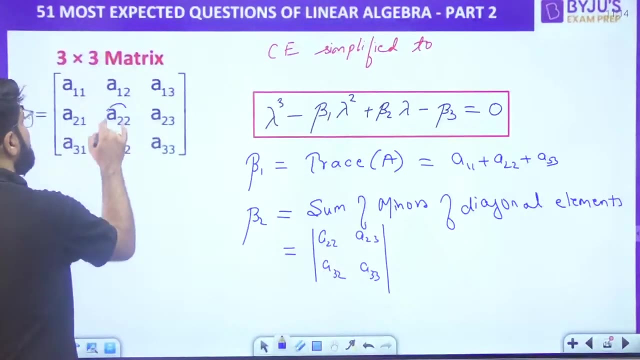 column right, delete its row and column. you get what? a 2, 2 a, 2, 3 a 3, 2 a 3, 3. this is the minor for the first diagonal element. this is the minor for the first diagonal elements. next, next diagonal: 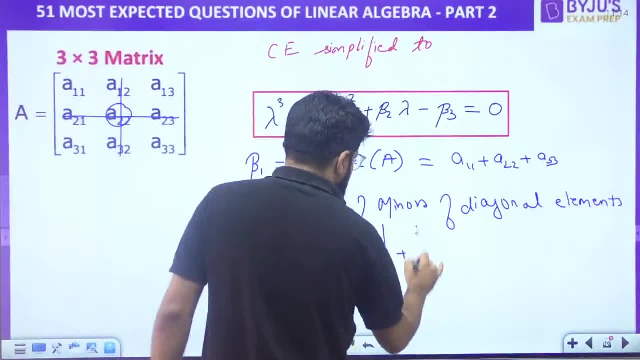 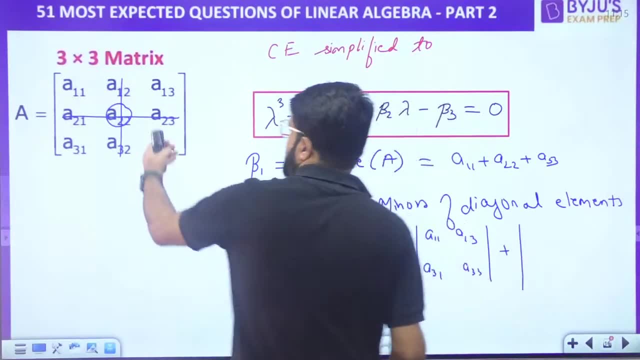 element a 2 to delete second row, second column. you are there with. you are there with a: 1, 1 a. 1, 3 a 3, 1, 3, 3. similarly, if you delete the third row and third column, you take the third diagonal element. delete third row and third column, you get a. 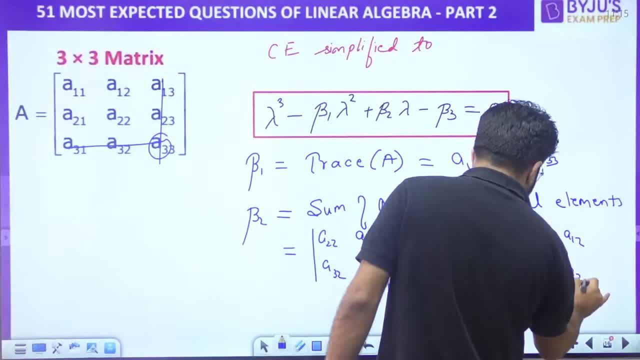 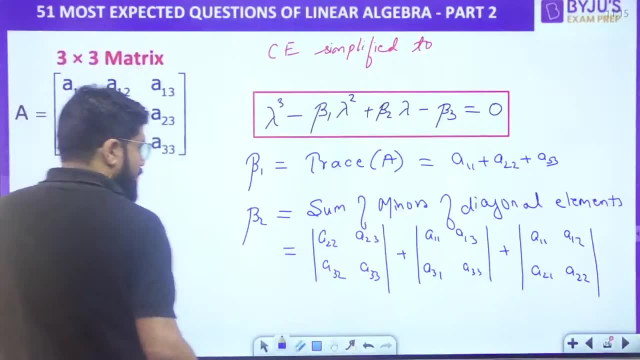 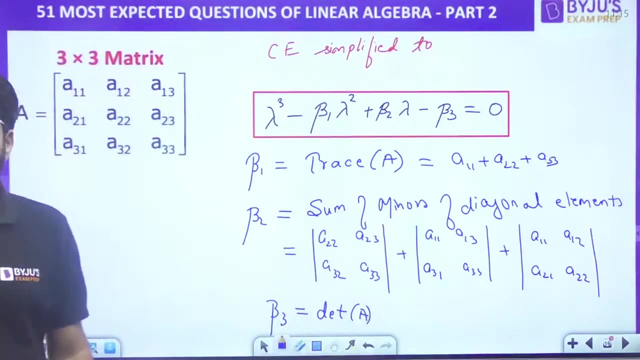 one, one, a one, two, eight, two, one, eight, two, two right. this is what is beta two. sum of the miners of diagonal elements. good morning, Nishu. okay, left is beta 3. what is beta 3? the last element, again determinant of it, it is again the. 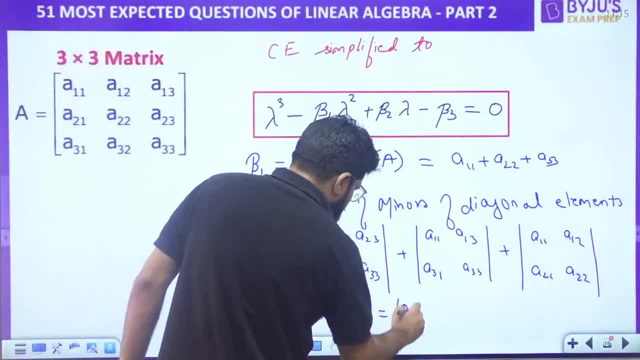 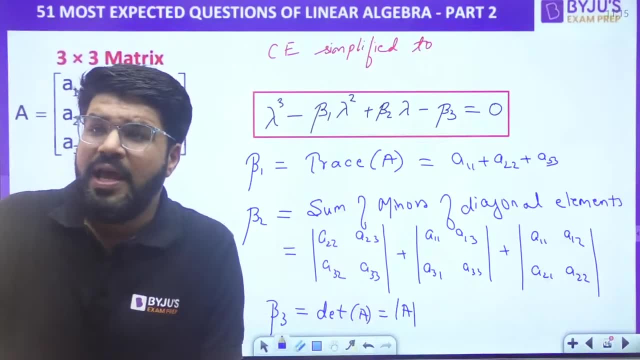 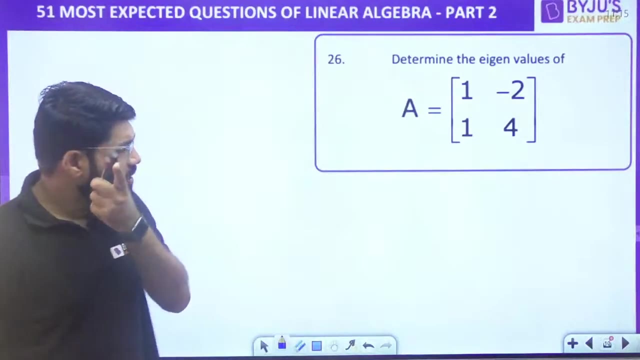 determinant of a modulus of it. now let us take, you know, two, three basic questions on this and then we will take a property. property based questions are very important and very frequent and they can be very good questions. I'm will cover all range of questions, don't worry. okay, let us go back, question number 26 and determine. 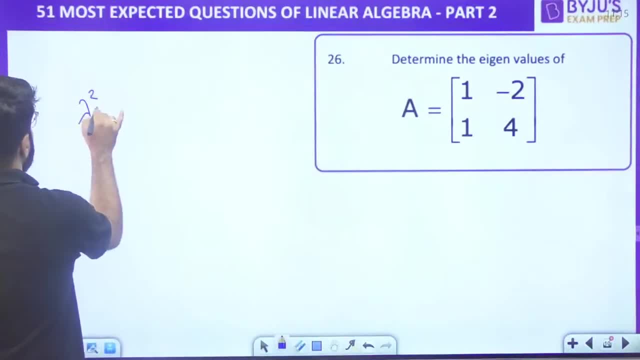 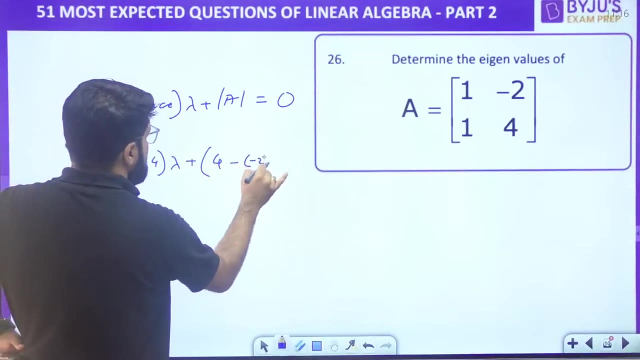 the eigenvalues. so what is the equation, guys? this is 2 cross 2 question: lambda square minus trace. lambda plus determinant equal to 0. put down the values: lambda square minus trace, trace is 1 plus 4 plus the determinant, 4 minus minus 2 equal to 0. so i have lambda square minus 5, lambda plus 6. 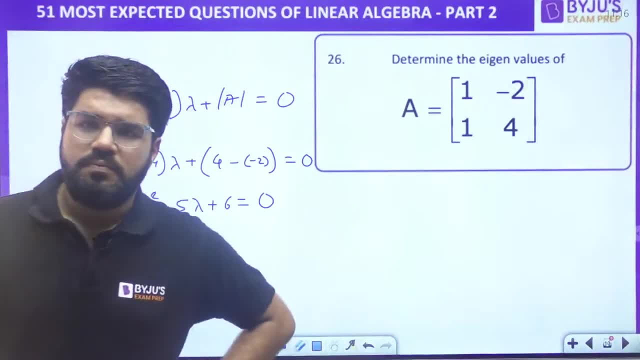 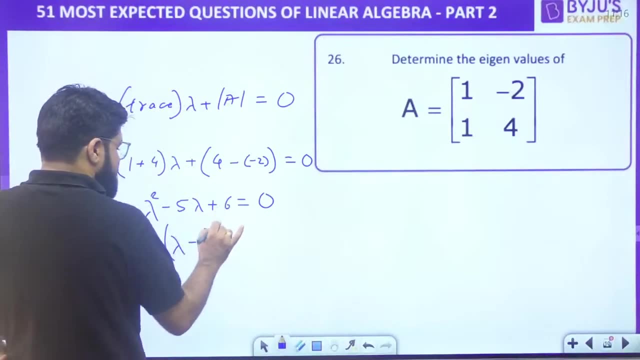 equal to 0. either apply the quadratic formula right, or either it is clearly factorizable: lambda square minus 5. lambda 5 is 2 plus 3. 6 is 2 into 3. so this is lambda minus 2 minus 3 equal to 0. lambda is 2 and 3. 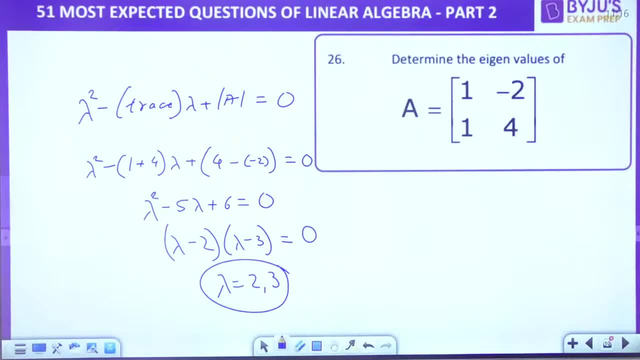 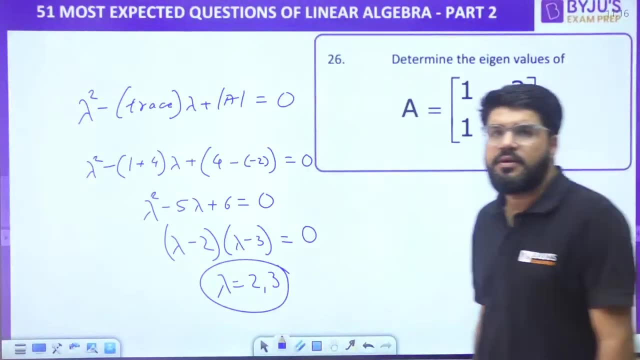 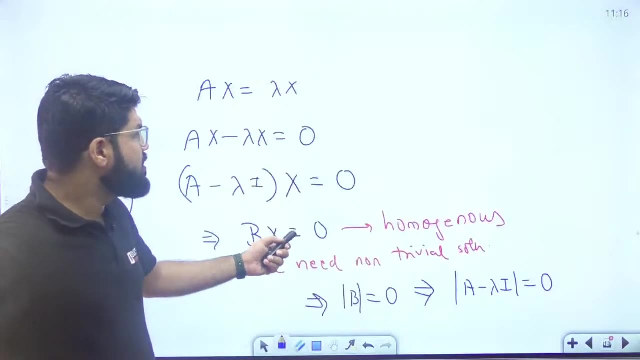 lambda is known as 2 and 3 right. so already for this question, you know many of you have already given the answer earlier: right- lambda is equal to 2 and 3, so let us move ahead to the question, next question, and keep sharing the session and if you are enjoying, do not forget to like the session. 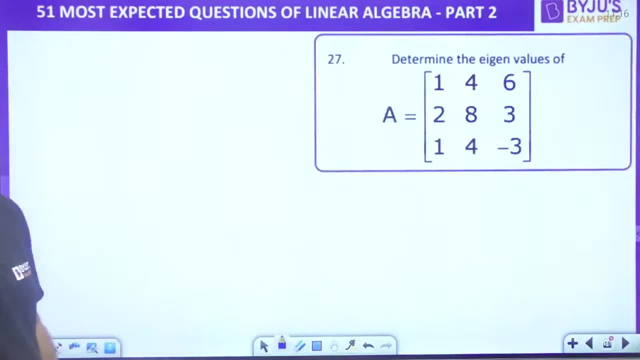 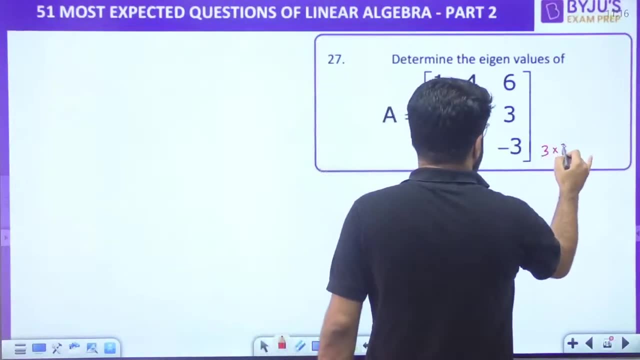 let's be all motivated in the early morning- it's not very early morning, but yeah, it's still it's morning. determine the eigenvalues of now. i'll take a 3 cross 3 case. now. let us take this 3 cross 3 case. everybody for 3 cross 3, we need to first find beta 1, beta 2, beta 3, because the characteristic 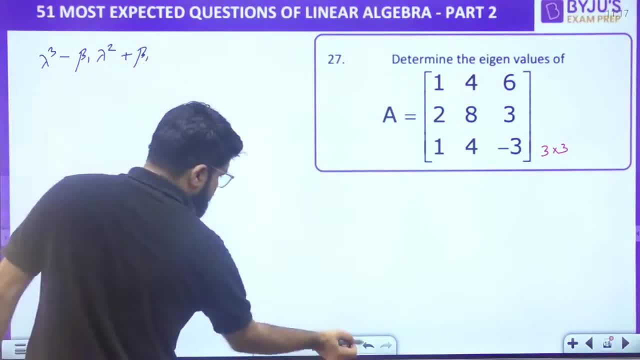 equation was: lambda q minus beta 1. lambda square plus beta 2. lambda minus beta 3 equal to 0. what is the beta 1? as i told you, it is the beta 1 lambda square plus beta 2. lambda minus beta 3 equal to 0. 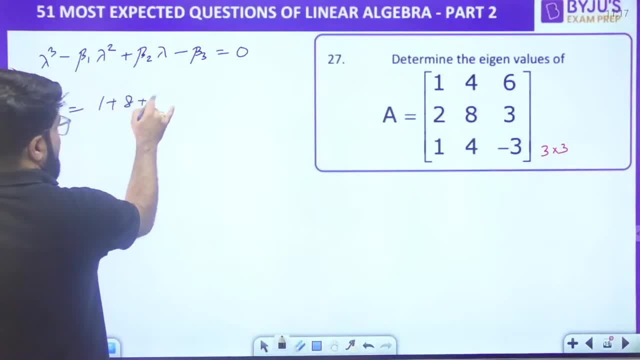 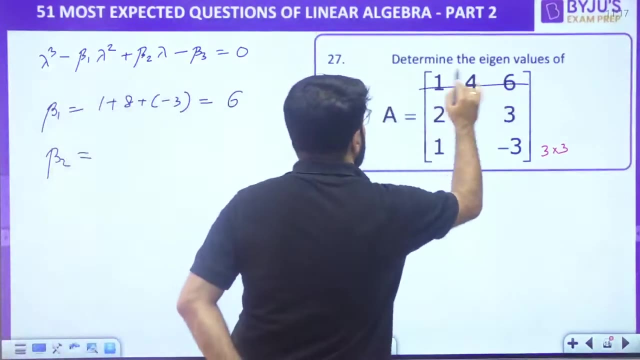 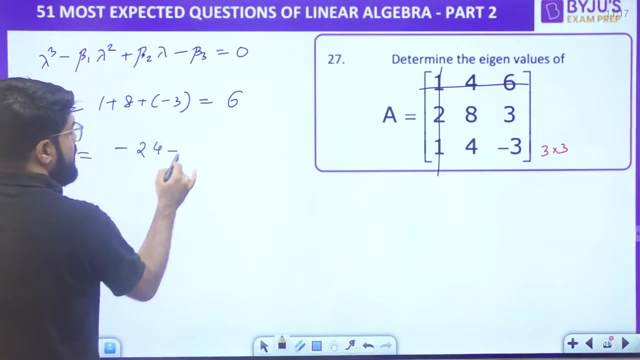 that is the trace directly at the elements. that is 1 and 8 and minus 3. that becomes 6, that becomes the 6 right. what should be the value for beta 2? the beta 2 is given by sum of the sum of the minus of diagonal element. first, diagonal element 1. delete the row and column, you get 8, 3, 4 minus 3. directly value 8 into minus 3, minus 24, minus 12. this is the first minor second. 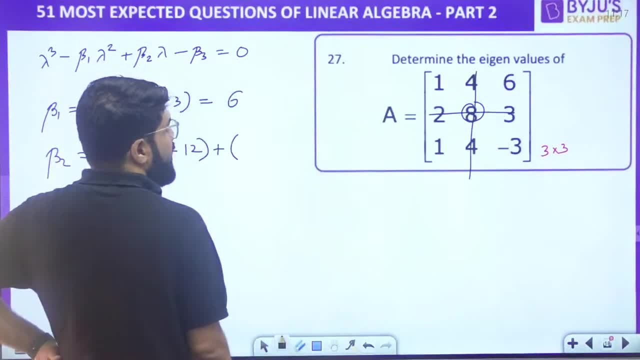 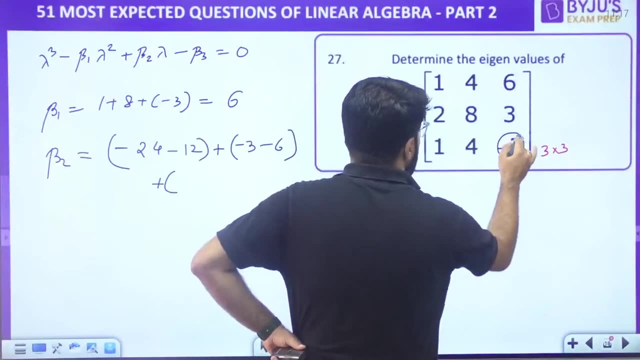 this is the second diagonal element. so, second row, second column, deleted. i have 1 into minus 3 minus 6 plus the third one, third one. this is the third diagonal element. delete the third row, third column. you are left with 1 into 8 minus 2 into 4. that is also 8. so, effectively, what is the value? 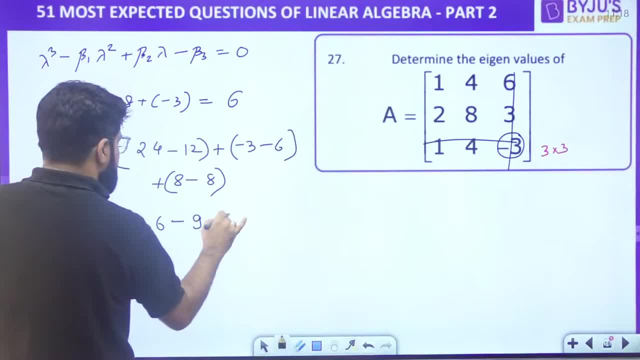 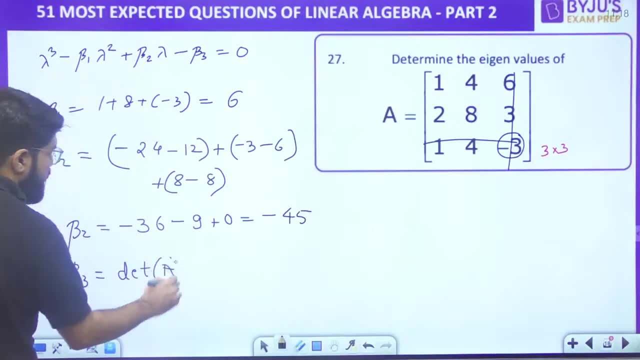 of beta 2 minus 36, minus 9 and plus 0, so beta 2 is equal to minus 45. then, guys, what is the beta 3? beta 3 is known as the determinant of the given matrix, whose eigenvalues are 0 and plus 0, so beta 2 is. 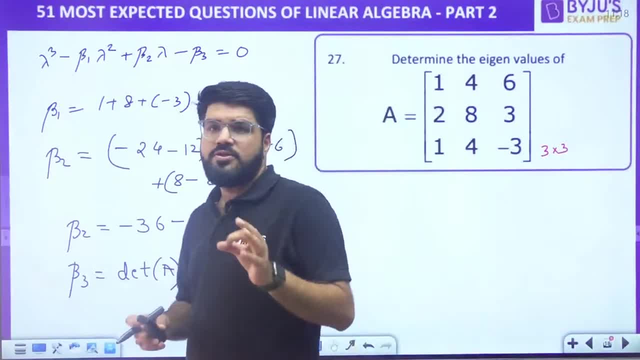 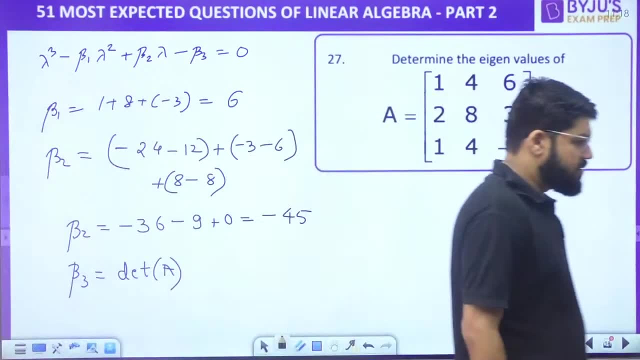 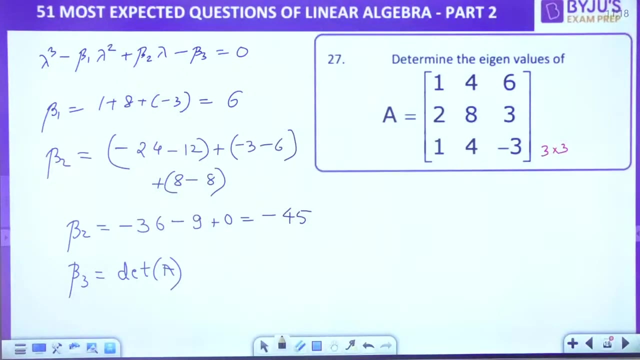 an eigenvalues are required. okay, beta 3 is known as the determinant of the matrix. beta 3 is known as the determinant of the matrix. beta 3 is known as the determinant of the matrix. so what will become its determinant? ok, very quick calculation for determinant. 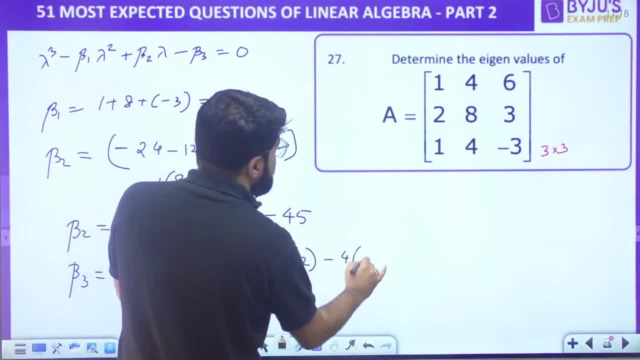 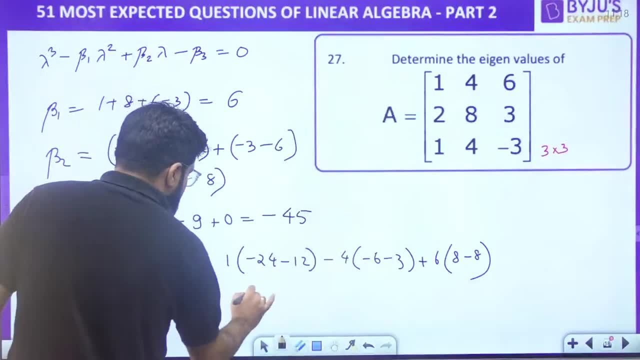 1 into minus 24 minus 12 minus 4 into minus 6 minus 3. plus of 6 to 4s are 8 minus 8. right, this turns out to be minus 36. uh, minus minus here. plus 4 into 9. this is again. 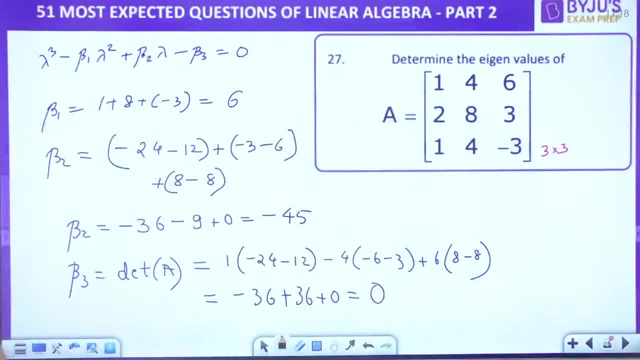 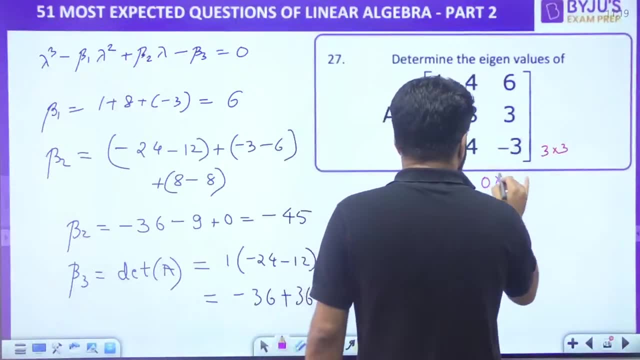 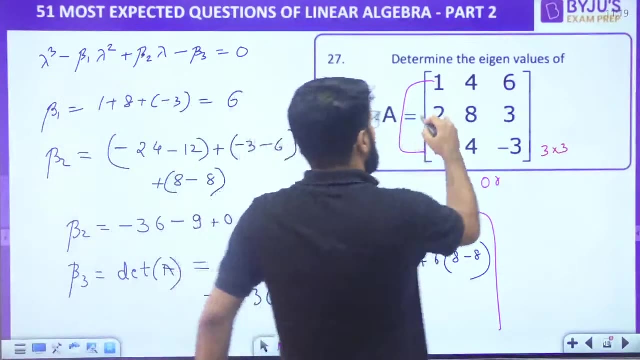 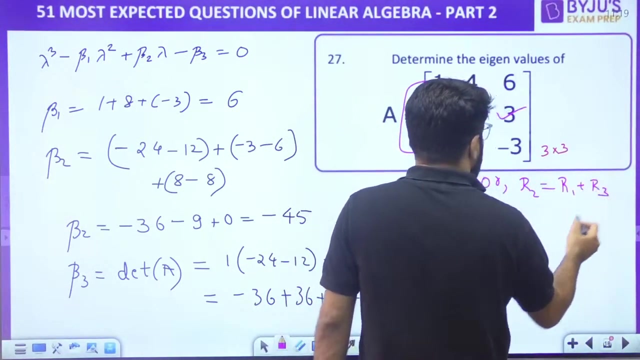 36, last part, is 0. the determinant is 0. determinant is 0, right determinant 0. or you can do like this also when you add these two, when you add these two, 1 plus 1, 2, 4 plus 4, 8, 6 plus minus 3, 3, so r2 can be written as r1 plus r3. dependent rows. 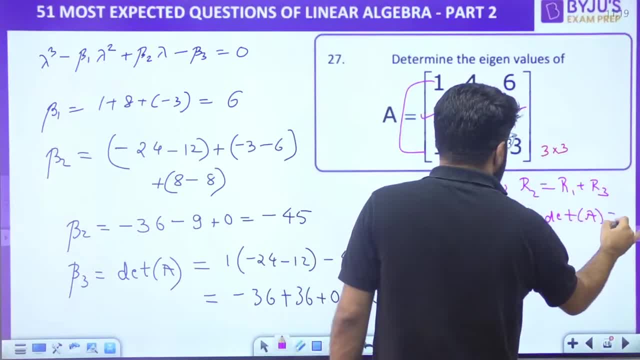 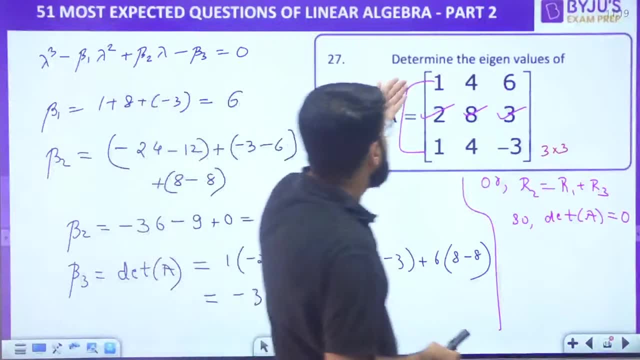 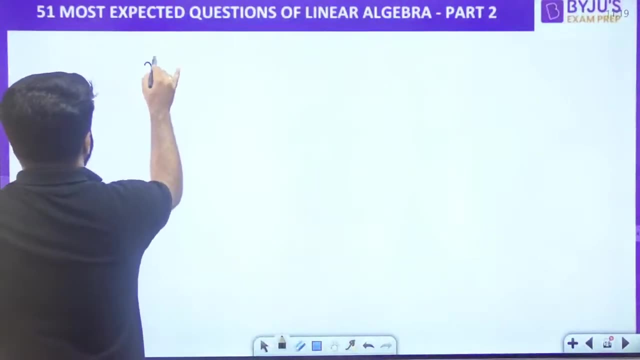 whenever you have dependent rows, determinant is always 0, one of the basic property of determinant. when the rows are dependent, the determinant will be 0. anyways, anyways, the determinant is 0. now, let's put down in that characteristic equation, dear. let us put down in that characteristic 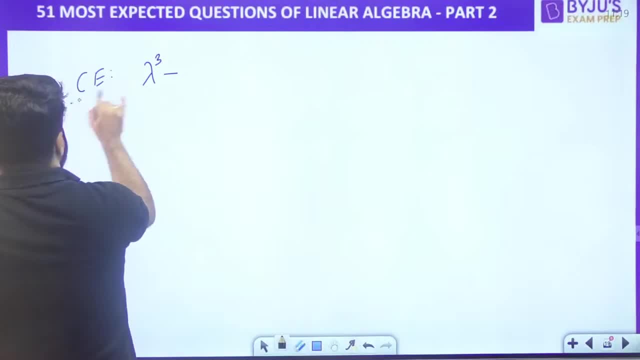 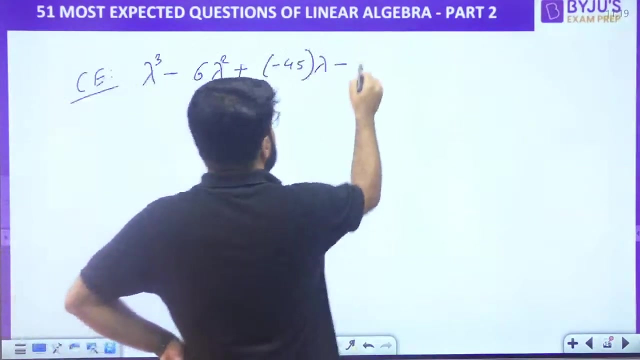 equation: lambda square minus beta 1: lambda square, sir. what is the beta 1? beta 1, beta 1: 6, the minus 6. lambda square plus beta 2. lambda beta 2 is minus 45, minus beta 3, but beta 3 is 0 and that is why it makes the problem simple: lambda will be common. 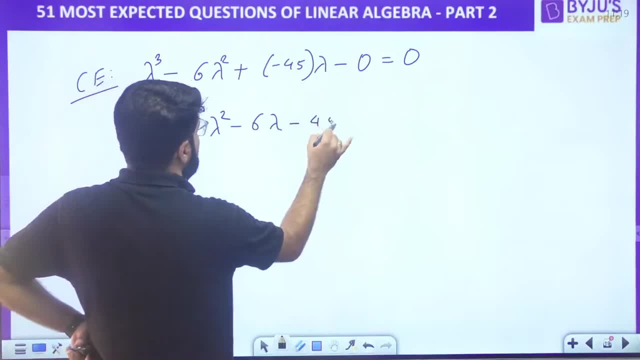 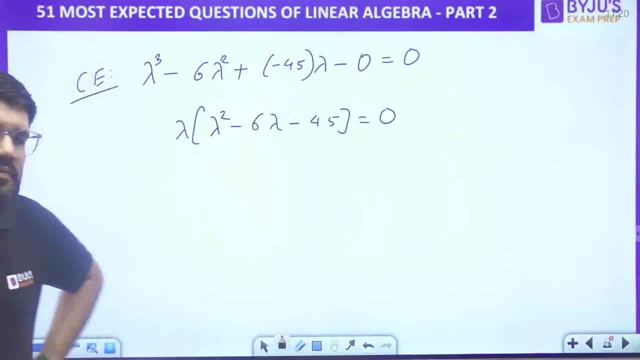 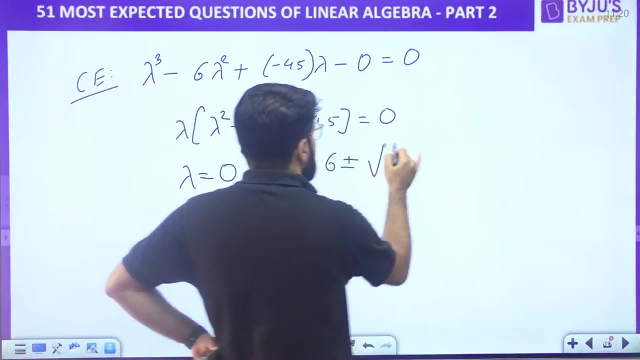 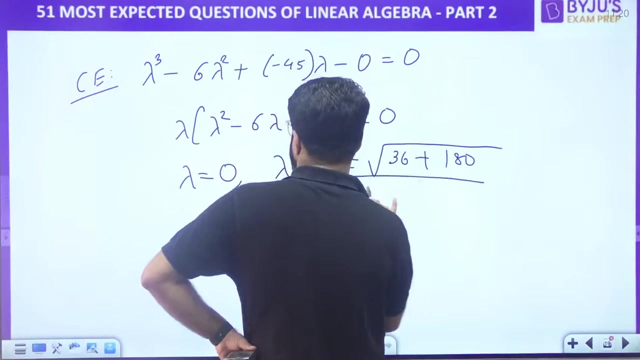 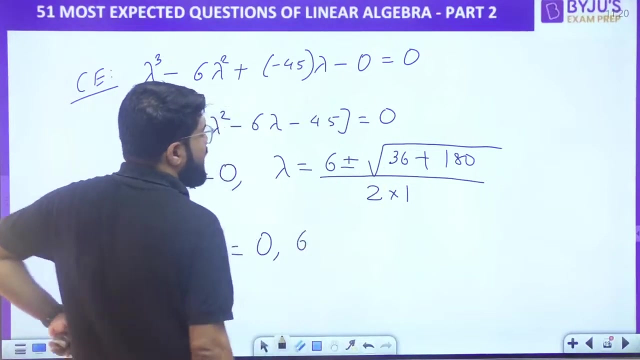 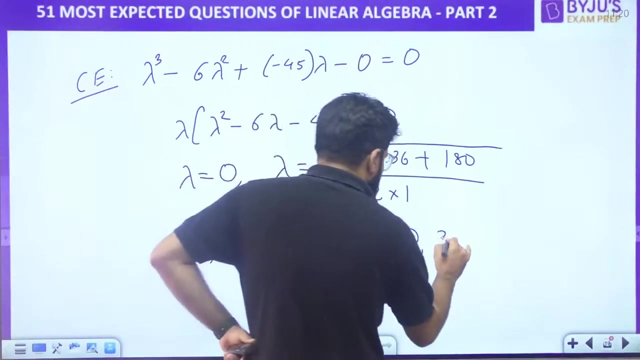 you are left with quadratic lambda square minus 6. lambda minus 45, equal to the 0. good morning, tushar. you, yes, what should be lambda. lambda is 0, or it is equal to 6 plus minus under root of 6 square. that is 36 minus 4, ac minus minus plus 45 into 4, 180 divided by 2a right. so lambda is either 0, 6 plus minus under root of 216, is 6 cube, and actually, though, under root link is 6 root 6, so 6 plus minus 6. root 6 by 2 or lambda is 0, 3 plus 3. root 6 is 6 cube, and actually so under root link is 6. root 6, so 6 plus minus 6. root 6 by 2 or lambda is 0, 3 plus 3. root 6 is 6 cube, and actually so under root link is 6. root 6, so 6 plus minus 6. root 6 by 2 or lambda is 0, 3 plus 3. root 6 is 6 cube, and actually so under root link is 6. root 6, so 6 plus minus 6. root 6 by 2 or lambda is 0, 3 plus 3. root 6 is 6 cube, and actually so under root link is 6. root 6, so 6 plus minus 6. root 6 is 6 cube, and actually so under root link is 6 root 6, so 6 plus minus 6. root 6 by 2, or lambda, is. 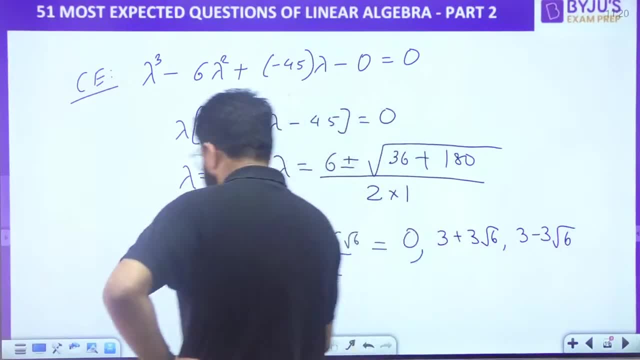 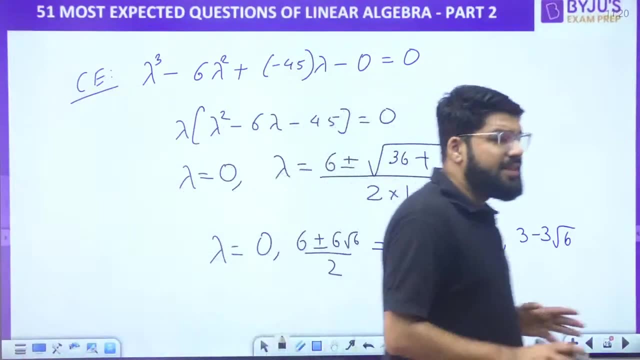 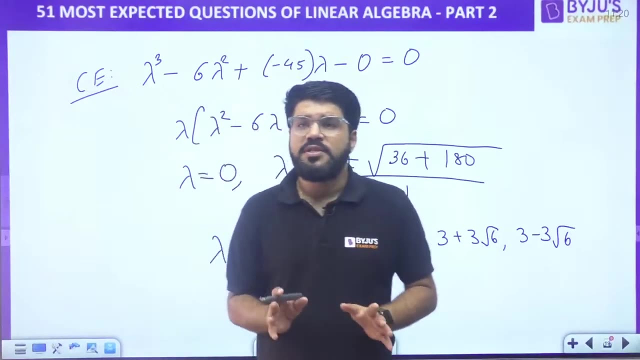 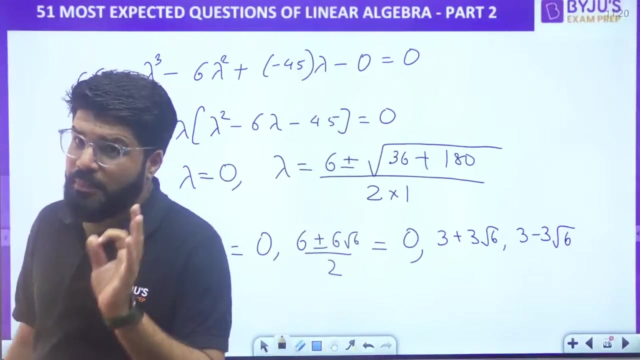 6, 3 minus 3 root 6, 3 plus 3 root 6, 3 minus 3 root 6. now the important point is important point is: in these days, in these days in the gate, scientific calculators are not allowed. and I have been telling you consistently: never use the scientific calculator for your practice. right, it is just a spoiler, it is just a party spoiler. your preparation spoiler actually: always stick to the virtual calculator, always stick to the virtual calculator, always stick to the virtual calculator. 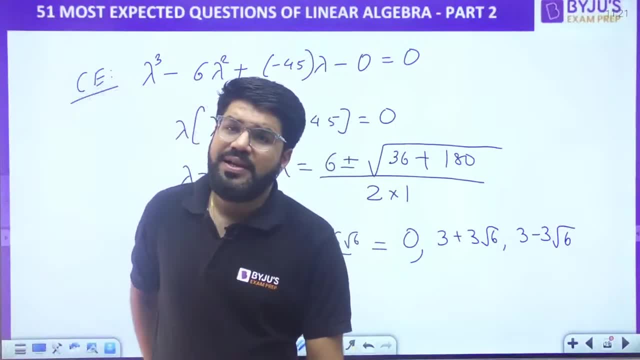 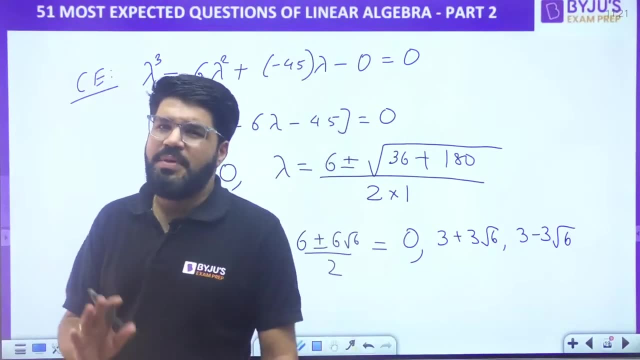 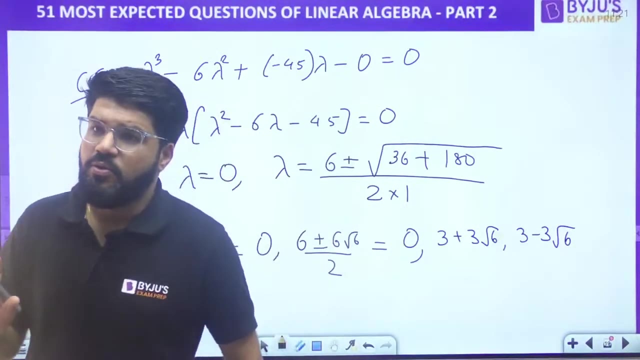 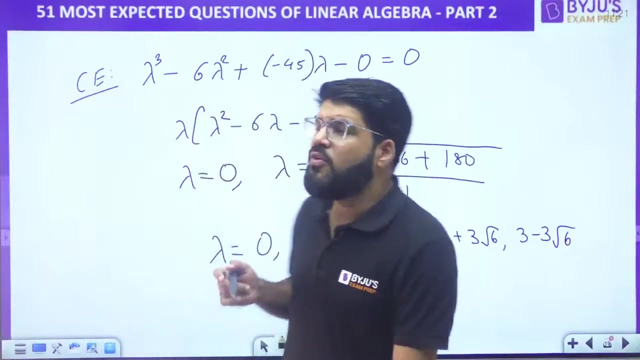 for gate right, always stick to the virtual calculator, see all the features. and if you are accustomed with all the features of virtual calculator, okay, then it is easy. only it has memory features. it has several things, don't worry, okay. but whatever it is, that is the only tool in the gate exam. so you should practice on that, without any doubt. 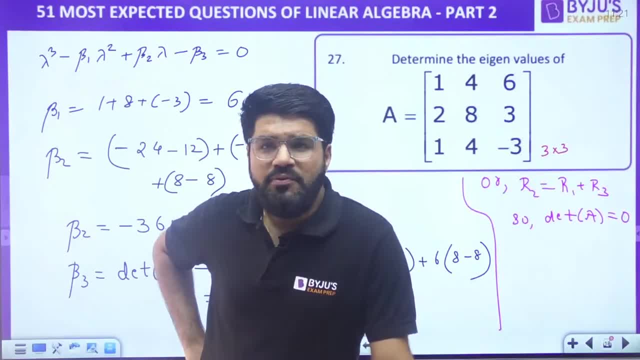 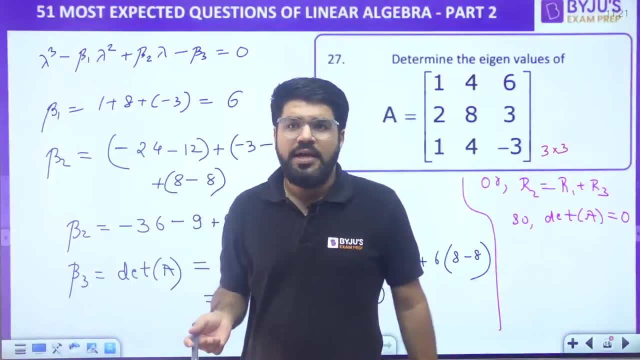 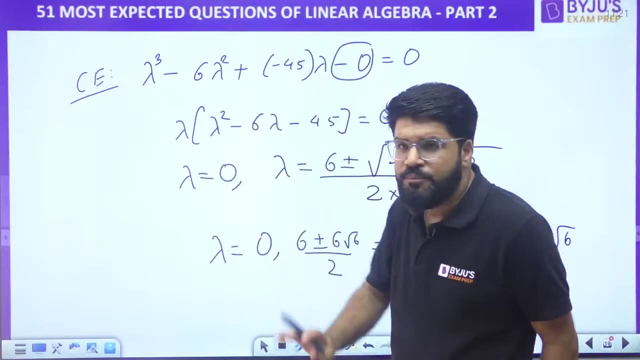 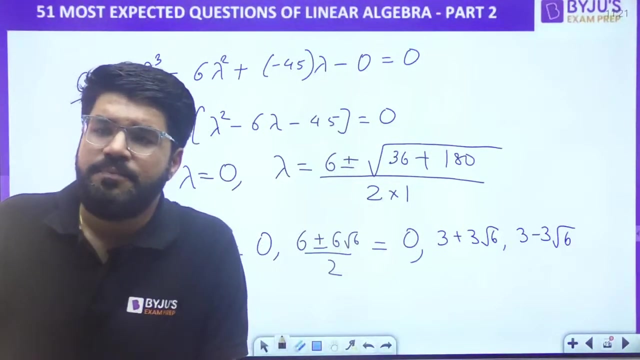 clearly IIT knows what tool they have allowed what type of question to make right. they were never. they will never, ever make a question where they have given a cubic equation to solve without calculator. see what happened here is if this is a type of question. beta 3 went 0, so ultimately, lambda common, you get quadratic. quadratic has the formula right. they will never make the question which will involve you in unnecessary time wasting. they will make the question on the concepts and on your logic, not on unnecessary wastage. 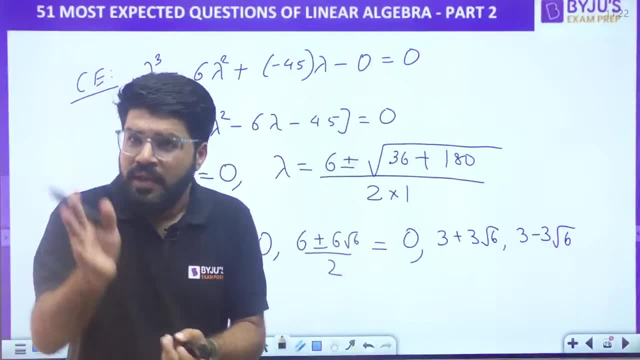 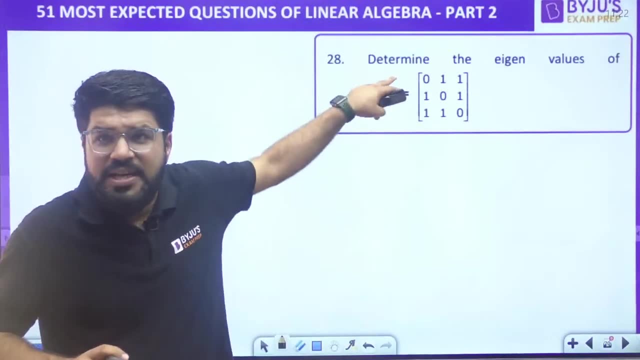 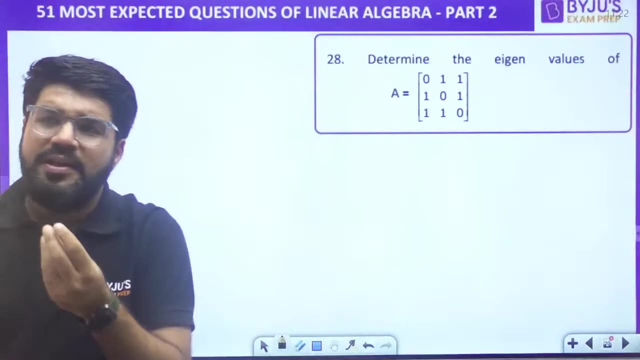 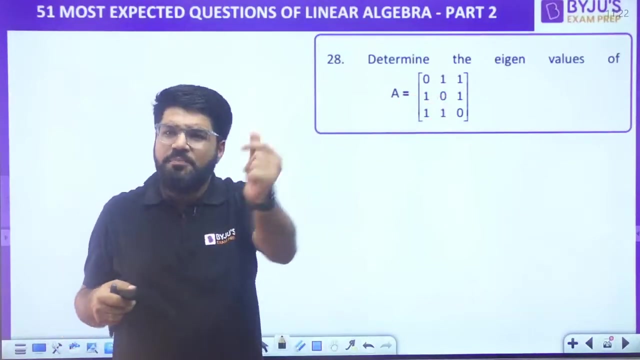 not come, it is converted to quadratic or, worst case, if it comes, a core question, they worst case if it comes. worst case if it comes, it will be a type of equation which I am going to show you right now: the let us see, let us learn some more thing, right, right, yeah, yeah, you can use. we are coming to property, or the only thing is, for any type question and for all range gate, easy. let us first be comfortable with the calculation, then properties are always there. just after one or two questions, properties and then rest. all property based questions need not worry about that. now have a look into this. have a look into 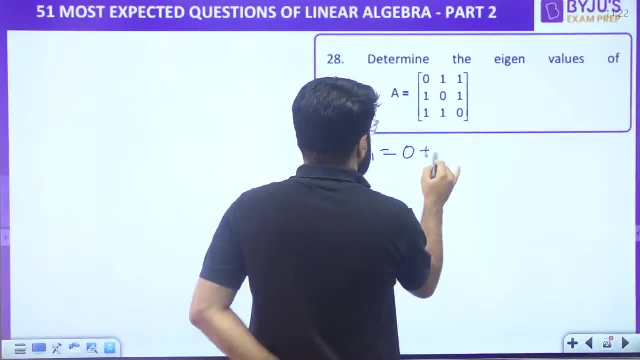 this. let us quickly calculate the numbers: beta 1: 0, 0, 0, that is 0. beta 2 is some of the minus 0 minus 1. quickly, I'm doing the calculation again: 0 minus 1. third, all of mine, or Nikola, that is also 0. 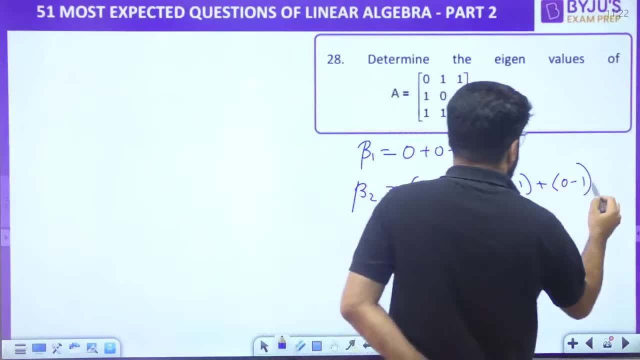 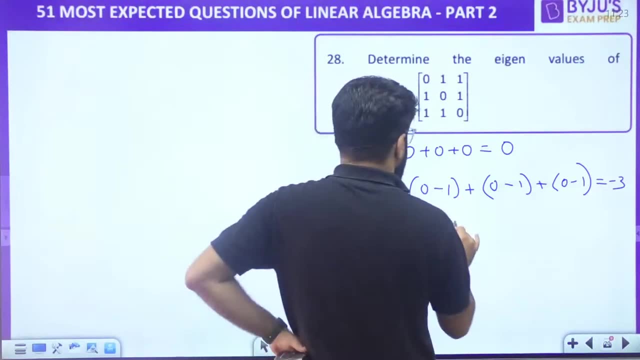 minus 1, so beta 2 is the minus 3. what about the beta 3? so the beta 3 is known as the determinant of a. what is the determinant here? 0. then I am minus 1 into 0 minus 1, plus 1 into 1 minus 0, minus minus plus, so beta 3 is 2. okay, now look here. beta 3 is also non-zero. 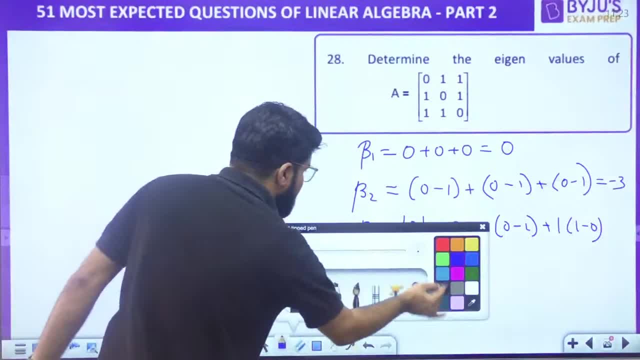 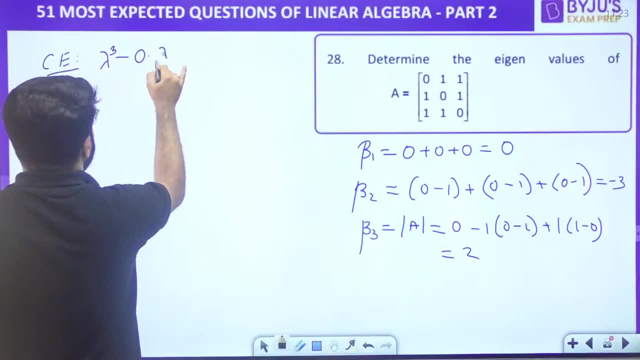 all the coefficients are present. then how will i deal with this cubic equation, right? what is the characteristic equation now? it is lambda cube minus beta 1. lambda square beta 1, 0 plus beta 2 into lambda minus beta 3, equal to 0. lambda cube minus 3. lambda minus 2, equal to 0. now here you. 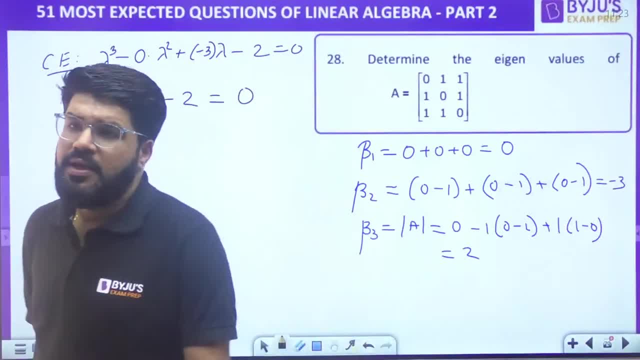 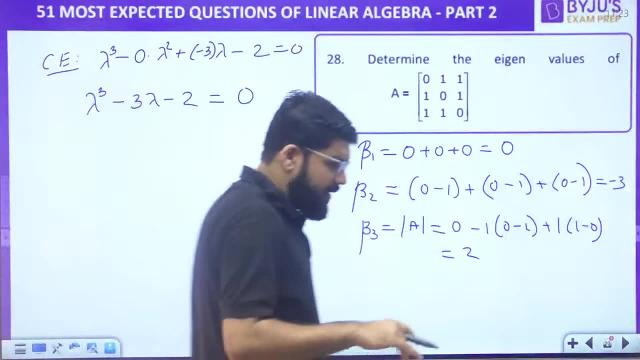 cannot factorize. now, here you cannot, you know, make it into quadratic case. here you cannot make it into quadratic case. so what to do in that case? what to do in that case? and suppose this is a question in gate? scientific calculators are also not allowed. scientific calculators are also not. 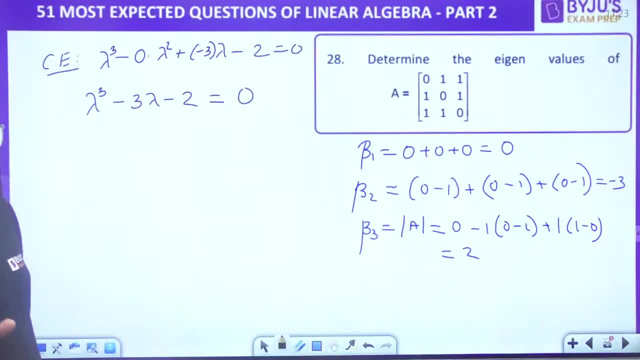 allowed. beta 2 is minus 1. no, no, beta 2 is minus 3, 0 minus 1 akg, it is minus 3. only suppose this is a question in gate. scientific calculators are also not allowed. so what i will try now is lambda cube 3, lambda. little bit of factorization will be tried now. 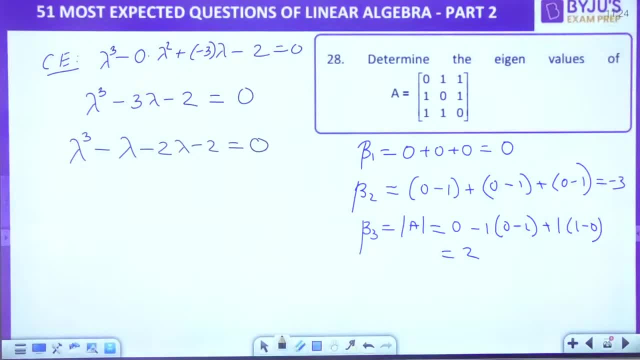 minus. lambda minus 2. lambda minus 2 equal to 0. now, from the first two terms here, take out the lambda common, you have lambda square minus 1. and from the last two terms, take the minus 2 common, you have lambda plus 1. now we all know that lambda square minus 1 is lambda plus 1 lambda. 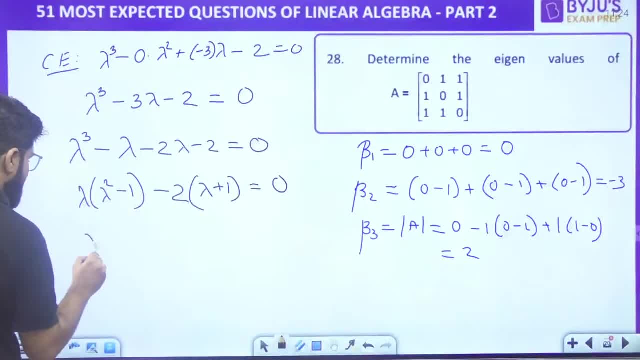 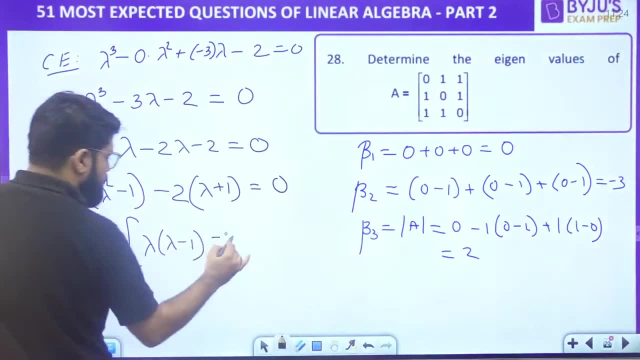 minus 1. so again, i have a factor in common. lambda plus 1 can be taken as common. so i am left with lambda. lambda minus 1. lambda plus 1 is outside minus 2. have a look into this equation now. right, i have lambda plus 1, then lambda square minus. lambda minus 2. 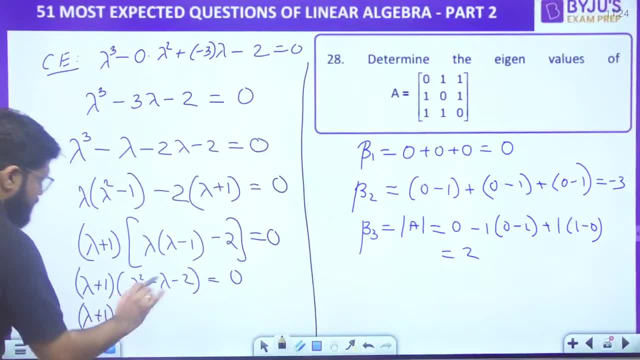 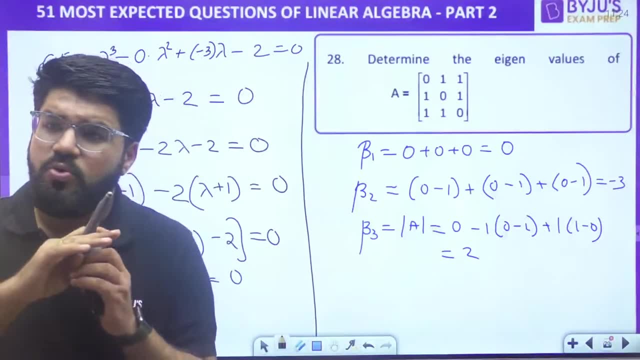 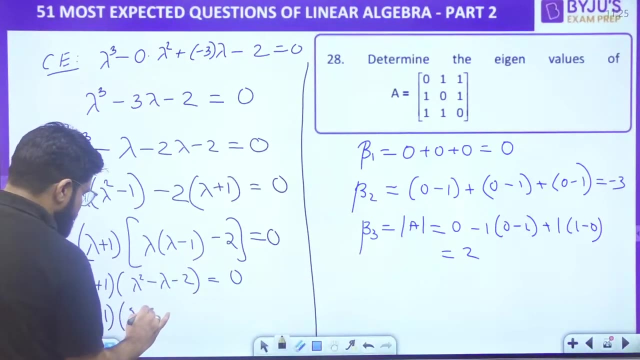 equal to 0, i have lambda plus 1. this can. now it is a quadratic case either you can find the roots, someone product with. i mean, don't worry, first i want you to be comfortable with all calculation, then properties and then tricks. okay, so this is factorizable. sum is minus 1, product minus 2, right, so lambda minus 2, lambda plus 1. 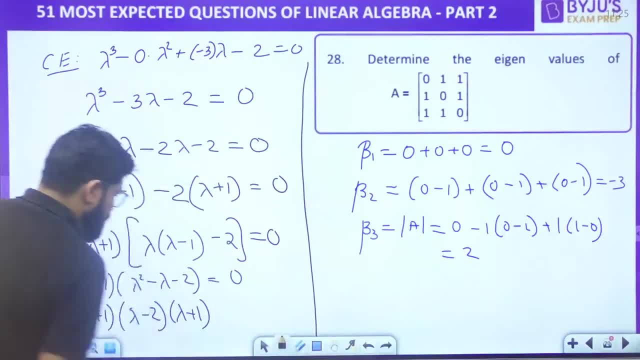 minus 2 plus 1 will become minus 1. minus 2 into 1 will be the minus 2, right, this is equal to 0. so what have you got eventually? lambda plus 1, lambda plus 1. so i get lambda plus 1 square. 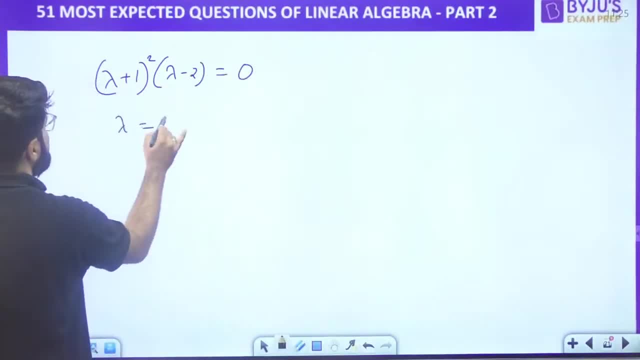 whole, multiplied by lambda minus 2 equal to 0. so lambda is equal to 2 minus 1 minus 1. lambda is equal to 2 minus 1 minus 1. without the need of scientific calculator, i have to calculate what i have solved this. there are the three eigenvalues 2 and minus 1 and minus 1, right dear. 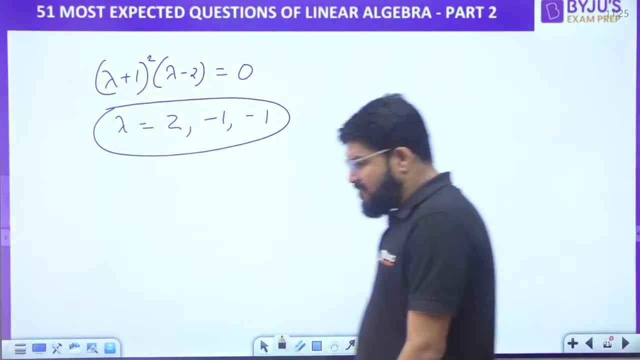 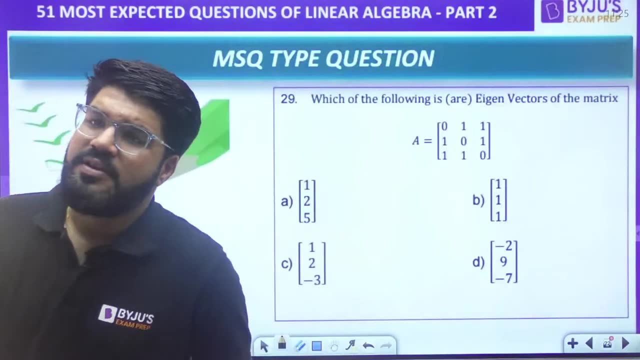 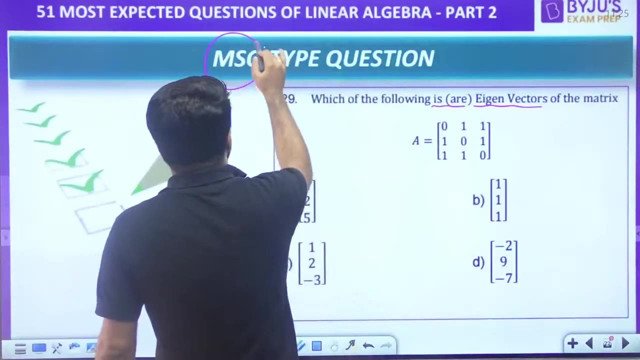 okay, now, before we take up the properties, one more question, and then, after that properties and that question, i am going to take up, with help of, with the with respect to eigenvectors. with respect to the eigenvectors, which of the following is, or are, msq type question? 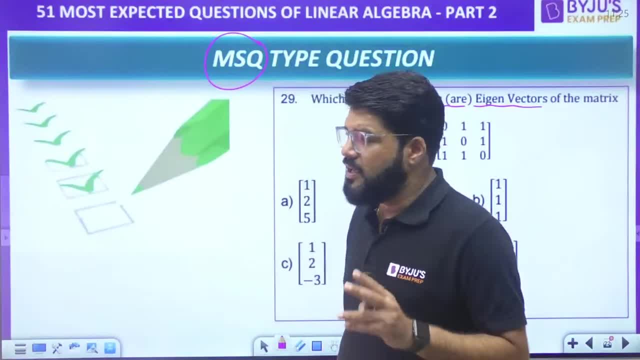 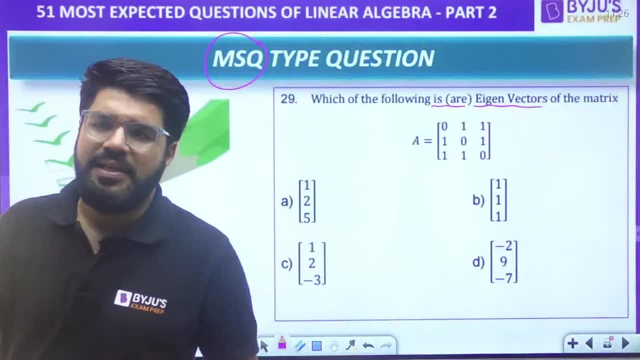 okay and msq type of questions is in this class. we have been seeing quite good number of msq questions in the class 22 exam only we have seen engineering maths producing msq question, quite good number of msq question and there were msq questions from linear algebra also, especially right. 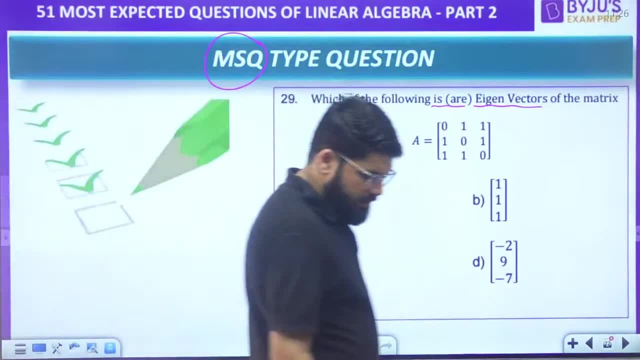 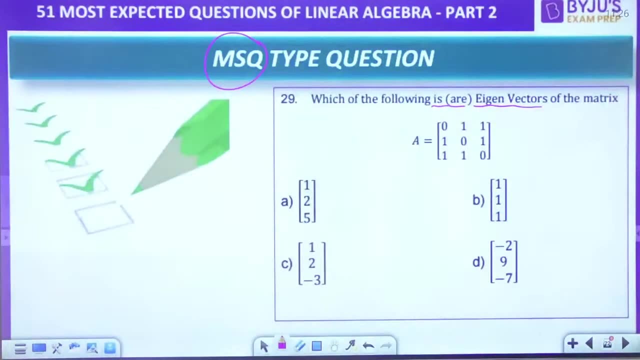 and you know, don't worry, i'm planning some sessions for you also. i'm planning some sessions for you also. okay, that is with respect to msq of the engineering maths, msq, practice of engineering math. so we will do that, but first let us have the normal session so that you learn, and then, after that, msq type of sessions for maths and other. 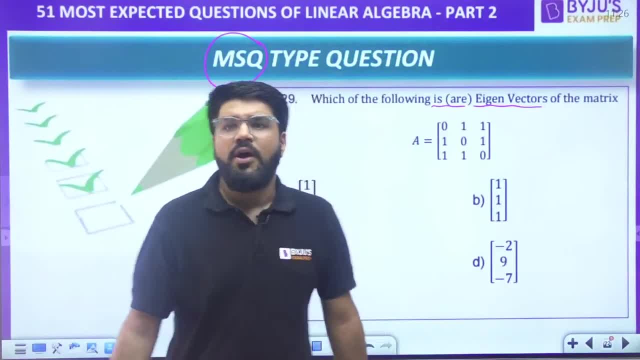 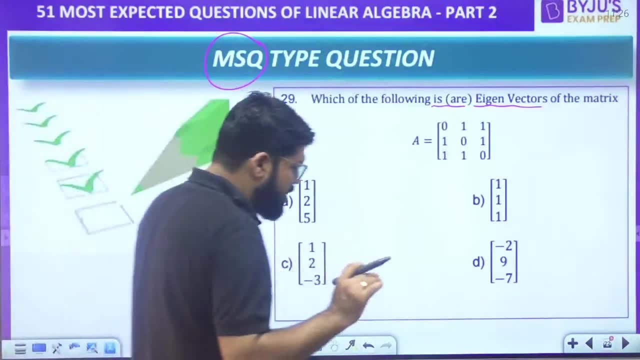 and other subjects also. we will plan for you. Okay Now, how to solve this question. Any question on eigenvector Right, Any value on the eigenvector, Any question on the eigenvector. You don't have to solve it up fully. Same matrix which I have used in the previous question, but you don't have to. 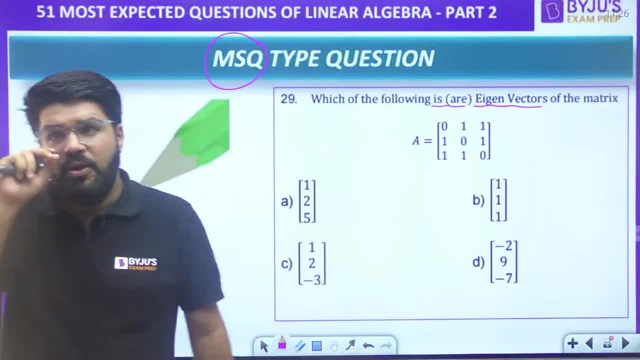 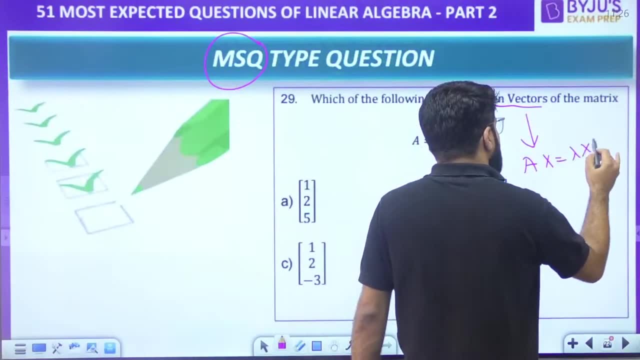 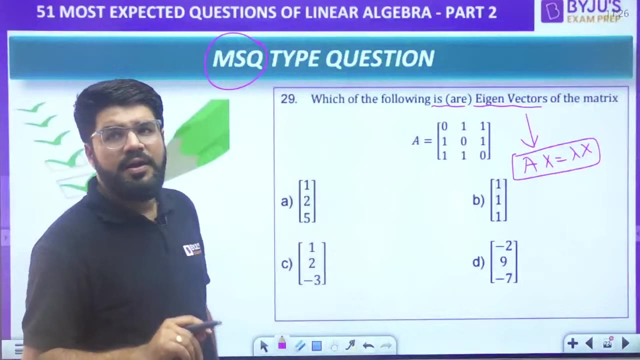 solve it up fully. You don't have to solve it up fully Because Because you should be directly using the definition of the eigenvector. What was the definition in the beginning? I have introduced that definition: Ax equal to lambda x. Ax equal to lambda x. Any type of matrix given Any type. 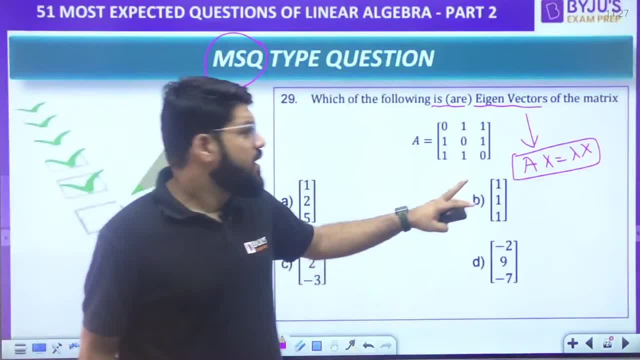 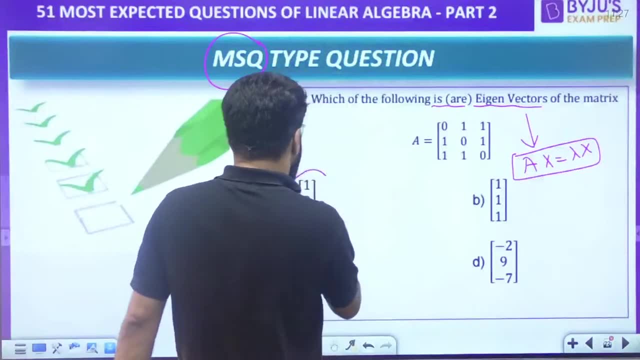 of question. I will take several more questions on eigenvector, But just use ax equal to lambda x to rectify your problems, To rectify your question. So let us start. Any vector, Any of this vector is an eigenvector. If a into x, Multiply this with x, You get answer which is multiple of x. 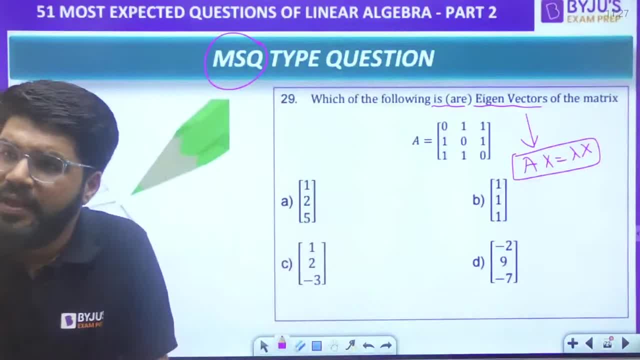 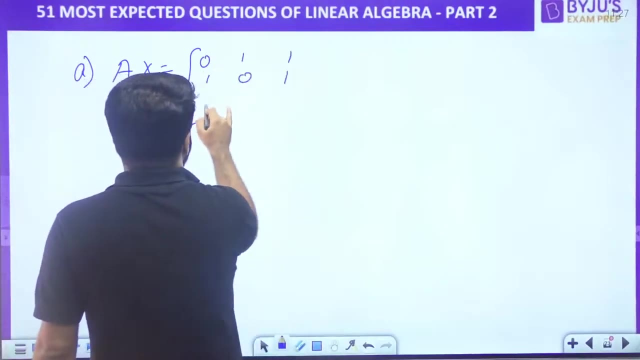 Like 2x, 5x, 10x, 100x, Anything, Anything. Right, Let us try with option no A. Let us try with this calculation part in the option a. What is the option a? Ultimately, you have to do an ax A matrix: 0, 1, 1.. 1, 0, 1.. 1, 1, 0.. Multiplied by x, X of option no A is: 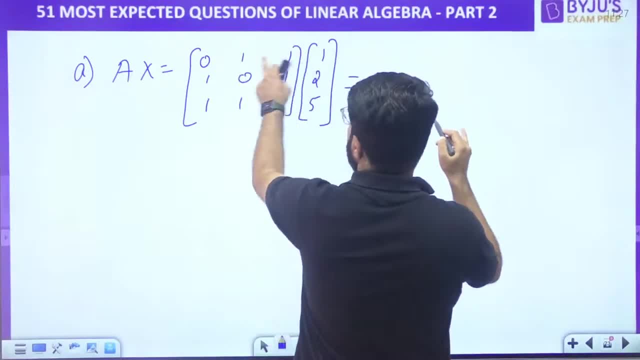 1, 2, 5.. Now multiply: First row, First column: 0, 2, 5, 7.. Next 1, 0, 5.. But in 5, 6.. Next is 1, 2, 0.. That is 3.. 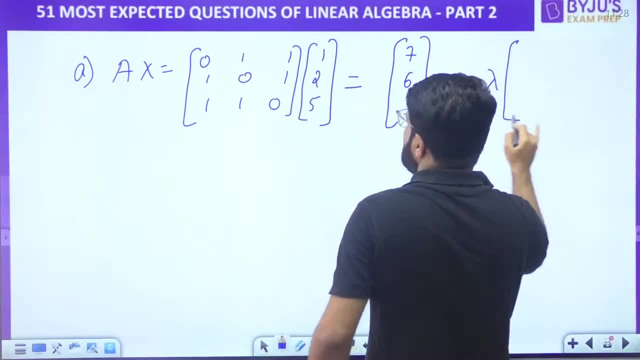 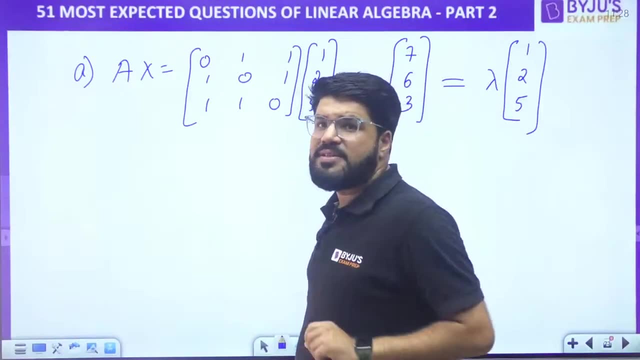 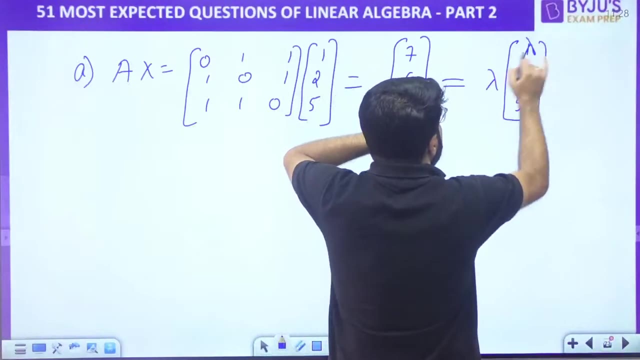 now in any case, can you write it as lambda into x. x is 1 to 5. can you find out any common lambda such that you can write it as lambda x? think about this. suppose suppose they are equal. suppose they are equal. so if they are equal, multiply lambda inside. this becomes lambda, so lambda should be. 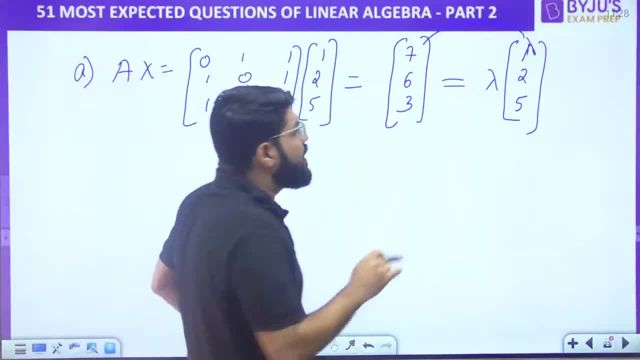 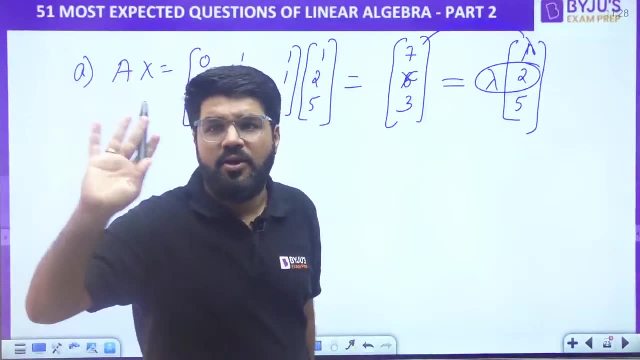 the 7, but if the lambda is 7, but if the lambda is 7, what should be the 2 lambda? 2 lambda should be 14, and this is not 14. but love they are. they cannot be equal. they cannot be equal. this is not. 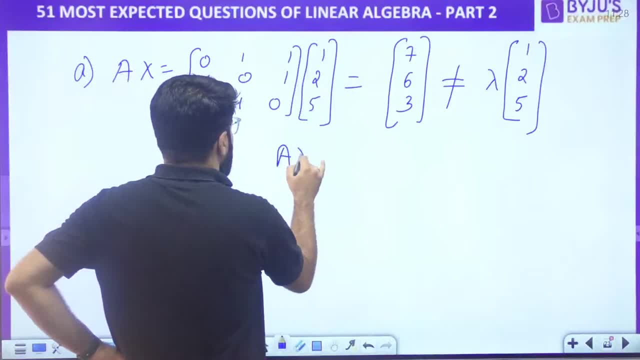 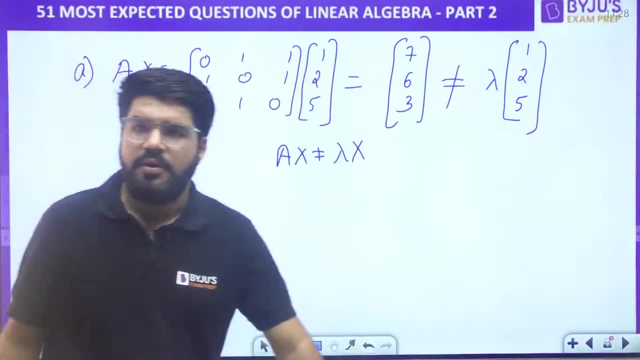 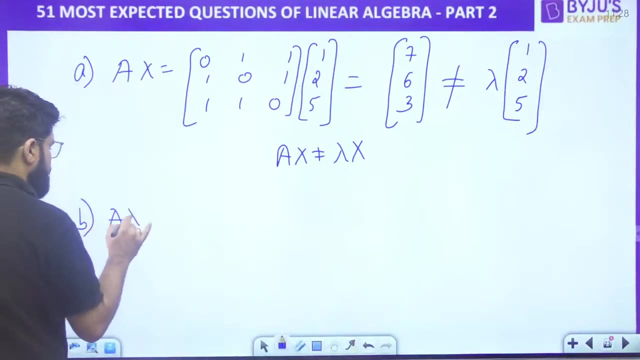 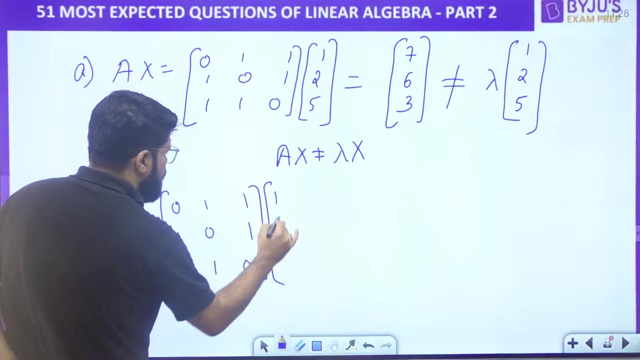 equal to lambda X. here a X does not equal to lambda X. okay, no problem, let us try the option number B. let us try the option number B. 1 1, 1 is the option number B. again, a into X, and option number B has the vector one. one one. now everybody multiply. first row, first column. 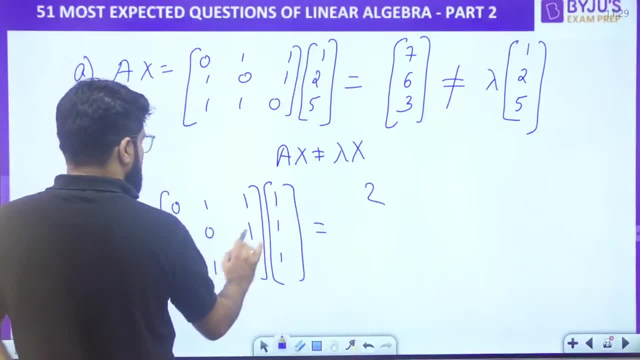 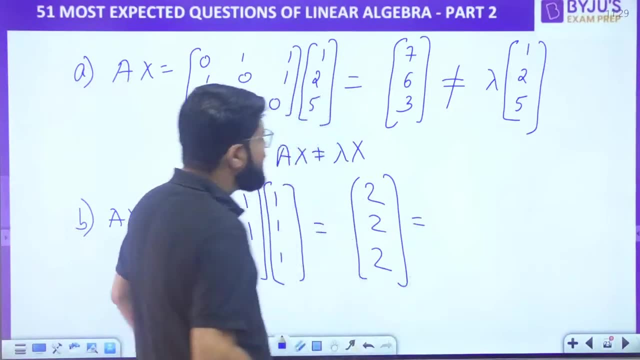 0 plus 1 plus 1, that is two. one zero one, that is again two. one plus one plus zero, that is again two. so clearly I can take the two common here. clearly I can take the two common and this becomes one one one. clearly I can take the two common and this becomes one one one. dear right you give. 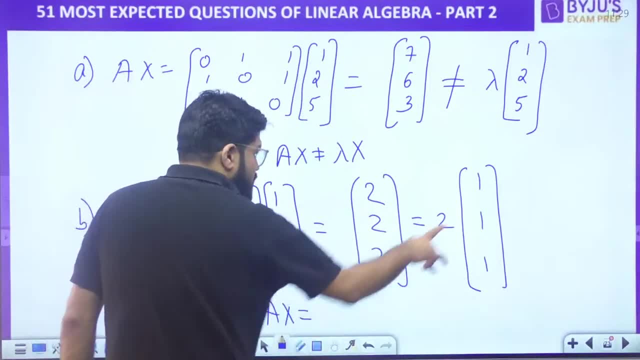 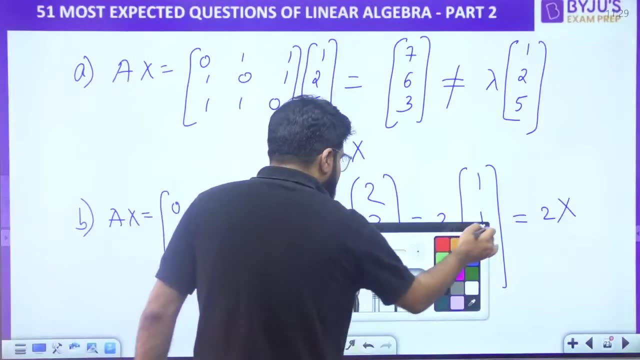 one, one, one now. well, clearly, a into x is what is 1? 1? 1? it is again the x. so a into x is 2x. so this is the correct eigenvector, with the lambda equal to 2. they have not asked the eigenvalue, but yeah, this is the. 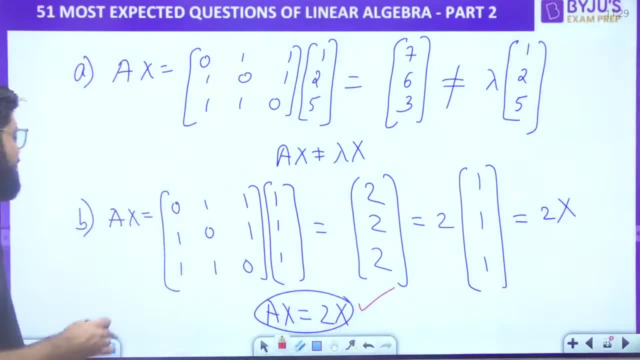 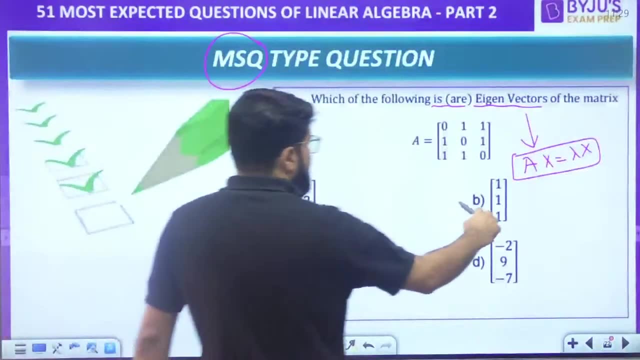 correct eigenvector with the lambda equal to 2, even if they ask what is the eigenvalue corresponding to this vector. the eigenvalue is 2, but so b is one of the correct answer. okay, but it's a msq question. we can't stop here. if it was mcq, we can stop. it is msq, right. so we need to try that is. 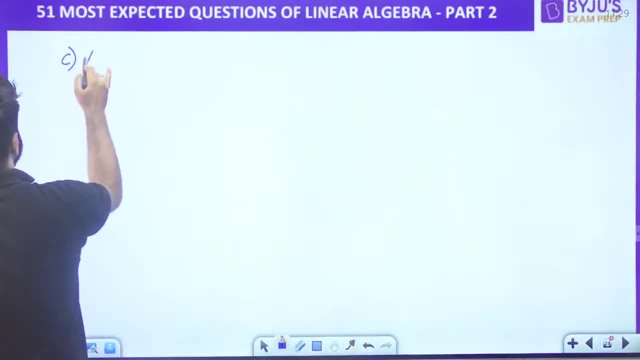 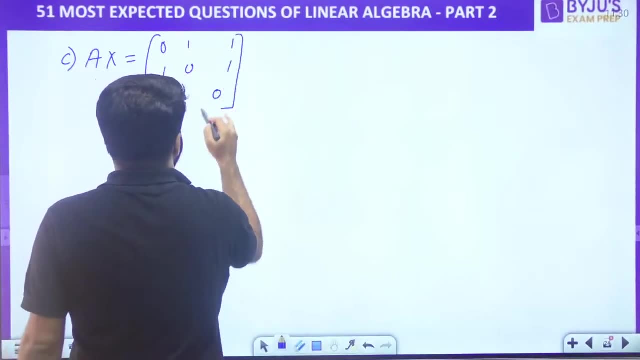 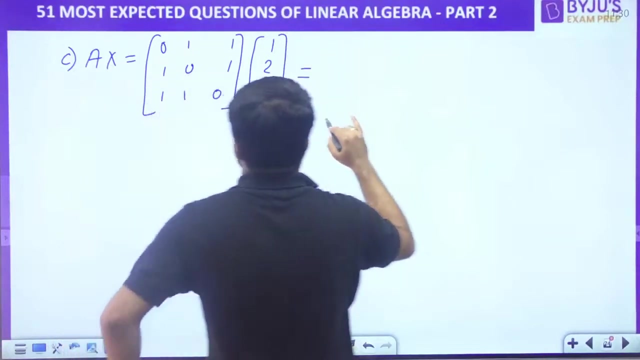 what msq may have to time. so let us try the option number c also, and let's try ax. what is the x? 1, 2 minus 3, multiply 0, 2 and minus 3, so minus 1, then 1, 0, minus 3, that is minus 2. 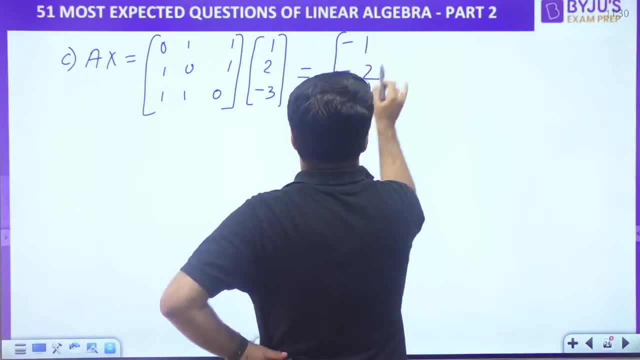 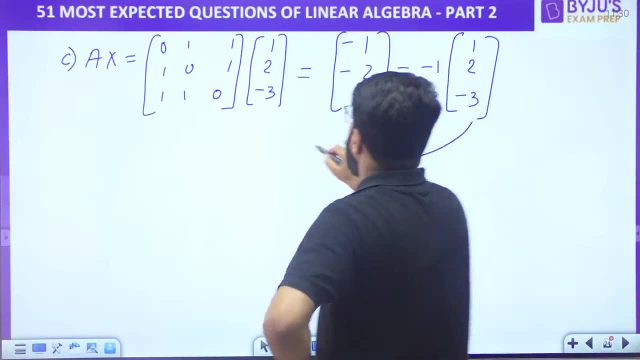 then 1 plus 2 plus 0, that is 3 already here, very clearly, take the minus 1 common, take the minus 1 common. you are there with 1, 2 minus 3 and that is again equal to x. that is again equal to the x, right? 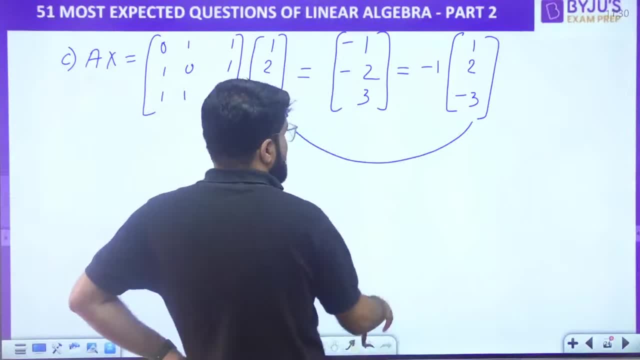 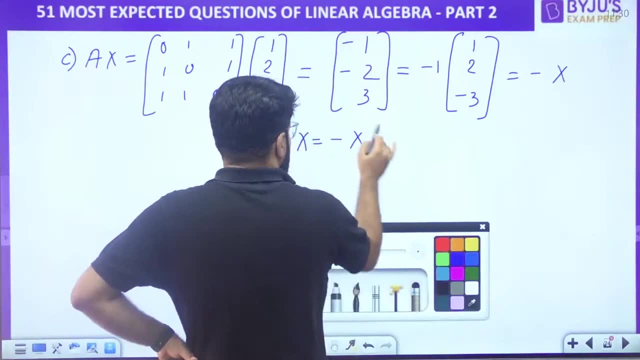 that is again equal to the x. so this is equal to minus of x. so here, ax equal to minus x, no problem, lambda can be negative also, but this is the correct eigenvector relation. whenever ax equal to minus x, you are there with 1, 2 minus 3 and that is again. 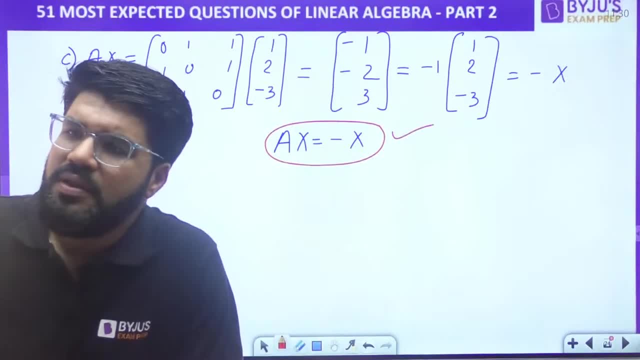 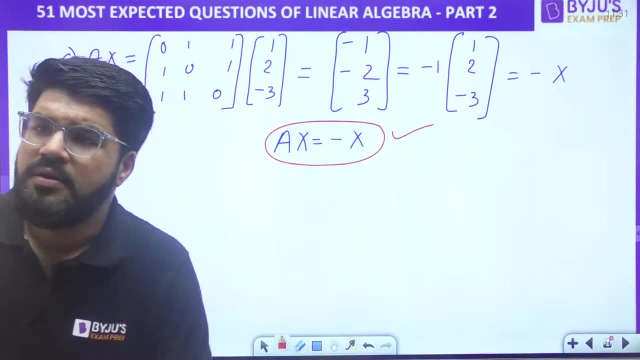 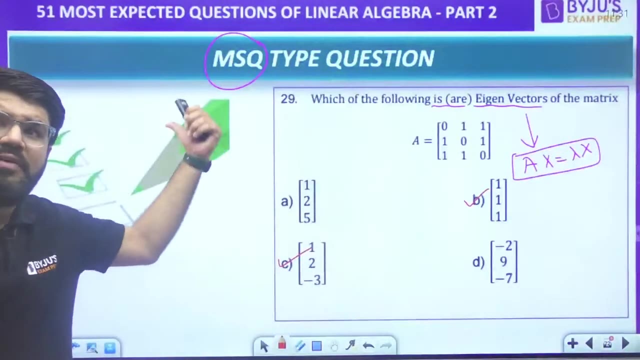 equal to lambda x. it is eigenvector last eigenvalue. which which last eigenvalue? no, without calculating eigenvalue. so we are not eigenvalue automatically coming. i am not putting any extra effort to calculate eigenvalue, don't worry, we don't have to solve eigenvalue like 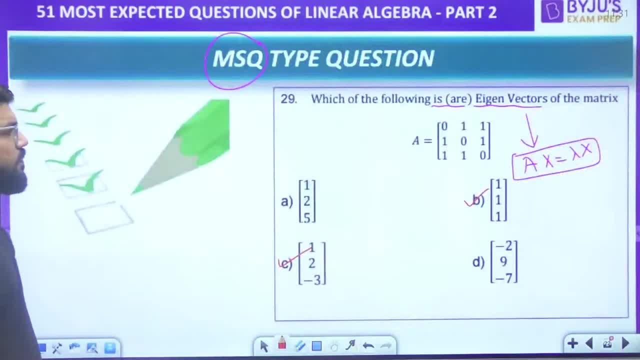 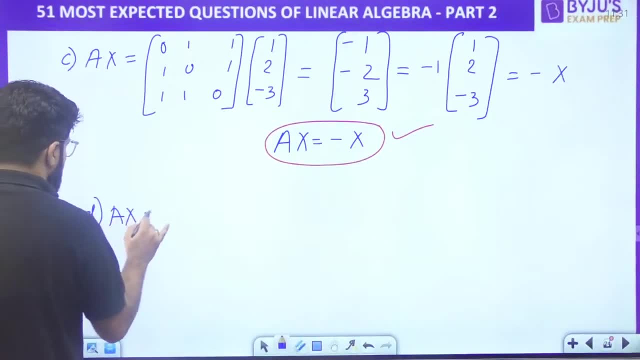 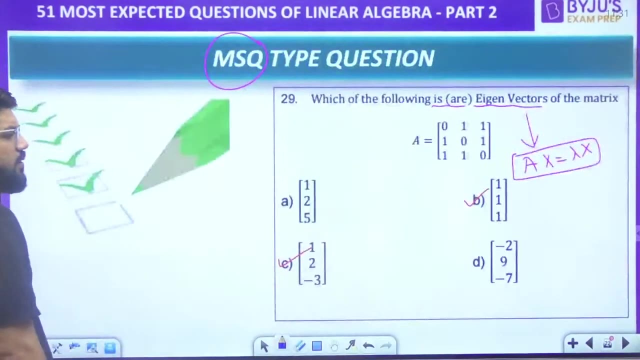 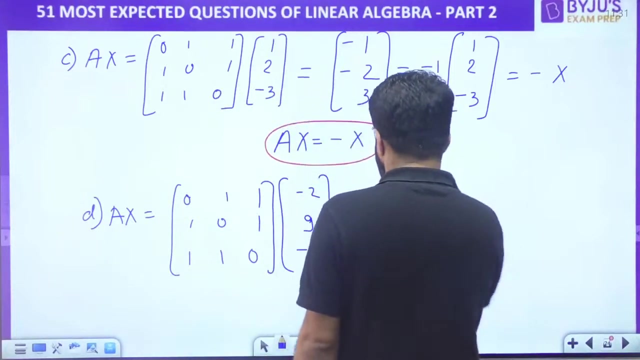 the previous question. right now, let's say the option number d also. let us try the option number d also very quickly: multiplied by what is the option number d minus 2, 9 minus 7, that is equal to 0, 9 minus 7, which are minus 2, right 9, and. 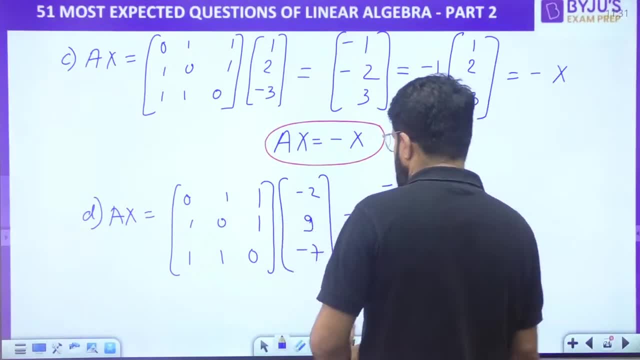 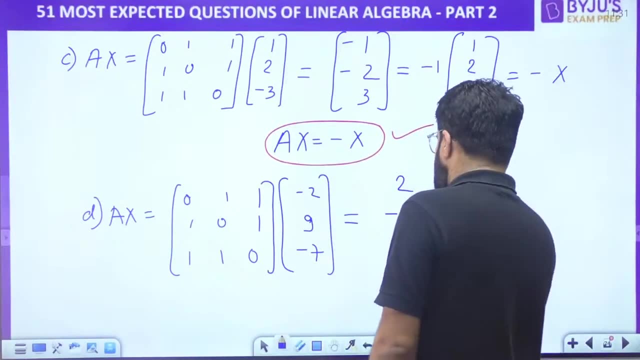 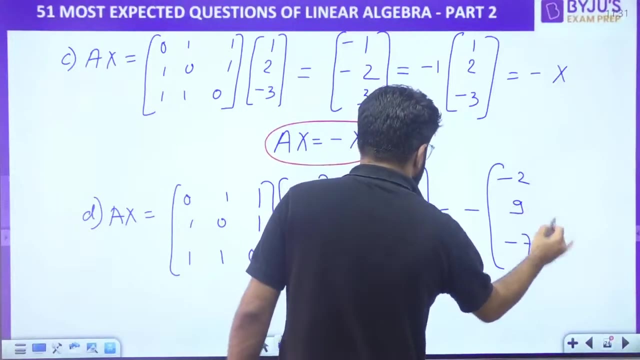 0, 9 minus 7, correct 9 and minus 7, that is plus 2. actually, next is minus 2 and minus 7 minus 9. next is minus 2 plus 9, that is 7. once again, dear, once again, take out the minus common, you get minus 2 plus 9, minus 7, and that is what is the given. 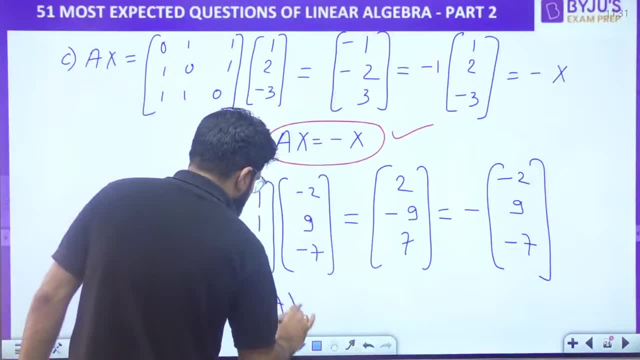 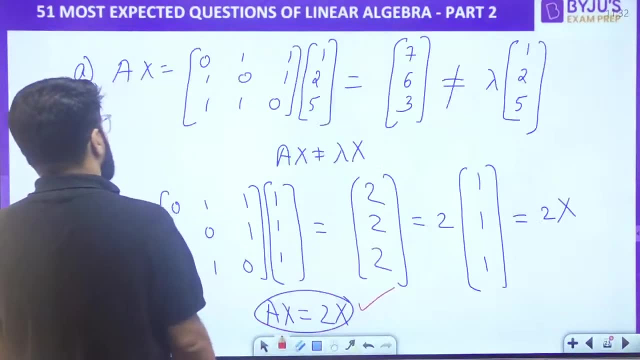 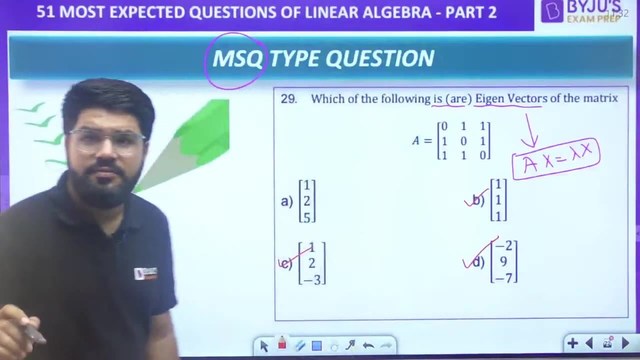 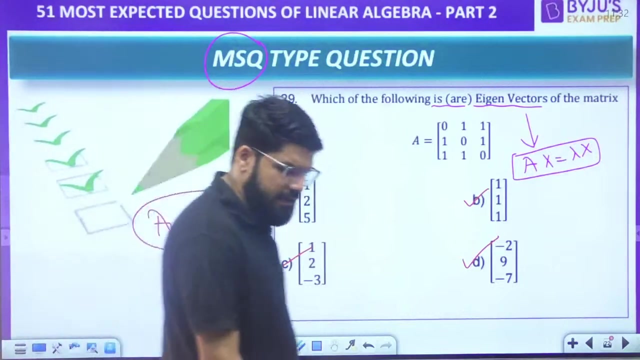 vector. so once again, ax is minus x. so this is also correct eigenvector with lambda equal to minus 1. but i don't want that lambda, i just want to tick mark the correct option. the correct answer for the multiple select question here is: correct answer for this multiple select question is b, c, d. 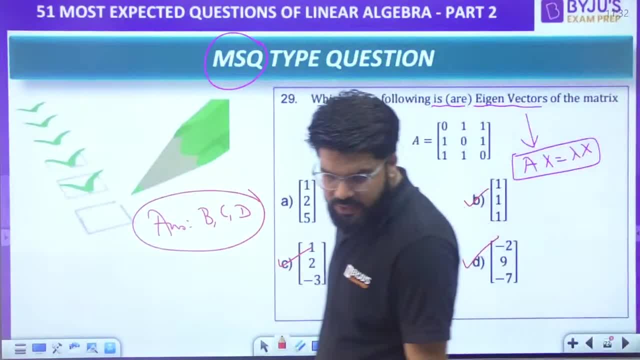 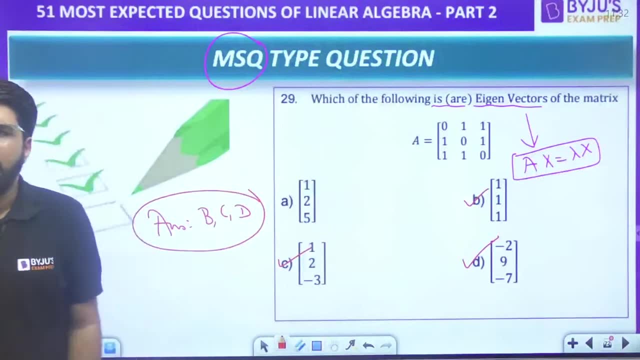 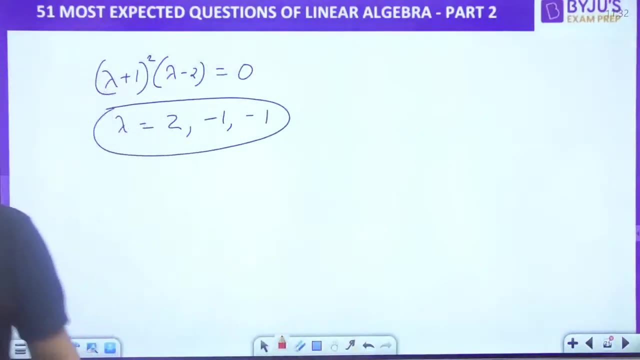 the correct answer here for the multiple select question is the b c d everybody. okay, it is the b c d. now, if i look into any of the previous question, suppose 2 minus 1 and minus 1. eigenvalue- eigenvalue- what came here? 2. 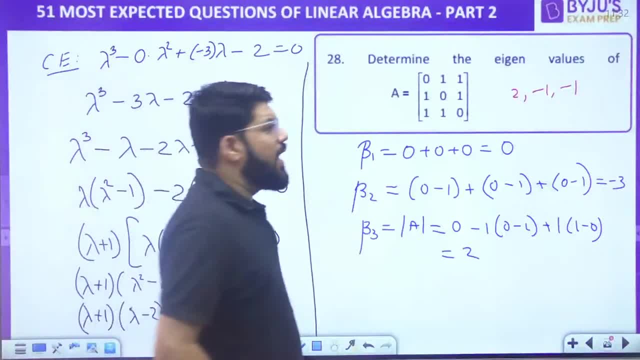 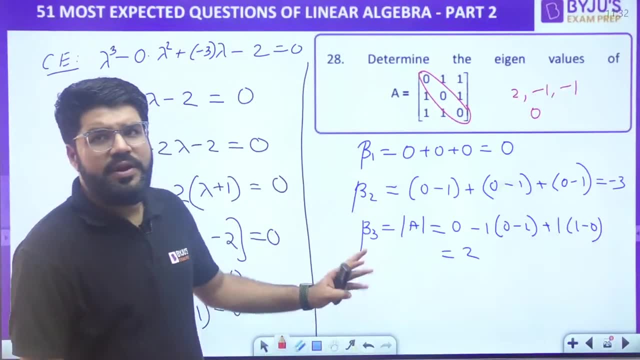 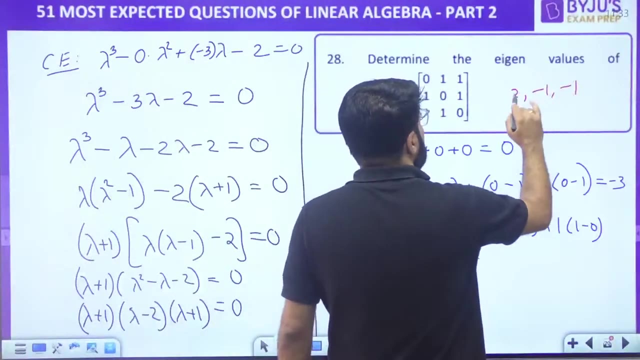 minus 1. minus 1. add all the eigenvalues, dear. add all the eigenvalues, you get zero. what is the trace? that is also zero. add all the eigenvalues, you get zero. trace is also zero. although we have solved, now let us come to the properties and simple techniques. right, multiply all of them 2 into. 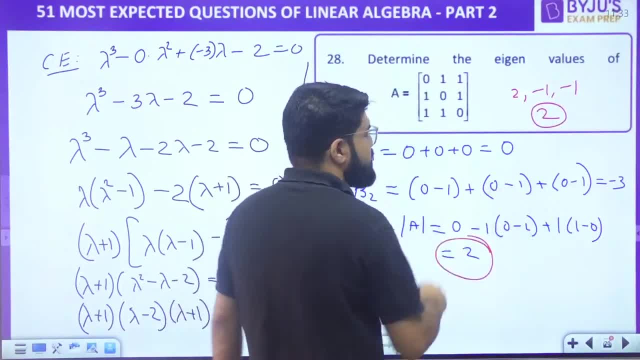 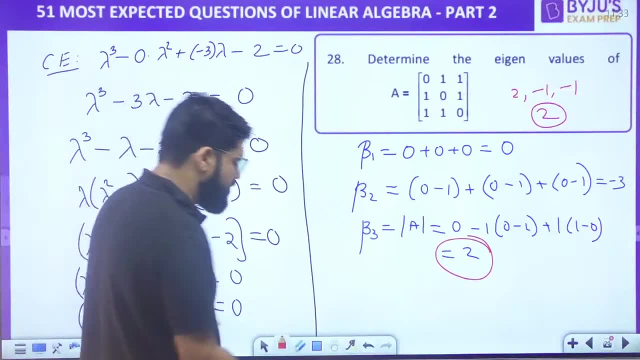 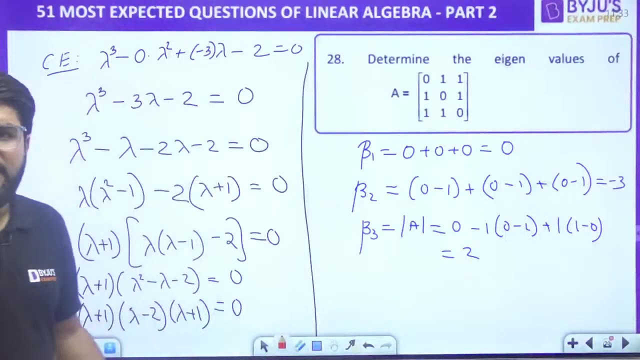 minus 1 into minus 1 minus minus plus, so it is plus 2. the determinant is plus 2. you can see with the previous question also. you can check with the previous question also, dear, you can check in the previous question also. okay, so there are some very, very important and common properties of the eigenvalues and eigenvectors. 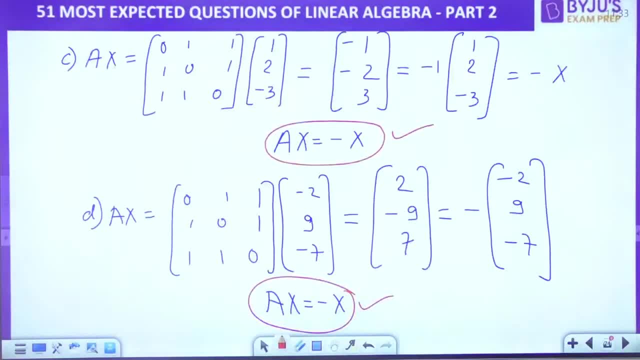 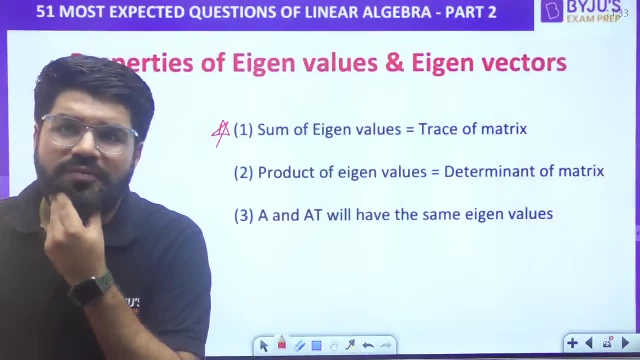 which you must remember. let us go through them also. this was the question number 29. and now: sum of eigenvalues is equal to the trace of the matrix. very powerful property which will simplify most of the questions. many of the questions can get over here. right, product of eigenvalues is always equal. 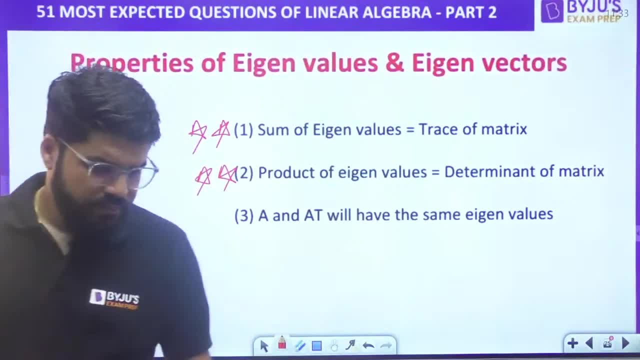 to determinant of the matrix. these two are the most important properties. product of eigenvalues is equal to determinant of the matrix. A and A transposed will have the same eigenvalue. just keep noting: matrix and its transpose will have the same eigenvalue. this doesn't change anything the rank of a matrix. now this is. 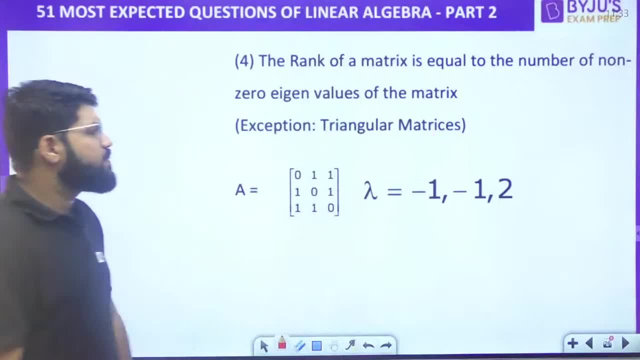 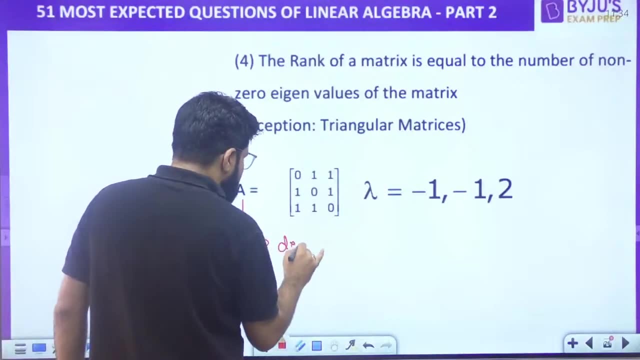 a property in which the triangular matrixes can leave the chart. the exception is the triangular, but for any other matrix? now have a look in to this matrix, this matrix. what was the determinant of this matrix? same previous question I have taken. determinant was equal to 2 right. yes, 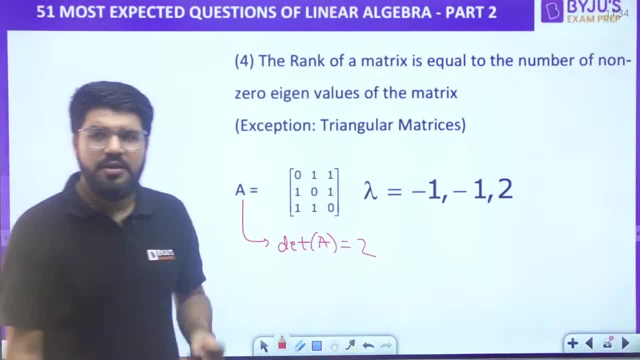 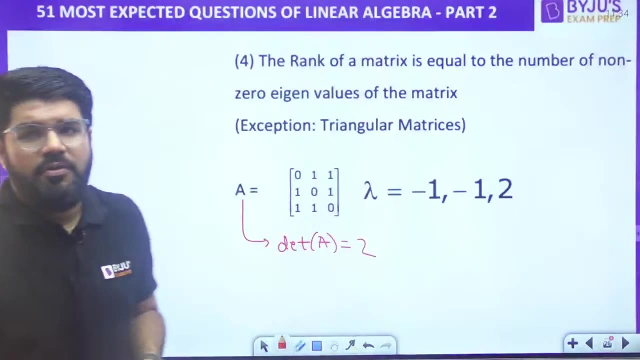 first and second, many questions are solved. solved, okay, say the doubts, akansha, if you have, because this is a review, review and question session. so, accordingly, thoda bhat speed rakhenge. but you have any doubts, please let me know. okay, this is not one of the session where i just want to take it from the very basic, because 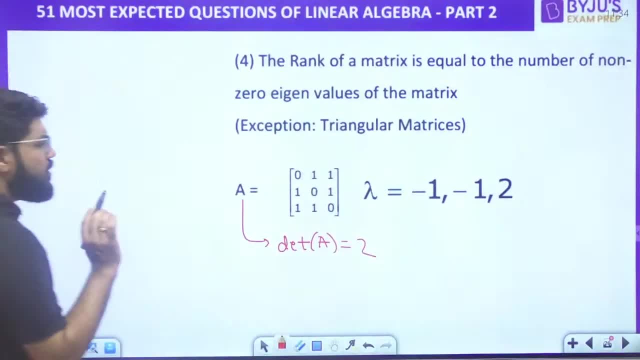 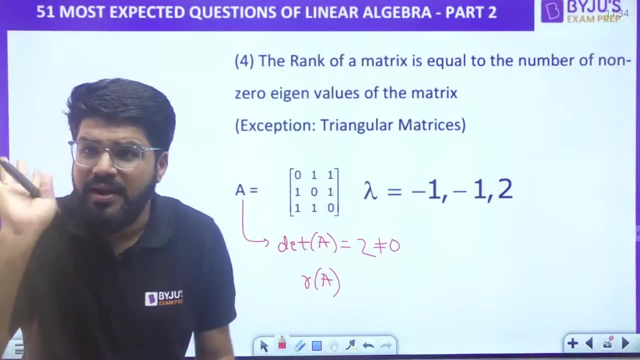 otherwise it will take the whole day. but you're open for any doubts. determinant 2: hai now, determinant of the matrix is non-zero. if the determinant of a square matrix is non-zero, then it should have the full rank. if the determinant of a matrix is non-zero, it should have the full rank. 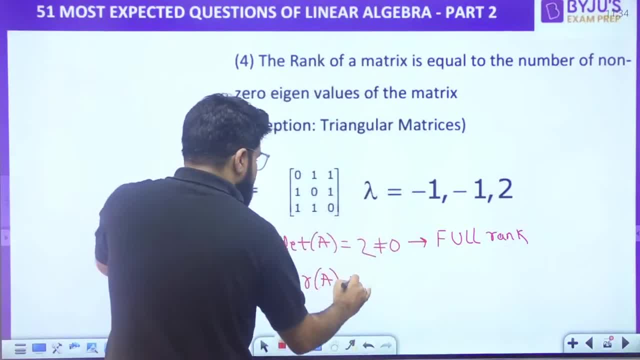 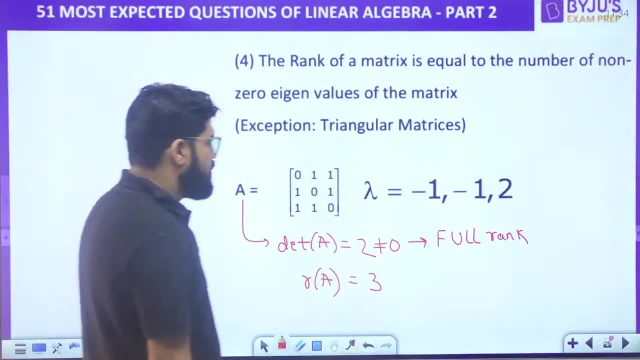 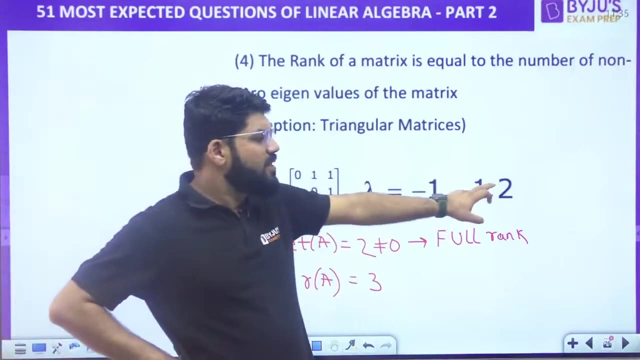 what is the full rank for a 3 cross 3 matrix? for a 3 cross 3 matrix, dear, the full rank is equal to 3. the full rank is 3. right now the rank of a matrix is equal to number of non-zero eigenvalues. now count the number of non-zero eigenvalues minus 1. minus 1, 2. all three are. 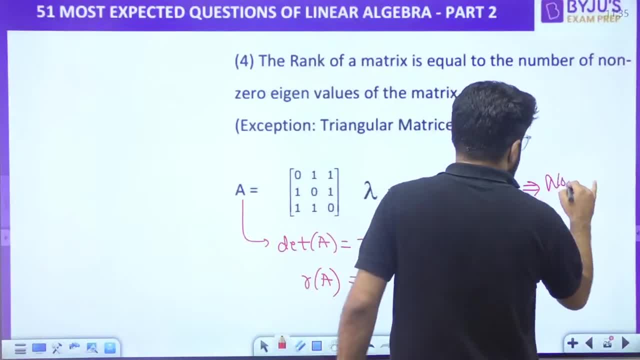 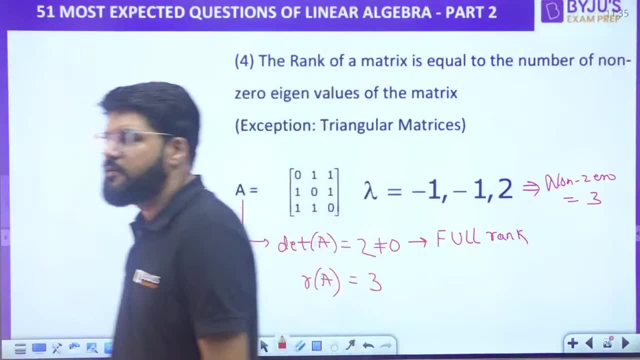 non-zero. how many are non-zero? how many non-zero eigenvalues? ye bhi 3 hai. how many non-zero eigenvalues- this is also 3 dear- how many non-zero eigenvalues are? that is also equal to the 3, correct hai? that is also. 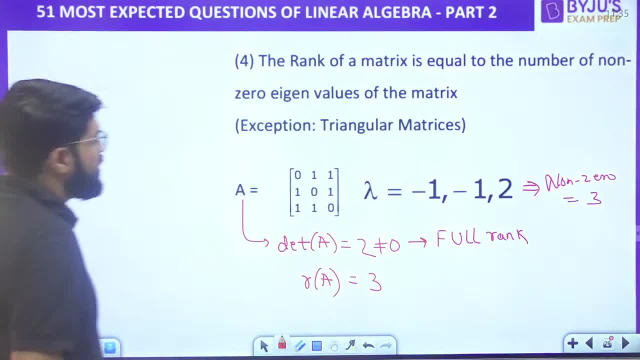 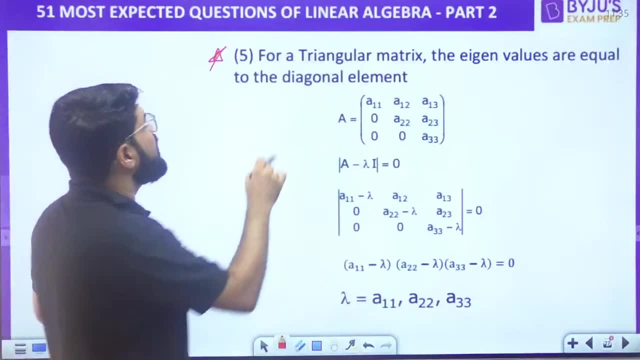 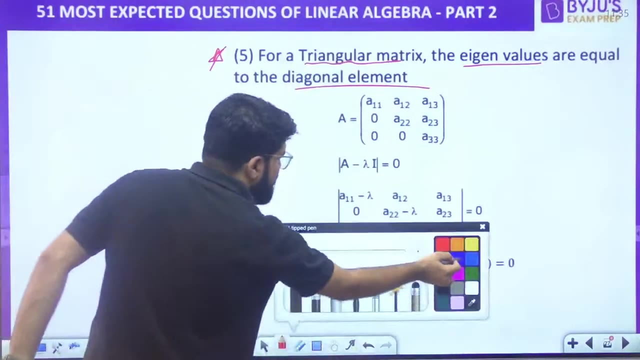 equal to 3. the rank is equal to number of non-zero eigenvalues. you can even check with the previous questions. this is always satisfied. okay, this is again important, helpful in many questions. for a triangular matrix, eigenvalues are equal to diagonal elements. for any triangular matrix, this is a proof. written. isko chhod dije. let us take a simple example, suppose i give. 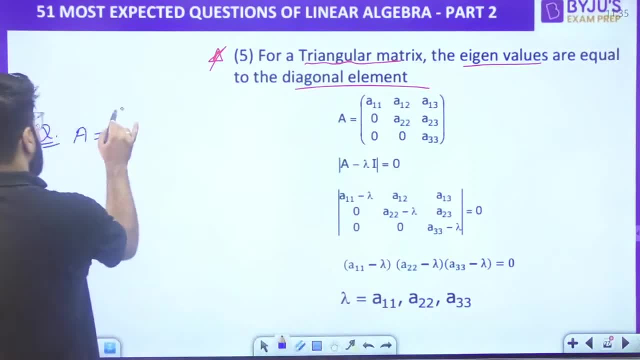 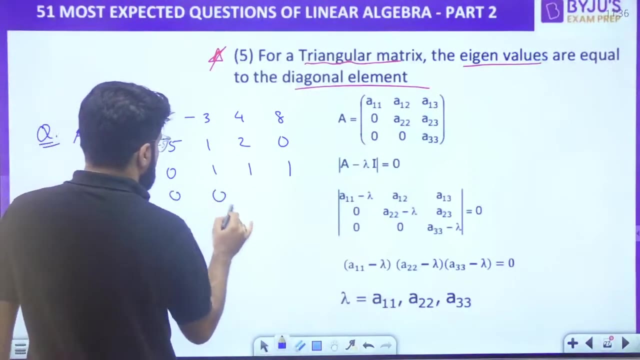 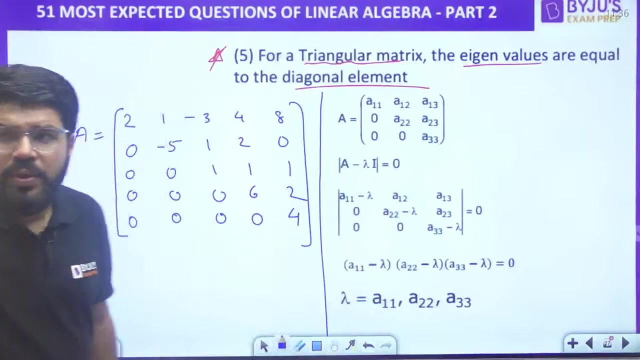 you a matrix. you know it could be any size matrix, right, be it 5 cross 5 case. also, what are the eigenvalues for any triangular matrix, be it upper or lower? be it upper or lower, the eigenvalues are just equal to diagonal numbers. you don't have to put any. 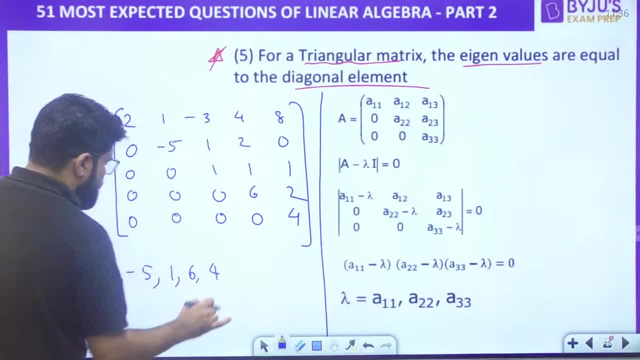 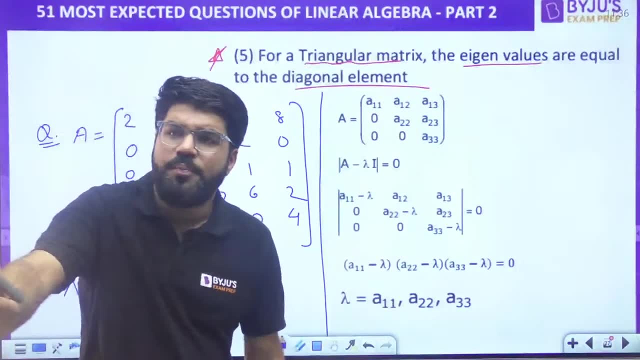 effort. this is 2 and minus 5 and 1 and 6 and 4, 2 and minus 5 and 1 and 6 and 4 right, 2 and minus 5 and 1 and 6 and 4 directly. you have to copy the numbers, diagonal numbers. that's it, nothing else. 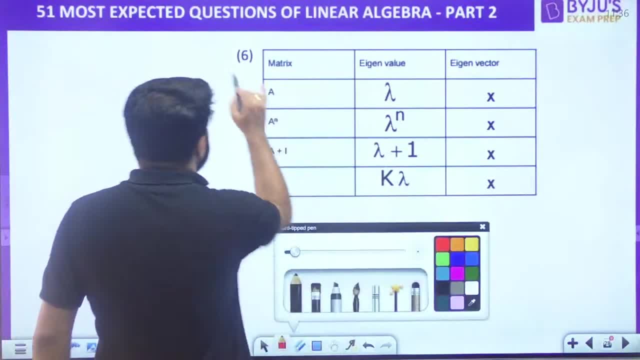 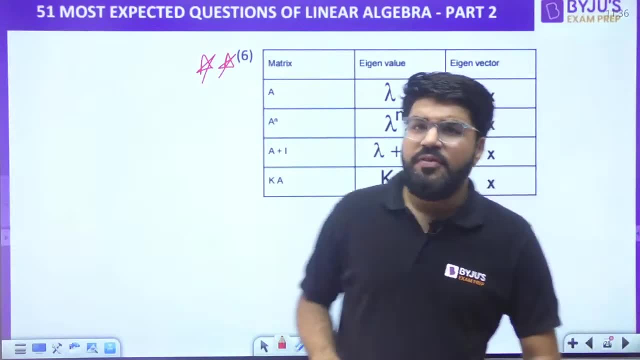 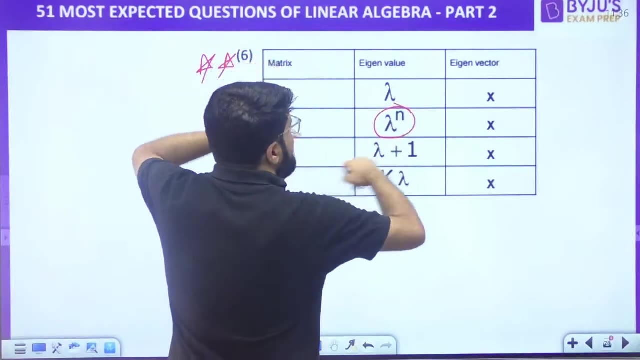 to be done right. this is again very important. jaha se questions- banta hai. this is again double star. here also lots of questions are made in the exam. the simple property is: if a has a eigenvalue lambda and eigenvector x a power n, you take any power of the matrix eigenvalue also lambda power. 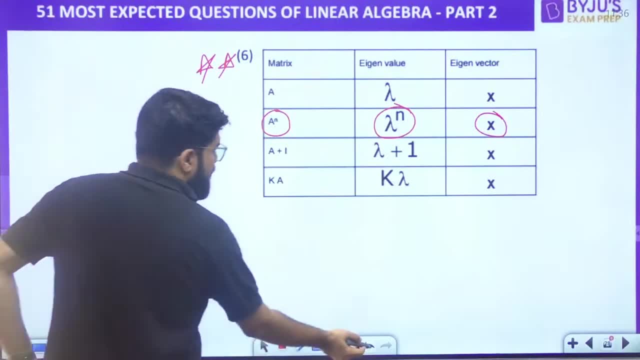 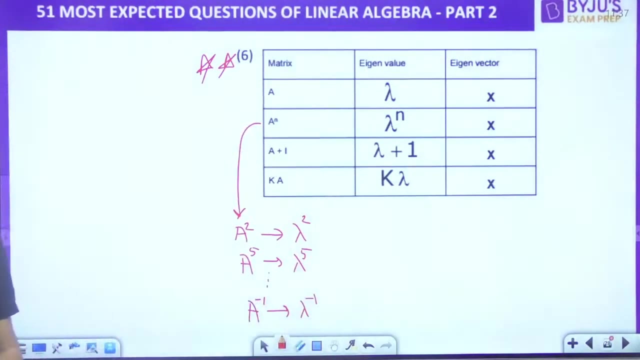 and same eigenvector. right, okay, so you know this can be. you know, suppose i take a square, aA² will have the eigen value lambda square. if i take a power 5, that will have the eigenvalue lambda power 5, etc. even if i take negative power, a inverse, what is the eigenvalue of a inverse? here eigenvalue of a inverse. it is lambda inverse, that is, 1 by lambda. the same value of a inverse here supposed to be 2 coordinates. so if, and the floor should be all right, so now what we callotes should be alpha 1, one squared, a square and emptied. 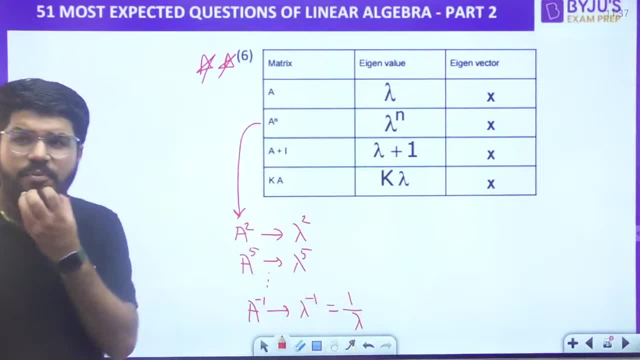 Porta thisweg has to be like this. we have to, because what this means, that byfelt that I know. you know what she said. fact is that, as you know, типа is an�иеse should give you a counter advantage. 1 by lambda. That property is also coming up, Akansha, Just wait, That is also going. 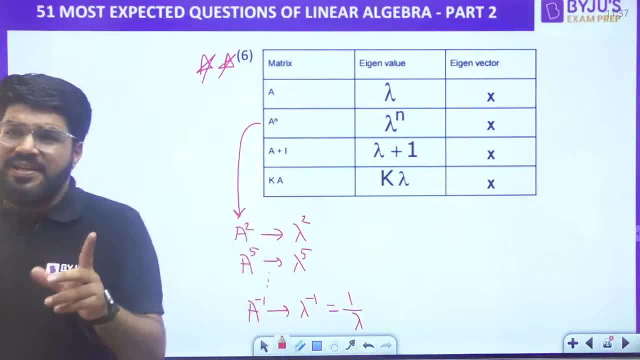 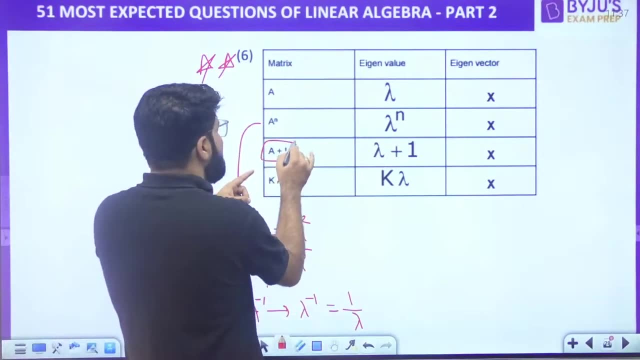 to come up Right Baki. what is linear independence? Independence, it is same as what you have discussed yesterday. also, Okay, A plus I. if you add identity to matrix, it should be lambda plus 1.. Plus 1 in the eigenvalue Same eigenvector. Eigenvector is not affected. Okay, Simple. 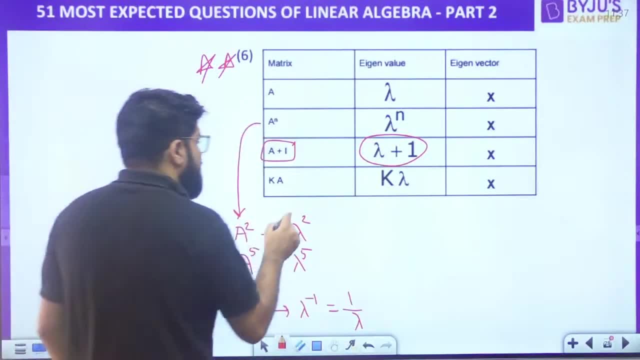 proofs are there but not required right now. Abhi ke well question and property pe focus: karenge, You multiply matrix by some number k, some scalar number, k, Eigenvalue also multiplied by k. Okay, Matlab, if the matrix is suppose 6A, the eigenvalue will be 6, lambda With. 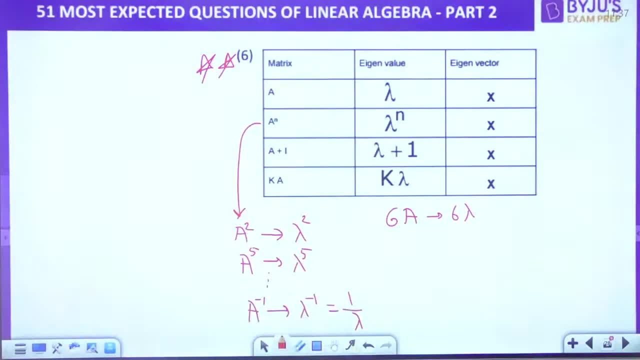 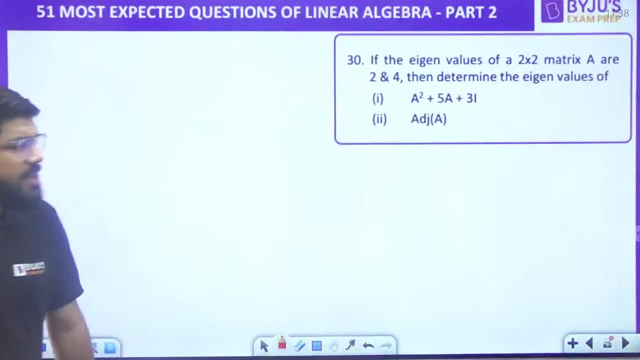 the same eigenvector With the same eigenvector, Right dear, Very important property. Okay, There are total 16 properties, which is going to cover every range of question, but let us take a question here, Question number 13, sequence: If the eigenvalues of a 2 cross 2 matrix are, 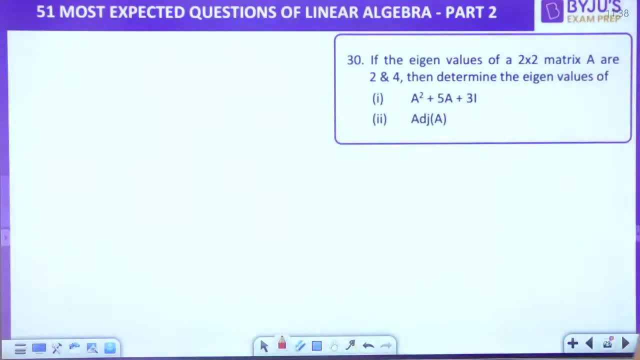 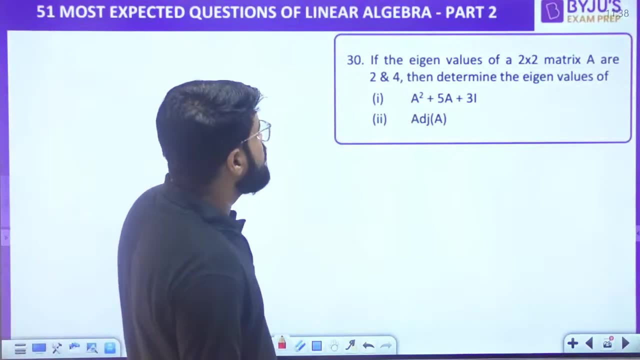 2 and 4, determine the eigenvalues of A square plus 5.. A plus 3I and adjoint of A And the adjoint of A If the eigenvalues of a 2 cross 2 matrix are 2 and 4, determine the eigenvalues of A square plus 5A plus 3I and the adjoint of. 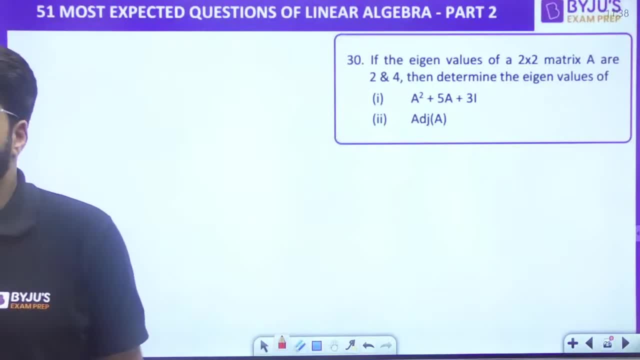 A Right. Tell me No for two different matrices. no, Gajendra, Not generally. Depend on the type of the matrix, but not generally. Not generally Okay If A and B are two different. if it B is like identity type of matrix, then it is okay, but not in general Identity wala. 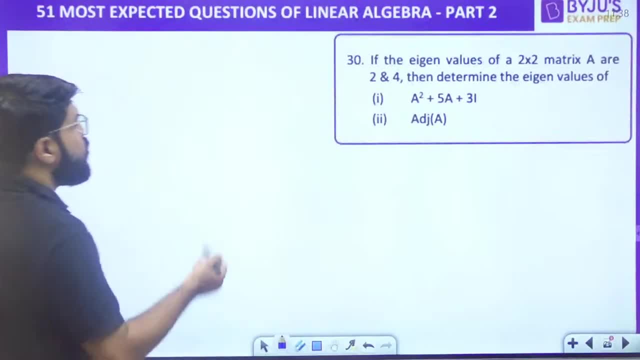 property. da mane boli diya A plus I. Okay, So if A has the eigenvalues 2 comma 4, what should be the eigenvalue of A square plus 5A plus 3I. So what you have learnt from. 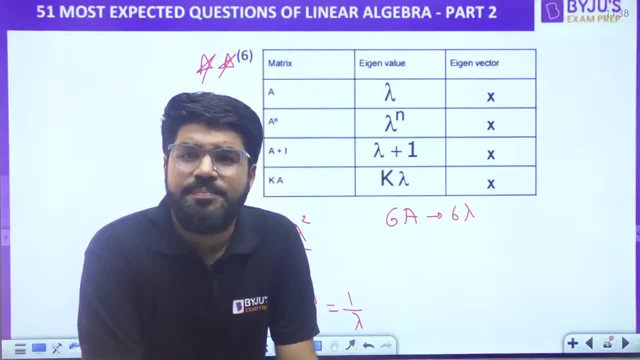 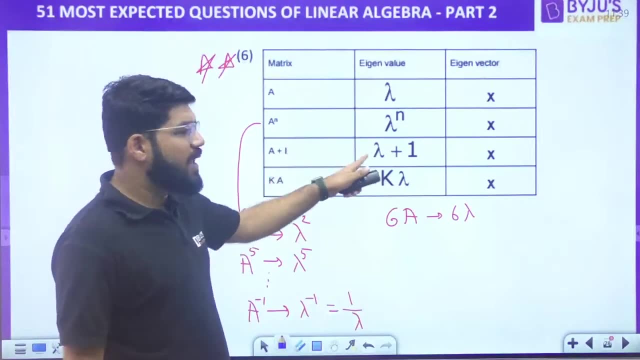 the previous property. Previous property simply is telling you that whatever operation you apply on, A, same applies to the eigenvalue A, power N, lambda, power N. A plus I, lambda plus 1.. Number hai wo K into A, K into lambda. Whatever algebra you apply on the, A same applies to. 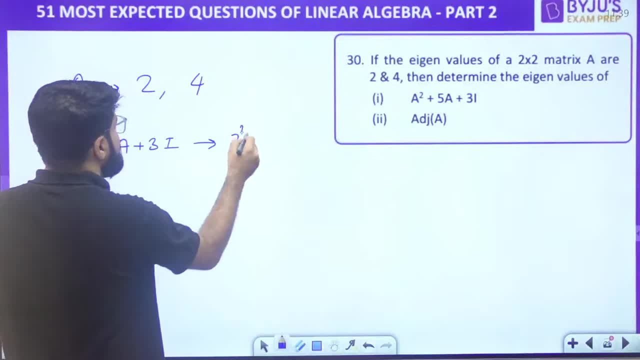 the lambda. So here it is A square plus 5A plus 3I. So first eigenvalue should be 2 square plus 5 into lambda, 5 into 2 plus 3 into I. I ki jagay banayega Right And the. 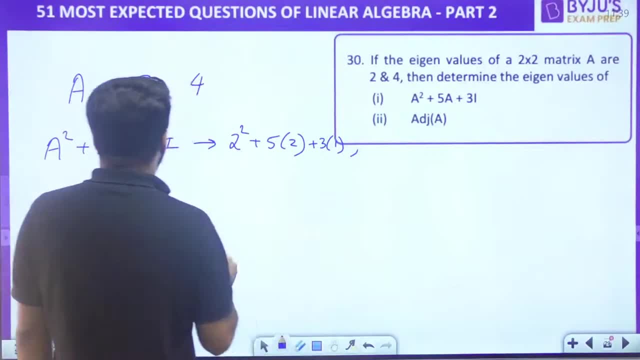 next one should be Right, And the next one should be 4 square plus 5 into lambda, 5 into 4 plus 3I, that is, 3 into 1.. So this corresponds to 4 plus 10 plus 3, 17, and next is 16 plus. 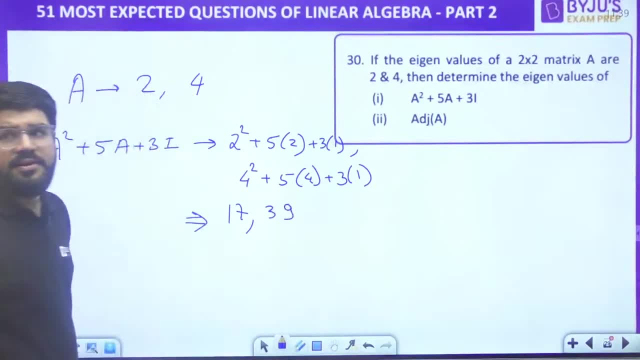 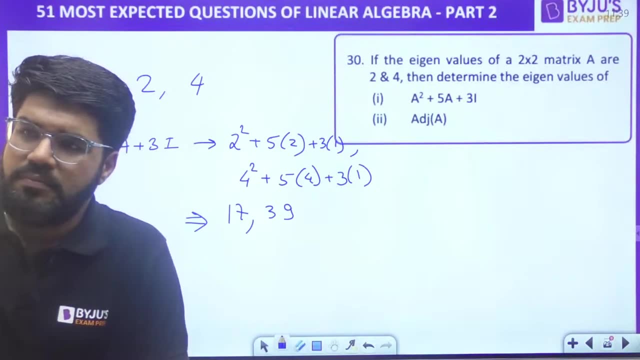 20.. 36 plus 3 is 39. So answer should be 17 and 39.. Kindly check 17 and 39.. Kindly check A plus 3I me A plus 3 lambda plus 3.. Correct, haa Nishu, correct. 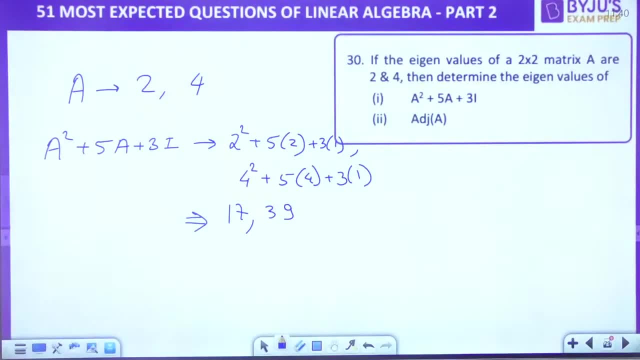 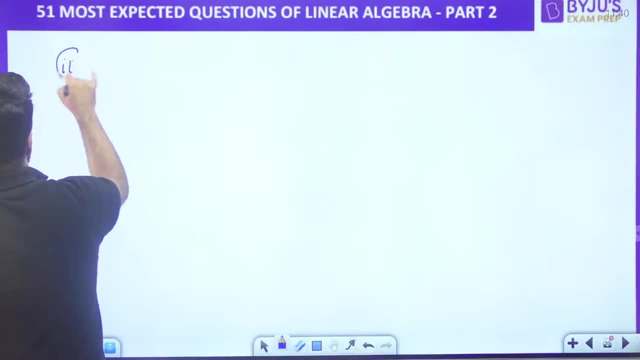 Okay, so this is what is one first answer. Second one: adjoint. Now adjoint, ko kaise solve karenge? A, B, C, Caa, caa? see, we know that adjoint of a divided by modulus of a is known as the inverse of the matrix. 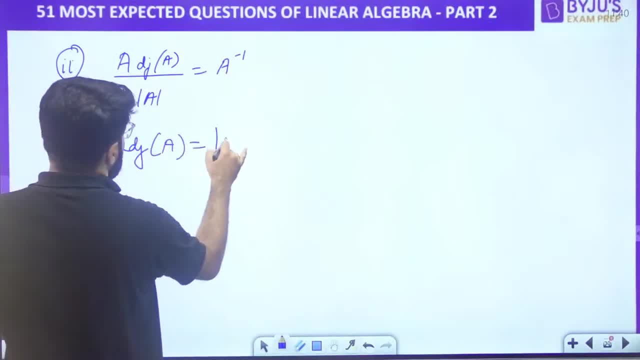 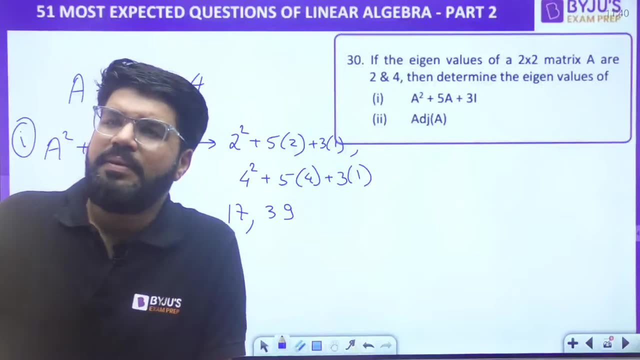 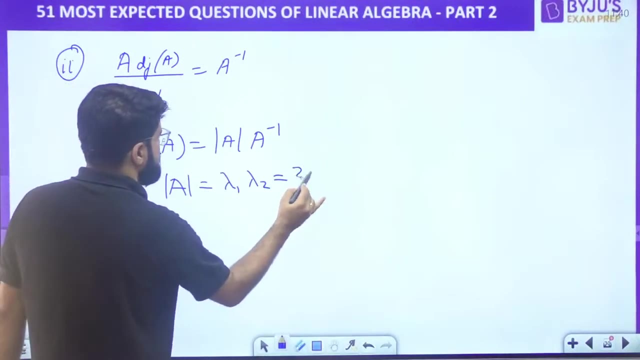 so what is the adjoint of any matrix? it is mod a into a inverse. what is the mod a matrix eigen? for the matrix, eigen values are given 2 and 4. what is the modulus of a product of the eigen values? okay, right, so for a, the eigen values are 2 and 4. so for a inverse, 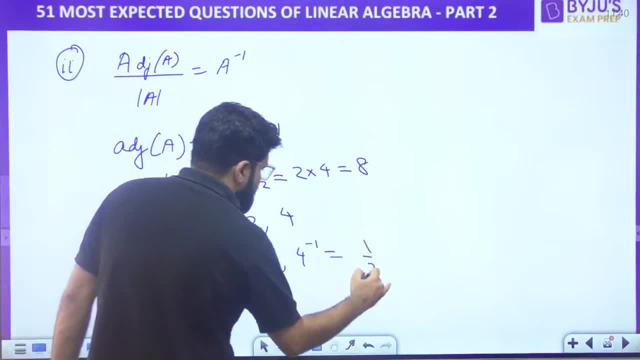 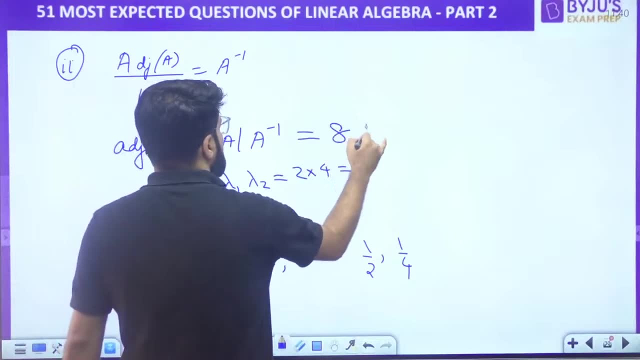 what should be the eigen values: 2 inverse, 4 inverse, that is 1 by 2, 1 by 4. so for the 8 a inverse modulus of a value, 8, for the 8 a inverse, the eigen value, you multiply 8. so 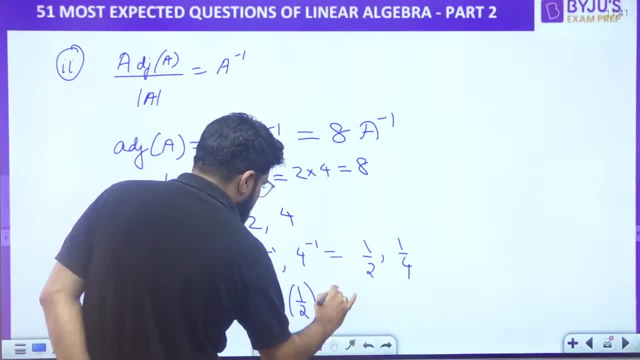 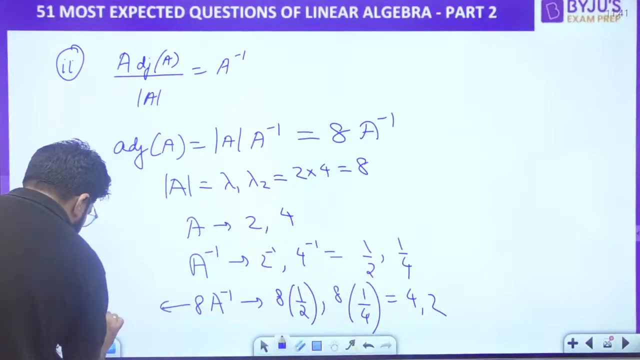 eigen values are also multiplied by 8. 8 into 1 by 2, 8 into 1 by 4, and that is equal to 4 and 2, and this is what is adjoint of a. so what is your answer? that is 4 into. it is just swapped. 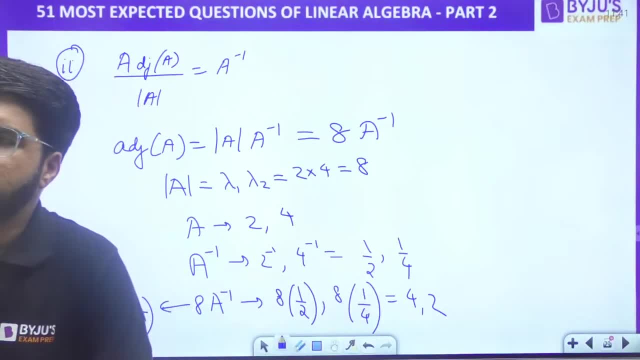 yeah, you can use this arvin and we are coming to that property also. you're coming, just wait. we are coming to, i told you, the 16 properties covering up every type of property, and that will help you to solve every type of question. just wait for it, okay. 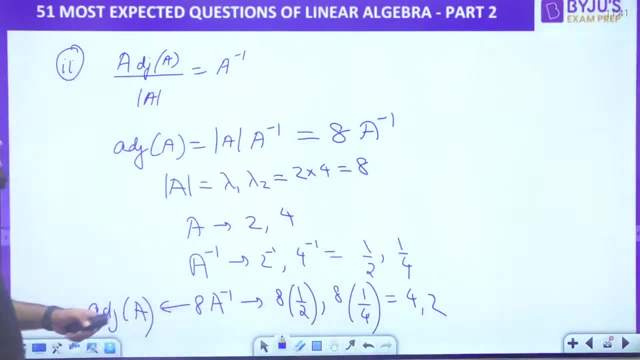 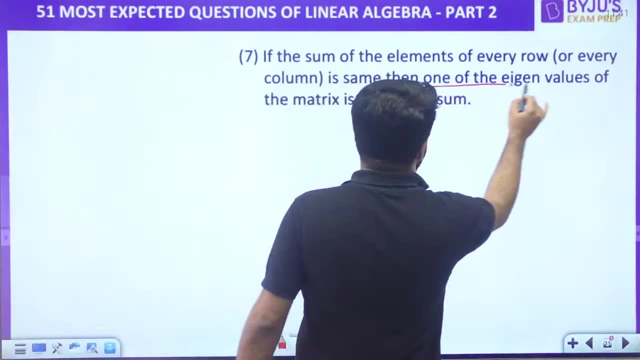 so both these questions are solved. okay, this was only property number 6. now property number 7. if some of the elements of every row is same, then one of the eigen values is equal to that sum. one of the eigen values is equal to that sum. okay, that's a for example. i'll 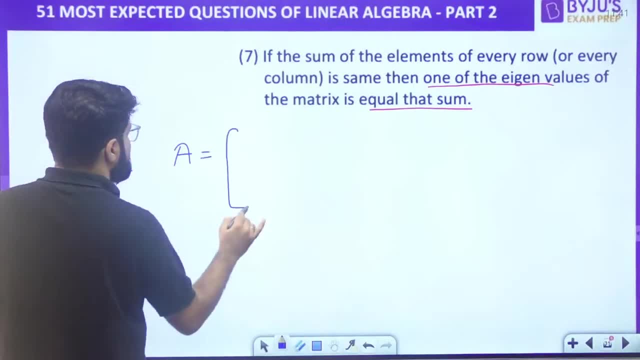 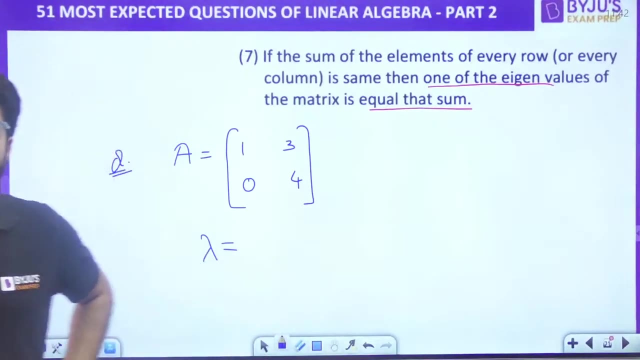 explain. you suppose there be a matrix. what are the eigen values of this matrix? good to morning misra. what are the eigen values of this matrix? it's a upper triangular matrix, dear simple matrix, i have written. for any triangular matrix, eigen values are equal to diagonal numbers. so 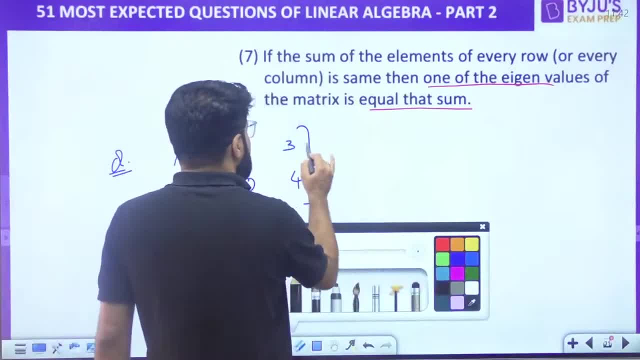 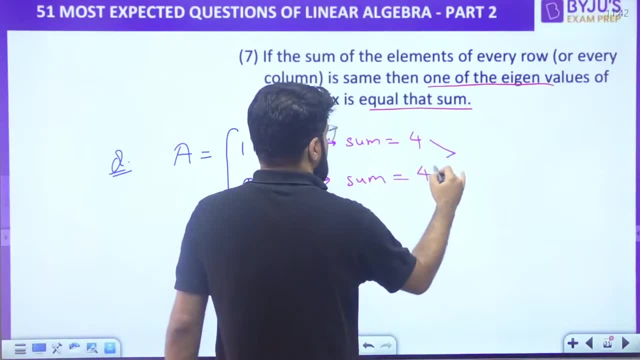 eigen values are 1 and 4. what is the sum of every row? sum here is 1 plus 3. sum of the next row, that is 0 plus 4. this is eventually same whenever sum of elements of every row is same. yeah, every column. 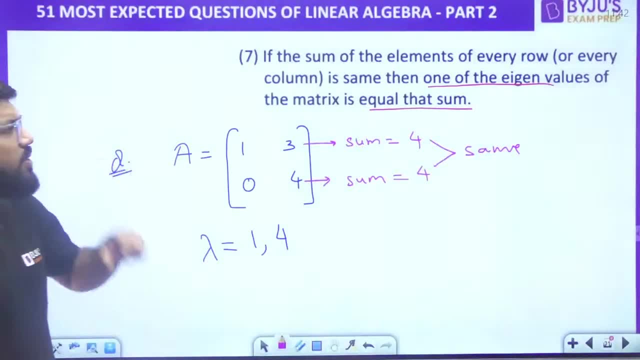 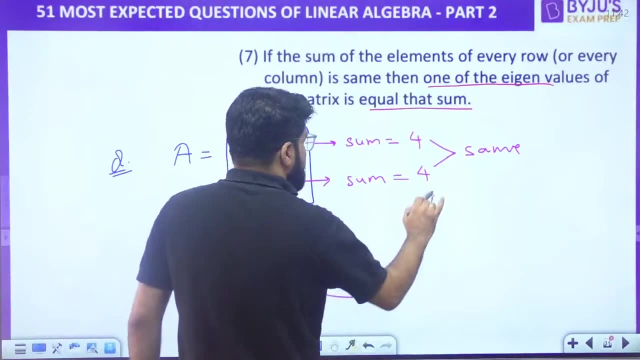 you have to see here row property is applicable. some of the elements of every row is same. then one of the eigen value is always equal to that same. to see one of the eigen value. one of the eigen value is equal to that. sum is equal to that. 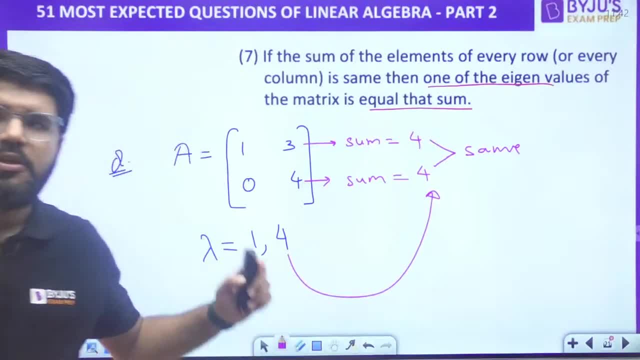 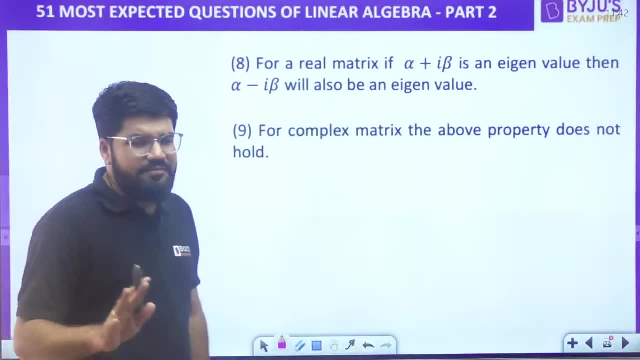 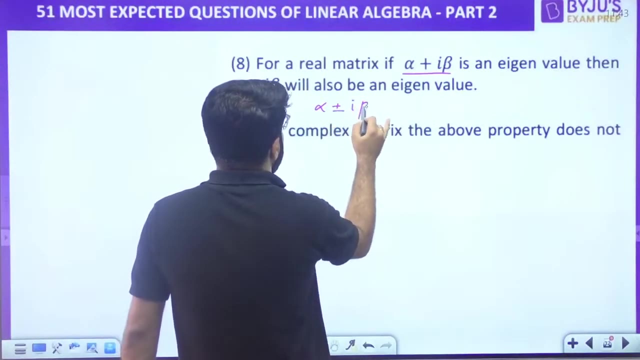 sum automatically. it came up now. next, for a real matrix: if alpha plus i beta is an eigen value, alpha minus i beta- complex eigen value- will appear in the conjugate pair. complex eigen value will appear for a real matrix. we will take the questions on this, don't worry. 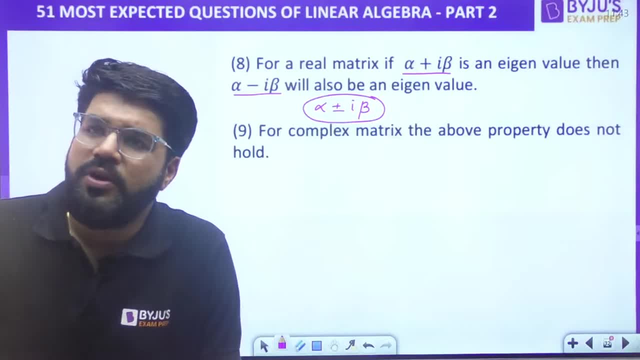 complex eigen values. if any, they will be in conjugate pair. for a real matrix, what is a real matrix? whose all elements are real? but if there is a complex matrix, what is a complex matrix? if any of the element is complex, then the above property may not be true. okay, then eigen values. 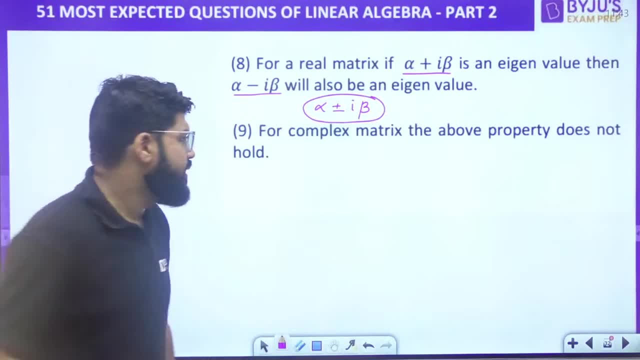 then complex eigen values can be standalone. there can be a eigen value plus 2i, but there may not be the eigen value minus 2i as a whole. sector for a complex matrix: okay, for a complex matrix? hello, next we'll see the questions on that. just wait on that, let's complete. 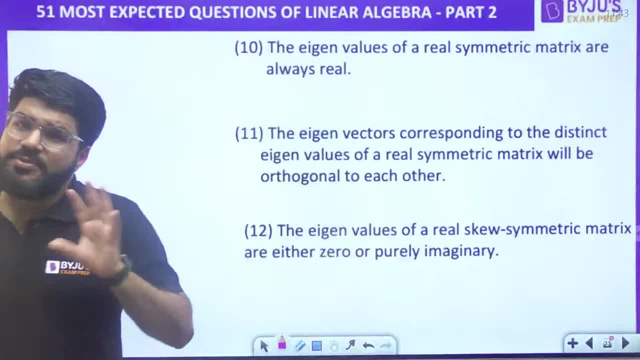 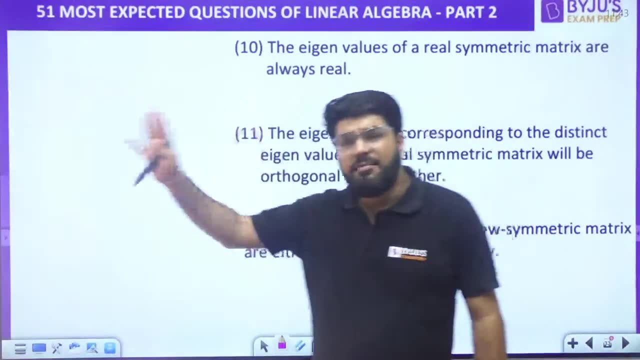 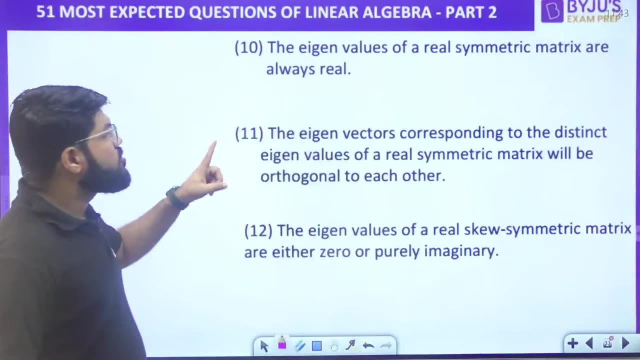 now there are some you know properties important for factual as well as numerical. these are more important for factual sometimes the gate has discussed previously and can be expected in future also, simple fundamentals, true or false, or simple property based questions. eigen values of a real symmetric matrix are always real. kylie hamilton. kylie hamilton, i will cover today only. 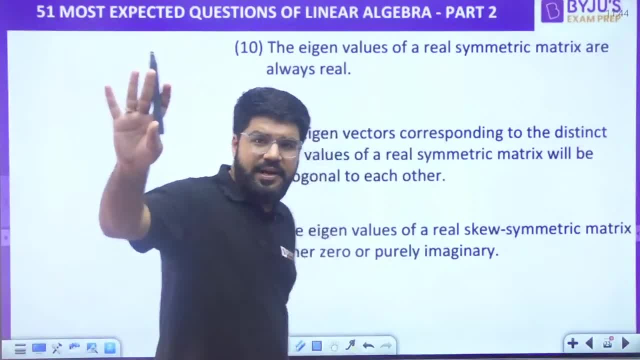 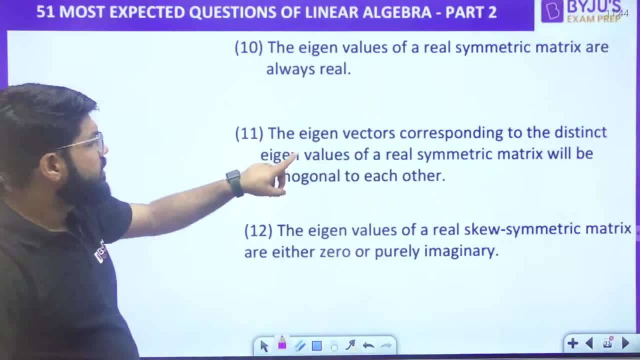 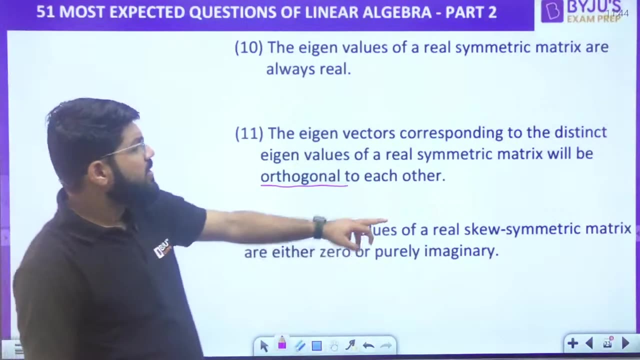 but at the last. okay, wait, kylie hamilton will be covered towards the end. first let us cover the eigen value regular question. okay, eigen vectors corresponding to distinct eigen values of a real symmetric matrix will be orthogonal to each other. perpendicular to each other. eigen values of a real skew symmetric matrix are either zero or pure. 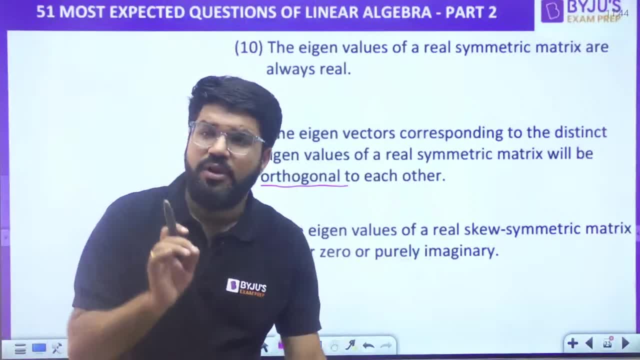 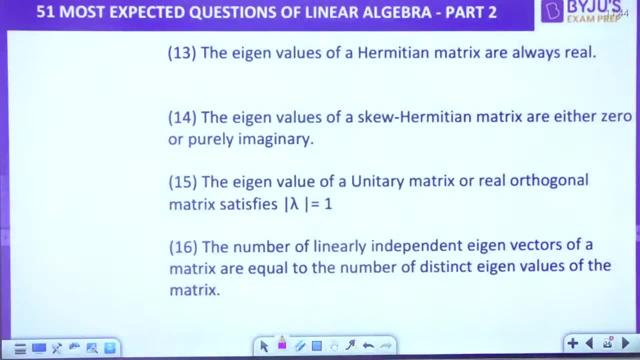 imaginary, okay, so i'm showing you, i'm giving you as a completion of notes. you have to remember you can expect the factual questions also here. okay, eigen values of hermitian and skew hermitian and unitary will include the hermitian matrix. eigen values are always real. skew hermitian matrix. again, eigen values are either purely zero. 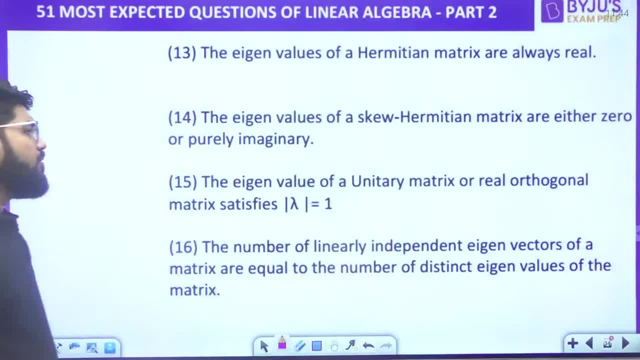 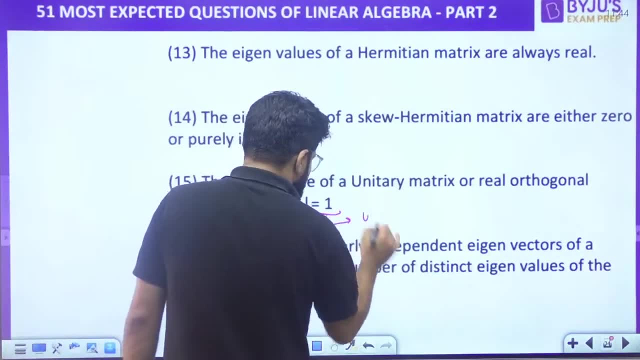 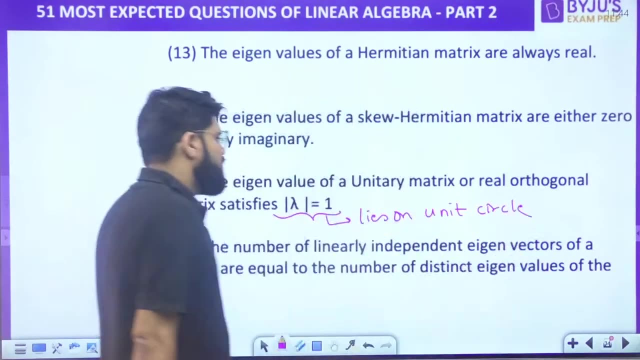 or purely imaginary, or zero for a unitary matrix or the real orthogonal matrix, the eigen values will lie on the unit circle, will satisfy mod lambda equal to one. that is, lies on the unit circle. it lies on the unit circle. right for your quick revision, let me keep writing. what is the real. 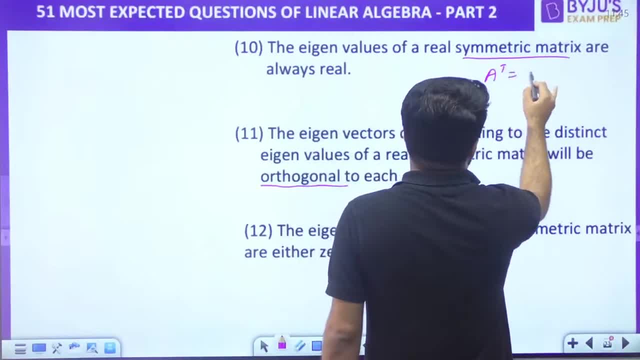 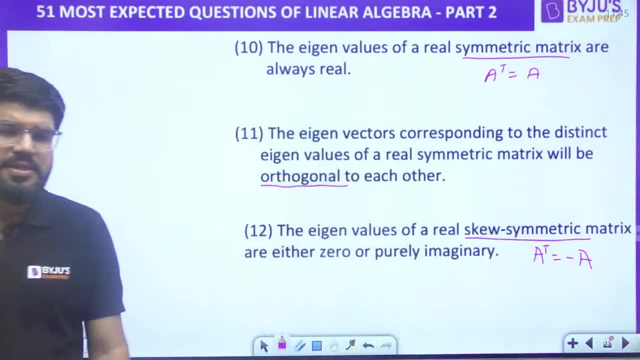 symmetric? yeah, what is a symmetric matrix in general? a transpose equal to a. what is a skew symmetric matrix? a transpose equal to minus a right eigenvectors corresponding to distinct eigenvalues. okay, this property is called. suppose, a matrix a has eigenvalues lambda 1 and lambda 2. 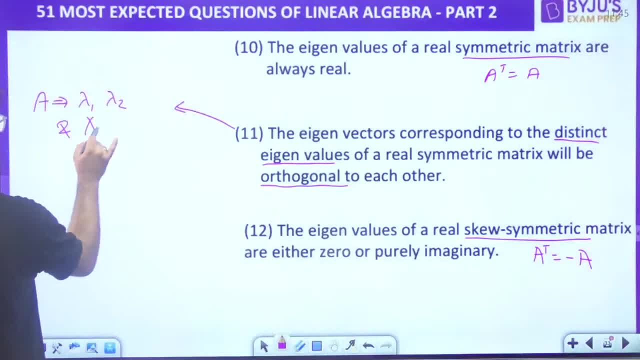 and the corresponding eigenvectors are. corresponding eigenvectors are x1 and x2. okay, suppose that the eigenvalues lambda 1, lambda 2 are distinct. they should be not equal. then the eigenvectors will be orthogonal. if lambda 1 not equal to lambda 2, then the eigenvalues will be orthogonal- orthogonal. 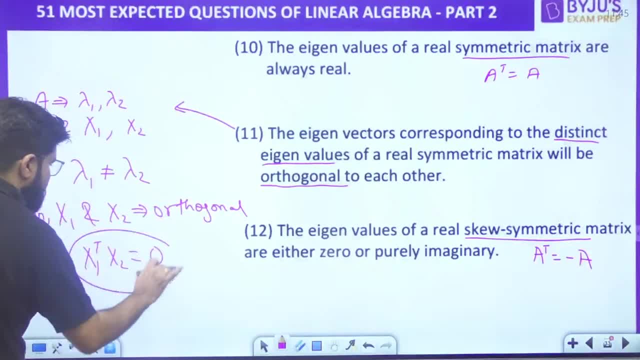 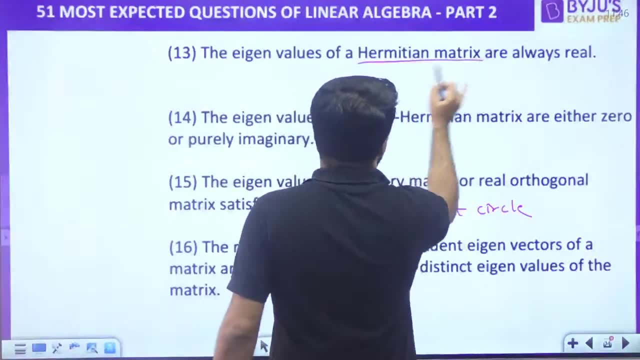 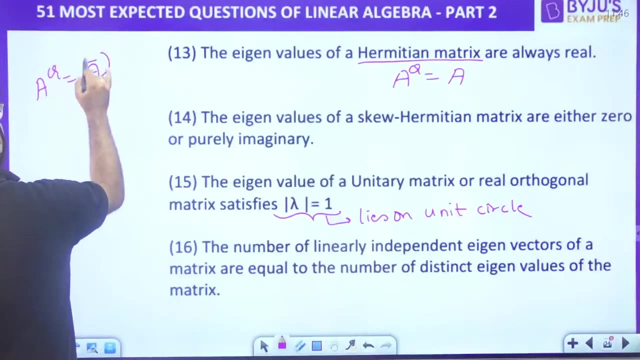 means when you take their dot product x1, transpose x2. it should be equal to the zero, zero, zero. it should be equal to zero. what is the hermitian matrix? hermitian matrix is one which satisfies aq, equal to a. what is aq for complex matrix? we take aq, that is, a conjugate whole, transpose. 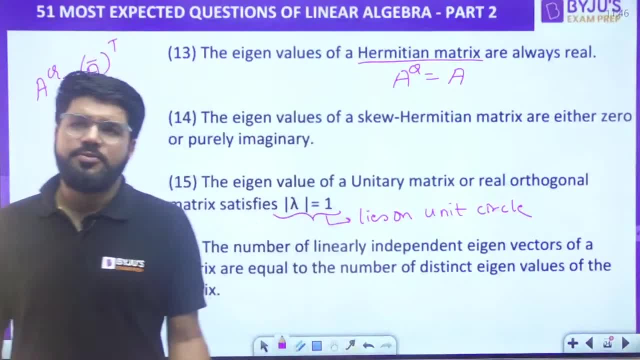 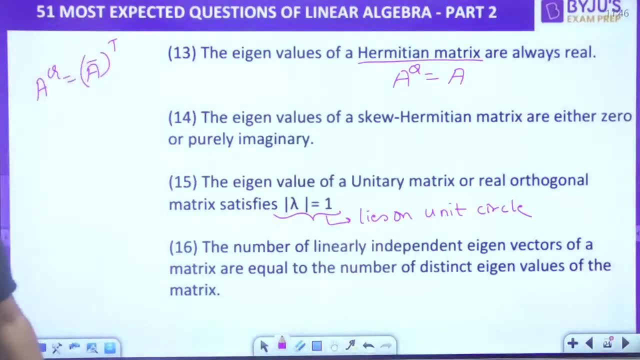 for real matrix we take a transpose transpose, you all know. for complex matrix we take a conjugate transpose. that means first take the conjugate of all the entries and then take the transpose of the matrix, and if aq is equal to a, that matrix is a hermitian matrix. skew, hermitian matrix just. 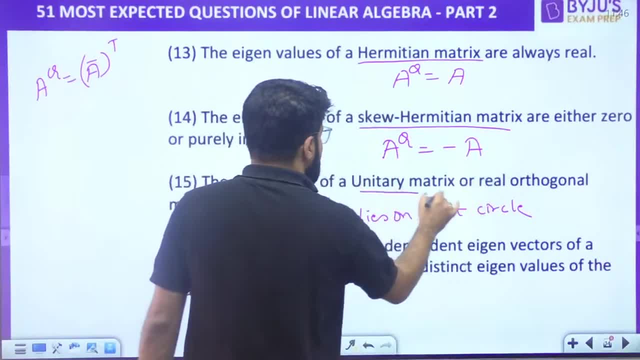 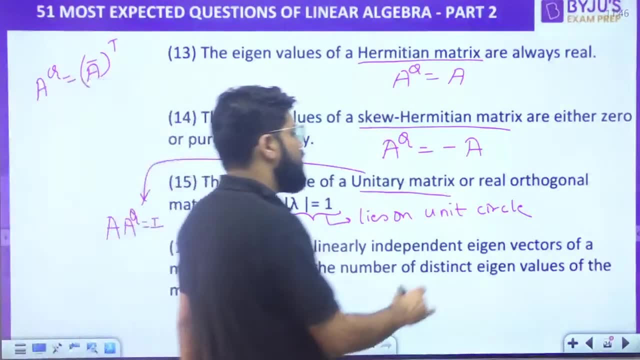 as a quick revision, i am telling you: aq equal to minus a. what is the unitary method, unitary matrix? unitary matrix is one which has a into aq equal to identity right. what is the real orthogonal matrix? a matrix which has a, a transpose equal. 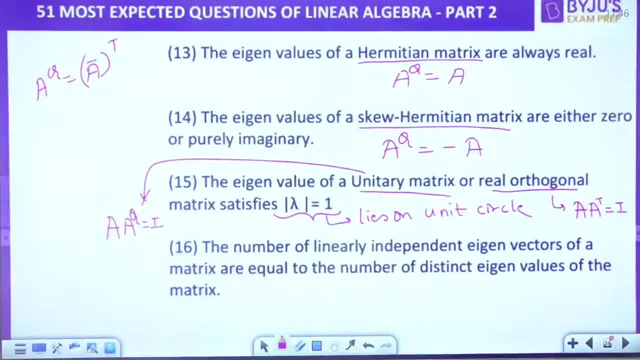 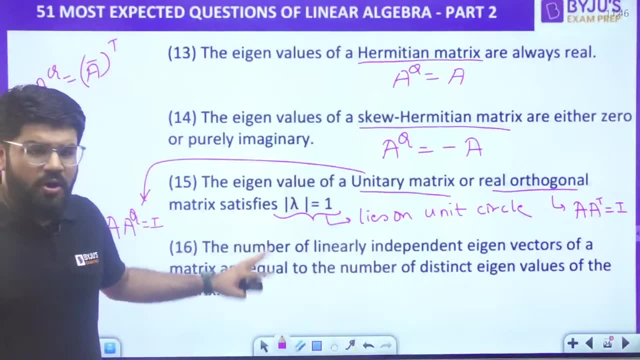 to identity. this is basics of matrix. just as a quick revision i am writing down. the number of linearly independent eigenvectors of a matrix are equal to number of distinct eigenvalues of that matrix. all of these will have some questions which we can relate okay. 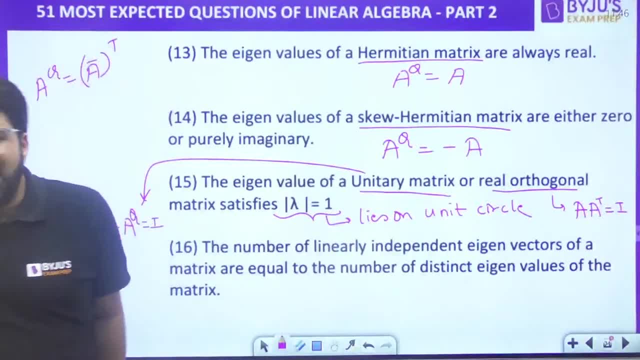 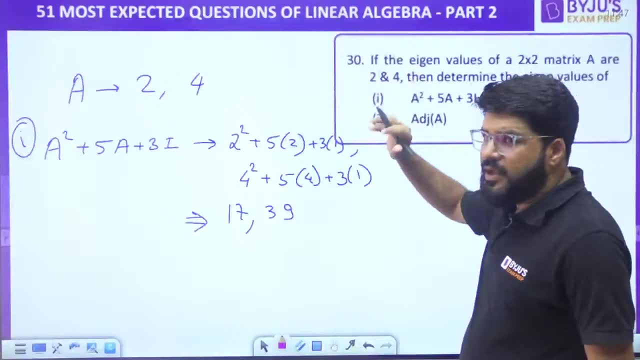 this is the list. i wanted to complete 16 properties. now Let us get carried with the questions and questions, All important type of questions. We have done questions till now, till number 30. Right, So 2021 questions are more there, which is going to cover all the properties that I have listed. 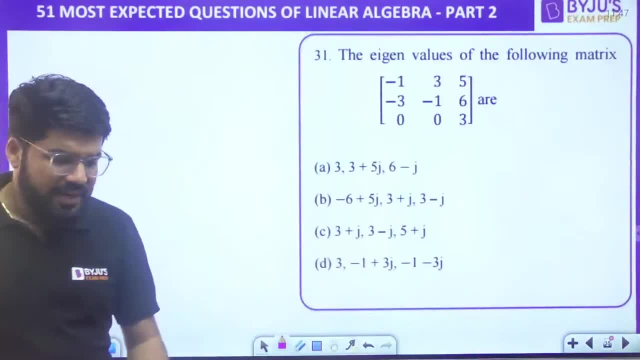 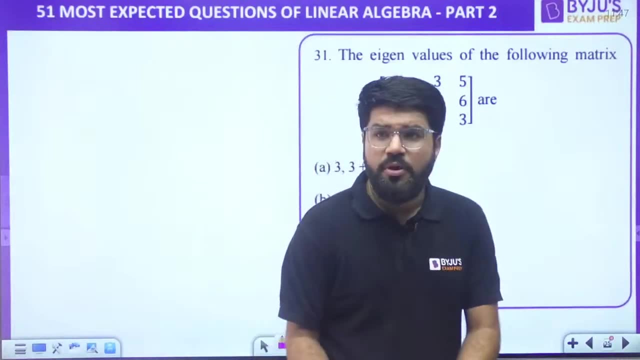 Okay, So that all your doubts are rectified, Let us go to the question number 31.. And I was telling you, many of the questions can be solved only by properties. Many of the questions can be solved only by the properties. What is the eigenvalues of the following matrix? 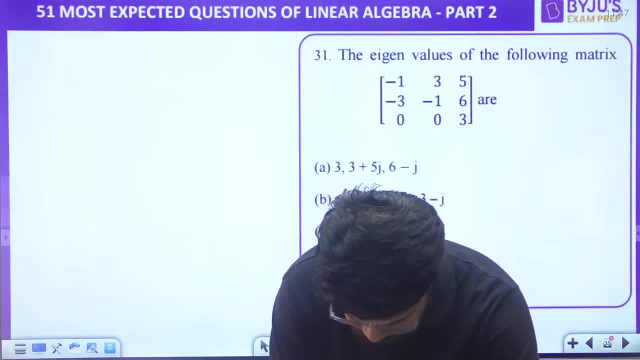 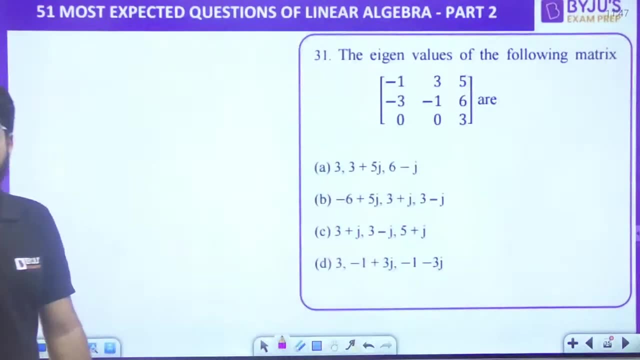 Come on, guys, Quickly. you should be able to tell me What is the eigenvalues of the following matrix. Very simply, you can say: no need to calculate. See, no need to calculate beta 1,, beta 2,, beta 3 here. 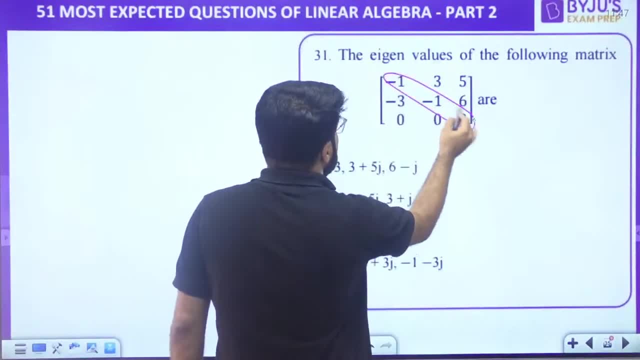 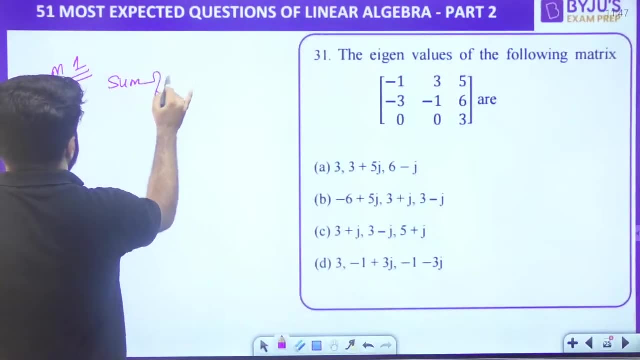 You can calculate very simply, Sir, how Eigen values is. the sum of eigenvalues is equal to trace. Okay, Method number 1.. The sum of lambdas is equal to trace of the matrix. And what is the trace Minus 1.. 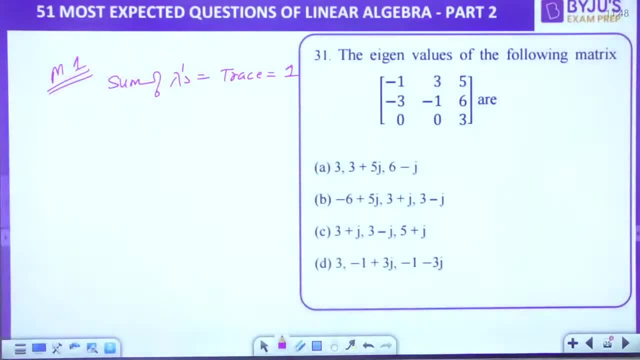 Minus 1 plus minus 3, that is equal to 1.. The sum should also be 1.. Sum should also be 1.. Right Option number D. Option number D: Any more property? Very simply, I can deal with that. 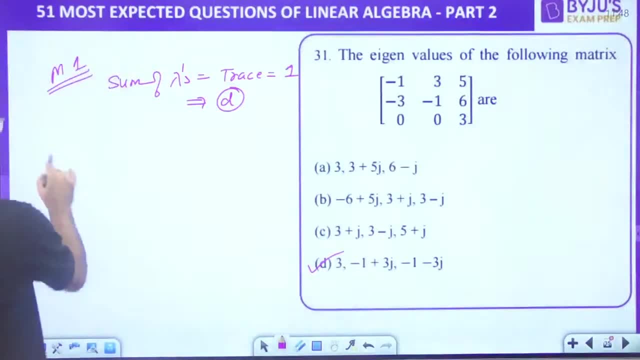 Any more simpler property? This is also simple. One more method can I specify here? You have a real matrix given to you. What is one of the property of real matrix? You are given a real matrix. All elements are real numbers. No, no determinant is also calculation. 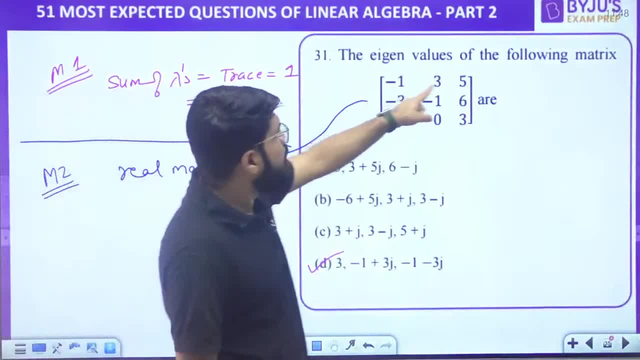 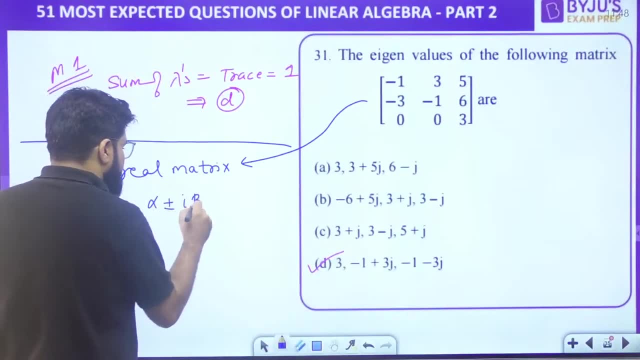 One property of observation. The given matrix is real. All numbers are real means the matrix is real And for a real matrix apply the alpha plus minus i beta property. If there is a complex eigenvalue it should be in the conjugate pair, otherwise not. 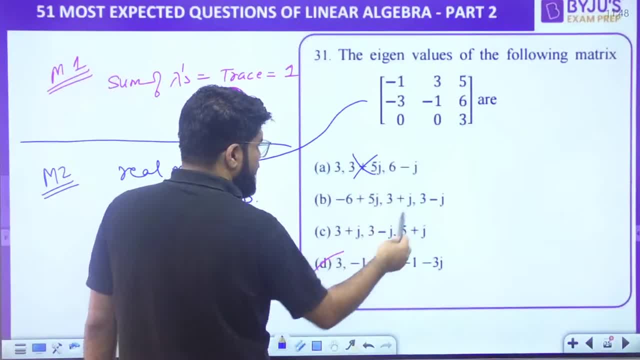 So here: 3 plus 5j. Where is the 3 minus 5j? Not here, Not available. This is in pair. but what about minus 6 plus 5j? Option number C: 3 plus minus j is a pair. 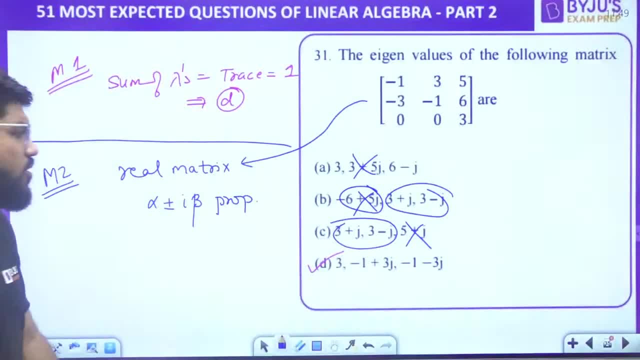 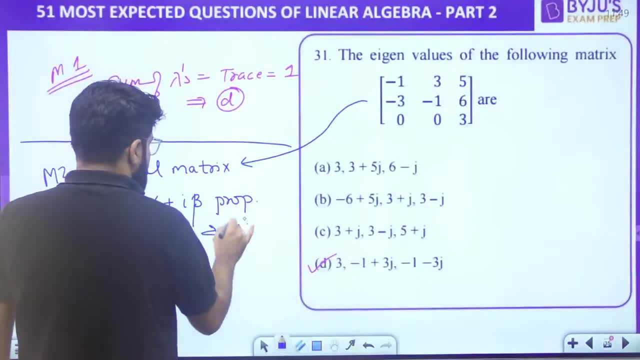 5 plus j does not have the conjugate pair. Only option number D is in the conjugate pair. Alpha plus minus i beta property: we apply. Still you have D, Simple observation. This is real No problem. But if there is something complex it has to be with the pair. 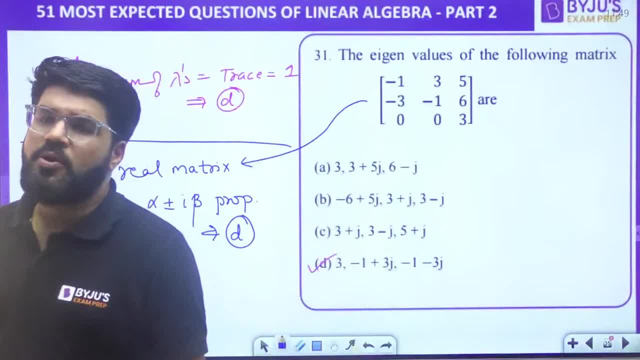 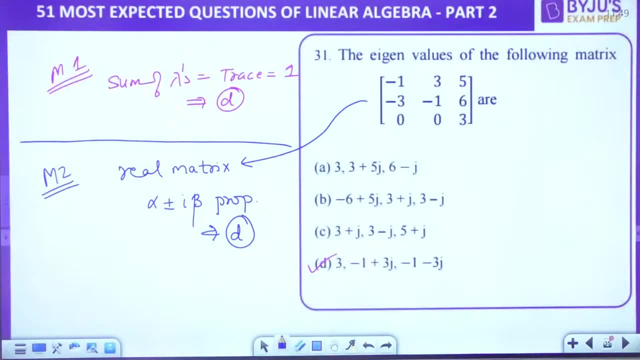 It has to be with the conjugate pair. Real can be alone, but complex eigenvalue should be in pair For a real matrix Observation. On this some more questions will come, Don't worry, Number 32.. What is the sum and product of eigenvalues? 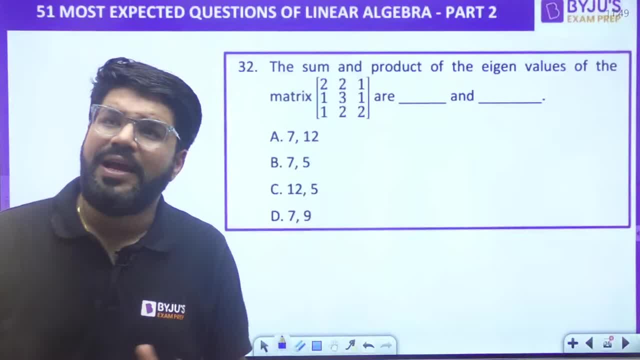 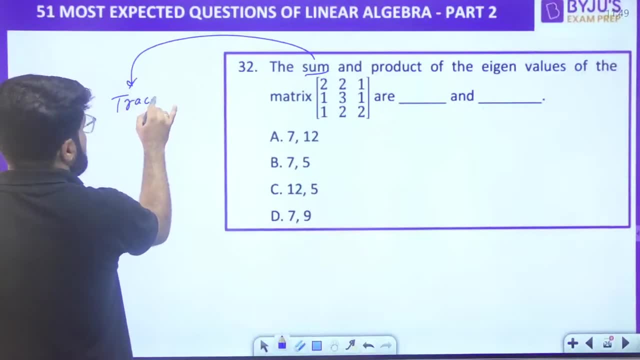 Yes, Ania, Very good. What is the sum and product of the eigenvalues? So you don't have to calculate the eigenvalues Sum and product. The sum is equal to trace. that is 2 plus 3 plus 2, that is 7.. 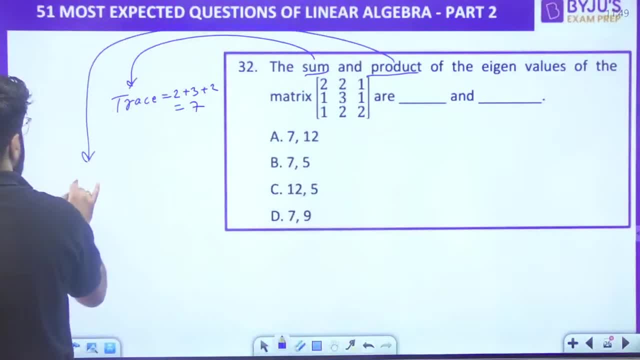 This is finished. The product is equal to determinant and determinant. let's calculate quickly 2 into 3. 2000.. 6 minus 2 minus 2, of 2 minus 1 plus 1, 2 minus 3, so this is 2 into 4, 8 minus 2 minus 1 looks. 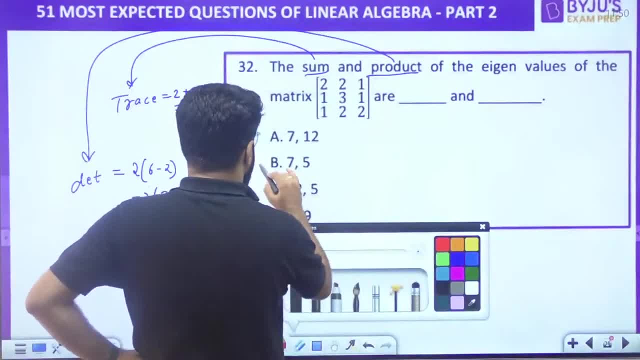 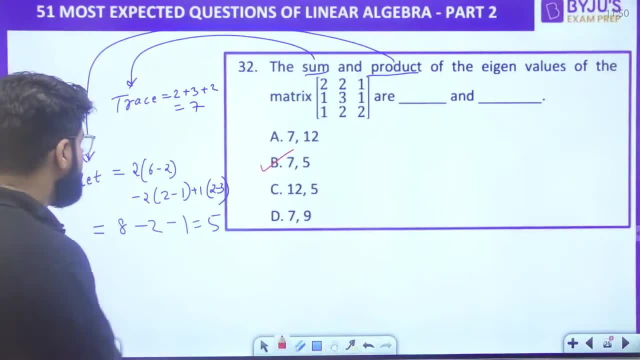 like 5, so 7 and 5. just rectify the calculation: 7 and 5. option number B: 7 and 12. 7 and 12. you are saying many of you are coming with A. let me just recheck that. there is some calculation. 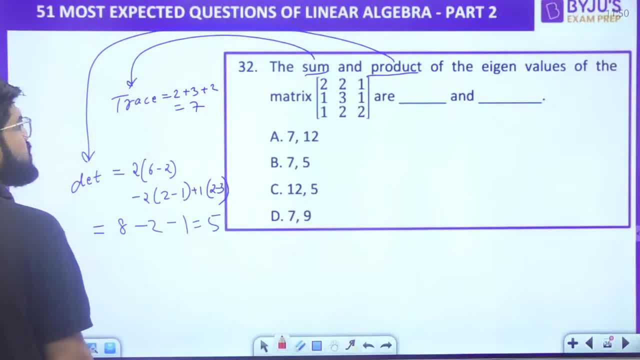 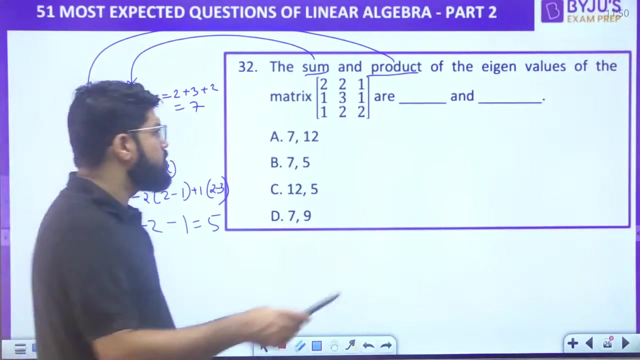 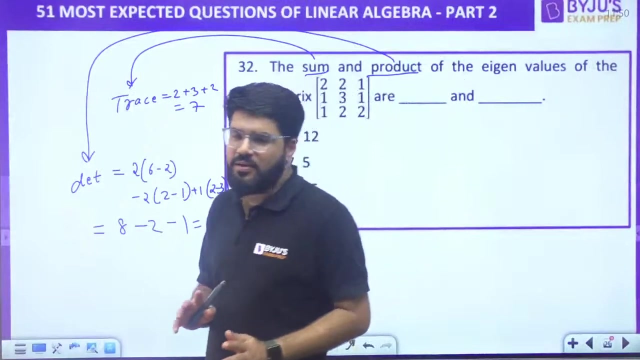 error. This is 2 into 6 minus 2. perfect, Minus 2 into 2 minus 1 and plus 1 of 1. sorry, 2 minus 3 all looks good. yeah, 4, 4, 2's are 8. this is minus 2, 5, 5, 5. just check it out, guys. it is coming 7 and 5. why you are giving 7 and 12? B, B, B, Mishra, correct, Ravi, correct, okay. so many of you just suddenly gave A. no, that is wrong. B is the correct answer. so this E, these properties are helping you, but you have to be really careful with the calculation. it should not be so hurry that you spoil the calculation and you lose the calculation. 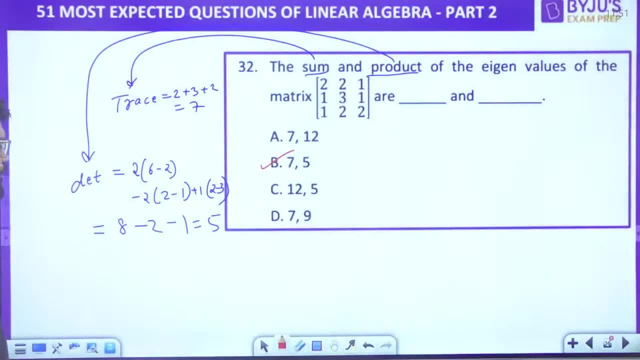 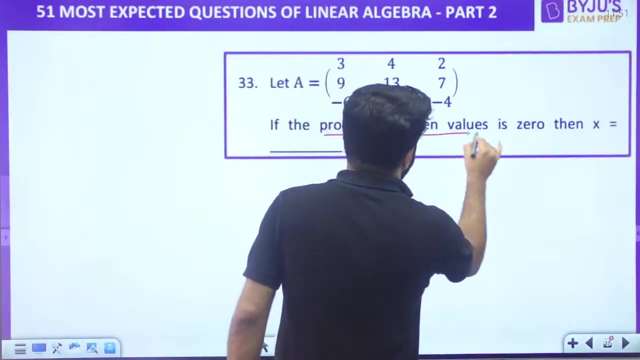 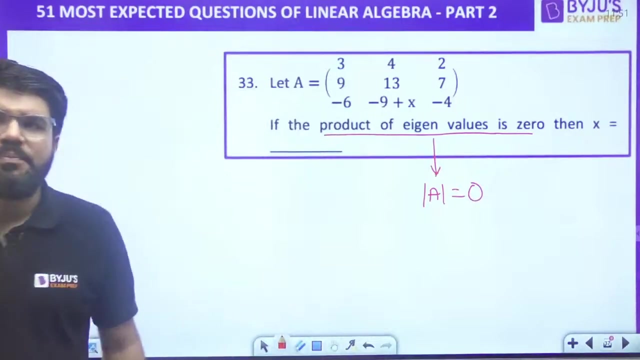 you lose marks. okay when you lose marks- okay, next one. okay, cool, next one. next question, number 33: let A is equal to some matrix if the product of eigen values is 0. so this question is taking you: what product of eigen value is 0? that means the determinant of the matrix is 0. this question is again a determinant type of question. the determinant of the matrix is equal to 0. 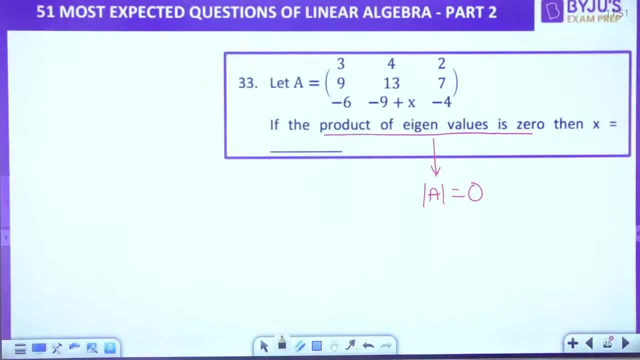 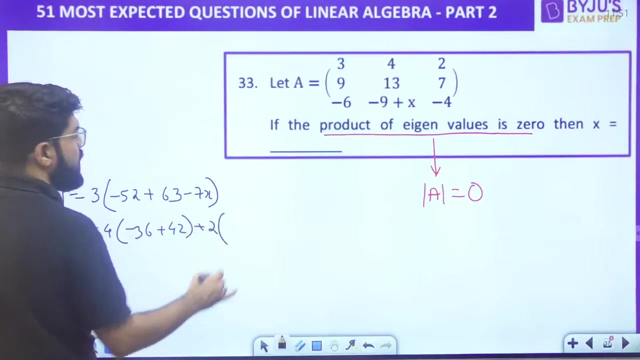 then the determinant of the matrix is equal to 0. what should be the determinant 3, 13 into minus 4 becomes minus 52 minus 7 into 9 plus minus 7 into minus plus 63 minus 7 x right minus of 4 minus 36 plus 42 plus 2. 9 into minus 9 minus 81 plus 9 x minus minus plus 78, and this should be total. 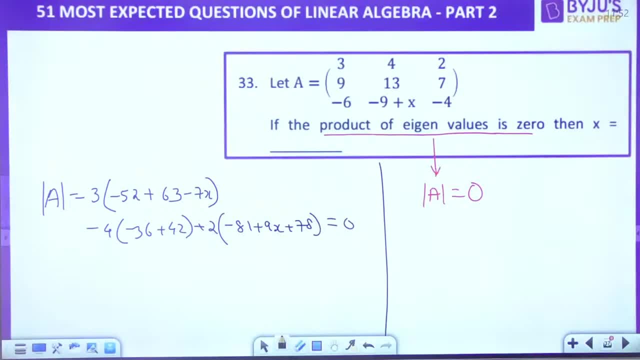 equal to 0. okay, from here you can get the value of x, from here you can get the value of x. so this becomes minus of 156. okay, so this is 11, so 11. 3 is a 33 minus 21 x. this is 6 into minus 4, so minus 24, and this is minus 81 plus 78. that is minus. 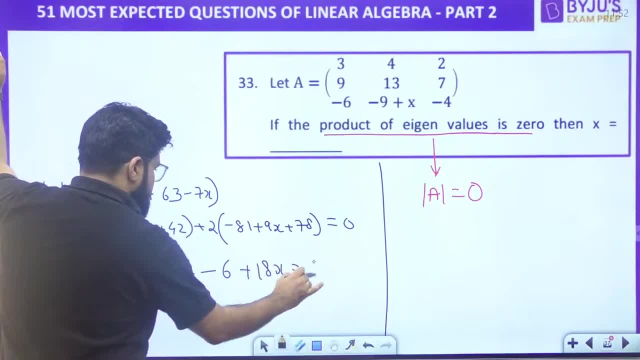 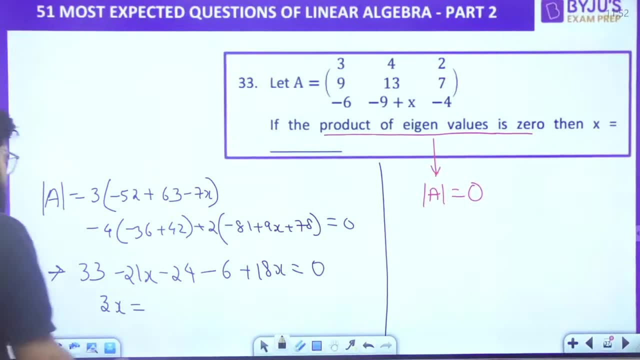 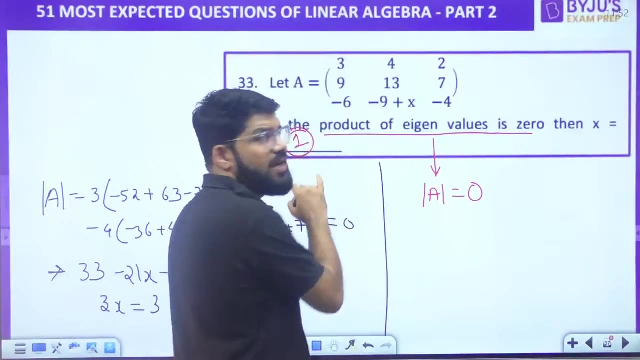 3 into 2 minus 6 plus 18, x equal to 0. so I am getting how much? 3x on the right side is equal to 3. so check key j1: x equal to 1 or I can just hurriedly verify the calculations. are you also getting x equal to? 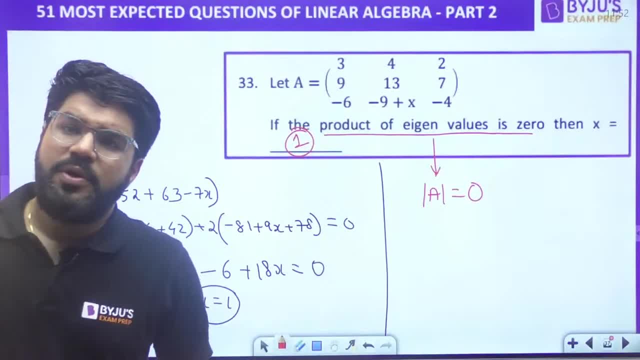 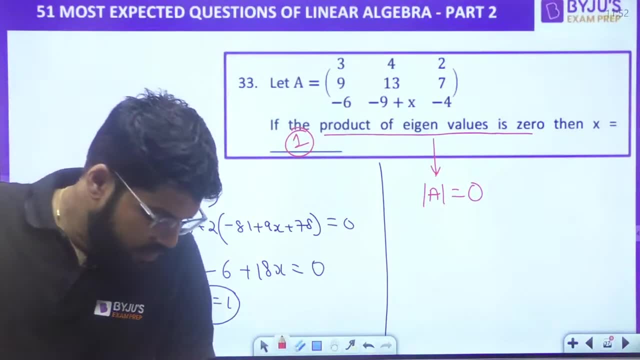 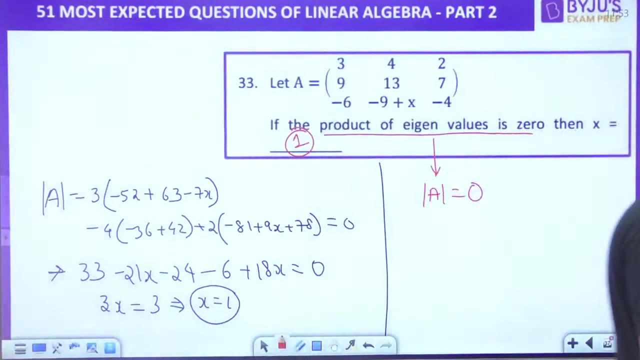 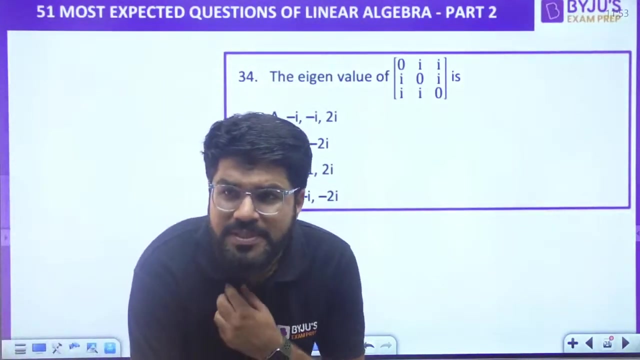 1 or you also getting the x equal to 1 quickly. rectify, right, if you are matching with the answer. keep liking the session. yes, x equal to 1. quickly confirm. yes, confirmed, okay, so number 34, the eigenvalue of this matrix. once again, try to be property specific and simplify the questions. try to be property specific and simplify the question. what about the trace of the matrix? 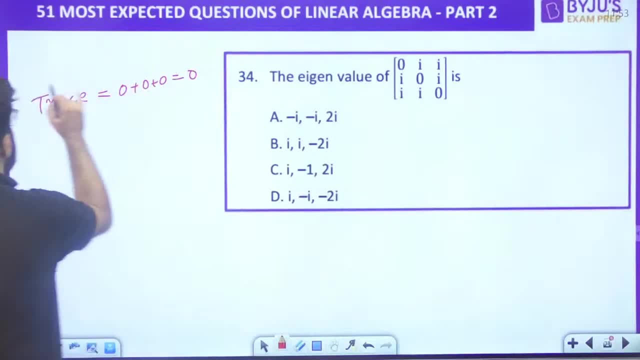 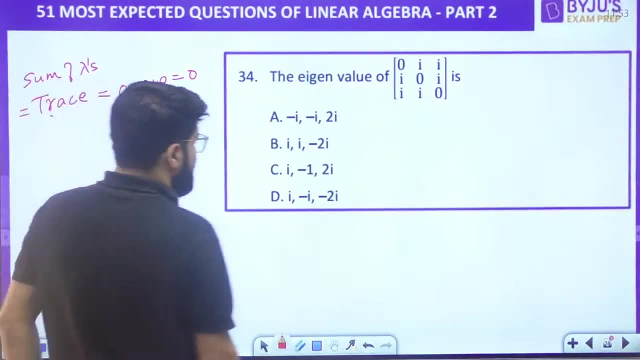 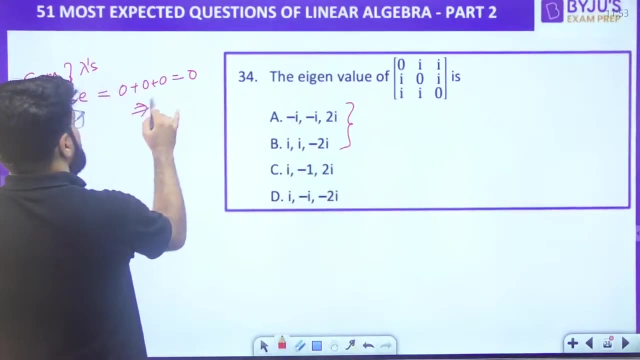 trace of the matrix is 0, zero, zero. that is zero. and sum of the eigenvalues is also equal to zero. right sum of the eigenvalue should be zero. so this is wrong. this is also wrong. so you are left with a and b. this is taking you. 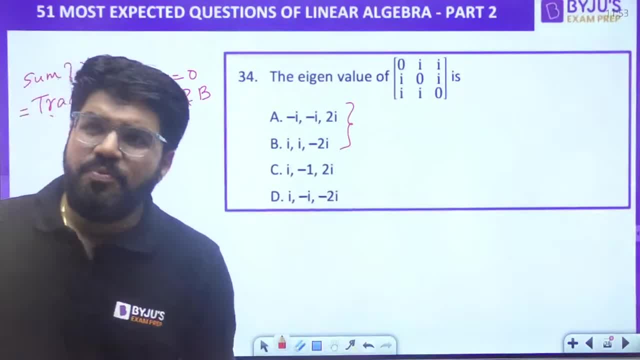 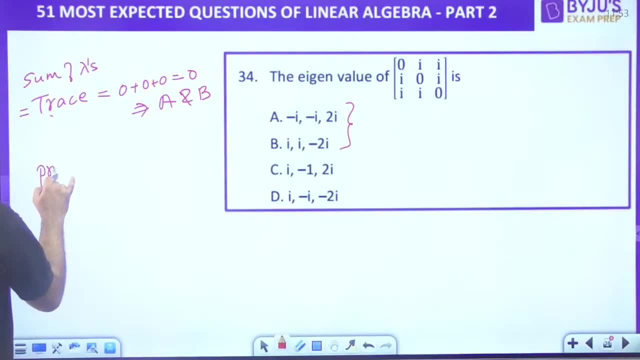 towards a and b right. so i'm not able to comment, so i will try one more property that is determinant, rather than calculating the whole process. that will be lengthy. so now let's simplify this. so what is the determinant? so product of the eigenvalues should be equal to the determinant. 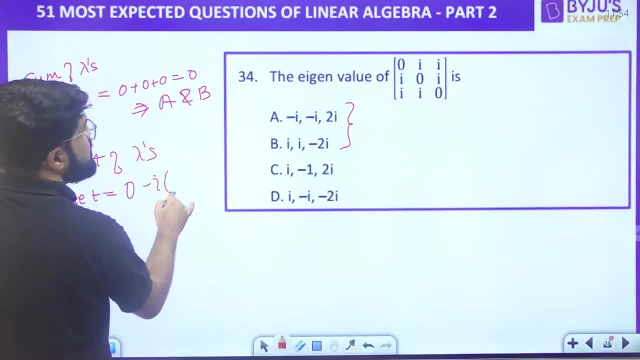 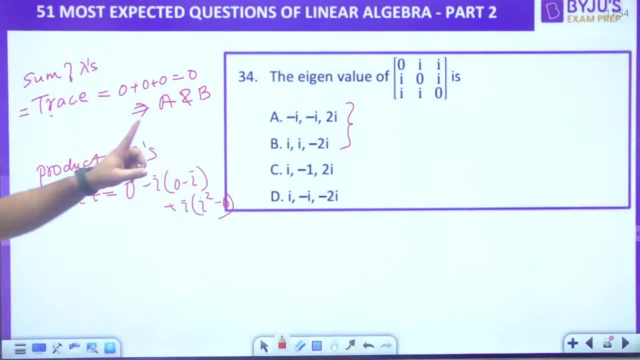 determinant quickly. first part is zero, then minus of i, zero, minus i, plus of i, i square minus zero, minus i, zero, minus i square. sorry. zero minus i square plus of i, i square minus zero. so this looks like minus, minus, plus i cube, plus i cube. this is. 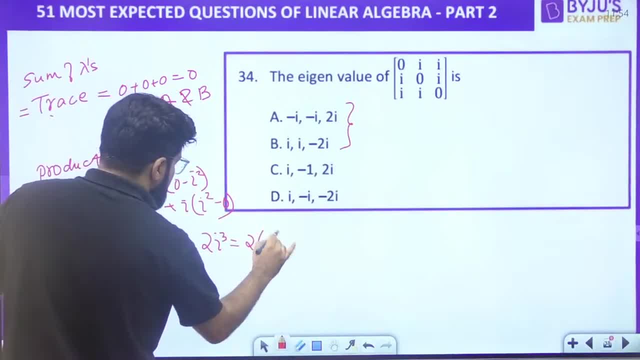 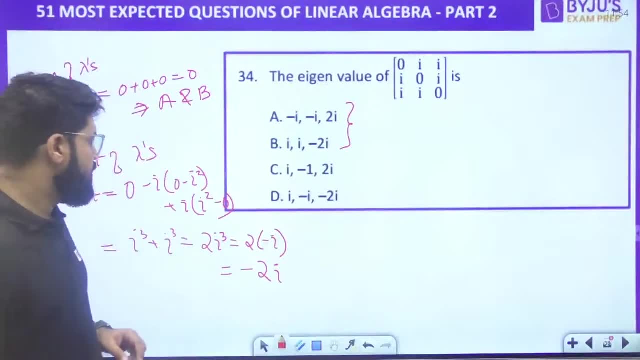 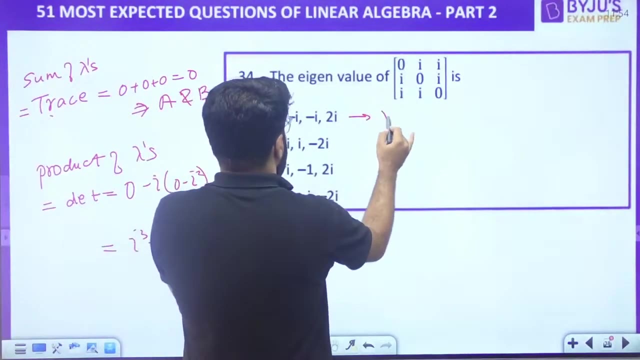 sorry, minus two i cube. i cube is minus i. i cube is given by minus i, so the determinant should be minus two. i determinant means product of eigenvalues. now multiply here. here, if you multiply, only option number a and b has to be tested right. what is the product? minus i into, minus i into two i. 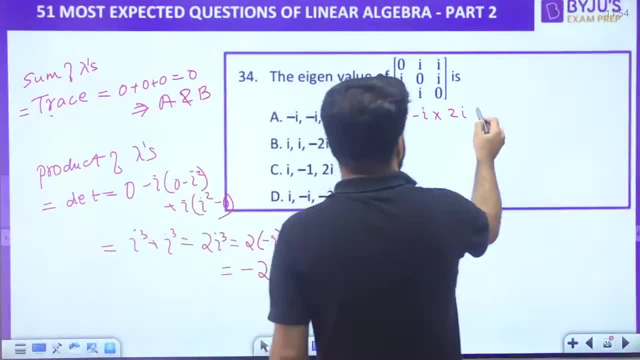 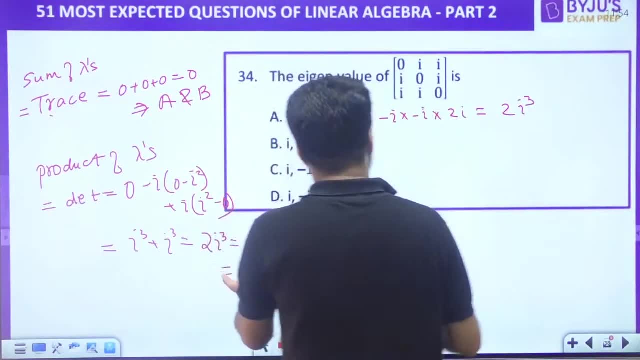 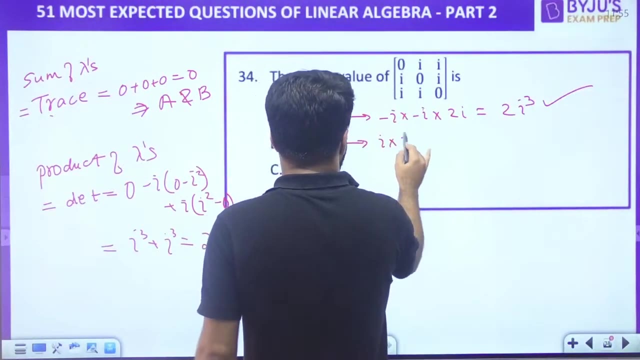 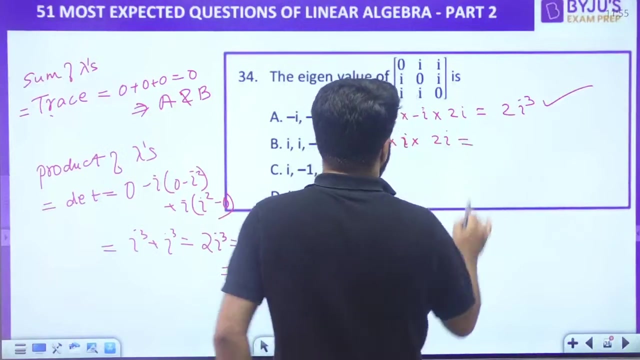 this is minus, minus, totally cancelled. this is total two i cube. yes, this is two i cube, and that is what this is correct, right here. if you take the product here, if you take the product i into i, the board has started creating some problem. now this should be a minus. this is minus two i cube. 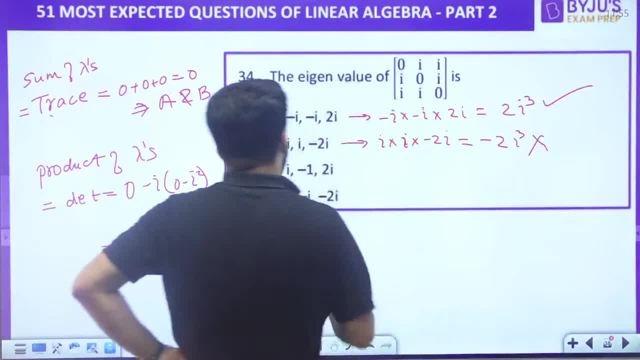 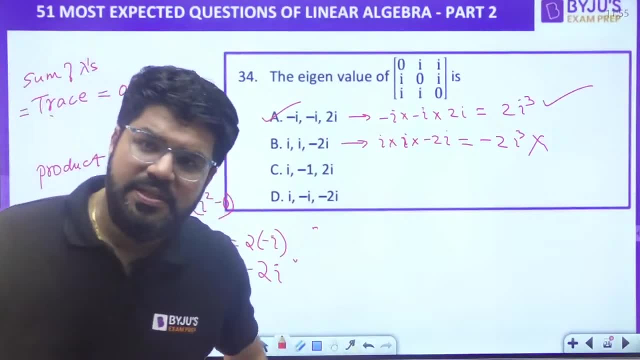 this is wrong. okay, so option number a: everybody rectify. option number a is the correct option by the properties. i am able to deal with many of the questions, although some more questions coming up will be little good also okay, but we are trying to cover all range, all variety of question. 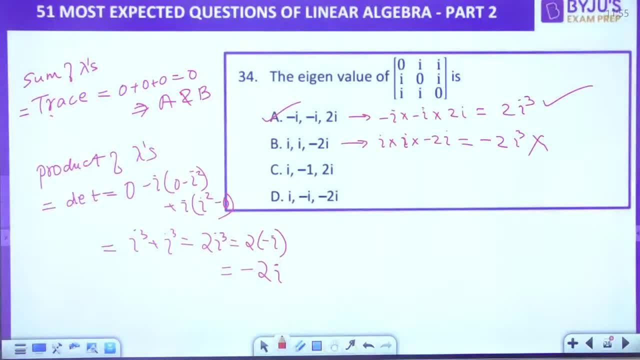 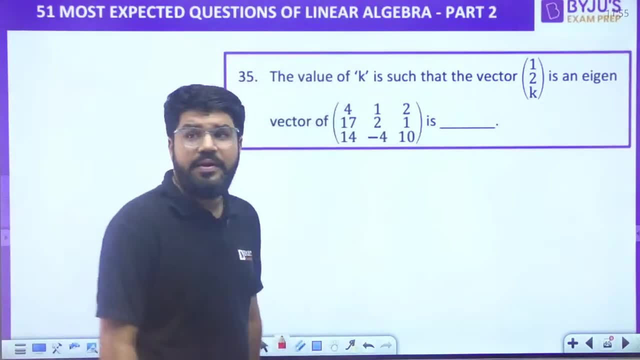 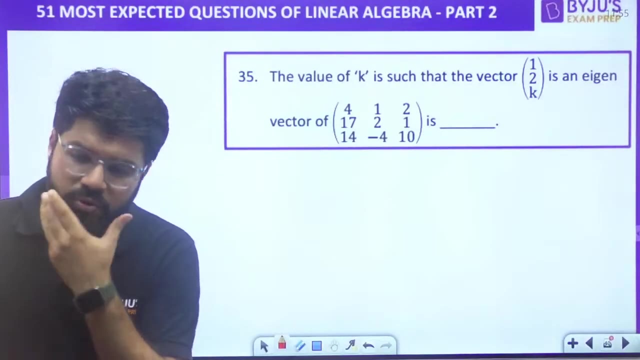 okay, next one, number 35: what is the value of k such that the vector 1 to k is an eigenvector of the given matrix? what is the value of k such that the vector is an eigenvector whenever a question strikes on eigenvector? what you have to do here: whenever a question strikes on eigenvector. 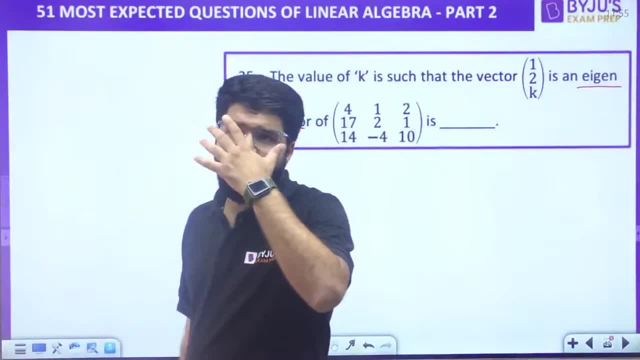 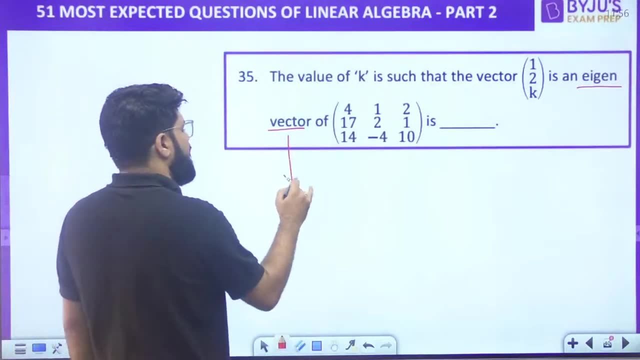 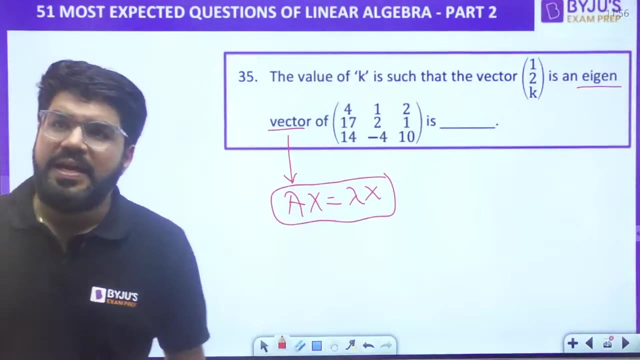 what is the approach you have to follow? what is that approach you must be following? okay, eigenvector, the same approach that i have told you continuously: ax equal to lambda x. ax equal to lambda x. it's a n80 type question. kindly solve everyone and give me the answer. 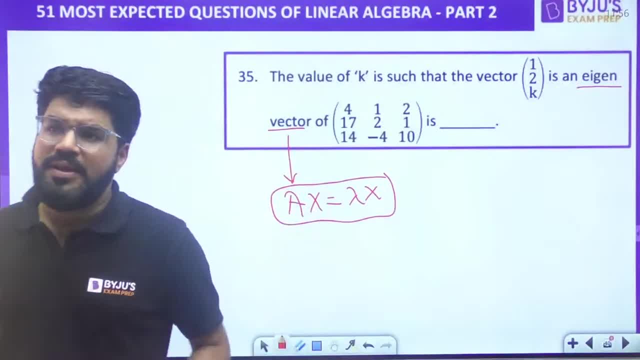 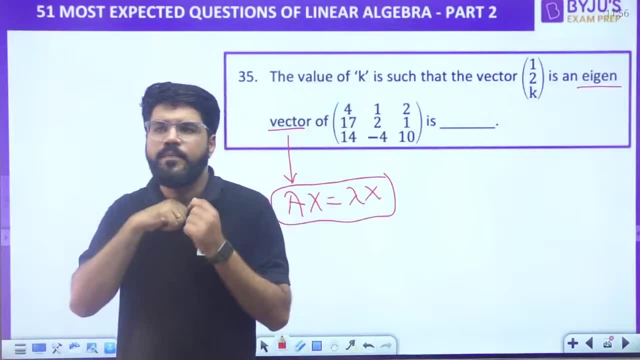 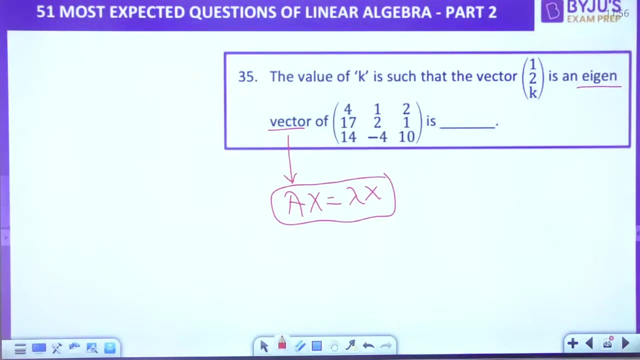 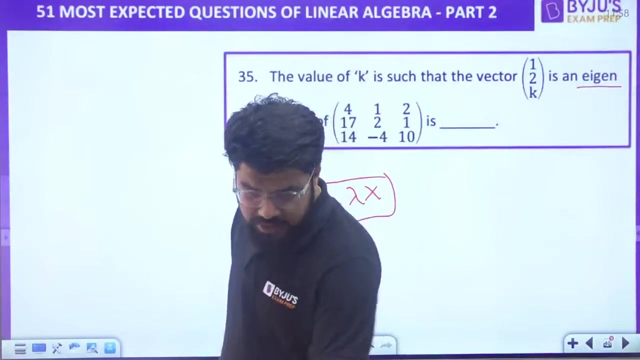 and allow me two minutes. i'll be back two minutes, two minutes or less than that. solve it up and give me the answer quickly. solve it up, give me the answer quickly up and give me the answer quickly. you, you, Yes, dear. so let us check the answer then. 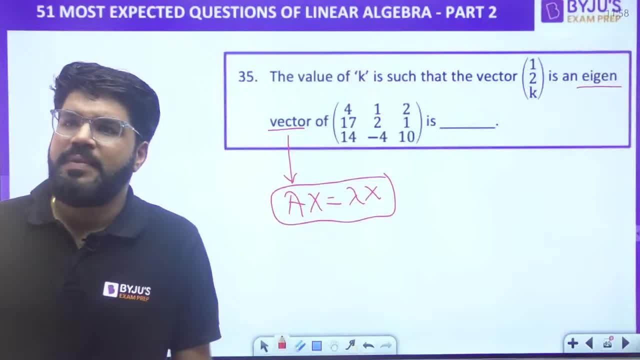 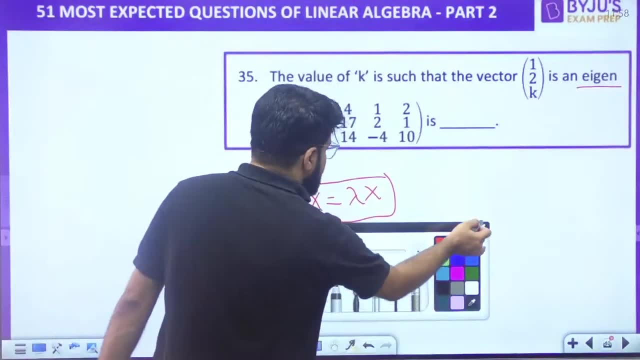 The value of k, such that the vector is an eigenvector of the given matrix. So let us check it up. then Let us check it up: Eigenvector AX equal to lambda X principle will again be applied to let us start solving AX equal to lambda X. 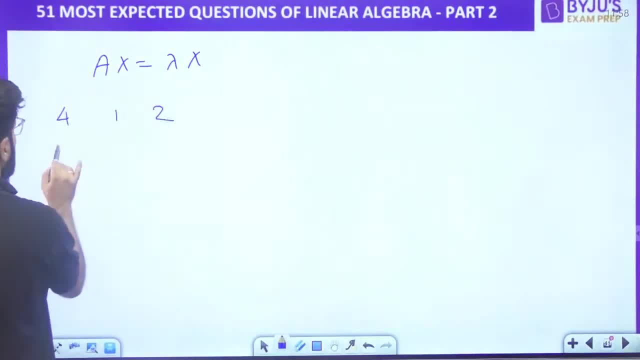 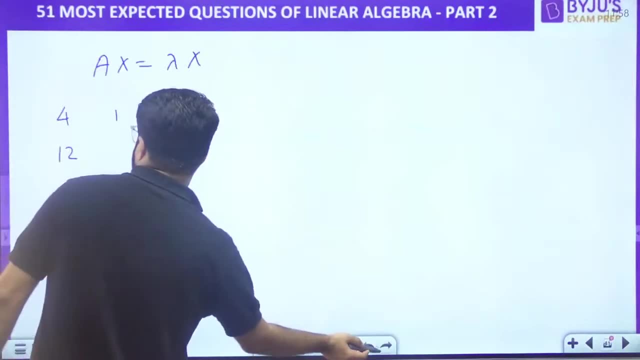 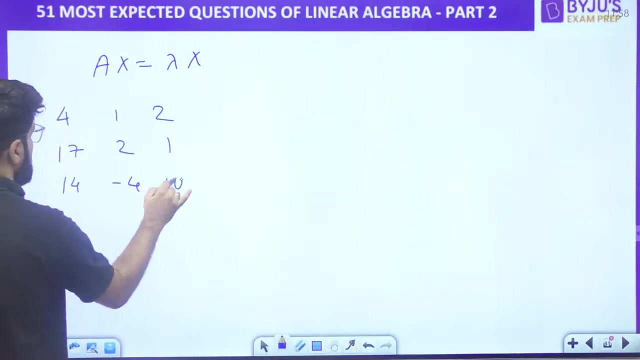 What A matrix. I will just write down: 4, 1,, 2, 12,- sorry, 17, 2 and minus 1, 14, 2 and 1, 14 minus 4 and 10.. Multiplied by the vector X. 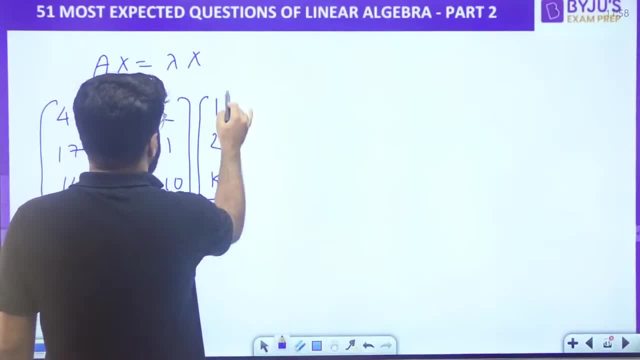 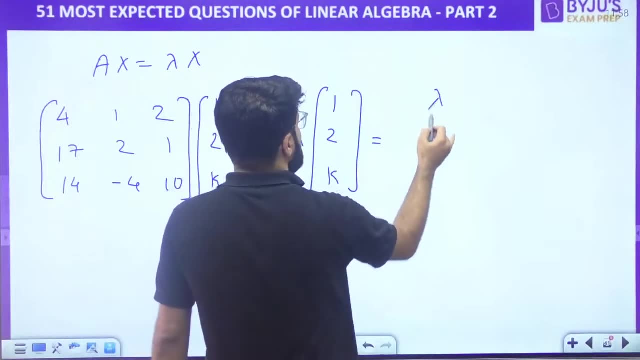 What is the vector that should be eigenvector? 1, 2 and k. For it to be eigenvector, it should satisfy AX equal to lambda X. Multiply the lambda, so it becomes 1 into lambda, 2 into lambda, k into lambda. 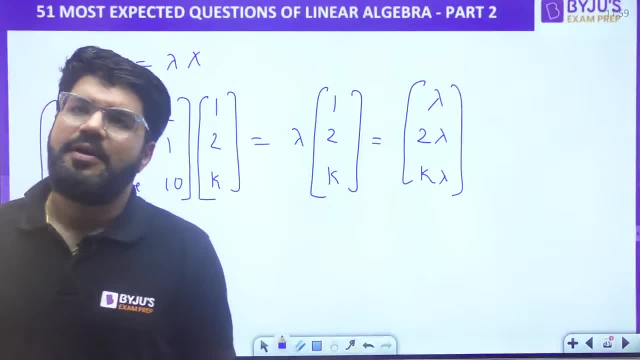 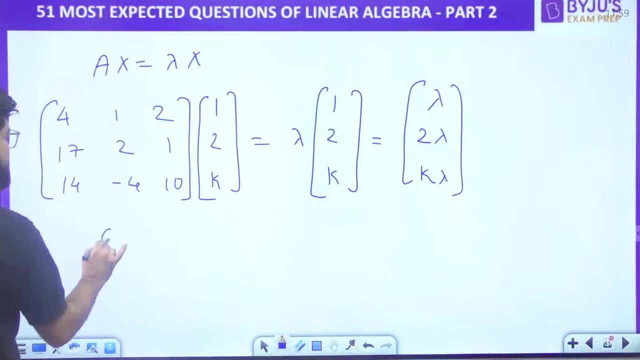 Now equate. How are the two matrices equal? Well, first multiply, left hand side multiply: this is 4 plus 2 plus 2k, that is 6 plus 2k. Then second row: 17.. 17 plus 2 to 4,: 21,. this is 21 plus k. 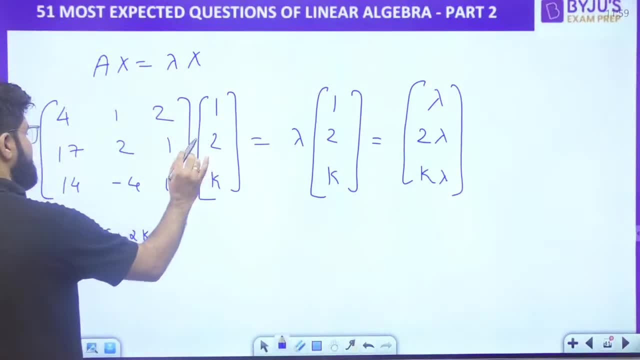 Last third row: 14 minus 8, that is, 6 plus 10k, And this should be lambda 2 lambda and k lambda. Two matrices, yeah, two vectors are equal if all the corresponding elements are equal. If all the corresponding elements are equal. 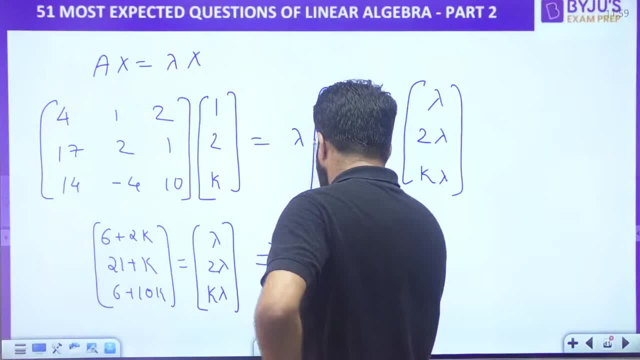 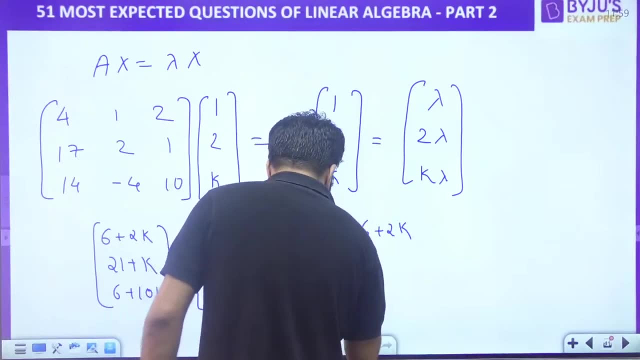 Okay, so here equation will be made, number 1. That lambda Lambda should be 6 plus 2k. But I don't want lambda, I want k. So let us use this equation. Third one we will use: 6 plus 10k is equal to k lambda. 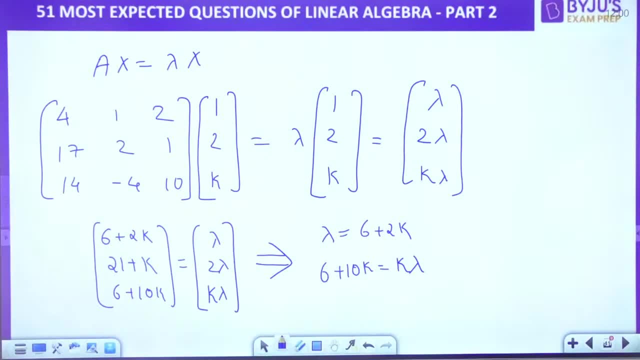 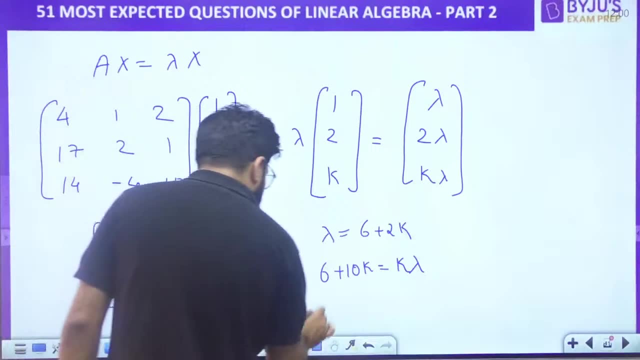 Right. Right Is equal to k lambda Right. Yeah, we will first take the value of k here, So this can become quadratic Right Better. 2 lambda is 21 plus k. Now what is 2 lambda 2 into 6.. 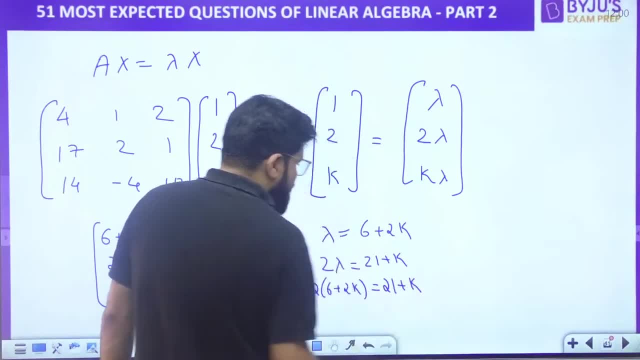 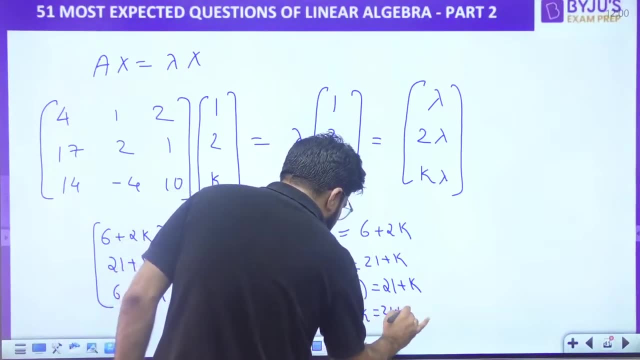 6 plus 2k Instead of lambda. 6 plus 2k is 21 plus k. Rather than going for quadratic, I am finding the value of k. Whatever method, it is all okay. 12 plus 4k is 21 plus k. 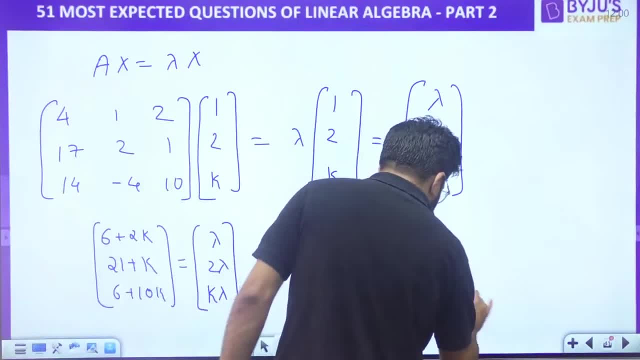 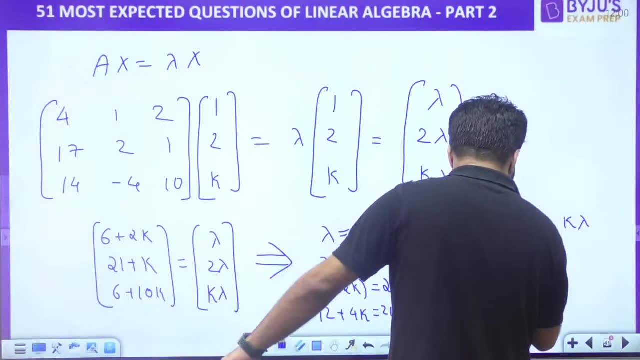 From here, 3k is equal to 9.. k is equal to 3.. k is equal to 3.. Now take the third element: 6 plus 10k is equal to k lambda. So 6 plus 30 is equal to 3 lambda. 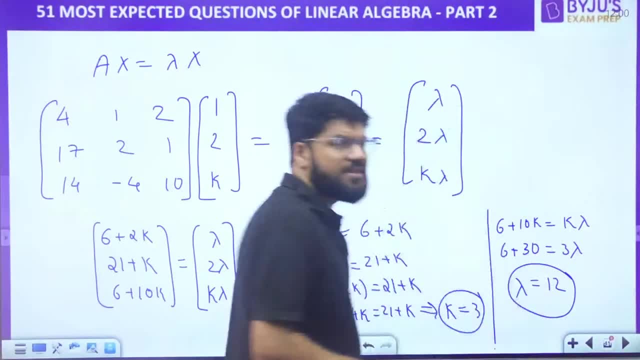 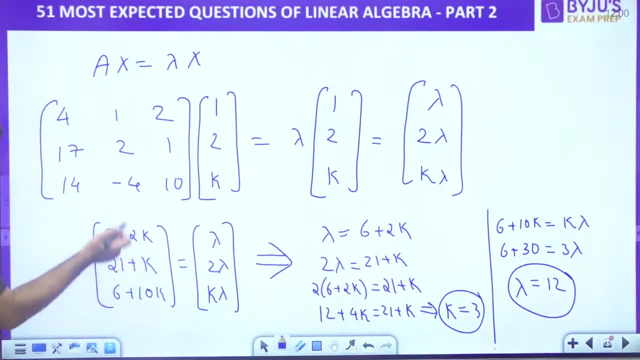 So 3 lambda is 36.. Lambda is 12.. Got this, Lambda is 12.. First, we have found the value of k by the first and second parts. Okay, This is lambda. This is 2 lambda, So we have equated them. 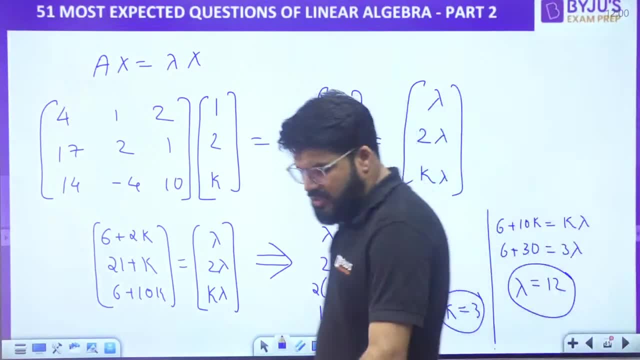 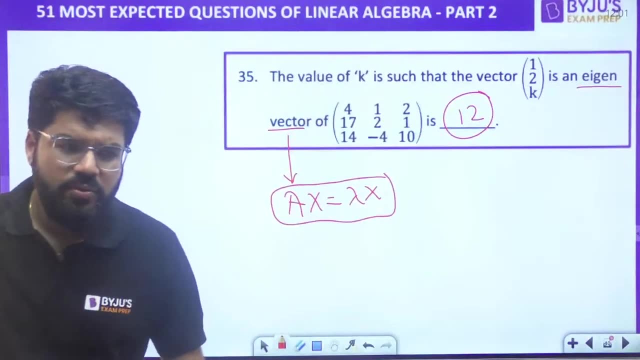 Okay, Okay. So, guys, again I tell you this is an entity type question. Again I tell you, any question based on eigenvector, just stick to ax equal to lambda x, Just fix to the ax equal to lambda x. 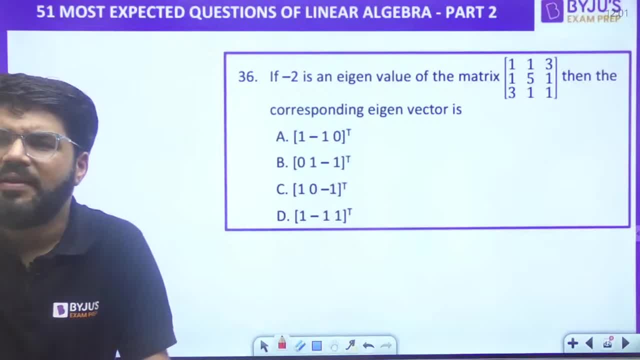 If minus 2 is an eigenvalue of the matrix, then the corresponding eigenvector, then the corresponding eigenvector of the matrix is the eigenvector of the matrix. So it's not like you have to, you know, search for minus corresponding to minus 2.. 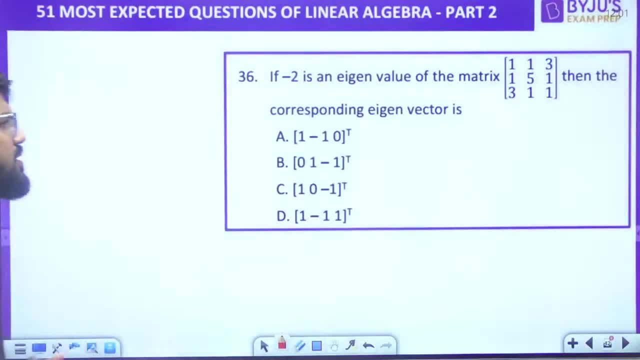 You just go with the options Again, follow the same method. Again, follow the same method. See. this question may give you an intuition. Let us apply method number 2 minus method number 1, the basic method Minus 2 is an eigenvalue. 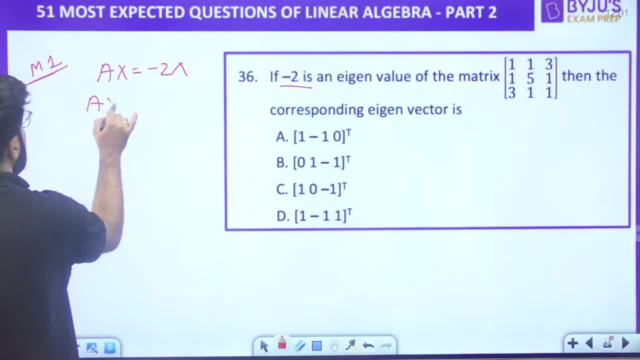 So ax equal to minus 2x, Yeah, ax plus 2x equal to 0, or a plus 2i into x equal to 0.. a is given to you, You add a plus 2y and then solve the equation right, and then solve the equation. 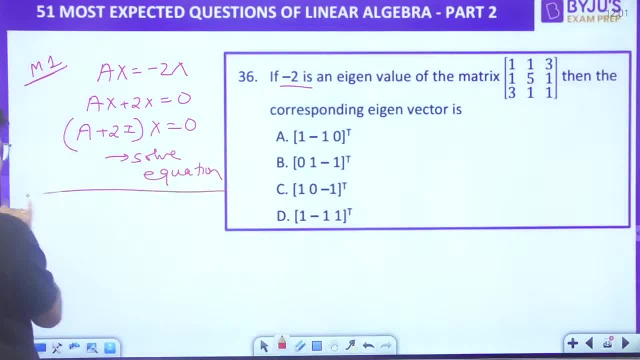 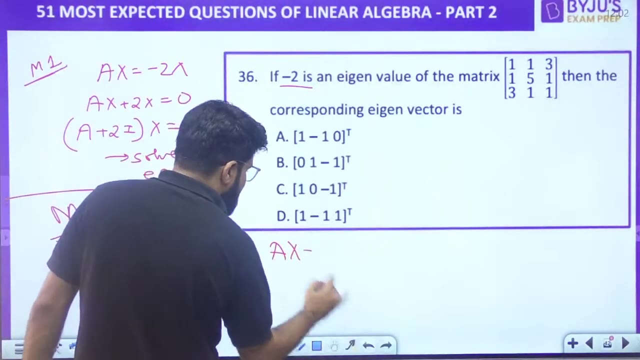 This is one method. No, Okay, this is one correct method. But what is my method? again, My method is again as per options. Options may ax equal to lambda x right, or ax equal to minus 2x. You have to just verify. 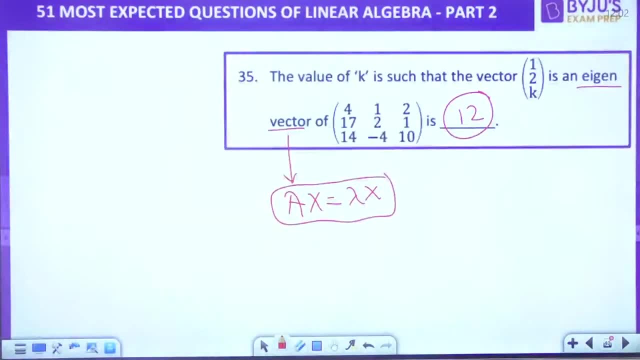 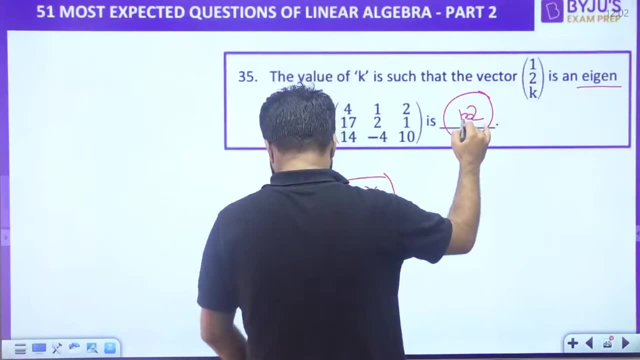 The same procedure, right, So there's the k value for the The previous question. Okay, there's the k value. I'm sorry, There's the k value, Just a second. The k value is 3.. The k value is 3.. 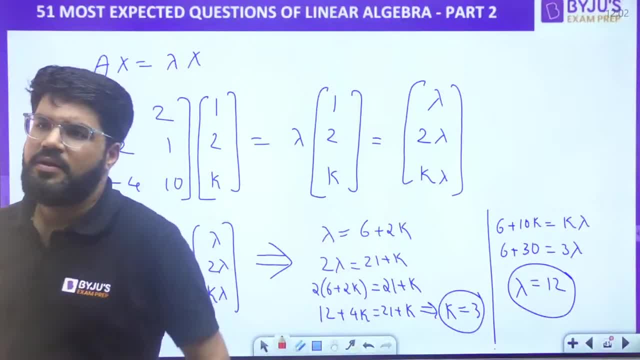 Then we can stop here also, But still, lambda is also. Okay, we can find Correct, k is equal to 3.. Correct, Okay, so we have found both. anyways, They can ask anything, k or lambda, What is the corresponding lambda? 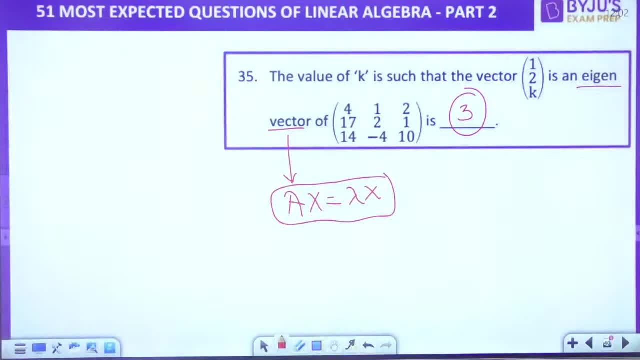 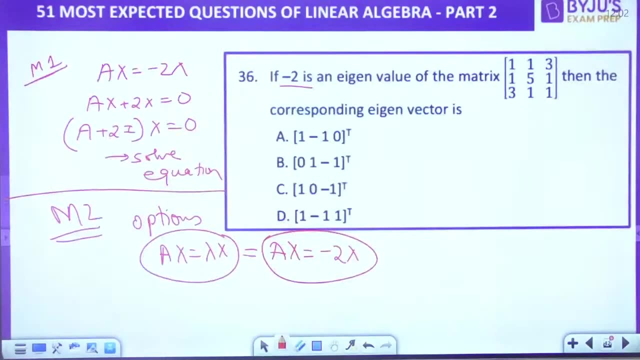 But they asked the k, So k was equal to 3.. Simple, Right. Good morning TI, RB, Polly. Okay, let's go. Yes, So where we are up to? So again, we have to just cross check the options. 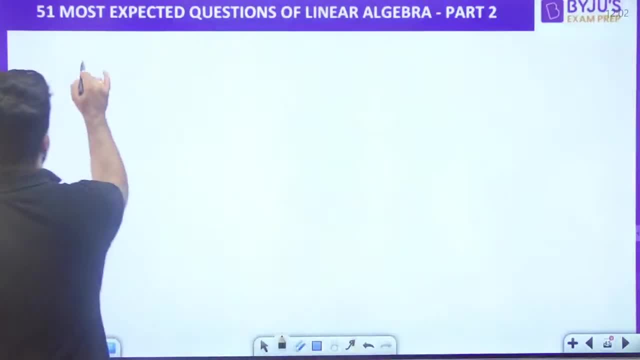 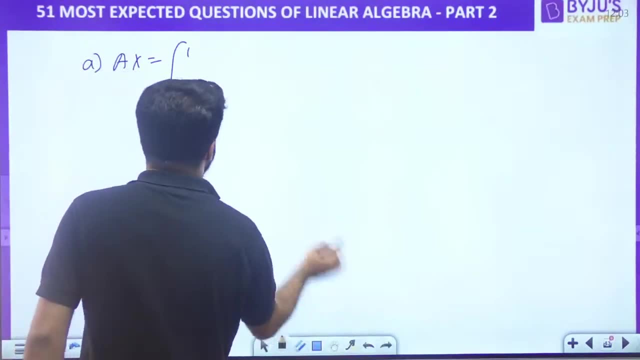 Nothing much So. option number a. I'll just start with the option number a. as always, Ax The a matrix is given to me: 1, 1, 3, 1, 5, 1.. 1 and 5, 1, 1.. 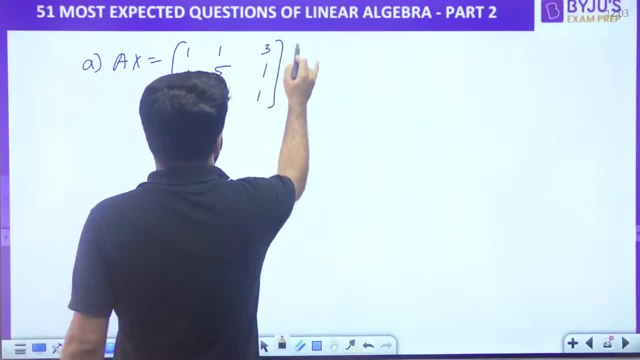 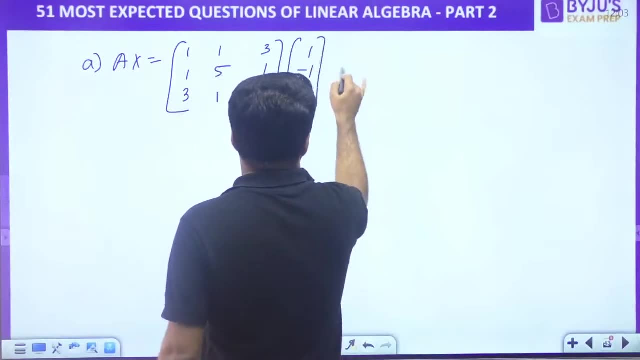 1, 1, 3, 1, 5, 1, 3, double 1.. Multiplied by the x, What is the x? 1 minus 1, 0.. This is equal to how much? 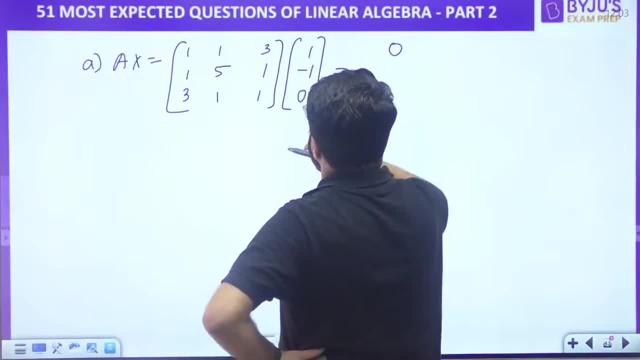 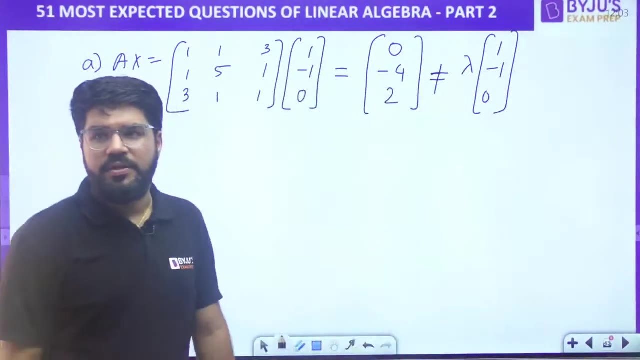 Okay, 1 minus 1, 0. Then 1 minus 5 minus 4.. Then 3 minus 1, 2.. Is it somehow equal to lambda into x? No, this is not an eigenvector only. 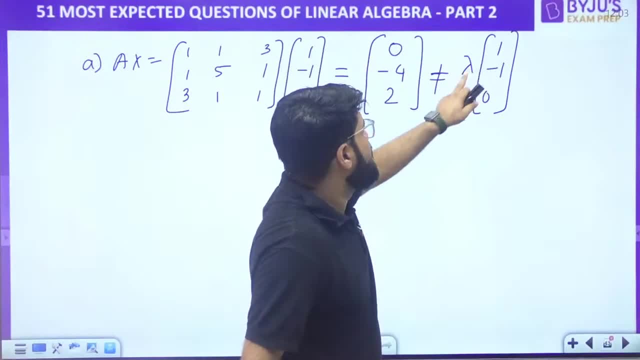 This is not an eigenvector: 0. If this is okay. if this is equal, lambda should be 0. And if lambda is 0, all elements will turn to be 0. This is not satisfying, Okay. Option number b: 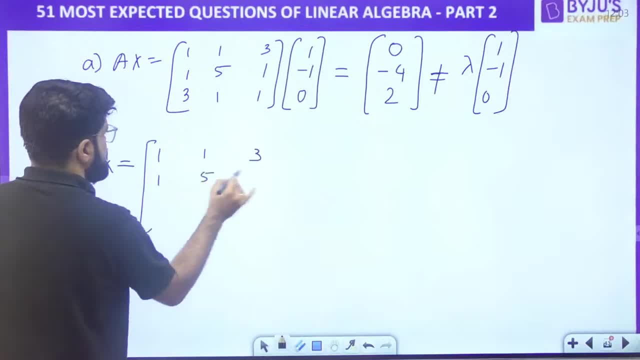 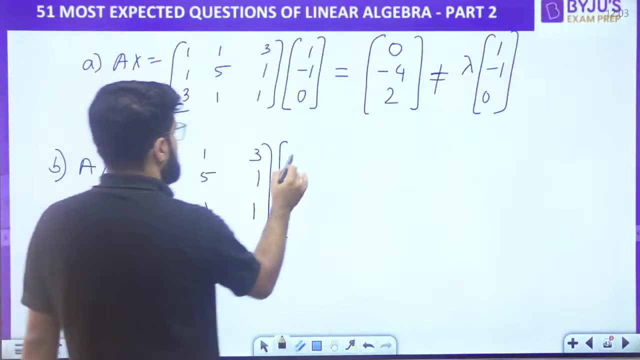 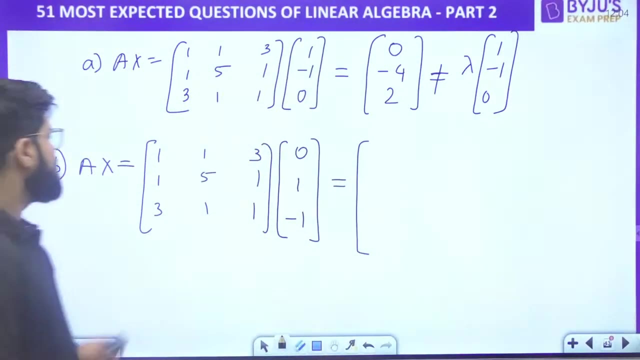 Ax x, x, x x. 0, 1, minus 1.. 0, 1, minus 1.. This is equal to how much? This is equal to how much This is: 0, 1, minus 3, minus 2.. 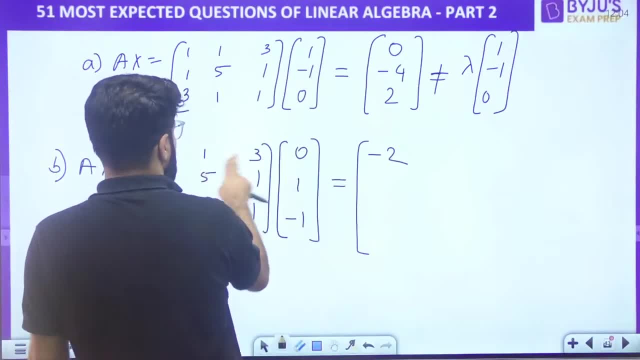 0, 1, minus 1.. This should not be 0, 1, minus 3.. Okay, And this is 0. 5, minus 1, 4.. And last, 1, minus 1.. 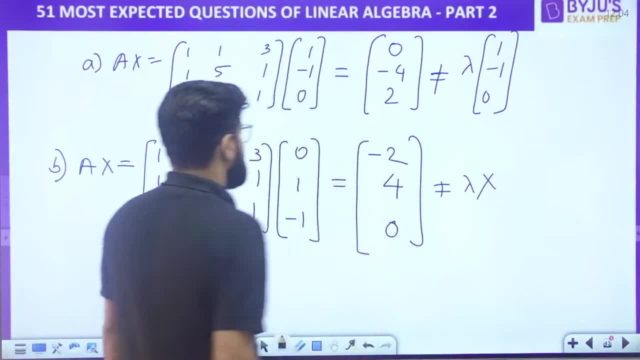 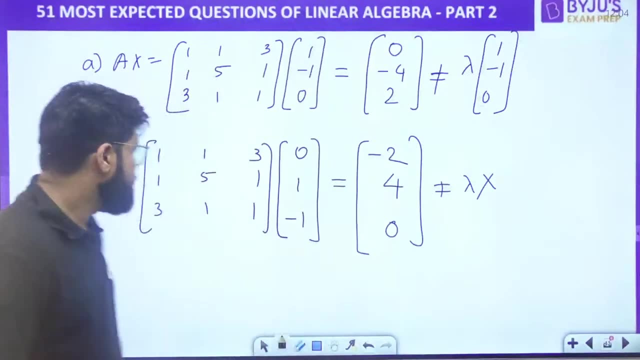 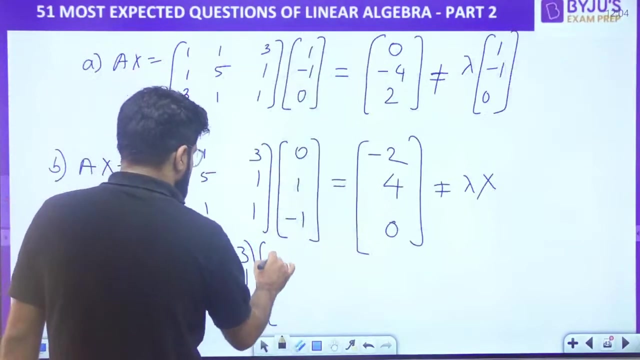 This is 0.. This is also not equal to lambda x. This is also not equal to lambda x, Correct? Let's check option number c once. Right, Option number c. Let us check once: 1, 0, minus 1.. 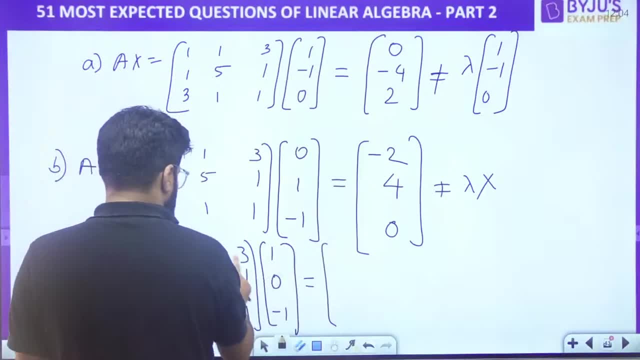 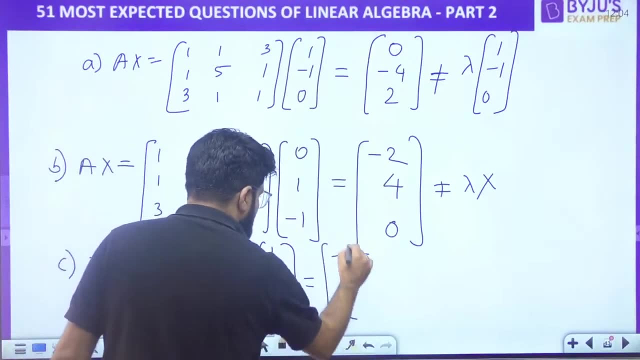 Cross check here: first, one 1, and minus 3, minus 2.. This is 1 and minus 1.. This is 0. This looks good: 3 and minus 1.. This is 2.. Now, what I can do here is what I can do here is: minus 2 can be taken outside. 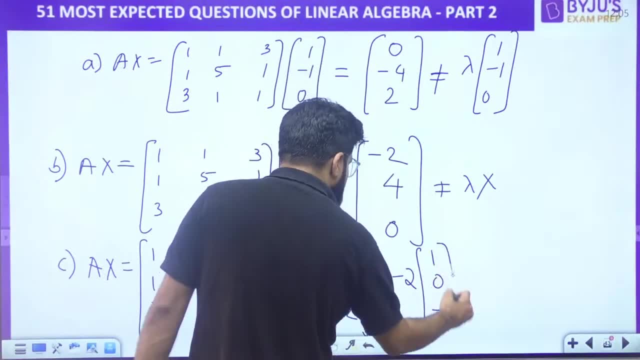 Minus 2 is taken common, So you are left with 1,, 0, and minus 1.. And that is what is the given vector x. This is equal to minus 2 x, And that is what you actually want. 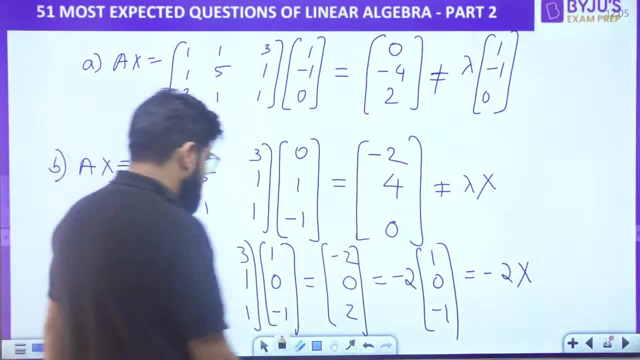 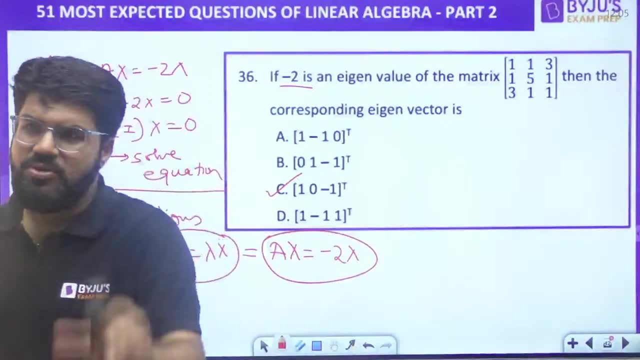 This is equal to minus 2 x, And that is what we actually want. ax equal to minus 2 x. So the correct answer for the question is c, 1, 0, minus 1. transpose: It is given in rows. 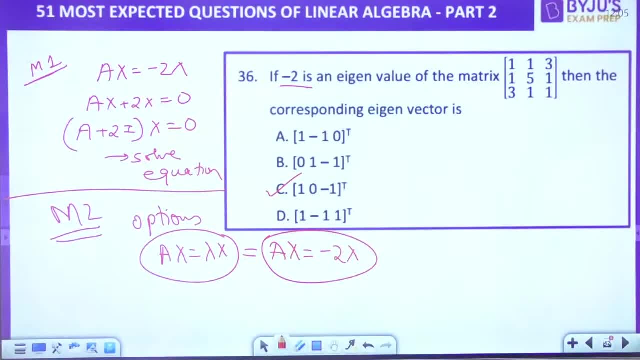 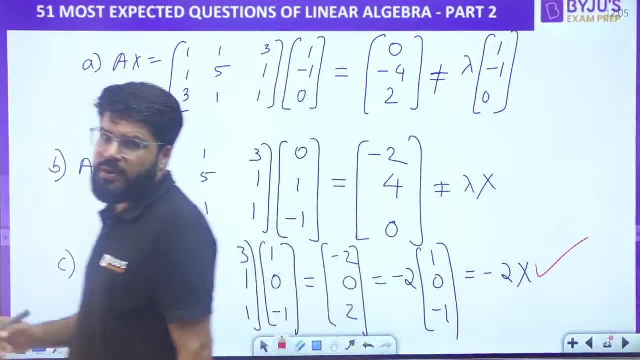 So transpose means it is the column Correct. Okay, So we want the eigenvector corresponding to minus 2 only, And c is the correct answer. Ax equal to minus 2 x. we want Right. Ax equal to minus 2 x. we want. 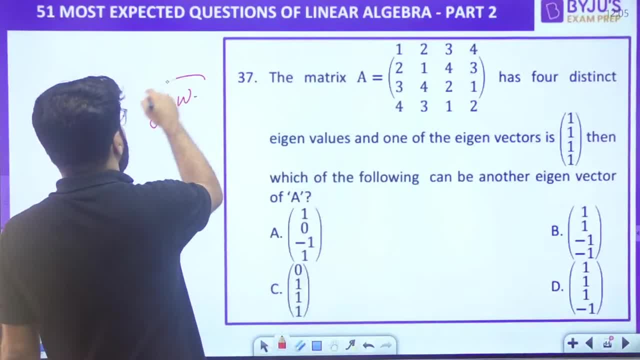 So one more question on eigenvector. Kindly take it as homework. Like yesterday also, I gave you homework. Okay, 2, 3 questions, I will give you homework also. This is the question number 37 as homework for you. 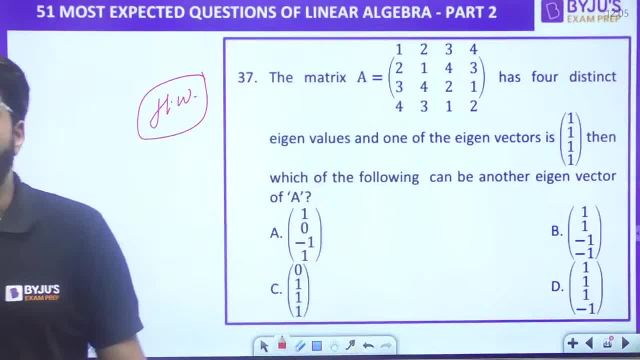 Again related with eigenvector. So try to follow the same approach. Try to follow the same approach. Try to follow the same approach. Has 4 distinct eigenvalues and one of the eigenvectors. No, No, You should not have the same approach for this. 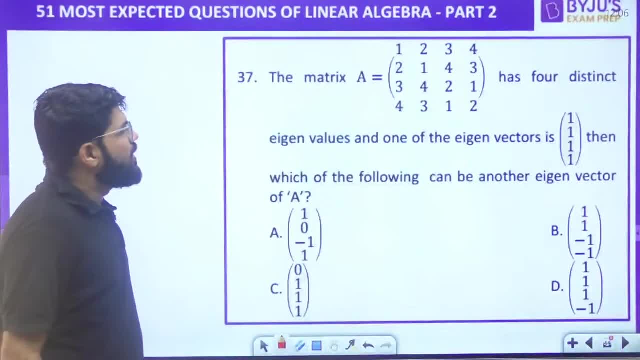 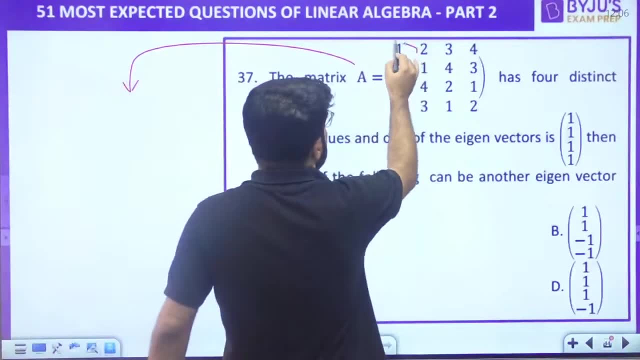 You don't need the same approach for this. Forget it, We will discuss it. Okay, See what is the type of matrix. What is the type of matrix? What is the type of matrix? Everybody, please see What is the type of matrix. 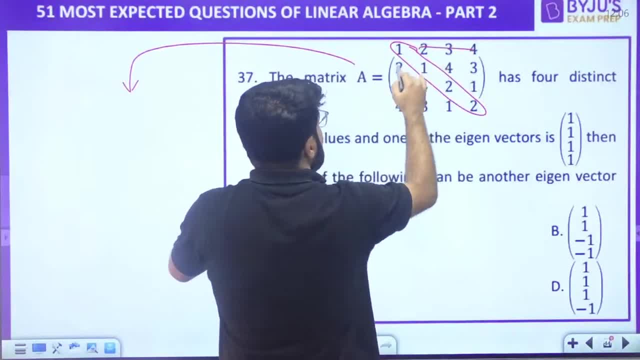 The elements above the diagonal, below the diagonal: 2, 3, 4, 2, 3, 4, 4, 3, 4, 3, 1, 1.. Elements above and below the diagonal are identical or mirror image of each other. 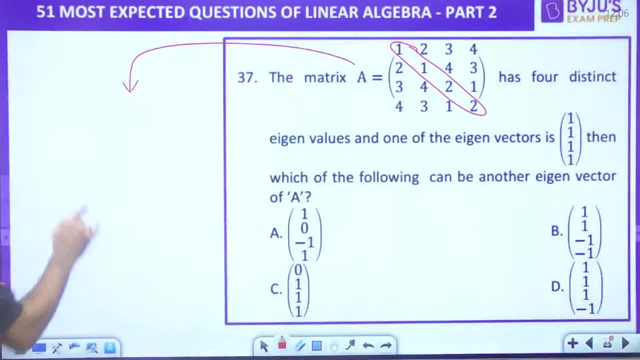 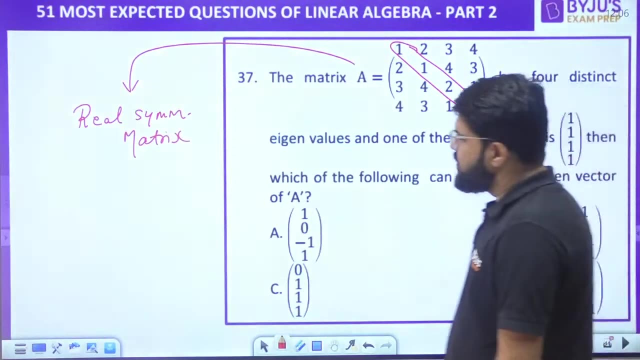 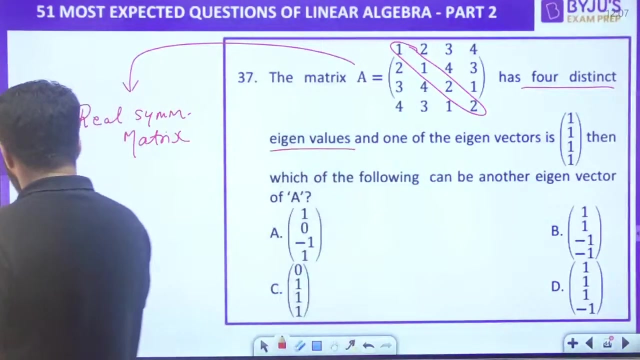 This is a symmetric matrix And that too, real. This is what This is: a real symmetric matrix. This is known as a real symmetric matrix. This is a real symmetric matrix And all eigenvalues are distinct. Has 4 distinct eigenvalues. 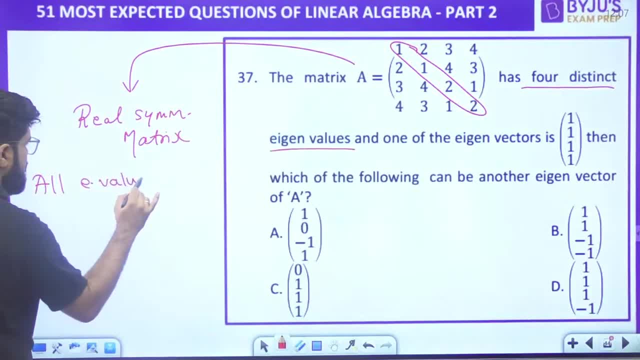 Right, Right. Okay, So all eigenvectors should be orthogonal to each other. Right Orthogonal means x1 transpose x2.. The dot product is 0.. Now how do you take the dot product? Now I can tell you. 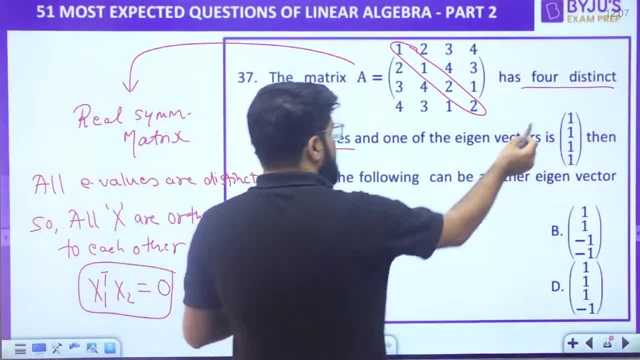 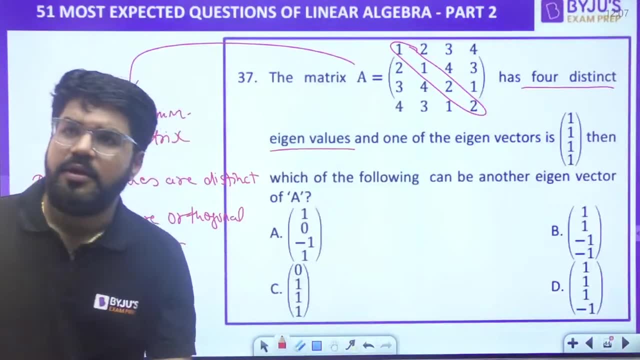 Now I can solve it orally. Now I can solve this simply orally. Take the dot product with option number a: Right. What is the dot product here? How do you take the dot product First to 1st component, 2nd to 2nd component, 3rd to 3rd component, like vector dot product? 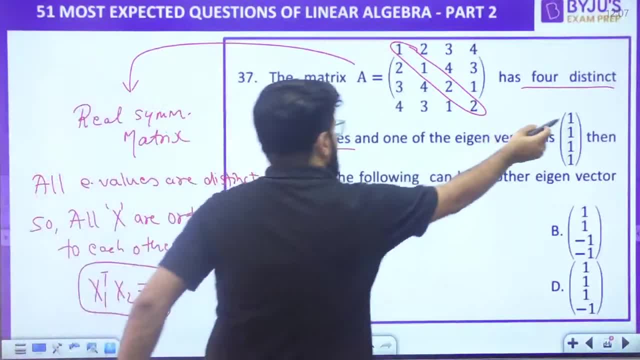 X to x component, Y to y component. Okay, So this is done: 1 into 1.. Then 0.. Then 1 into minus 1.. Then 1 into 1. Plus 1. This is total not equal to 0.. 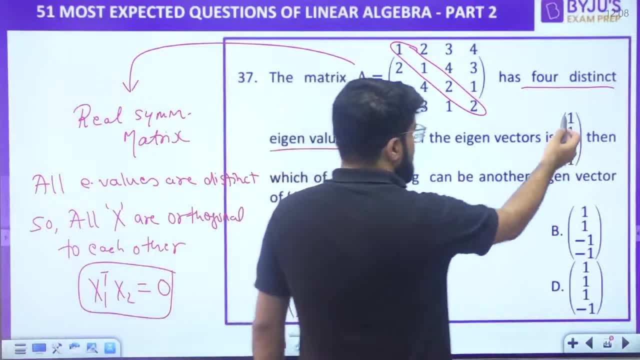 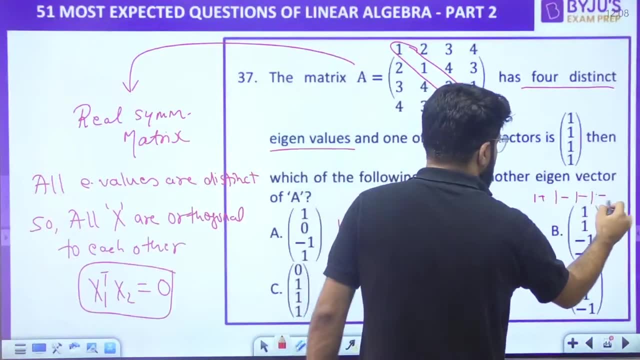 Right. Try with the option number b: 1 plus 1 into 1.. 1 into minus 1.. Then 1 into 1.. Then 1 into minus 1.. Then 1 into 1.. into minus one. last may have one into minus one. yeah, yeah, zero. so this is the. 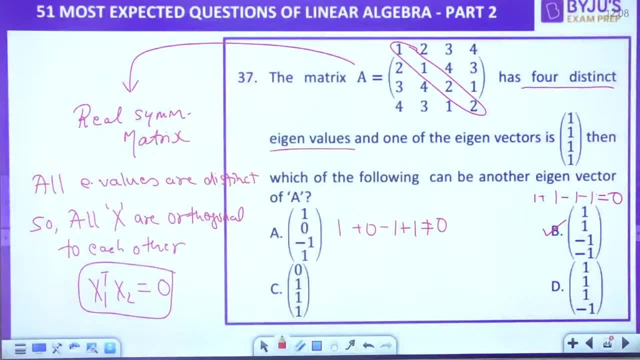 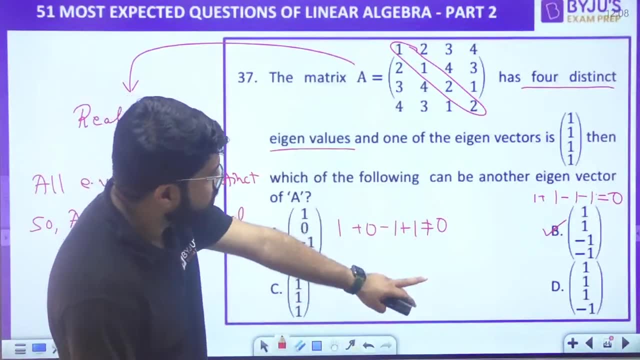 correct answer. which of the following can be another eigenvector? option number B. option number B: Baki, maybe checker language. this is 0 plus 1 plus 1. this is also not equal to 0. that is also 1 plus 1 plus 1. 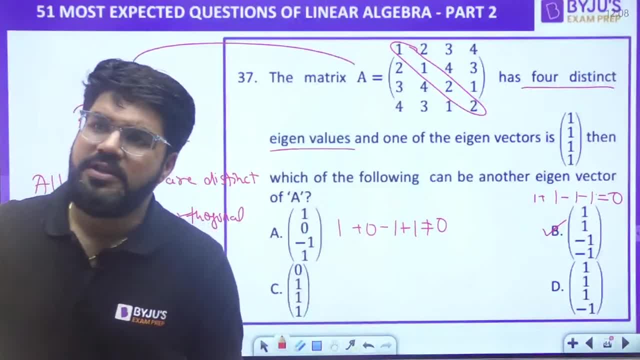 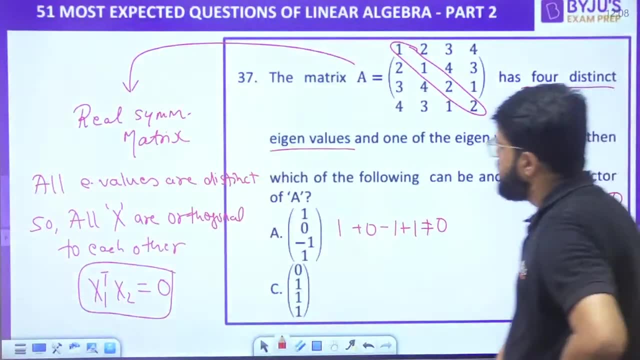 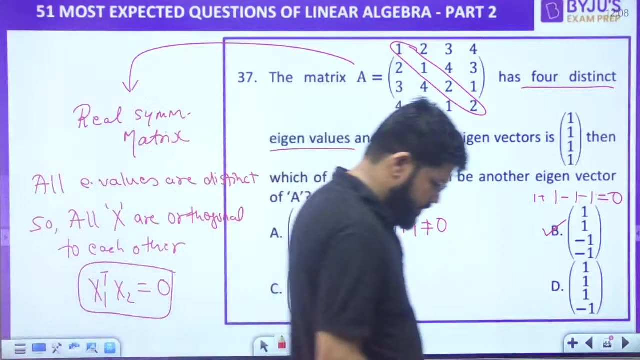 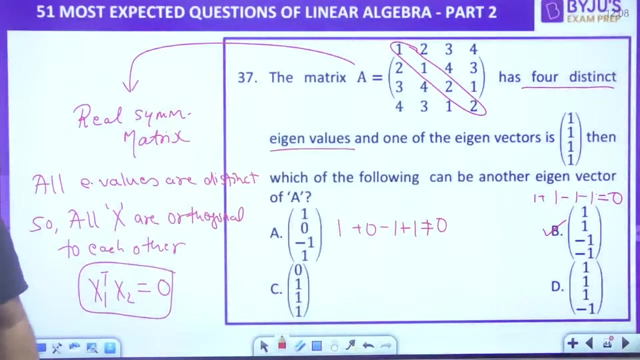 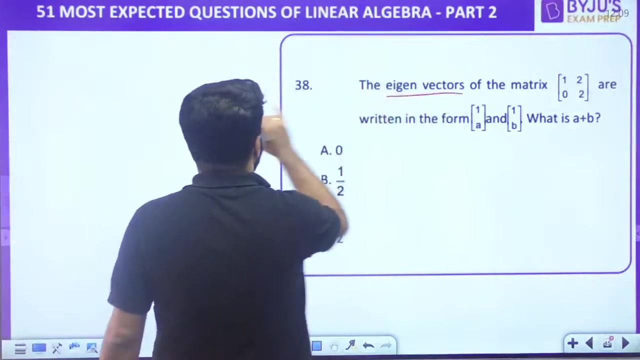 minus 1, that is not 0. option number B match did say MCQ question finished. yeah, so this is not on the regular approaches. let's discuss Kalia, right, okay, everybody, okay, everybody. B is the query correct answer. okay, let us move to the next question. so love a question. it's eigenvector, regular question, so I 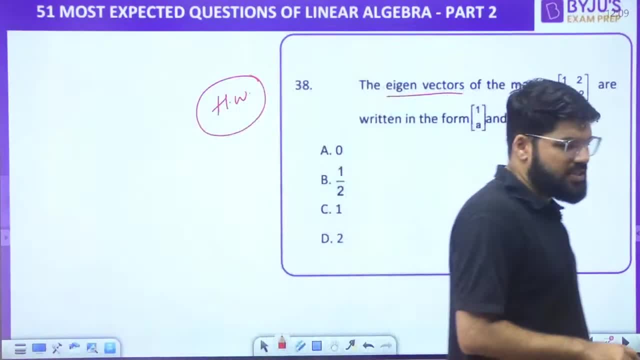 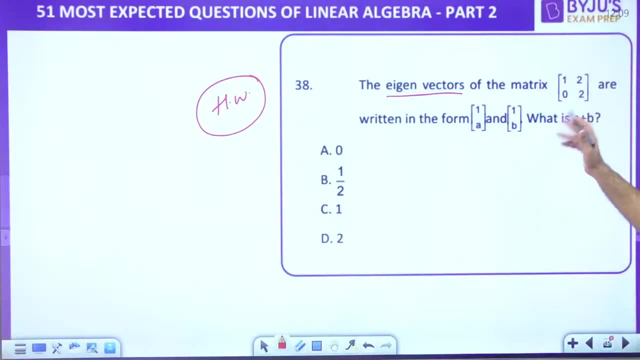 shall give you this question as homework. please kindly take this question as homework. the last one was done, okay, eigenvectors at. so this you have to take by a X equal to lambda X. the two eigenvectors are in the form of 1 by a, 1 by B. what should be the value of a plus B? if you want the? 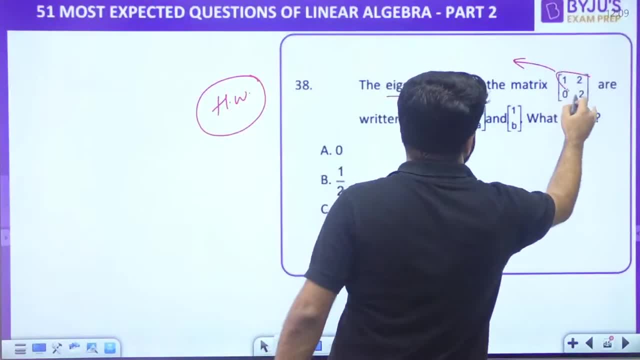 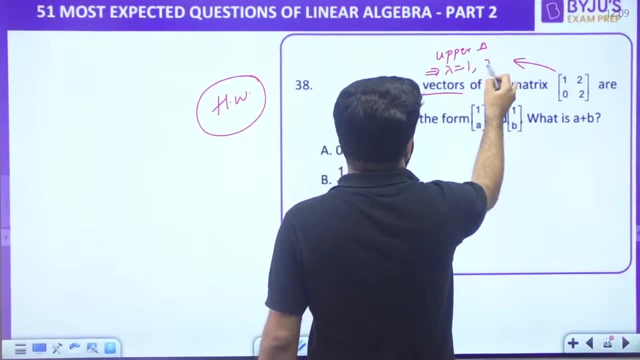 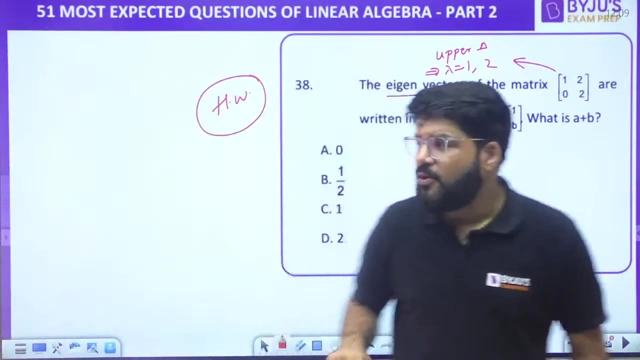 eigenvalues of this matrix. this is what type of matrix? this is the upper triangular matrix. what does a hint, a DMA now go? this is upper triangular, so what are the eigenvalues? diagonal numbers. the eigenvalues are diagonal numbers. that is 1 and 2. that is 1 and 2, take it, oh yeah, up. 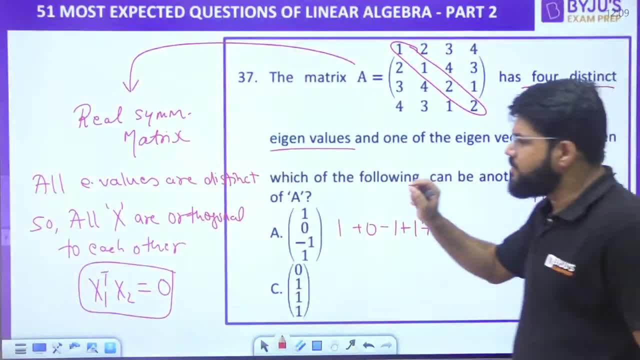 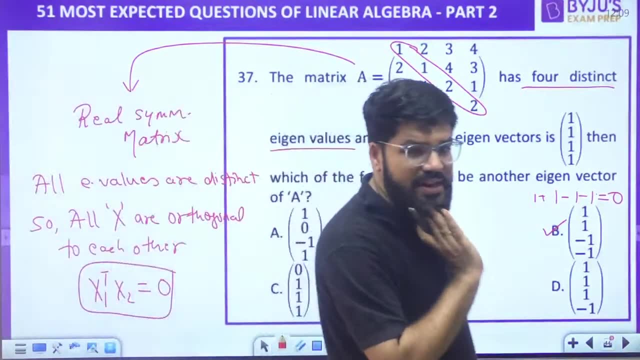 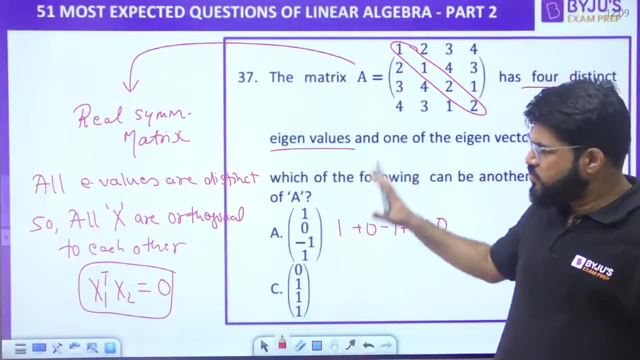 K home, bakuga. now, in the previous question I have used the concept that all X are orthogonal to each other. all the X are orthogonal to each other because all eigenvalues are distinct. for a real symmetric matrix, for the real symmetric matrix. now there is okay, this we have solved easily. there is one question that 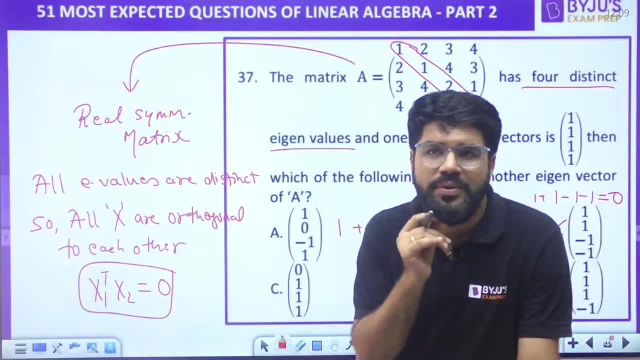 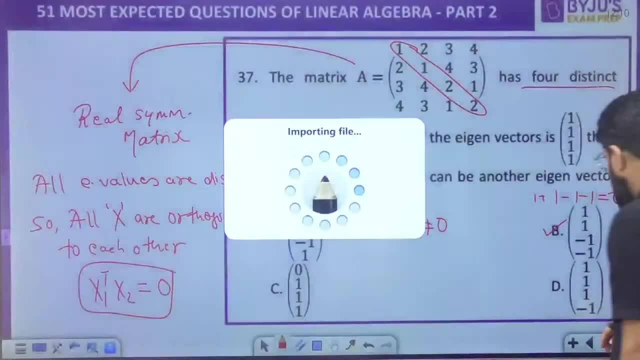 has come up in the gate and I call it as a good question, good conceptual question, and I have brought that question specially for you. let us discuss one gate question also. I want you to understand that because it is related on this. so let me change the sequence for a moment. let me change the sequence. 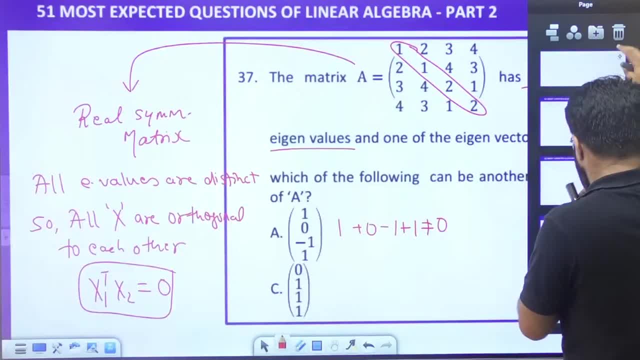 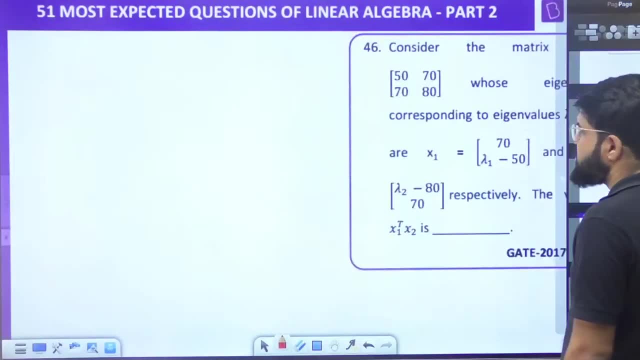 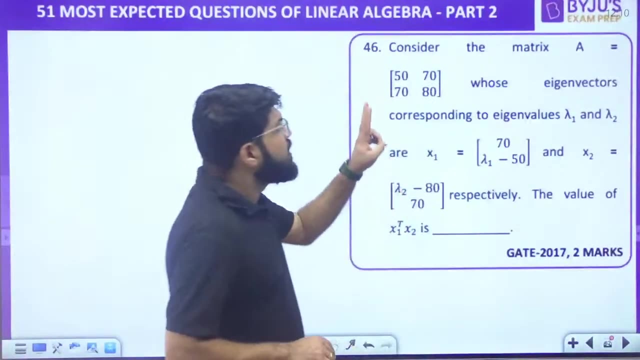 for a moment. let's come to for question number 46. I have that here. I want you to see this question. it's a gate question. I am intentionally discussing a gate question here. consider the matrix a given to you, whose eigenvectors corresponding to eigenvalues lambda 1, lambda 2 are X 1 and X 2. find the. 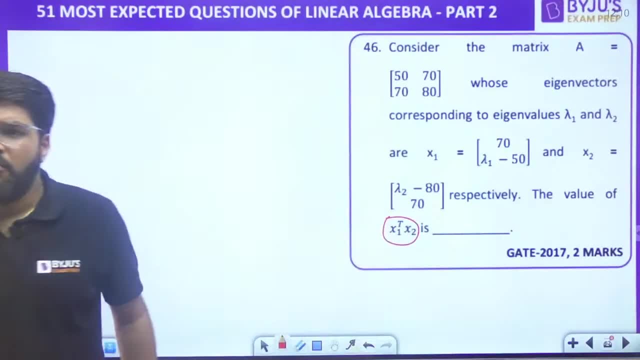 value of X 1 transpose X 2. find the value of their dot product inner product: X 1 transpose X 2. find the value of X 1 transpose X 2. come on, let's discuss this question. so there can be two, two methods here. okay, one is the direct method. 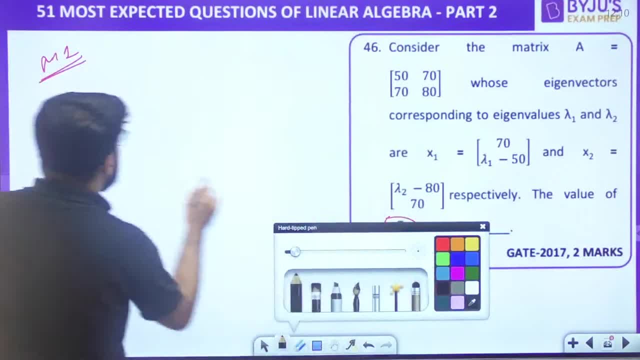 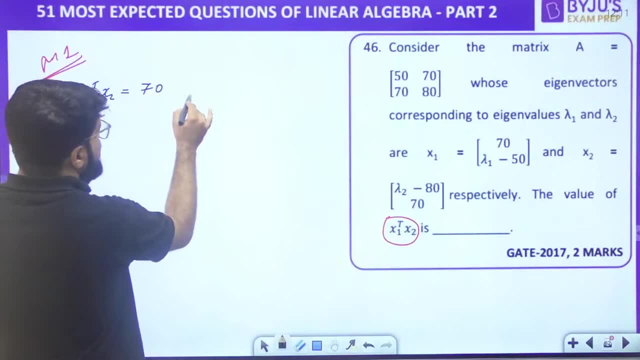 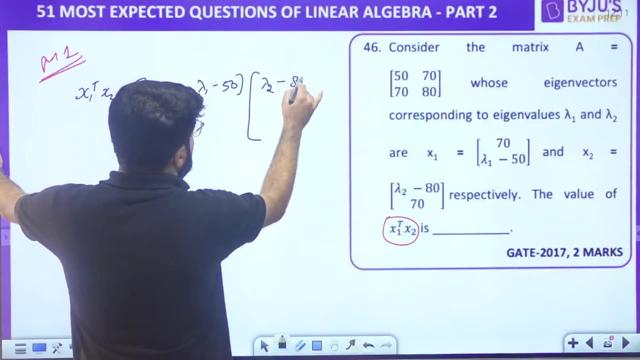 directly somebody. they have no property clicks now. direct is what they need. X 1. transpose X 2. what is X 1? transpose its column. convert into row, so that is 70 and lambda 1 minus 50 multiplied by the X 2. what is the X 2? lambda 2 minus 80 and 70, right? so when? 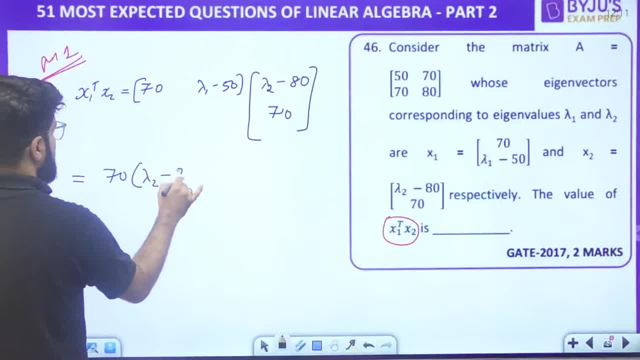 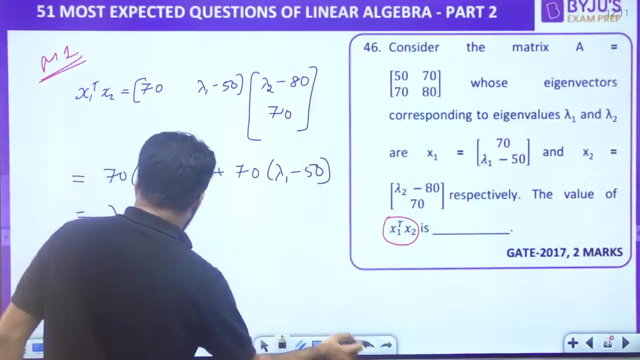 you take its dot product, I get 70 lambda 2 minus 80 plus 70 lambda 1 minus 50. right now you may think that I have to first find lambda 1, lambda 2. no, not required, actually not required, okay, they go. 70 can be taken common. then you have 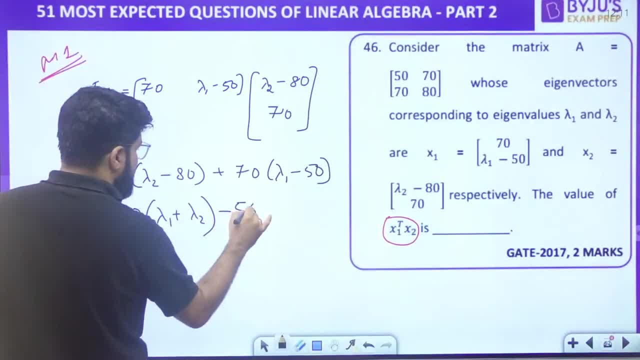 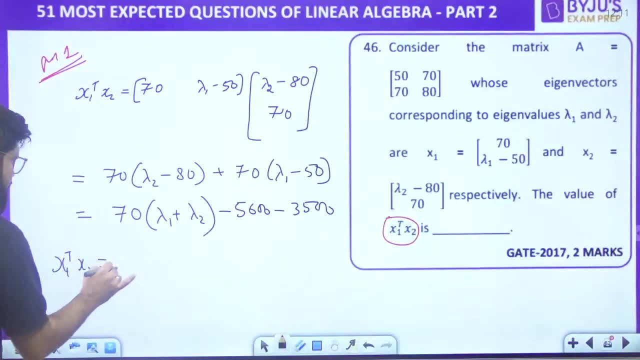 have lambda 1 plus lambda 2 minus 7, 8 the 56. so this is five, six double zero. seven F 35, this is three, five double zero. so what is the X 1 transpose X 2? it is equal to 70. lambda 1 plus lambda 2 is also equal to the trace of the matrix. 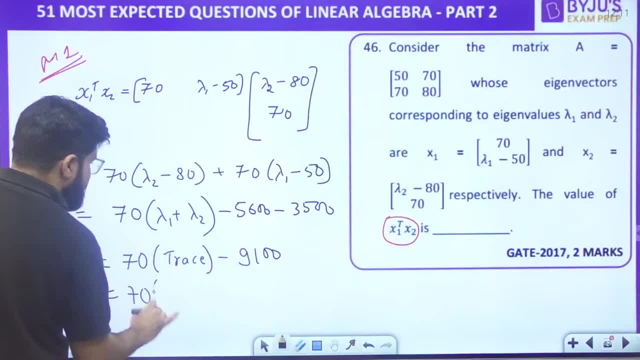 minus this is 9: 1 double zero. sir, what is the trace of the matrix? fifty plus eighty, one thirty, okay, one, thirteen, two, seventy, again nine. one double zero minus 9. one double zero. answer is T and 1 minus 7 lego zero. this is higher than that: 9: 1 double zero. this is: 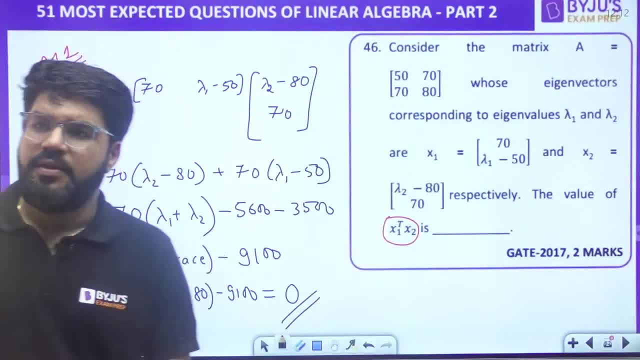 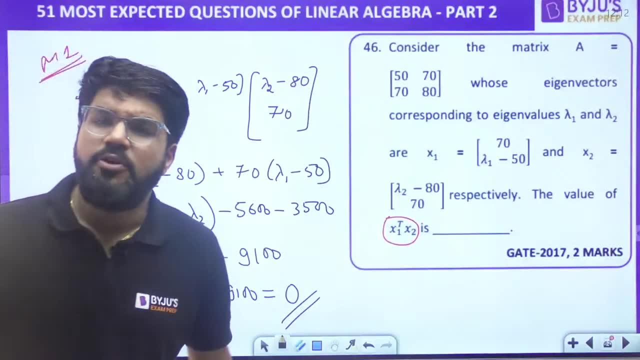 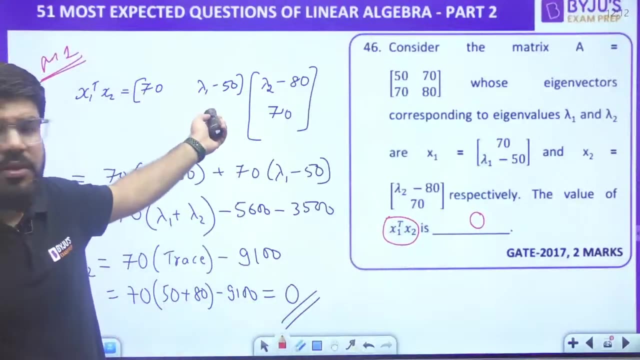 should be 0. answer should be 0. yes, Ashok, correct, correct, Swabhagya, right, right, you don't have to find lambda, you will be just wasting the time. you will be just wasting the time. the answer is 0. now the method number 2. that is related to the previous question. that is related to the previous. 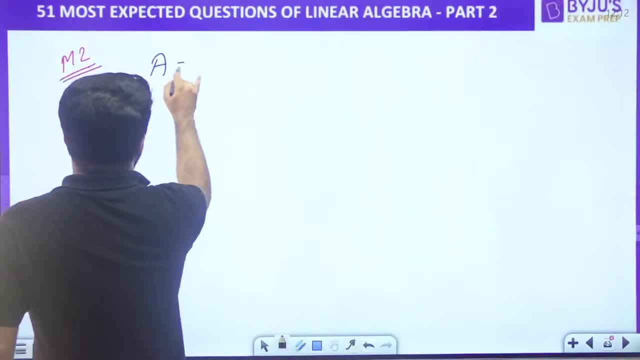 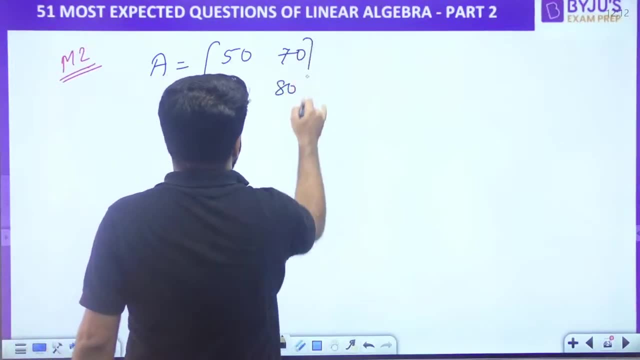 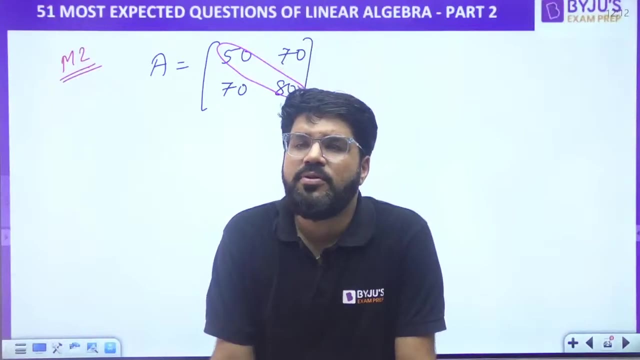 question: if I write down the matrix a once again, what is the matrix? 50, 70, 70, 80? have a look into this matrix again. the elements above and below the diagonal, the elements above and below the diagonal are same. that means it is a symmetric. and what symmetric real? all elements are real. 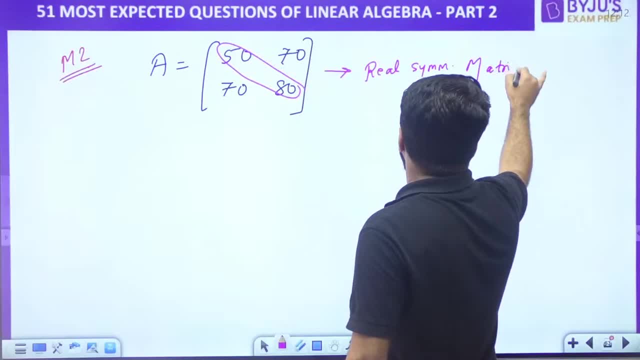 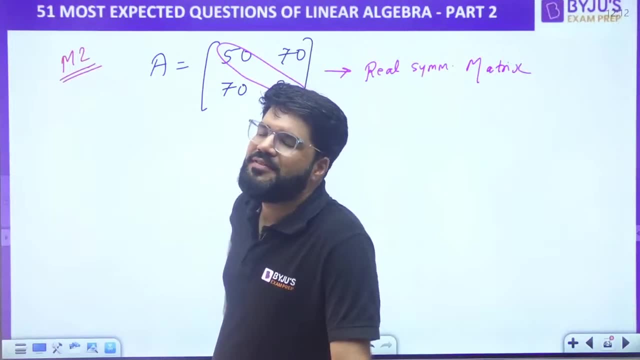 so it is definitely a real symmetric matrix. okay, eigenvector should be orthogonal. nah, not always eigenvalues. eigenvectors are not always orthogonal. they are orthogonal if eigenvalues are distinct. you have to rectify that, otherwise you may commit the mistake. eigenvectors are orthogonal if eigenvalues are distinct. if eigenvalues are. 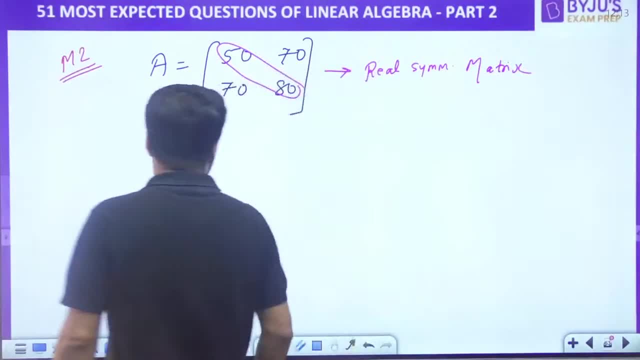 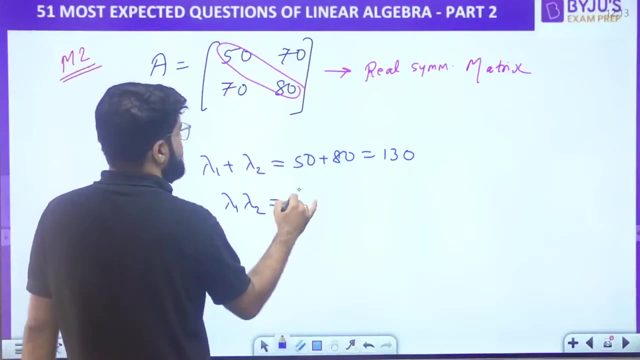 distinct eigenvalues are distinct right. so what about the eigenvalues? lambda 1 plus lambda 2 is 50 plus 80.. that is 130.. the product of eigenvalue is equal to determinant. that is, 50 into 84, 000 minus 70 into 70. 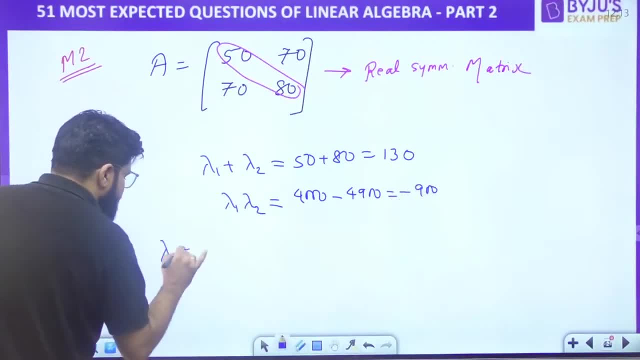 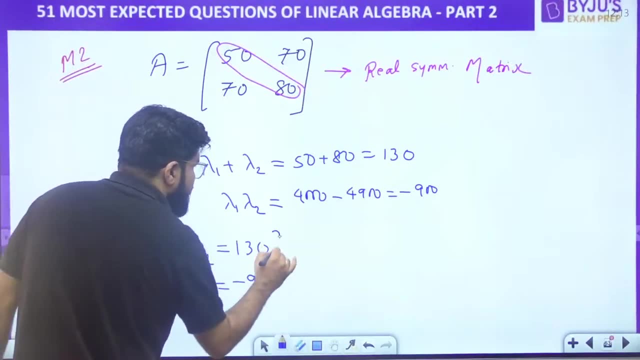 4900. this is minus 900, right? so if I take here lambda 1 plus lambda 2 is 130. lambda 1, lambda 2 is minus 900. no need to solve. but can you guess lambda 1, lambda 2? the nature of that, don't have to solve. 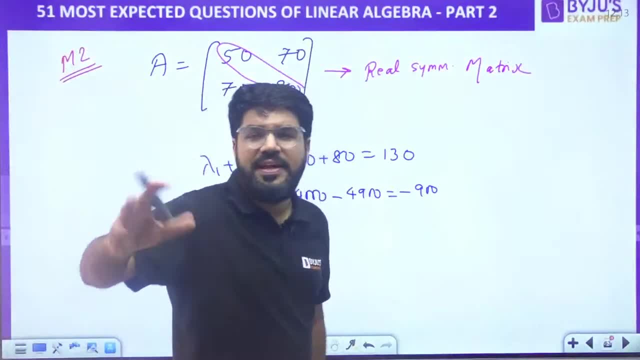 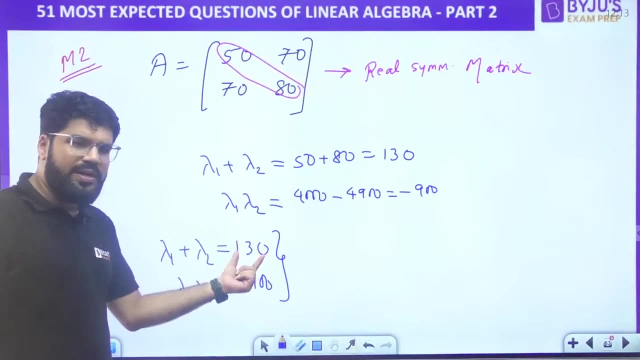 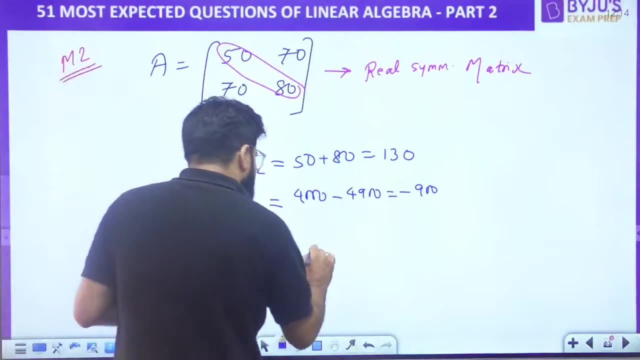 it up. but suppose they are equal. I want to check now whether they are distinct or whether they are equal. suppose equal, so suppose if they are equal. suppose lambda 1, lambda 2 equal. so 130 equally divided over 65. so 65 into 65 is not minus 900. so they are not equal. okay, I am clearly getting. 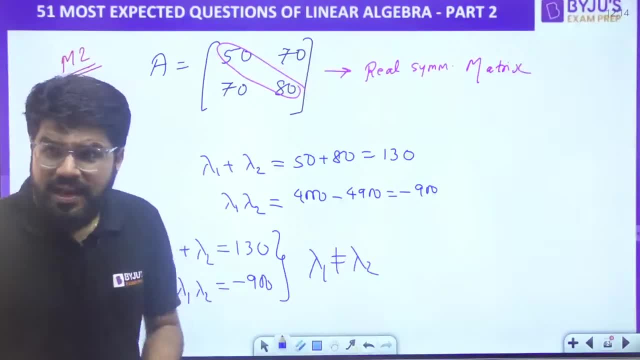 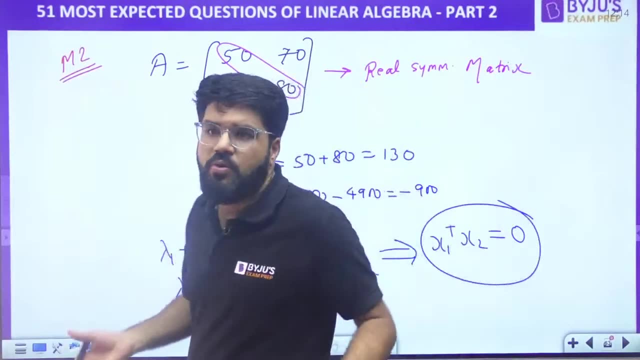 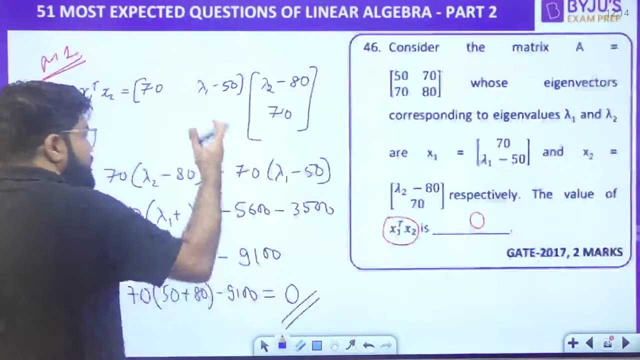 an idea that they are not equal and for distinct eigenvalues. eigenvectors are orthogonal. orthogonal means dot product is zero. what is orthogonal vectors whose dot product is zero, so by this property also is zero, and even by the simplest property of trace and all the eigen value, the answer: 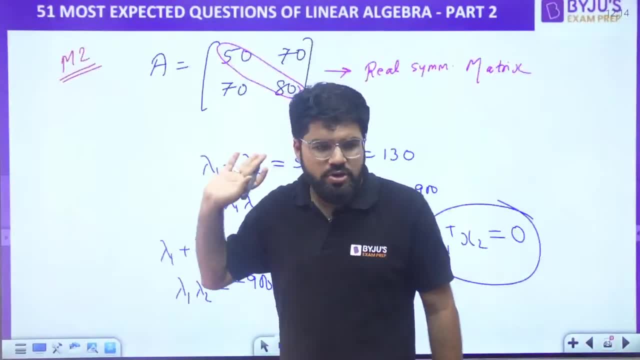 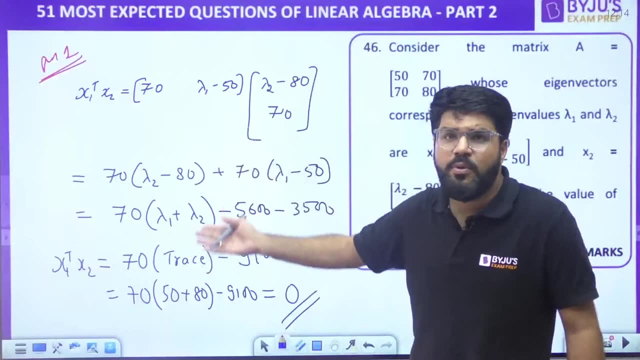 was zero, no need to specially think about symmetric matrix also. ok, that is also a correct approach, but I have solved this by the very basic approach also: x1 transpose x2. how much time did it take? because this does not require any thinking. this is direct method, because 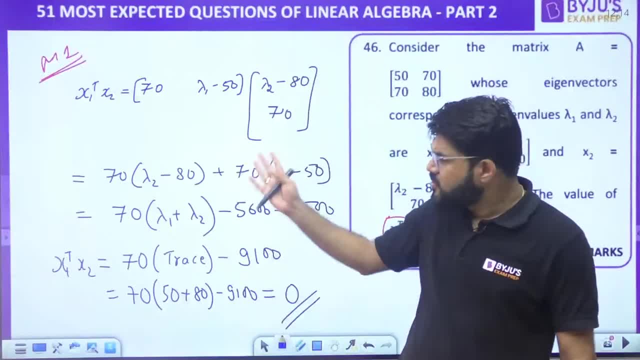 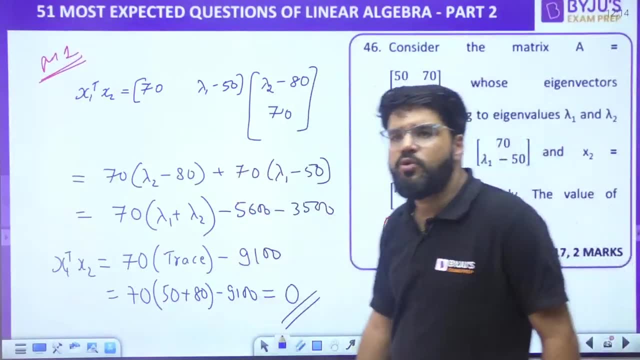 many of you are very practice with the trace and determinant property at least, so this is also very simple and comfortable method. this is a good method. this is a good method. here is the concept. this is simple method. I have told you both. I have told you both. 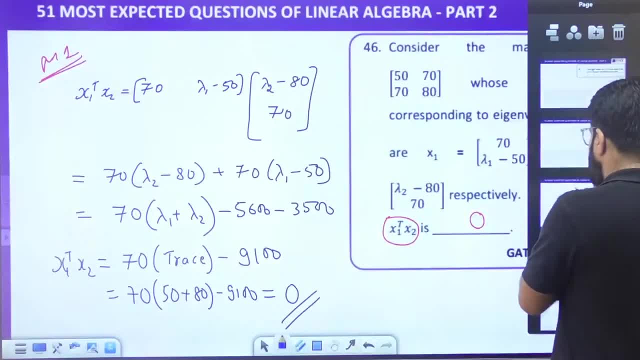 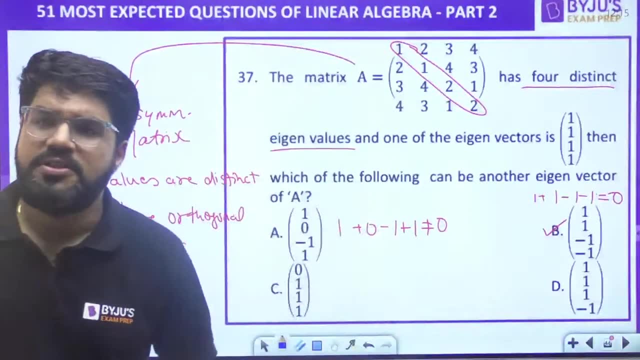 right. so I specially wanted to discuss this gate question. let us come back to our discussions. yeah, ok, and again on the same fundamental eigen values are distinct of a real symmetric matrix. we have solved this. one question also. 37, 38 was homework for you. let us move ahead. 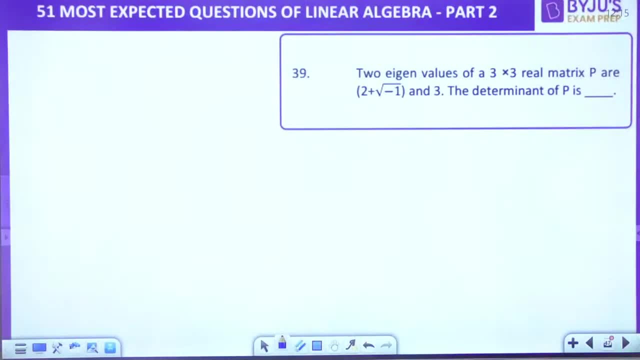 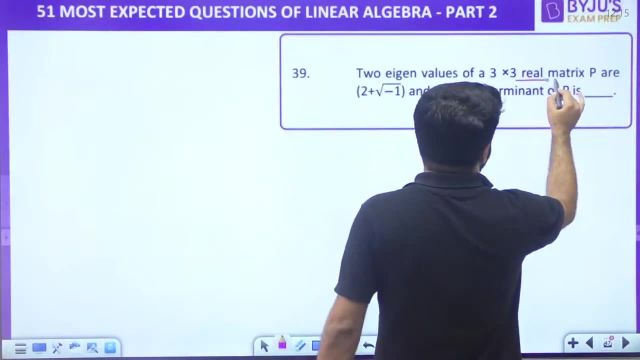 to the next 39. the two eigen values of a 3 cross 3 matrix are 2 plus minus 1 under root, minus 1 and 3. what is the determinant of 3? see very simple again: property real matrix. the eigen values of a real matrix are 2 plus under root of minus 1 and under. 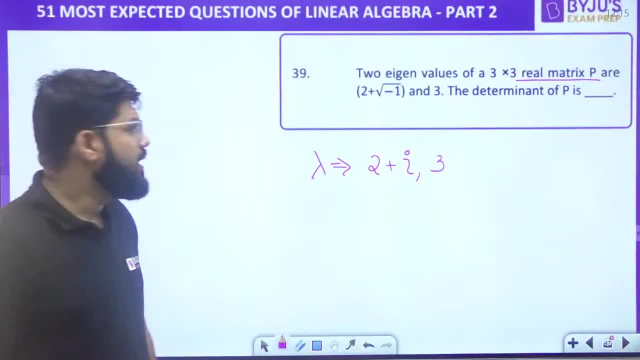 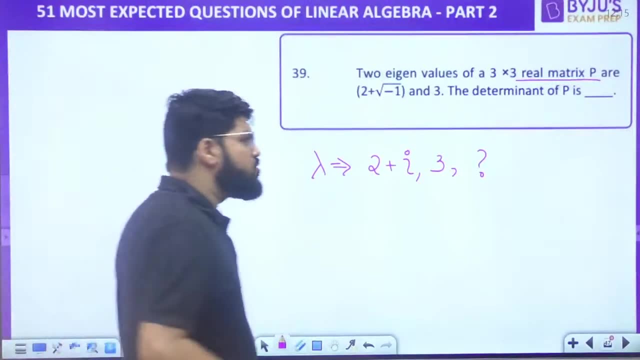 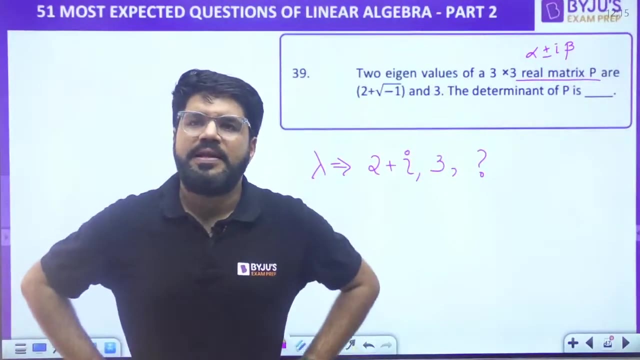 root of minus 1 is iota, imaginary number i, and then 3 and then question mark. so what should be this question mark for a real matrix? what is the important property that should click in the mind? alpha plus minus i beta property. alpha plus minus i- beta property. 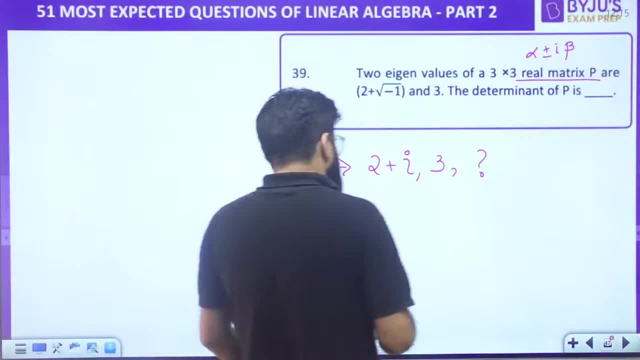 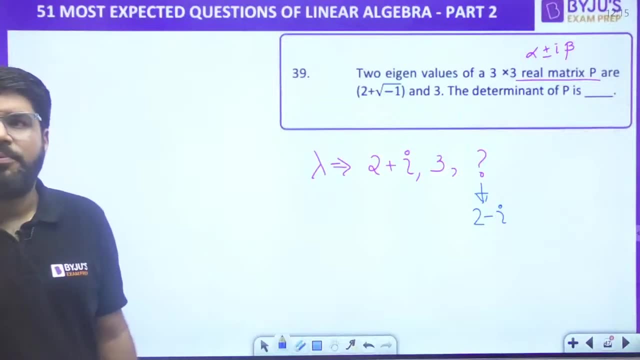 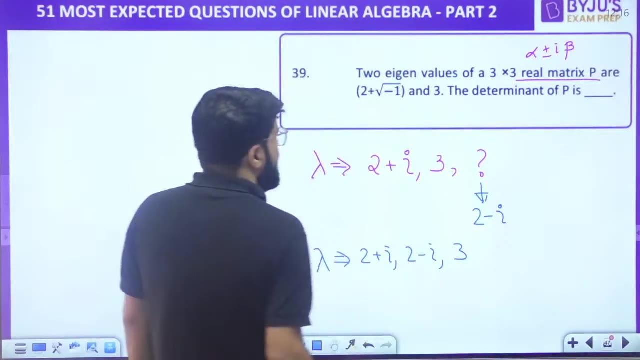 if there is a complex eigen value, it should be in the conjugate pair. it should be in the conjugate pair. what should be this question mark? it should be 2 minus i- alpha plus minus i- beta property. right, so now i can say that my list is complete: 2 plus i, 2 minus i and 3. right. so now, what is the? 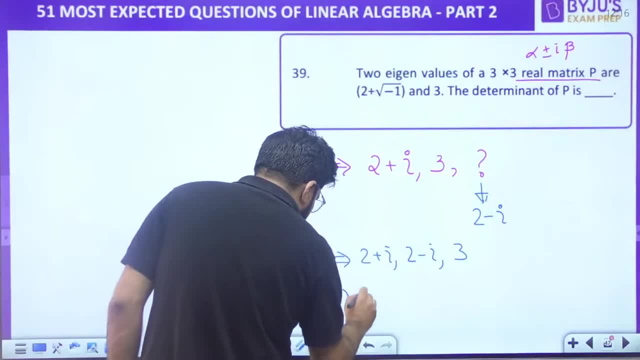 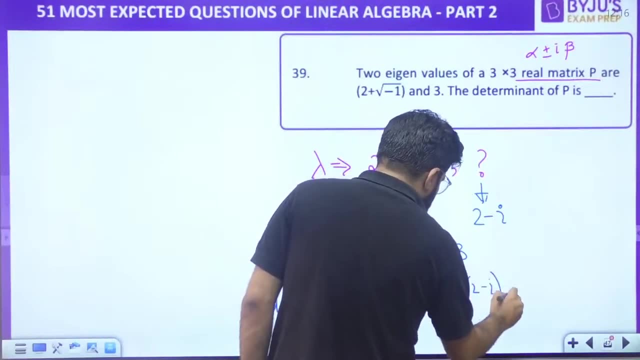 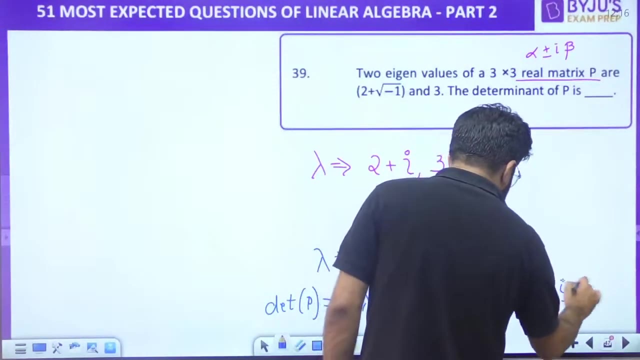 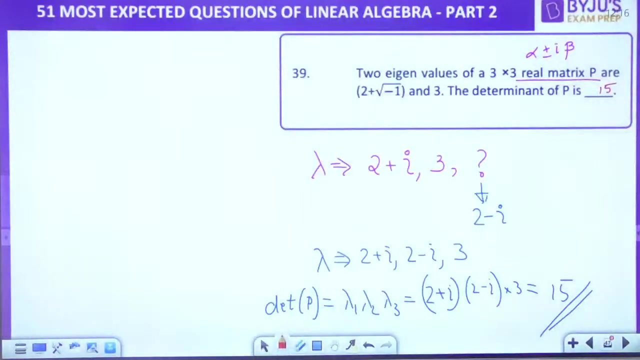 determinant of the matrix. p. determinant of matrix is product of eigenvalue. 2 plus i, 2 minus i into 3. this is 2 square plus 1 square 5 multiplied by 3. answer: please check it up. it should be 15. the answer for this nat type question is 15. so two simple properties here. 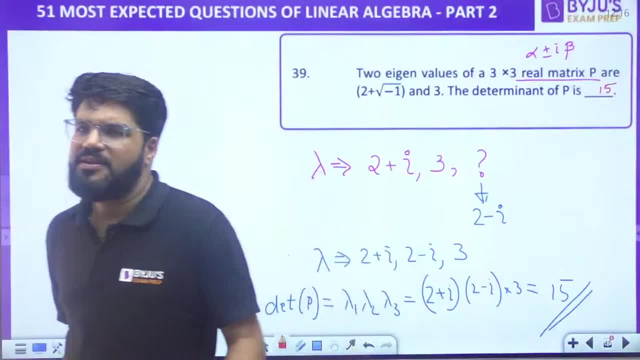 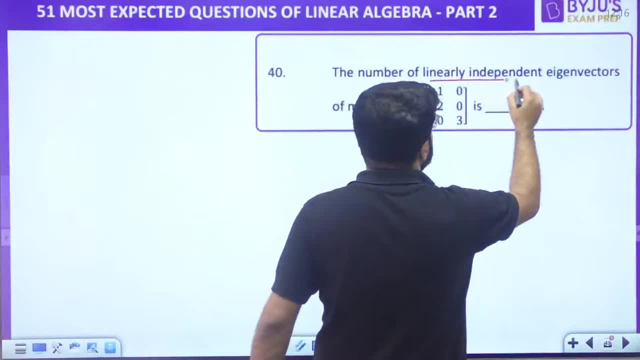 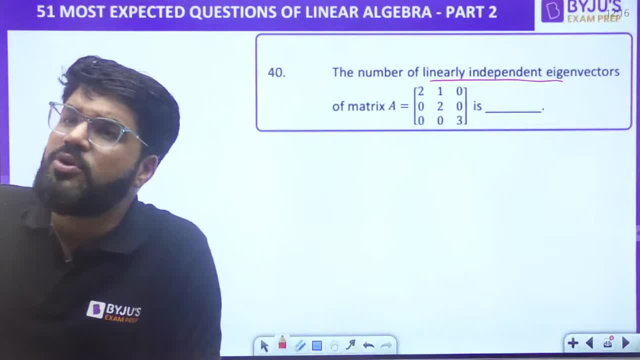 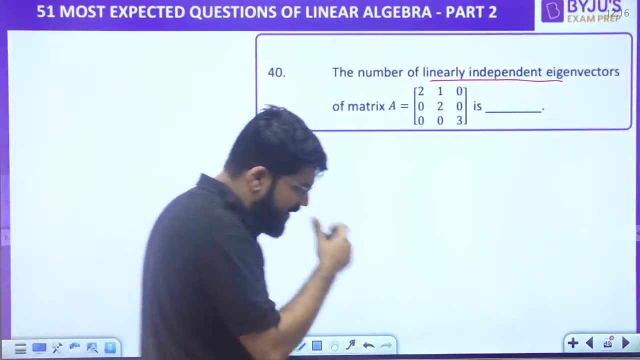 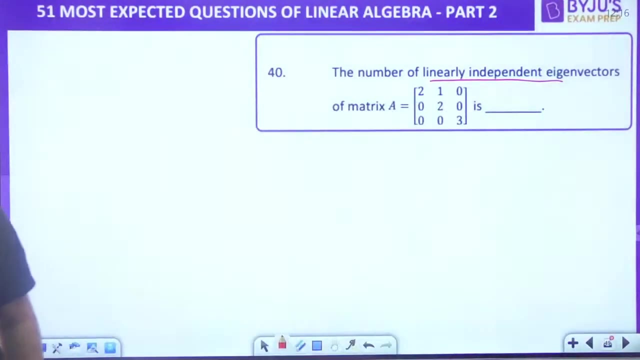 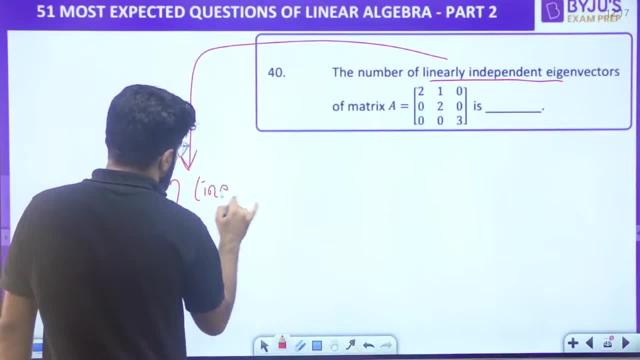 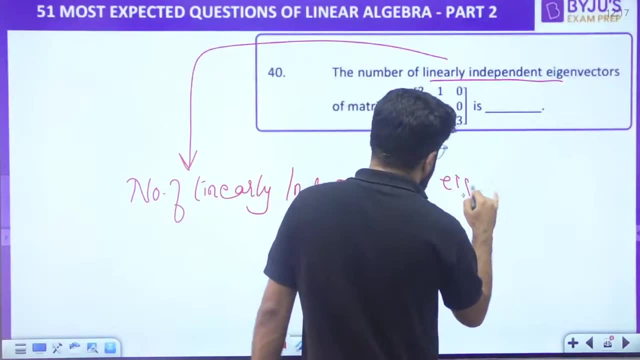 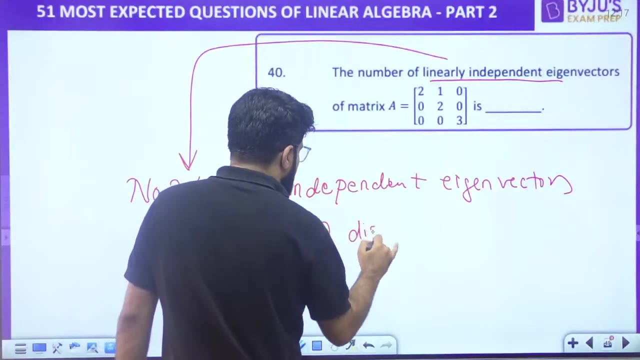 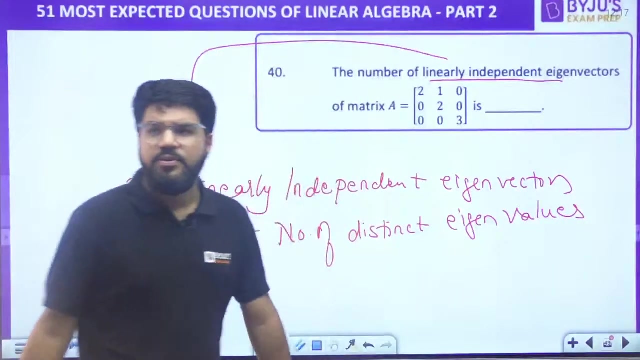 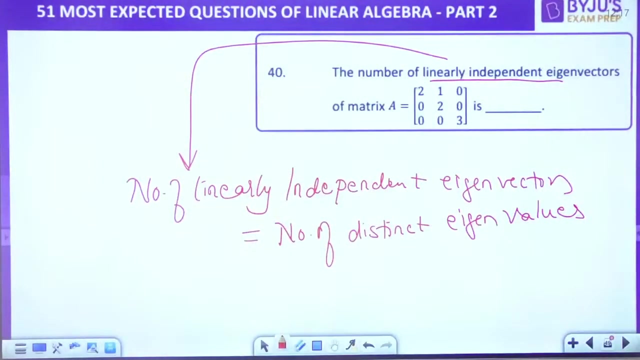 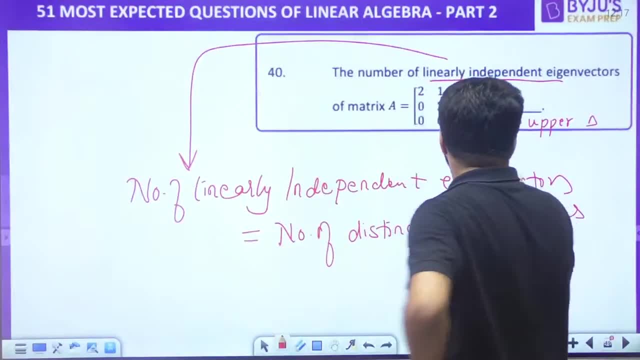 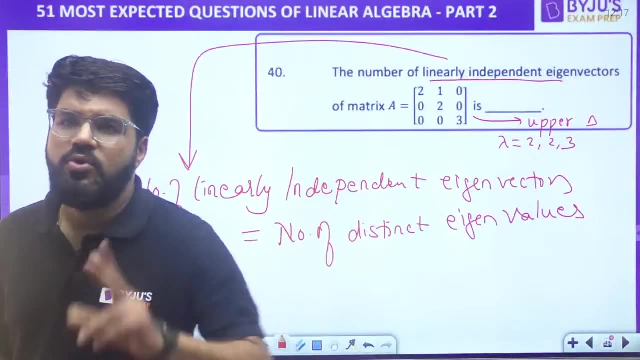 upper triangular. I don't have to put the effort for finding the eigen values. what are the eigen values? two, two, three. how many of them are distinct? how? how are How many of them are distinct? 2 and 2.. Repeat How many of them are distinct: 2 and 3.. 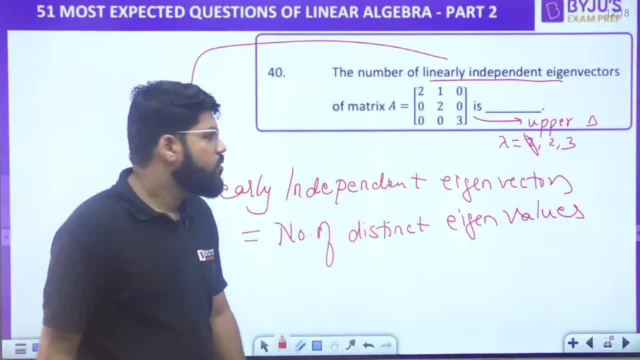 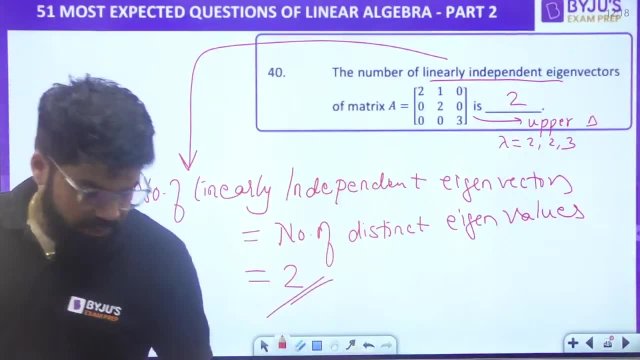 We will consider this as repeat. Remove this 2 and 3.. So how many of them are distinct? 2. Your answer is 2. The number of distinct eigenvalues, The total number of independent eigenvectors, is equal to the number of distinct eigenvalues. 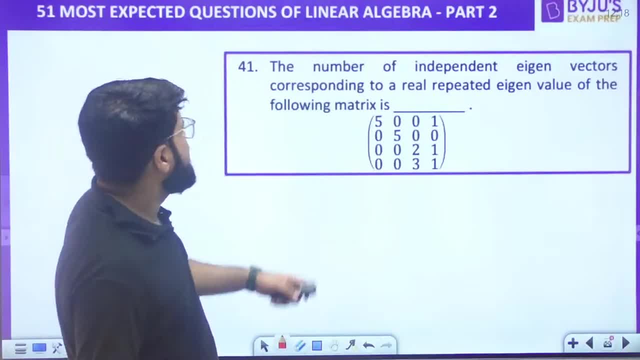 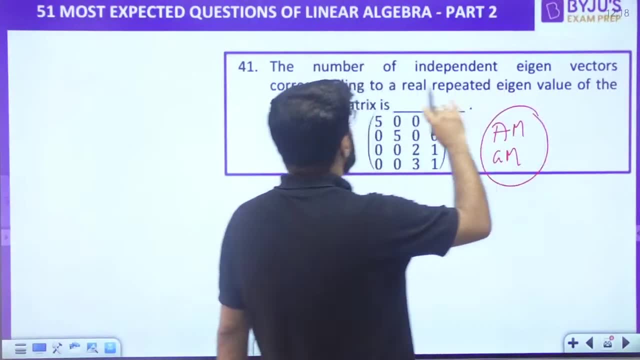 Number of distinct eigenvalues. Number of distinct eigenvalues: 41.. We will do this later, because here I need to explain you the concept of AM and GM. So this is a new concept. I will explain you. number of independent eigenvectors corresponding to a particular eigenvalue. 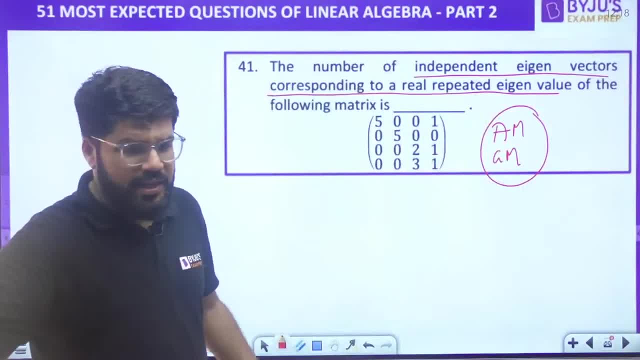 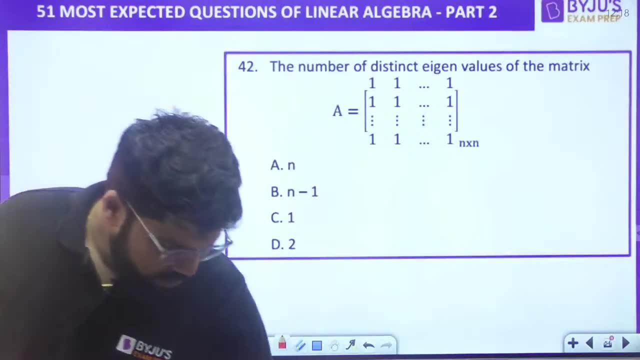 Corresponding to a particular eigenvalue. So I will come back to this. Any new explanation, I will come back to that. Let us solve other questions first. First, let us complete this First. let us complete the questions that you have been regularly seeing. 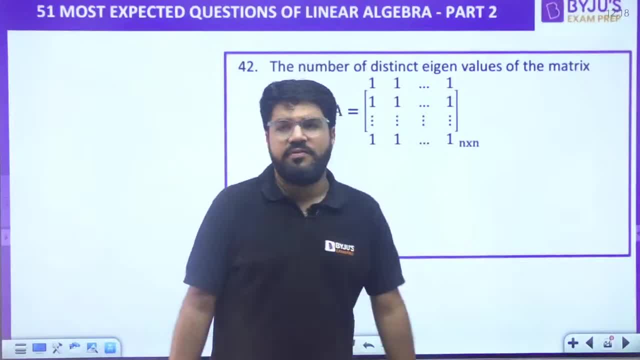 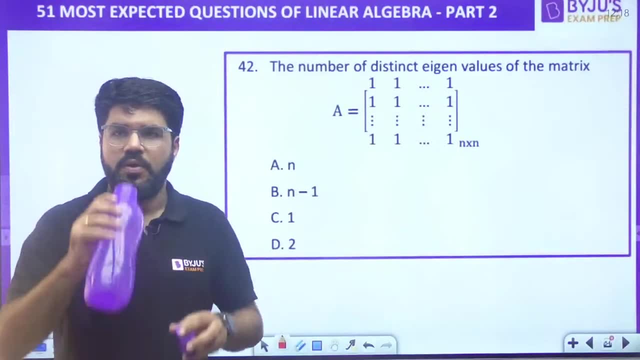 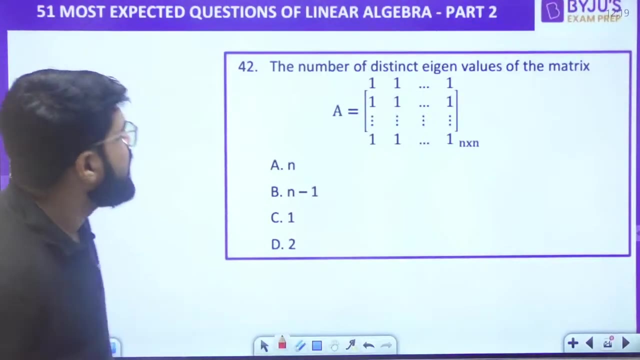 We will come back to that question. Number of distinct eigenvalues of the given matrix. Tell me this. This is again a good question. This is also a good question, dear Number of distinct eigenvalues of the matrix? Tell me, tell me, tell me. 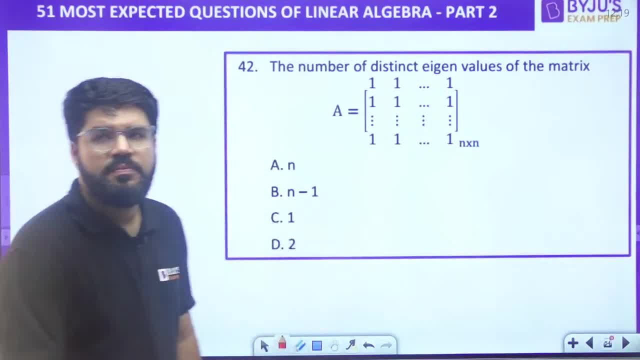 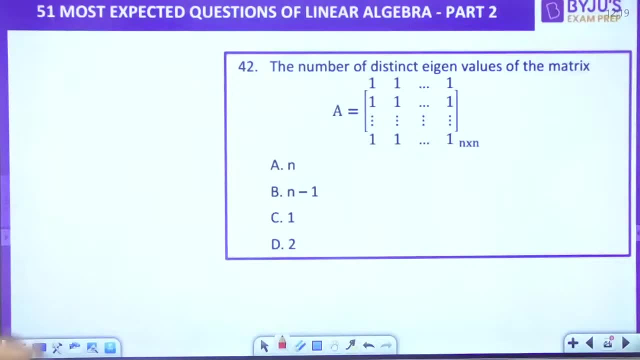 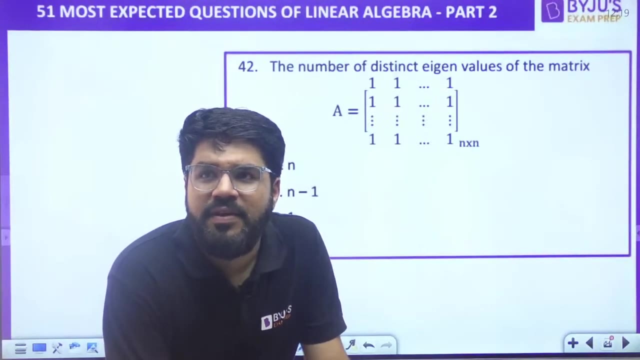 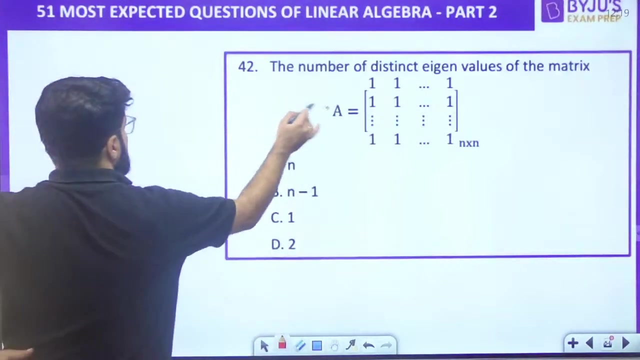 Number of distinct eigenvalues of the matrix. Think and let me know Number of distinct eigenvalues of this matrix. Look, it is a matrix in which all the rows are same, All rows are same, All rows are identical. So what should be the rank of this matrix? 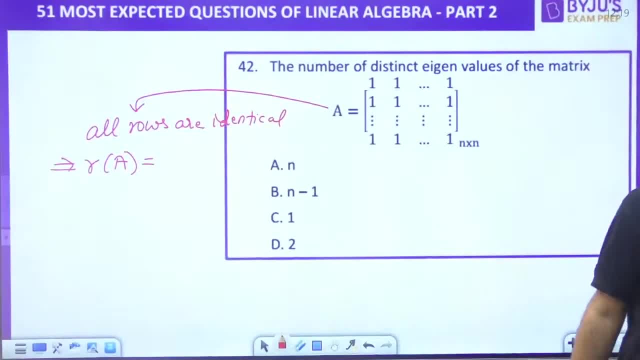 We have seen that yesterday. A matrix in which all the rows are same or identical, it has the rank equal to 1.. In which all the rows are same or identical, the rank is equal to 1.. The rank is equal to 1.. 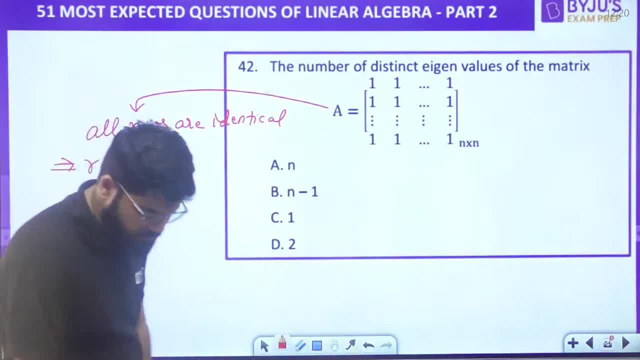 The rank is equal to 1.. Okay, The rank is equal to 1.. 1, 1.. Okay, Very good. Now what is one more property for rank? Today we have learned: rank is equal to number of non-zero eigenvalues. 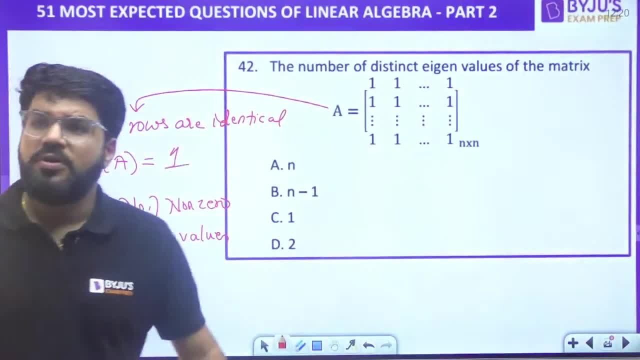 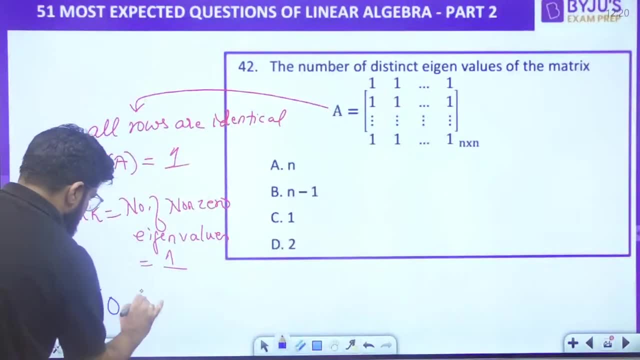 Right, And that is equal to 1.. Rank is number of non-zero eigenvalues. So there should be only one non-zero eigenvalues, Right? So what are the eigenvalues? So what are the eigenvalues? Only one, non-zero. 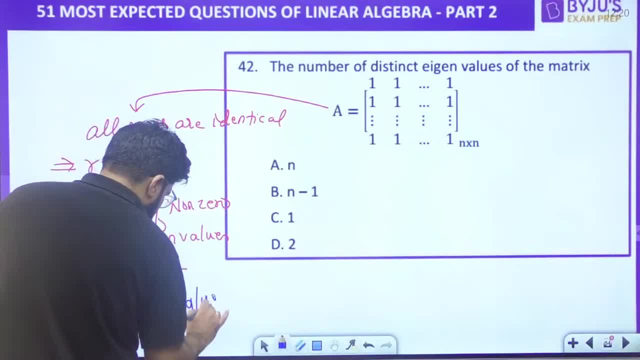 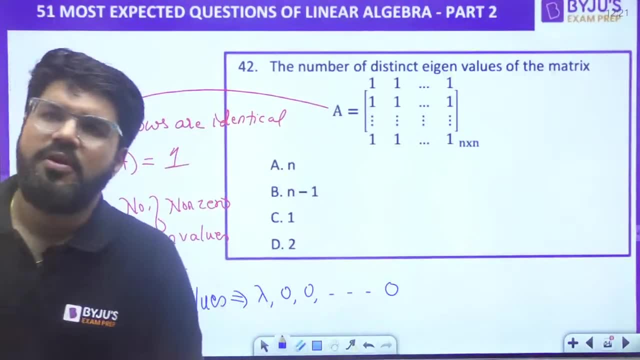 So what are the eigenvalues? Only one non-zero rest, all will be zeros. Rest all will be zeros. Only one non-zero rest, all will be zeros. Zero, zero, zero, zero, zero And only one non-zero. that is lambda. 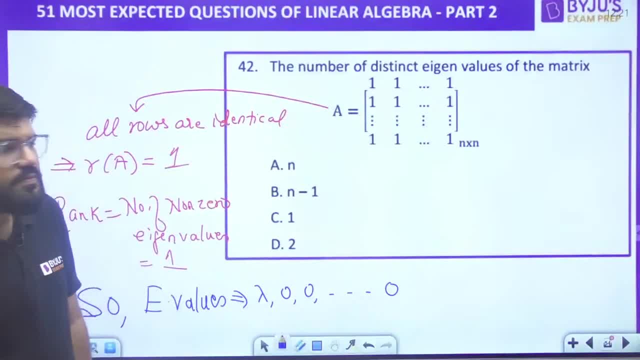 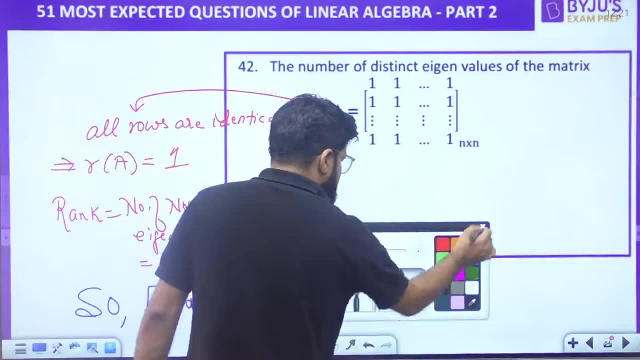 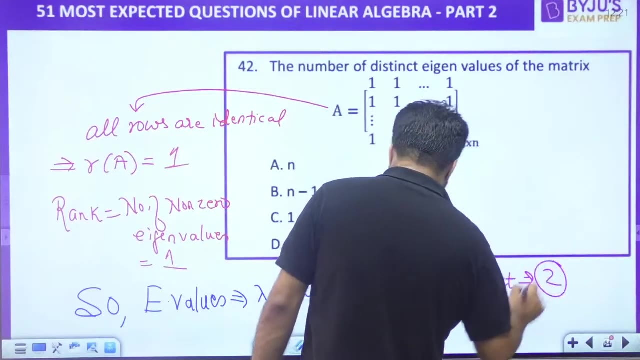 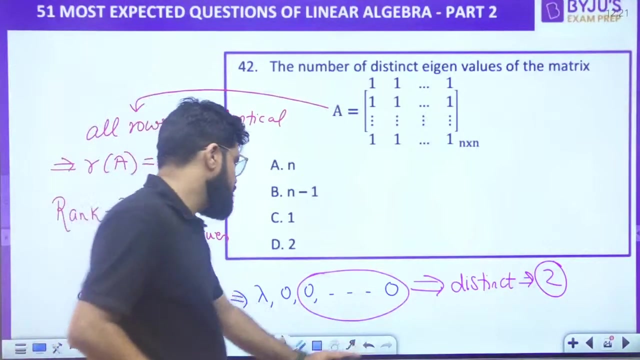 That is lambda, Correct. So how many distinct eigenvalues it has? How many distinct eigenvalues it has? One is lambda, One is zero. All this is repeated. Only two distinct eigenvalues: One is lambda, One is zero. Answer is two. 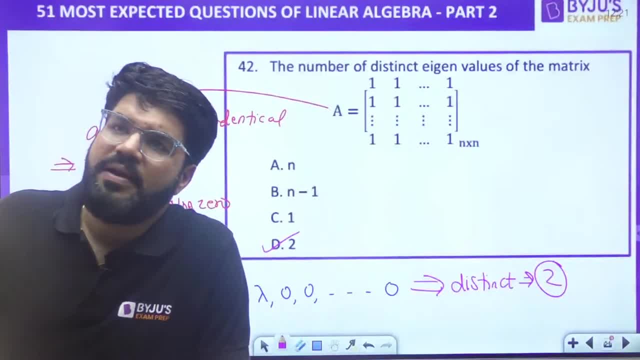 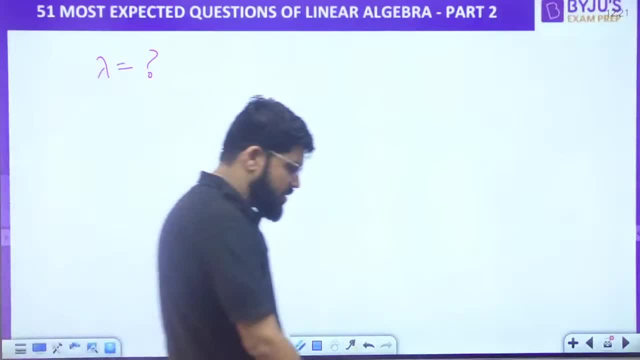 Answer is option number D. Whatever may be the size of the matrix, Whatever may be the value of n, Only two distinct eigenvalues. Okay, Now let me put up a question here: Can you find out all the eigenvalues? Can you find out all the eigenvalues? 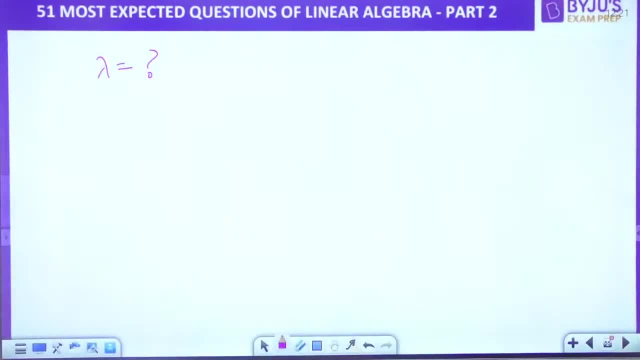 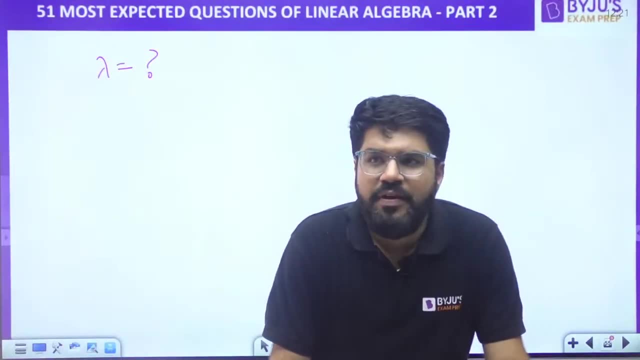 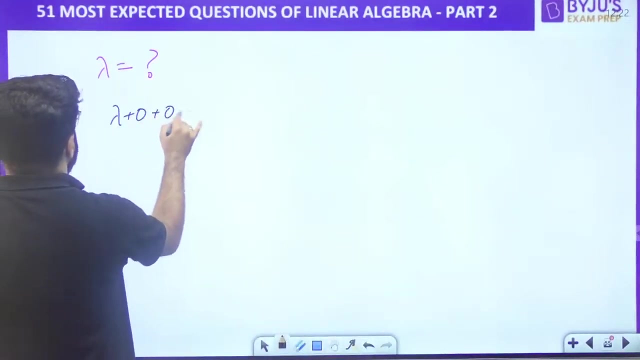 Can you find out all the lambdas? can you find out all the lambdas? can you find out all the lambdas? how to find out the eigen value by the trace property. lambda plus 0 plus 0 plus 0. sum of eigen values should be equal to. 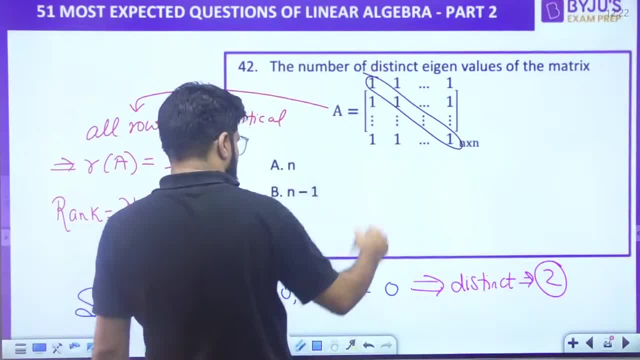 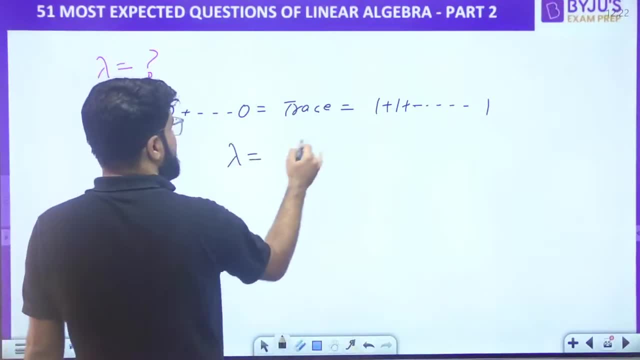 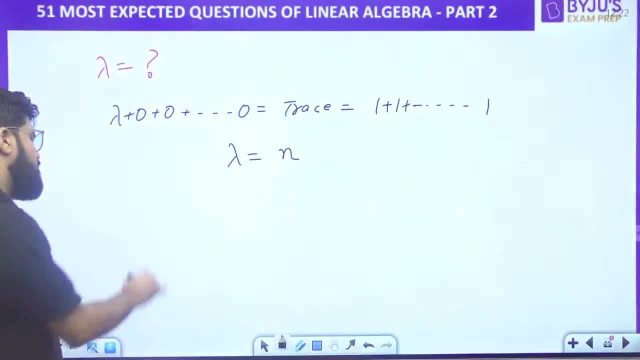 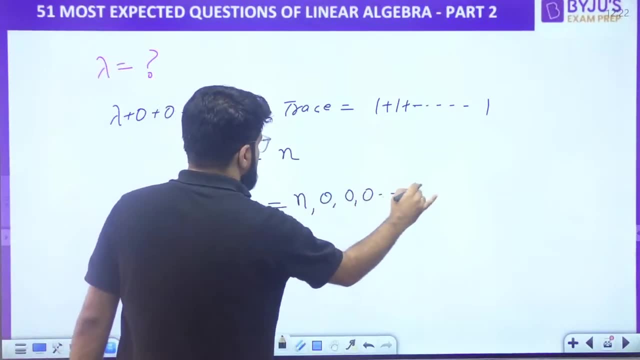 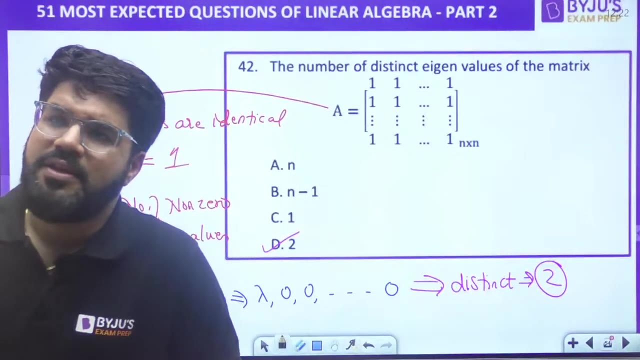 so lambda is equal to n, right? so what is the final set of eigen values? it is n 0 0 0. this is a good question. a matrix in which all entries are 1, the eigen values will be n 0 0 0 0. 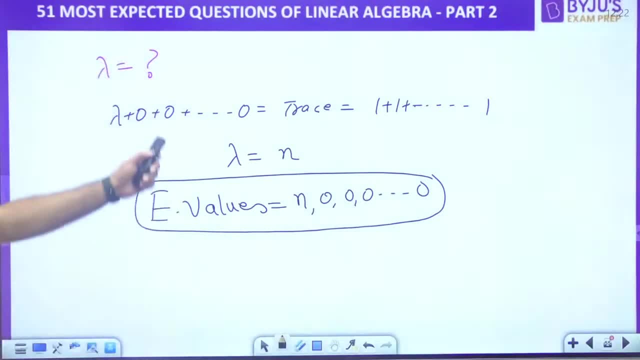 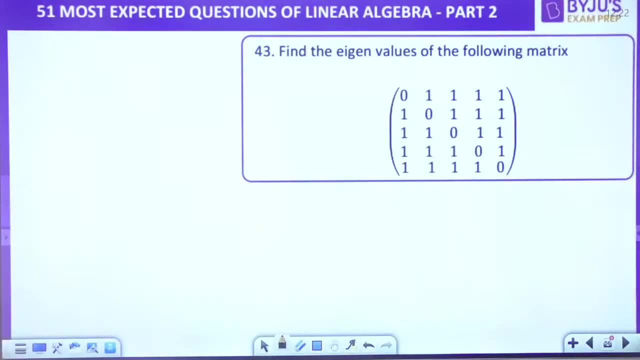 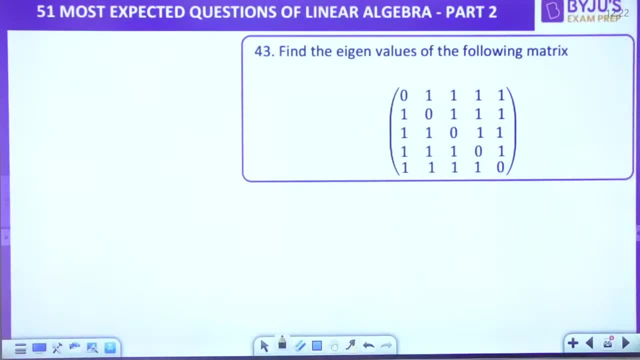 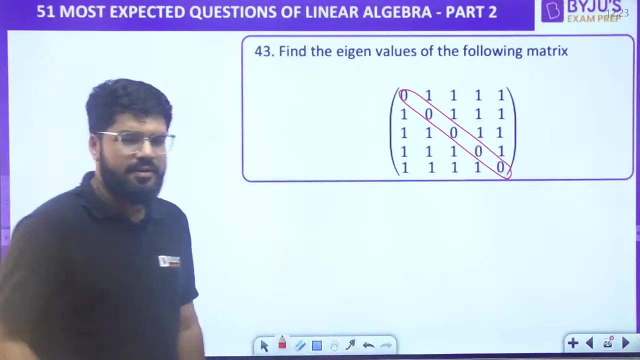 find the eigen values of the following matrix. now see, this is a matrix in which most of the entries are 1, except the diagonal. most of the entries are 1, but it is except the diagonal. what to do if you make the diagonal as n, 0, 0, 0, 0, 1, n. 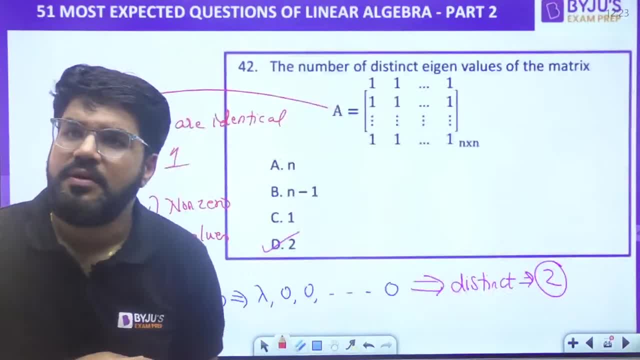 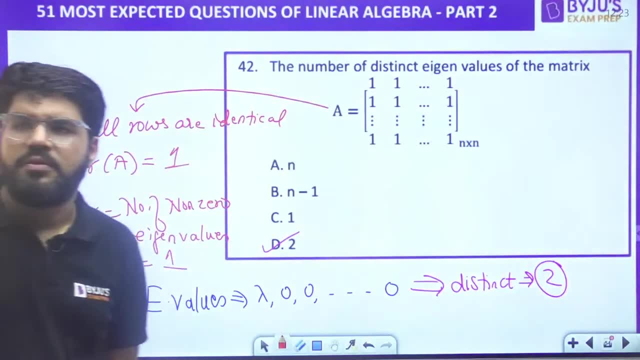 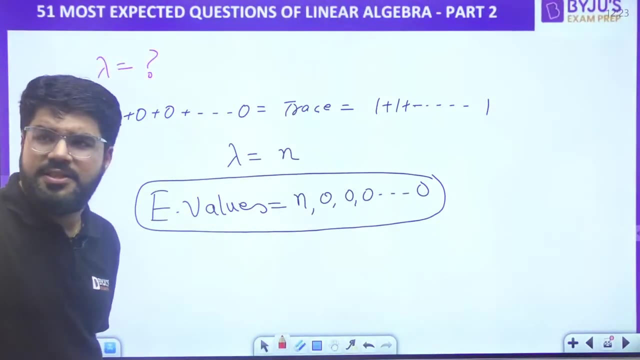 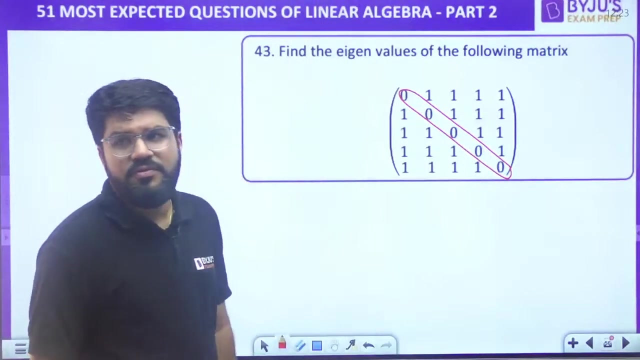 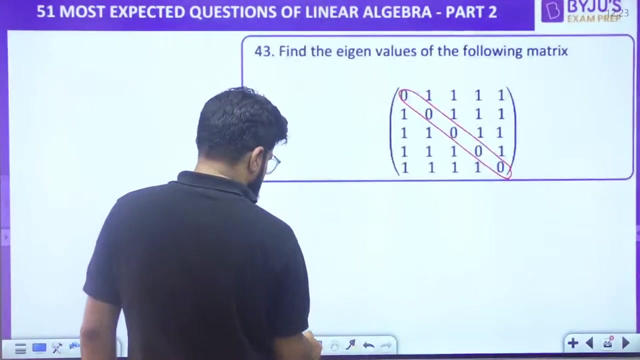 signal elements also one. then it becomes the previous type of question. then it becomes the previous type of question. right, right, correct, yeah, some of all entries is same. that is also okay for the previous question. so tell me, find the eigen values of the following matrix what it should be. so if all of these are one, now how to make it as one? okay, okay. 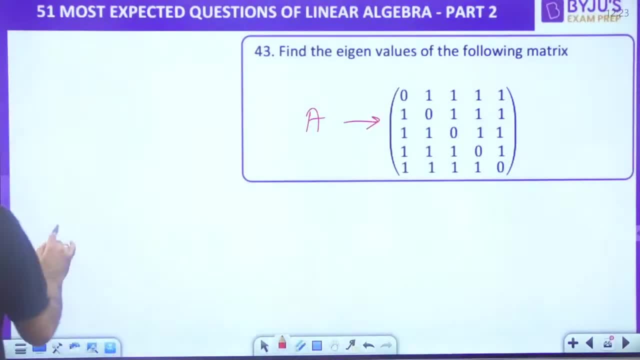 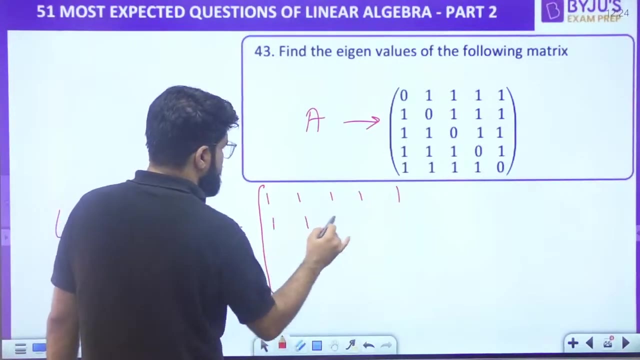 let's say this is some matrix. a guys, let b is equal to a plus i. to make the diagonal elements into one, to convert the diagonal elements into one, you should add the identity matrix. and as soon as you add the identity matrix you get all ones, okay. 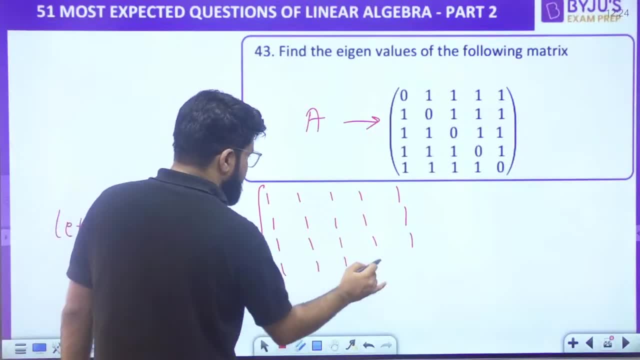 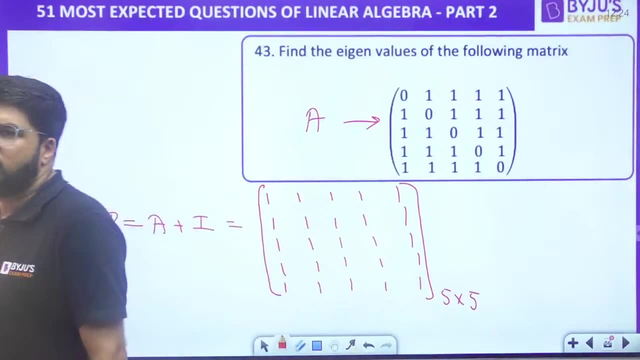 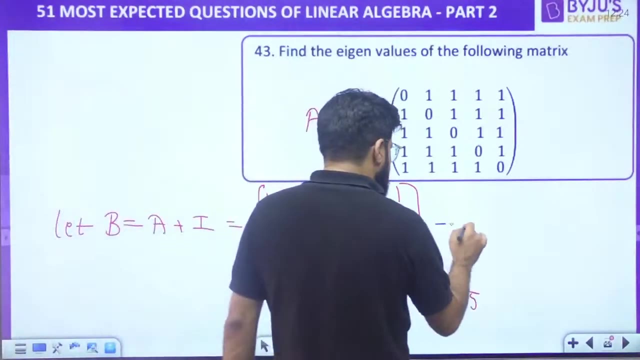 okay, okay, okay, what is the size? five cross five. actually, what is the size five cross five size is given to? you guess i is given a five cross five. okay, now we know the eigen values of this matrix. what are the eigen values of this matrix? a matrix whose all elements are one. the eigen values. 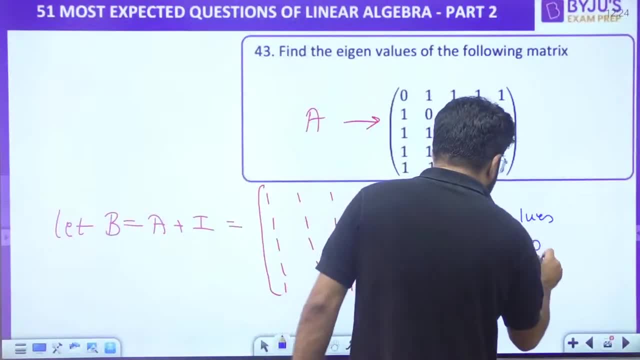 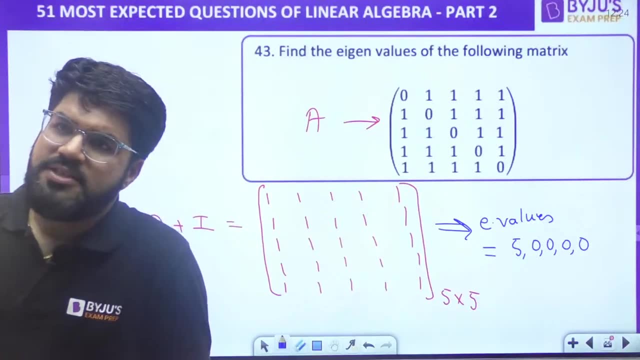 are given by n: zero, zero, zero, zero. what is the n? five, five and all rest four will be zero. total five eigen values: first is one and all rest five remaining is zero. okay, that is five, zero, zero, zero, zero. that is eigen value of b. now, what is the a? it is: 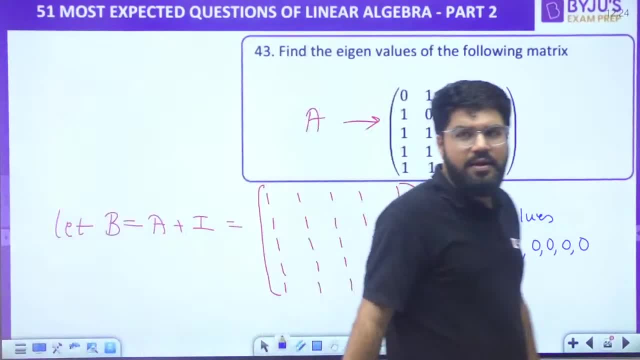 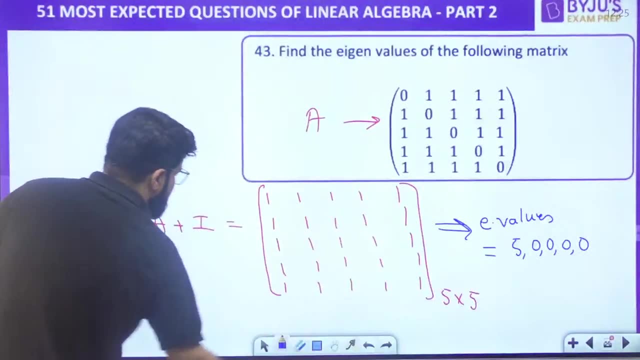 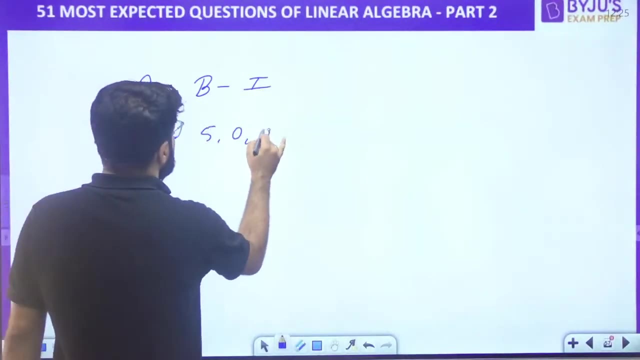 b minus i. i want the eigen value of a. i have nothing to do with b. i have nothing to do with b. so what is a then? what is a from here? it is b minus i, right, so if the eigen values of b are known to you, what are the eigen values of b? it is five zero, zero, zero, zero. what are? 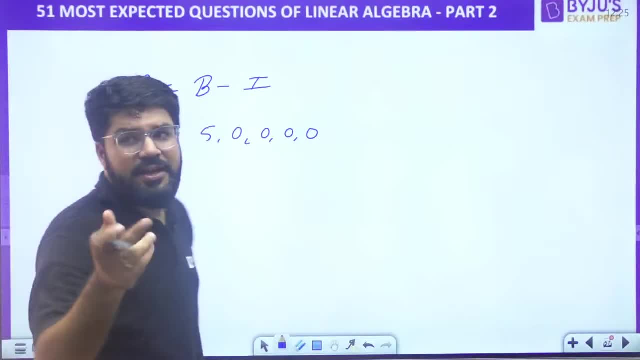 the eigen values of a then minus i matrix is known to you. what are the eigen values of b? it is five, zero, zero, zero, zero. what are the eigen values of a then minus i matrix, minus i, so eigen value minus one eigen value minus one, five minus one, zero, minus one zero. 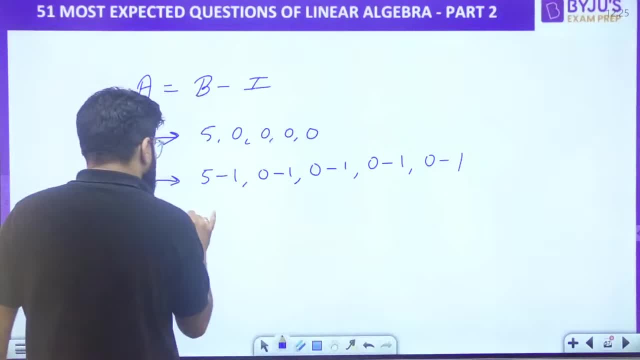 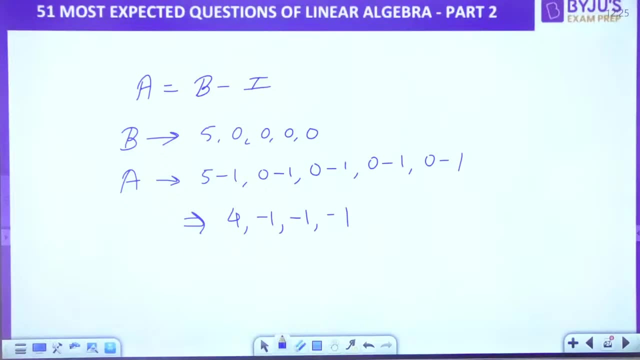 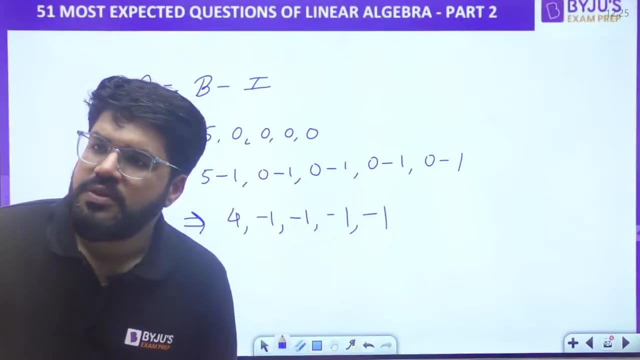 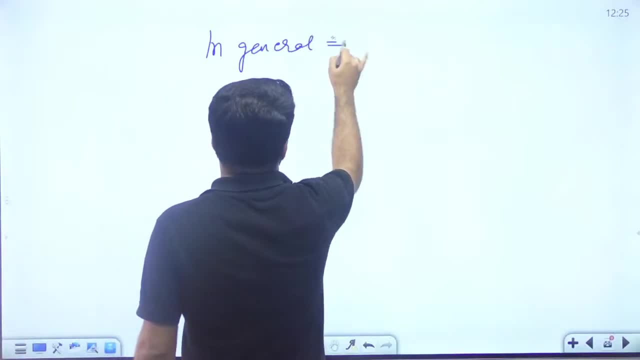 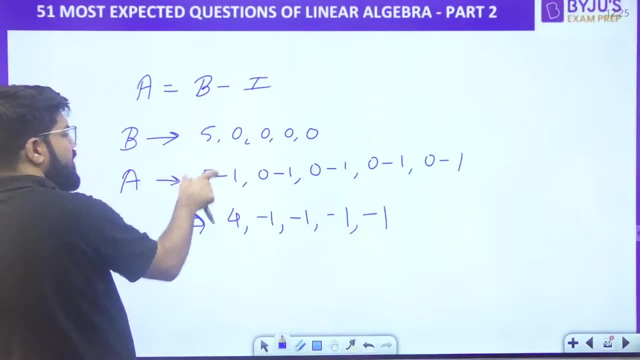 here it was 5, 5 because the size was 5, otherwise the value will be n and 0, 0, 0, 0, then subtract i the subtract 1, so in general it will be n minus 1, and then minus 1 minus 1 minus 1, up to remaining. 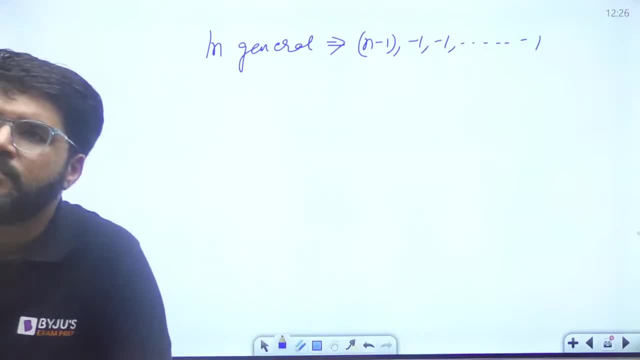 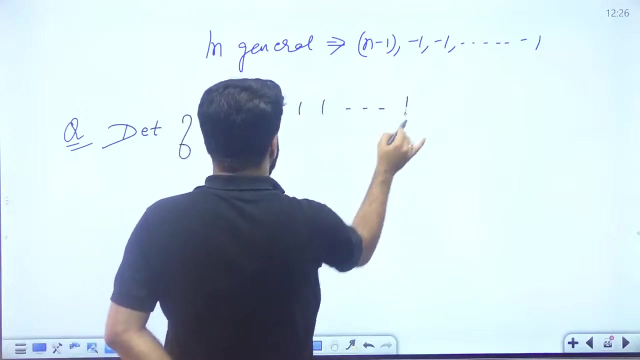 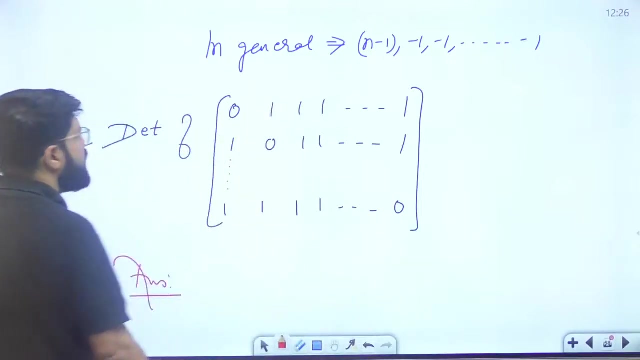 times. so i ask you a question now. i ask you a question now. question can be like this also: find the determinant of right, find the determinant of this matrix. this becomes a good determinant question: find the determinant right. so what should be the answer then? what should be the answer? determinant is product of eigenvalues. 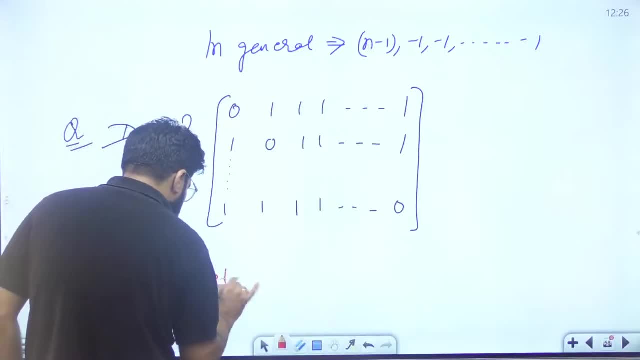 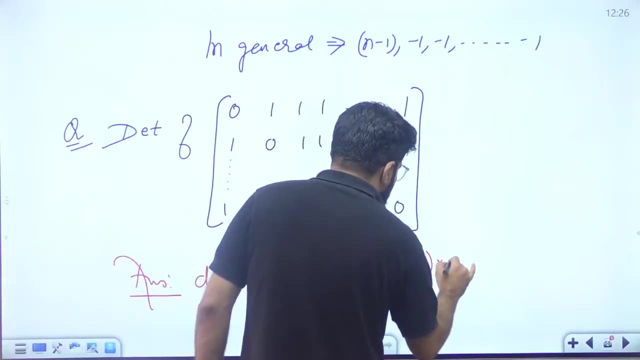 determinant is product of eigenvalues and that will become n minus 1 multiplied by minus 1. multiplied by minus 1. how many times minus 1 is multiplied n minus 1? so it is given by the formula minus 1 k power, n minus 1. 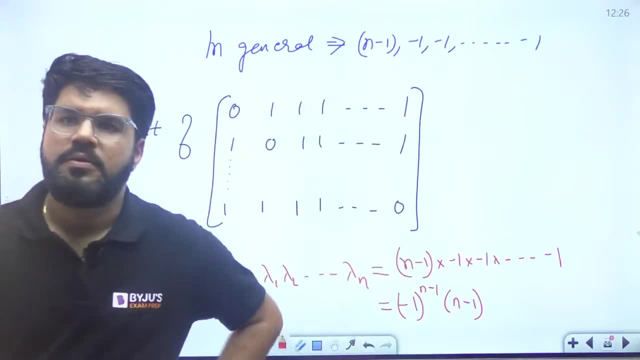 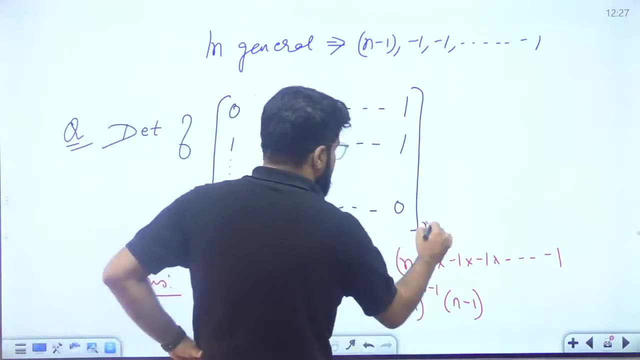 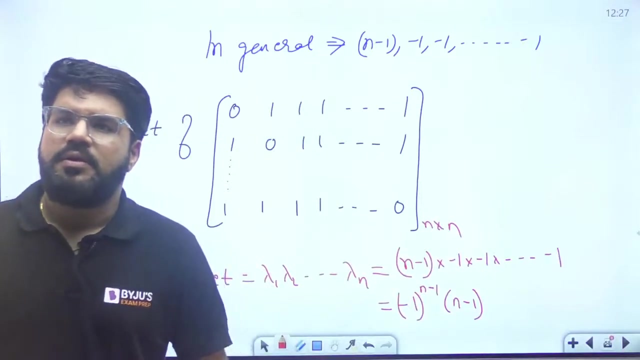 whole multiplied by n minus 1 minus 1. k power n minus 1 whole multiplied by n minus 1. that is the formula if it is a n cross n matrix. if it is a n cross n square matrix with all diagonals number 0. remaining elements: 1. Determinant directly: nikalenge. it may be little. 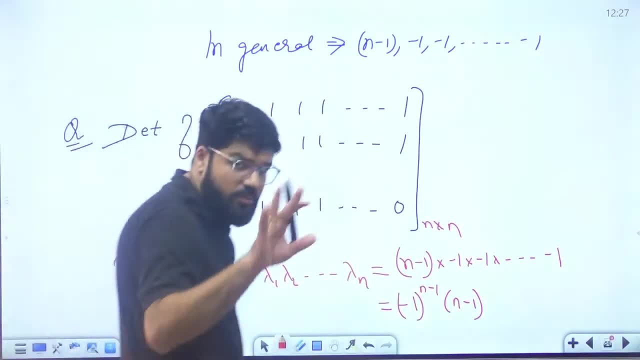 lengthy, but by the eigen value it is a very simple process. I have related this to a determinant type of question also, But by the approach of eigen values, But by the approach of eigen values Got this Chalo. These are good questions, Thik hai. These are good questions, Thoda. 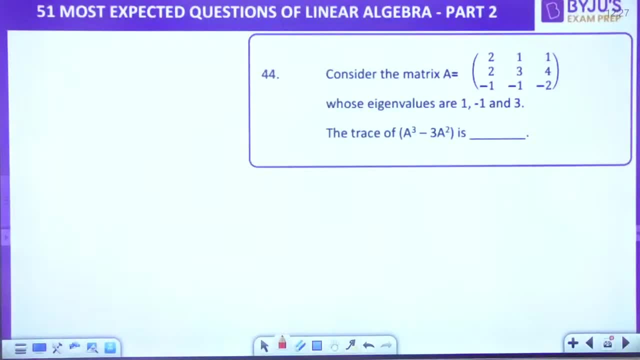 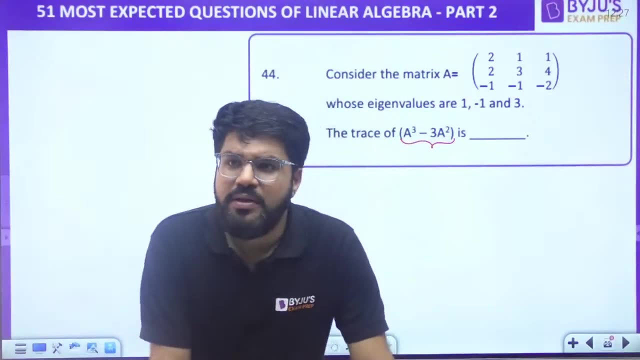 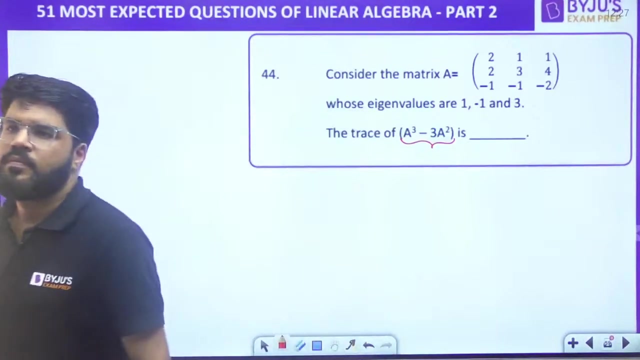 se unique wala hai. Next, Consider the matrix, whose eigen values are given to you. What is the trace of a cube minus 3a square? Now, does it mean that first you have to calculate a cube and a square? Does it mean that you have to calculate a cube and a square? Does 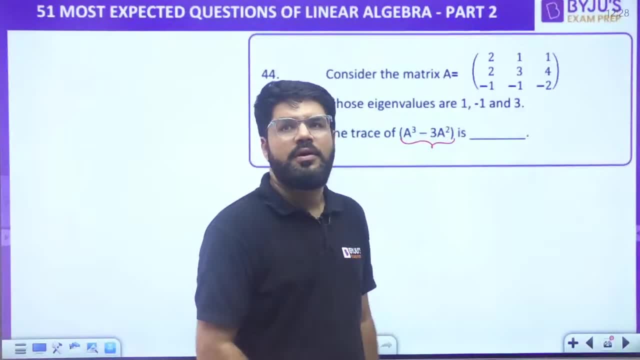 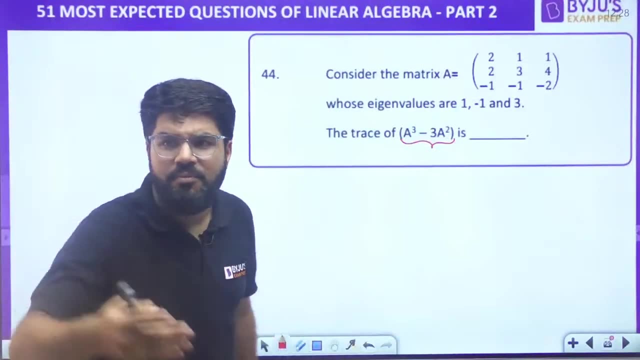 it mean that I have to calculate a cube and a square? Not at all. Trace is some of the eigenvalues. can I find the eigenvalues of this directly again by the property algebra, a power and property right. the eigenvalues of a are the eigenvalues of. 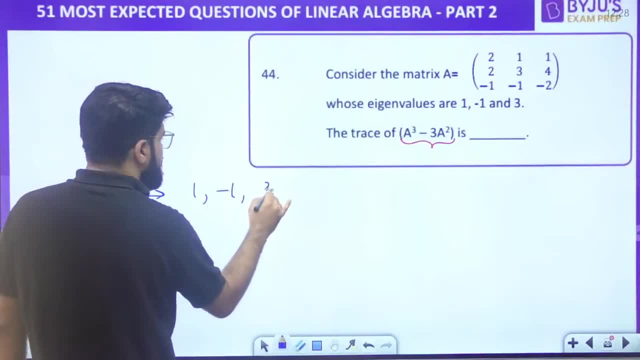 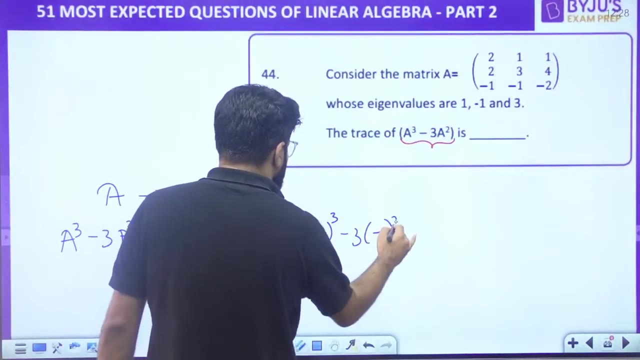 a are that to. it is given to you 1 minus 1, 3. so what should be the eigenvalue for a cube minus 3 a square right? that is, 1 cube minus 3 into 1 square comma. next one minus 1 cube minus 3 into minus 1 square. whatever algebra you apply on a. 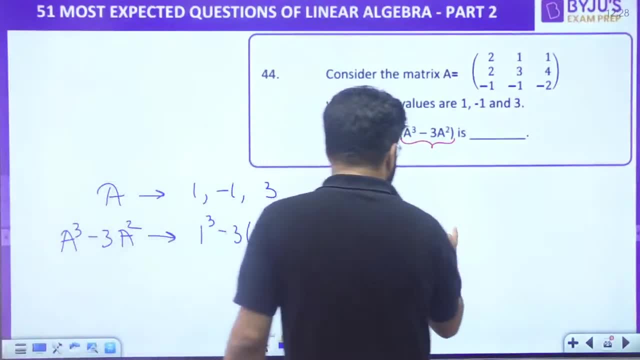 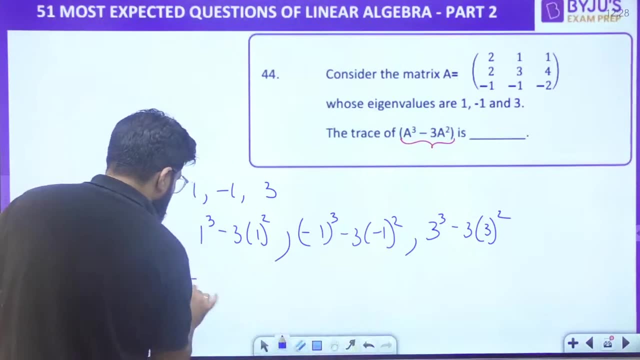 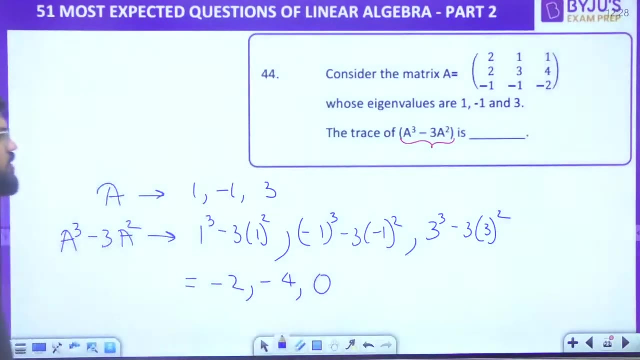 same has to be applied to lambda. and next is 3 cube minus 3 into 3 square. there your total. get now again: 1 minus 3 minus 2 minus 1 minus 3 minus 4, 3 cube minus 3 cube 0, the minus 2 minus 4: 0. now what is the trace? now? what is the trace? 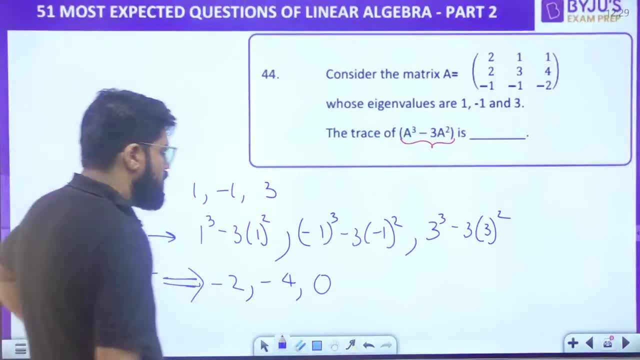 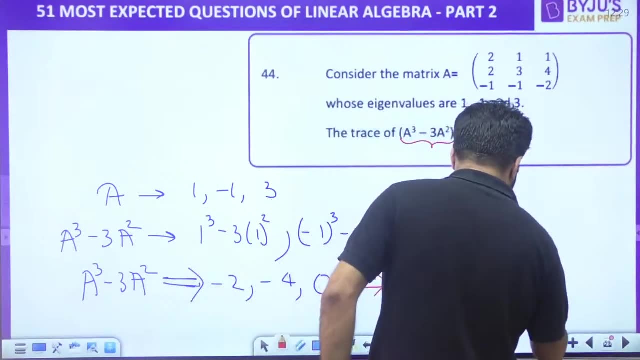 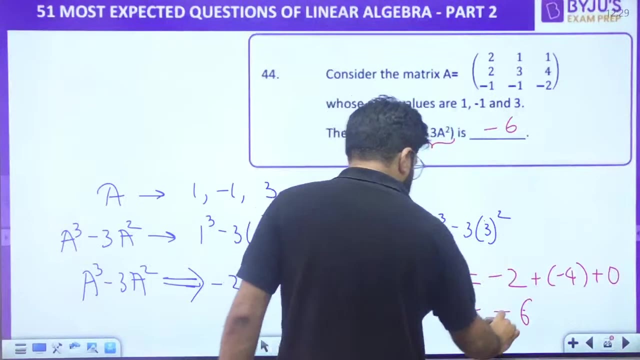 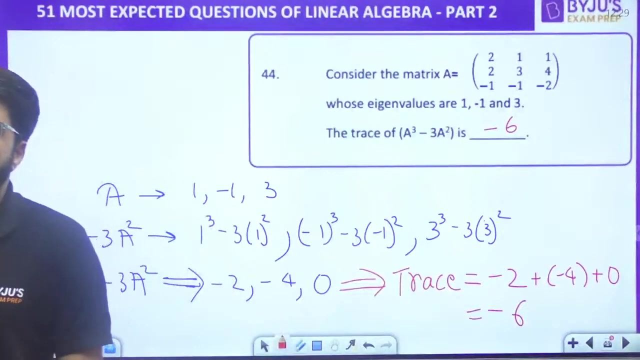 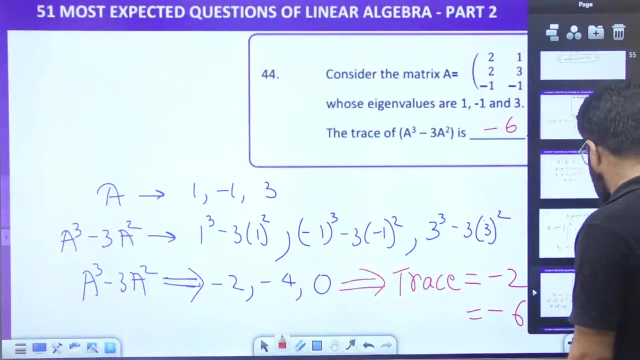 so what is the trace? the trace of matrix is sum of eigenvalues and the trace of the matrix should be minus 6, simple one. the trace of the matrix there is minus 6. every question has some learning process associated. every question has some learning associated. next question: let a. 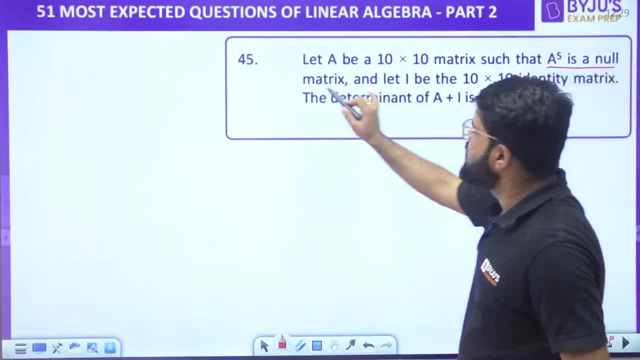 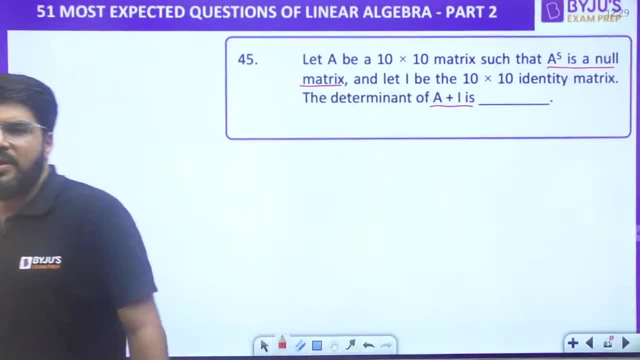 be a 10 cross 10 matrix, such that a power 5 is a null matrix. right, let I be the 10 cross 10 identity matrix. what is the determinant of a plus I? what is the determinant of a plus I? a power 5 is equal to null matrix. and what are the? 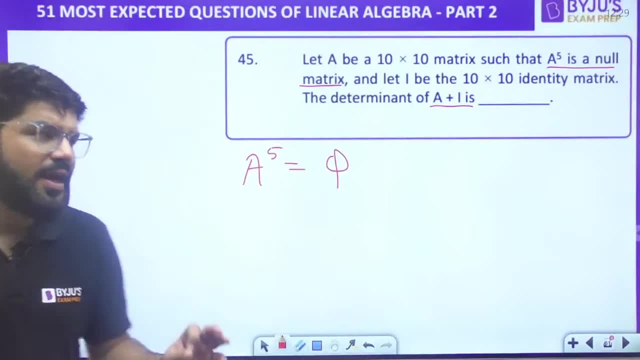 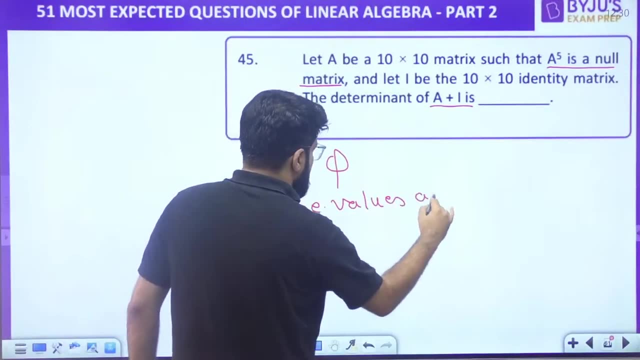 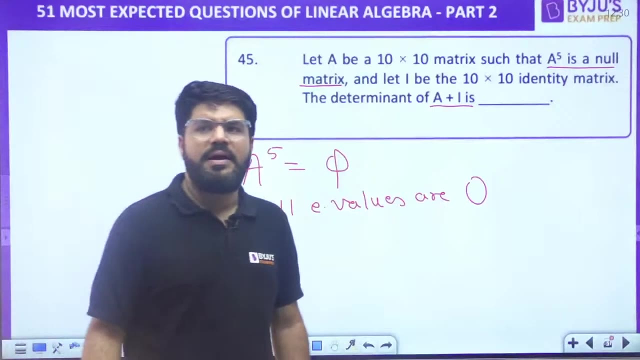 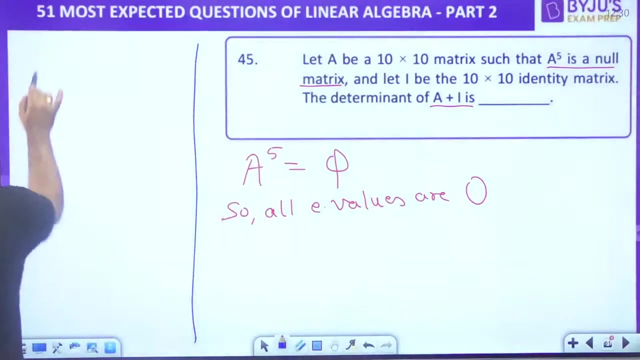 Eigen values of null matrix. what are the Eigen values of null matrix? Eigen values of null matrix? guys, please make a note, should remember all eigen values of path will. matrix is just zero, zero, zero, zero, zero, zero, nothing. okay, utcha observe, if a has eigen value, lambda, a power 5 will have eigen value. 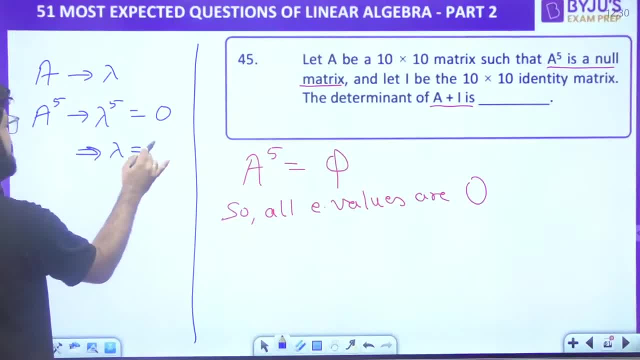 lambda power 5 will produce surprised parallel 84, 8 hertz, all kinds of exponential, pá шåban infinity. sorry, 5, but that is 0, so that means lambda is also 0. so what are the eigenvalues of a? also, what are the eigenvalues of a? they are also all 0. how many zeros? 10 zeros. it is a 10 cross. 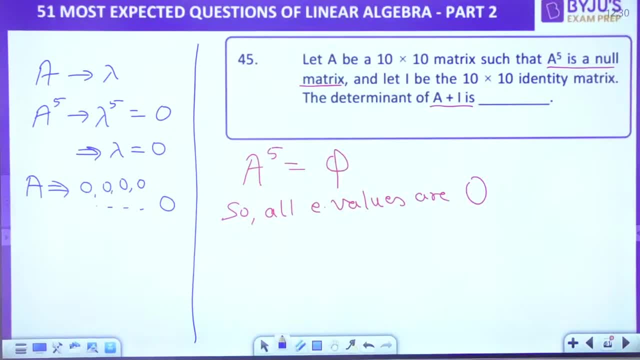 10 matrix. it will have 10 eigenvalues, right? what is the determinant of a plus i tell me. so what should be the eigenvalues for a plus i? a plus i means lambda plus 1, so that will be 0 plus 1. so 1, 1, 1, 1, 1, up to 10 times. what is the determinant of a plus i determinant? 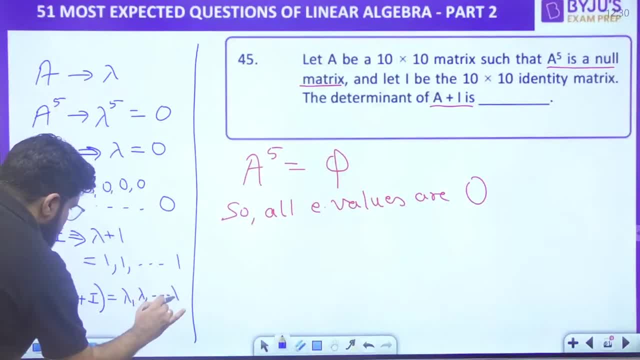 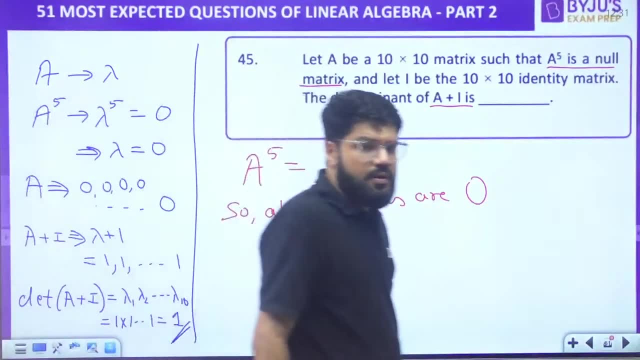 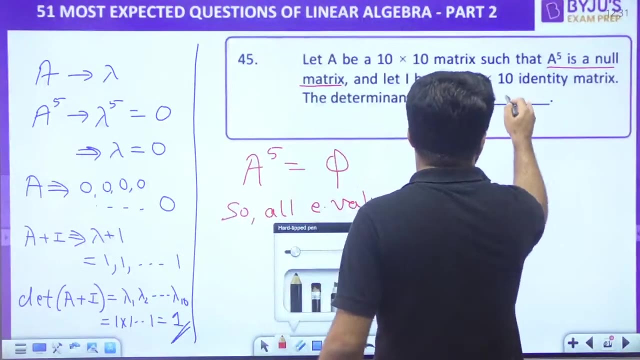 of any matrix is product of these eigenvalues, lambda 1 to lambda 10. but all are 1, so answer is also 1. all are 1, so the answer is also equal to the 1. you have to be strong, strong with the properties. you have to be strong, strong with the properties. 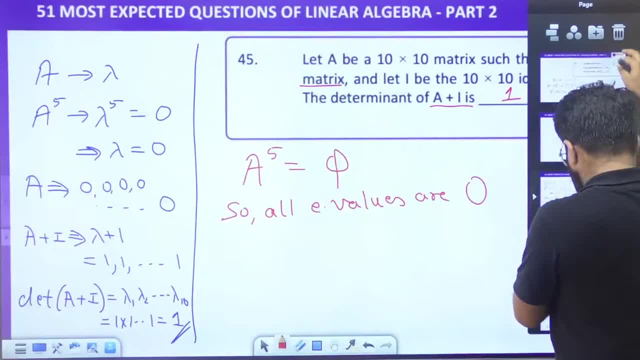 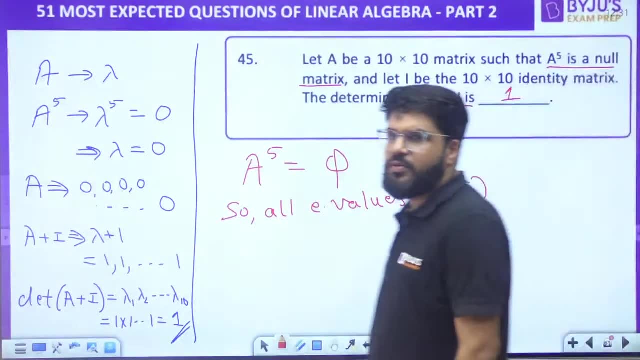 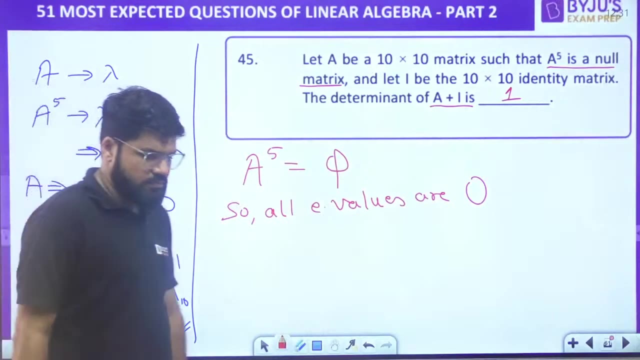 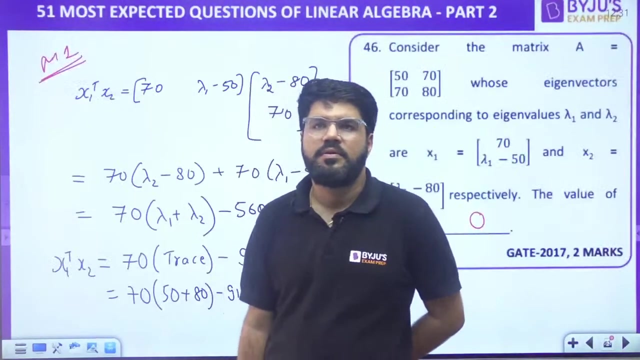 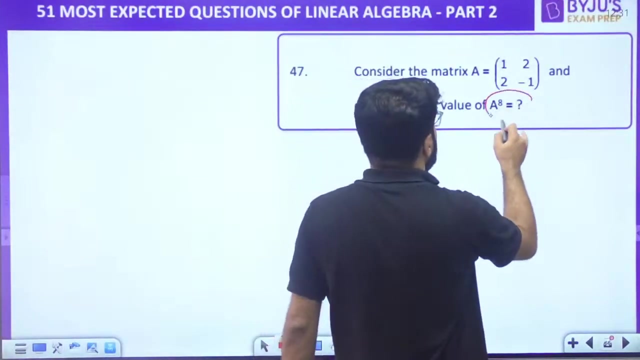 you have to be strong and strong with the properties. you have to be strong and strong with the properties. next one, next one, moving ahead to the next one. this 46 was already done. coming to the question number 47: determine the value given the value given the matrix and determine the value of a power 8. can anybody tell me this question? 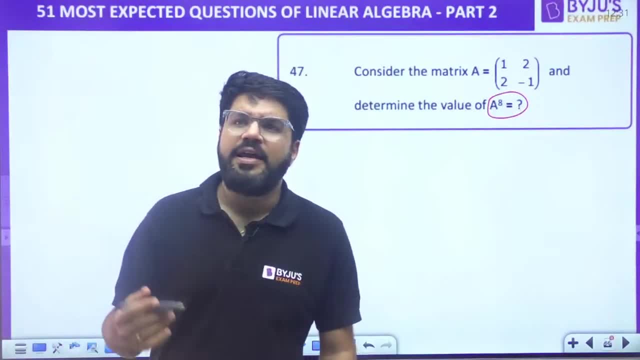 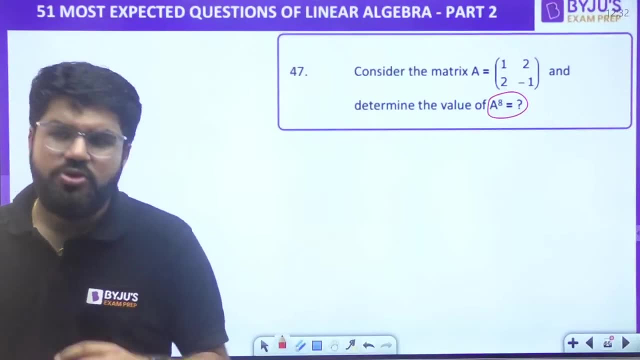 should be based on what matrix a and find the higher power of a. do you really need to? you know calc. multiply a, a a several times, then it is just a lengthy approach. what should be this question based on? what should be this question based on anybody? yes, perfect. so what is the eigenvalues of? 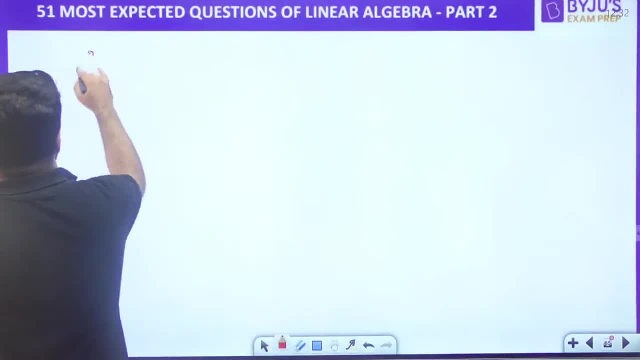 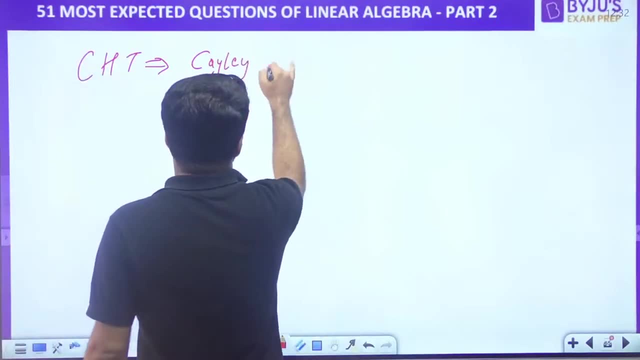 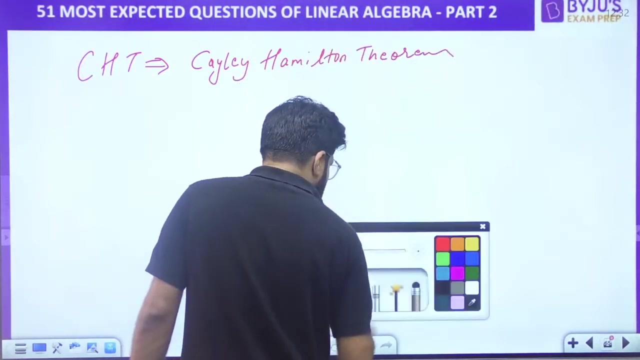 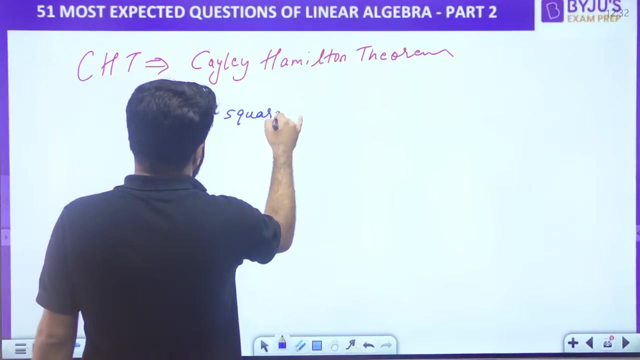 ht erased. so you are following rationally somebody. yes, perfect, it has to be actually based on cht, that is kiley hamilton theorem. so let us revise this too. what is that kiley hamilton theorem? it states that every square matrix has 0 plus and minus. that is calledかな. 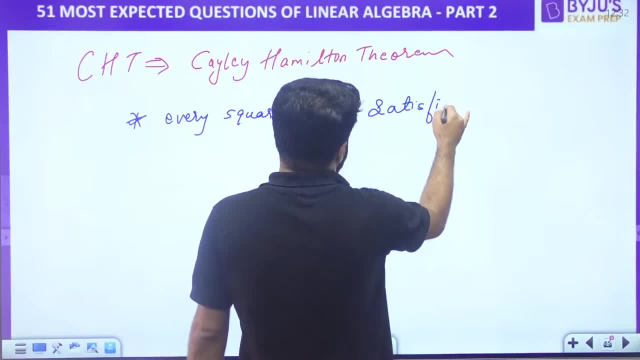 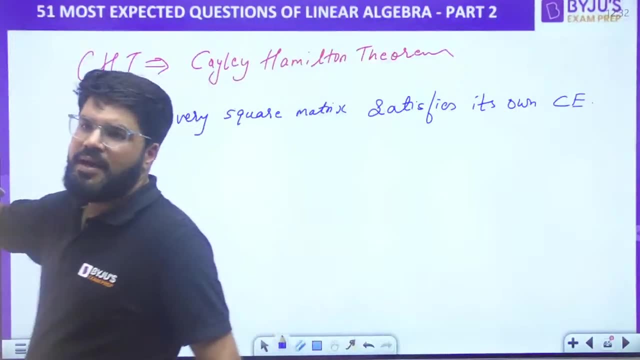 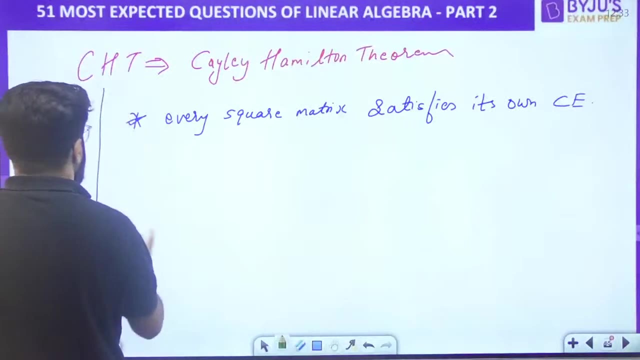 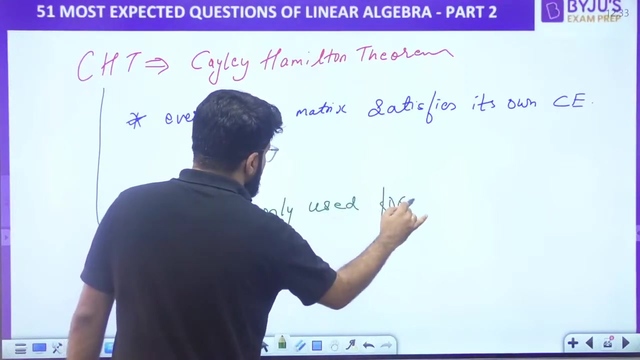 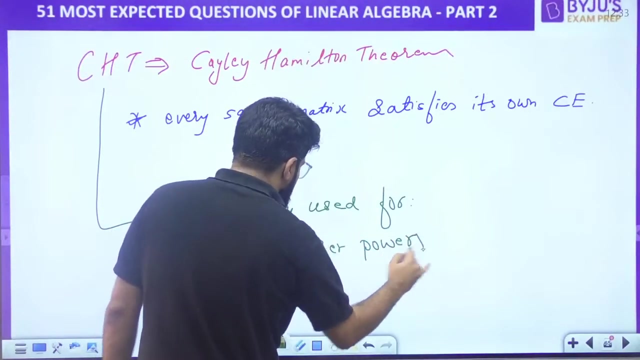 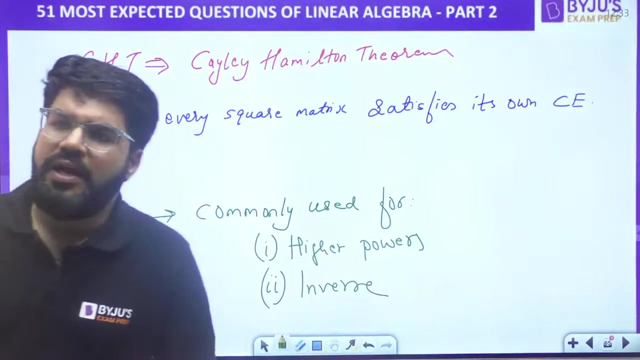 ip will find whichheiten that every square matrixc j is the only possible element of satisfies its own characteristic equation. every square matrix will satisfy its own characteristic equation. right kiley hamilton theorem commonly used for number one to determine higher powers of a right and number two the inverse calculations of the matrix. commonly this is used for higher. 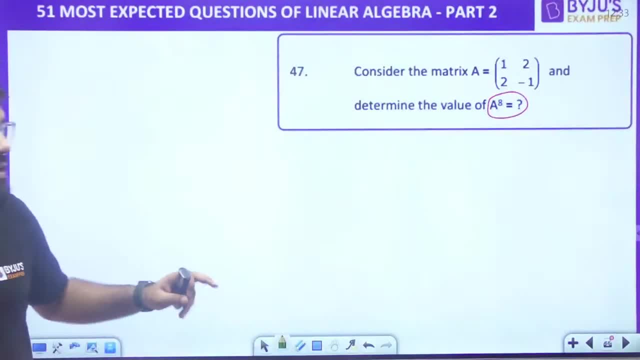 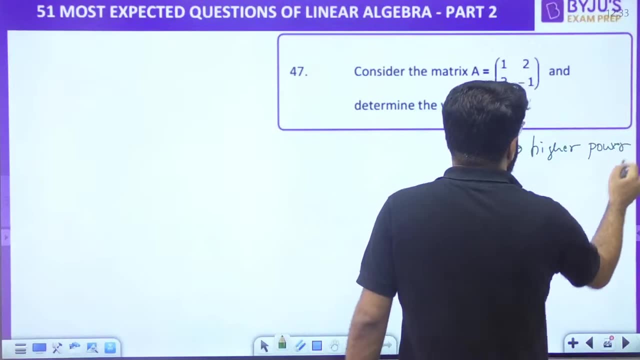 power calculation or inverse calculation of any matrix. now, here this is the question of a power 8. that means it is a question taking you towards the higher power. calculate the higher power. whenever a question on higher power you see, think about kiley hamilton theorem. think about the kiley. 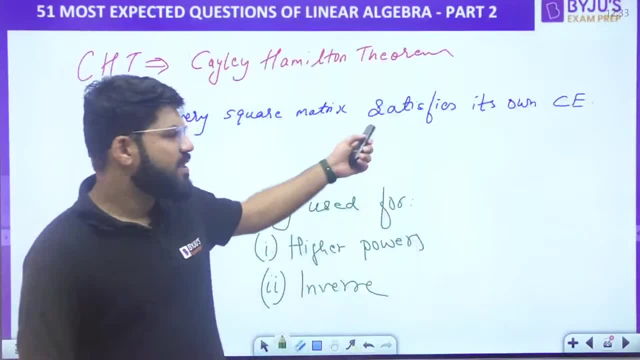 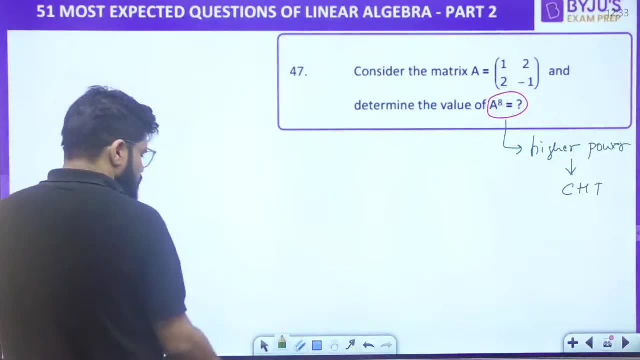 hamilton theorem. now how to apply on this characteristic equation, will explain you through the question. every square matrix satisfies the characteristic equation. sir, what is the characteristic equation? it's a two cross, two matrix. now we can easily write that. what is the characteristic equation? lambda square minus trace into lambda plus. 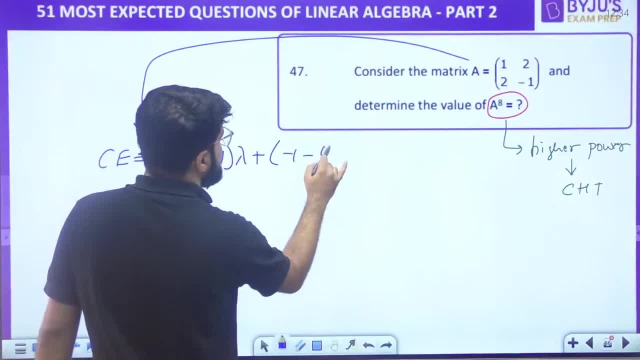 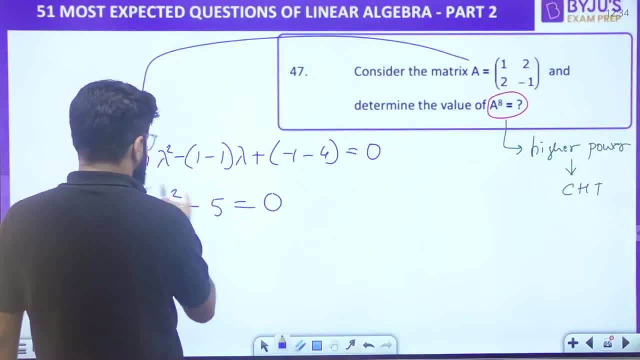 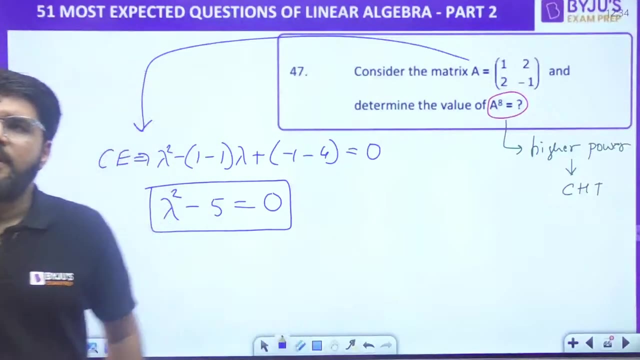 determinant. minus one minus two, twos are four equal to zero. so i have lambda square. the center one is zero minus five equal to zero. this is the characteristic equation. now, every square matrix will satisfy its own characteristic equation. every square matrix will satisfy its own characteristic equation, right? so if i apply the kiley hamilton theorem, every square matrix will. 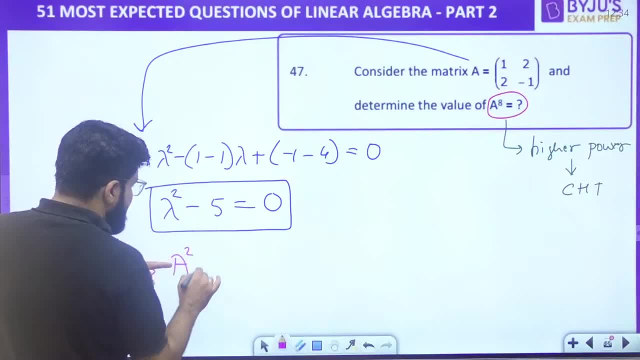 satisfy this equation. so in place of lambda you can put a. so this is a square minus five. now, a is a matrix, a square is a matrix and matrix minus number is not possible. so what you should do: multiply by the identity unity part, unity matrix part. that is i, so a square minus five i. 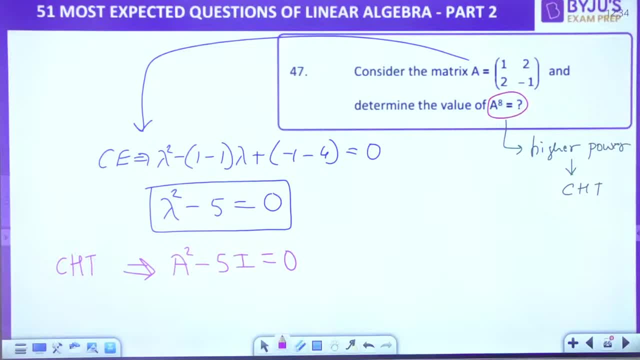 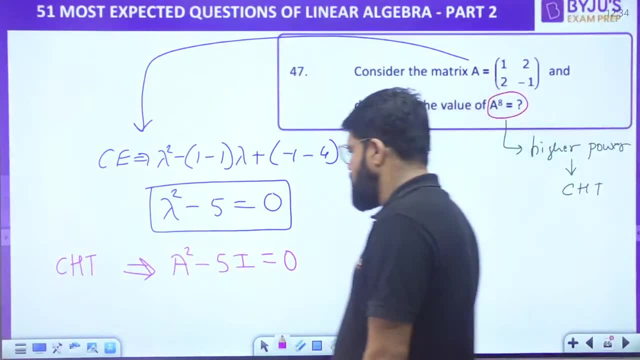 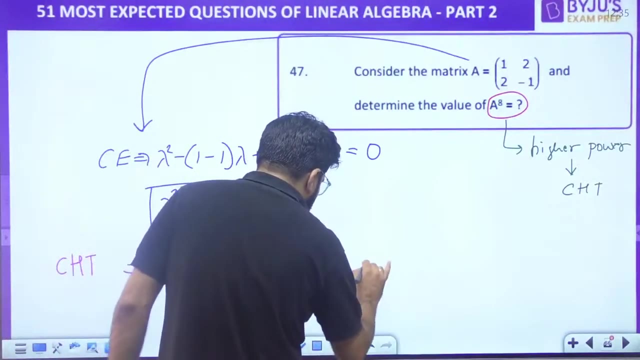 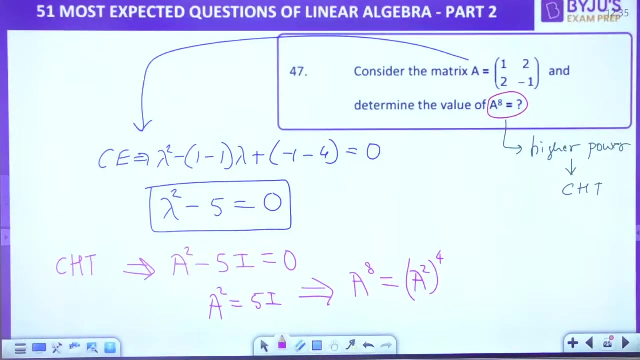 is equal to the zero. a square minus five i is equal to zero. so from here i have got what should be a square. that is five. i right, if a square is five, i question is asking: a power eight? a power eight is a square. power four. a power eight can be written as a square key: power four. what is the a square five? i? 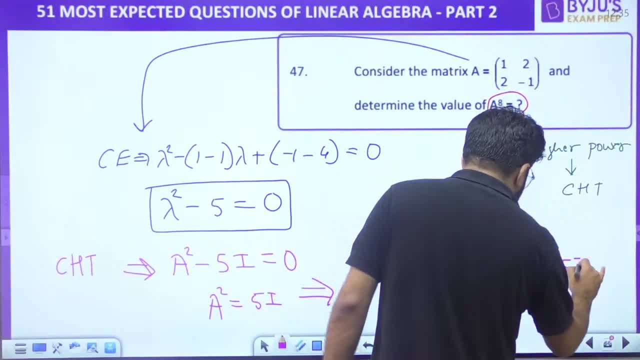 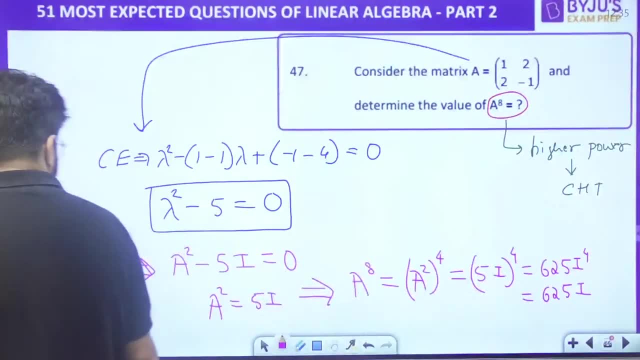 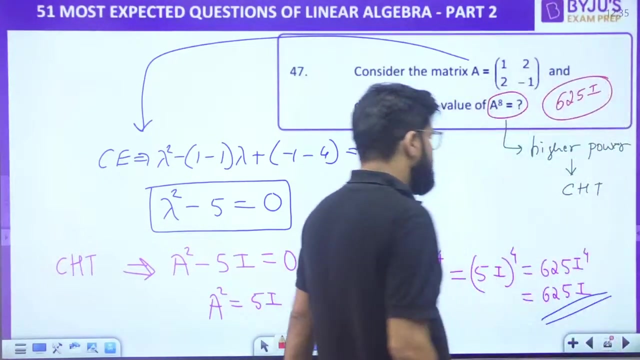 five i key power four, that is 625 i. power four and that is 625 i. that is 625 i. that is known as 625 i. so what is the answer for the question 625? i determine the value of a power eight. your answer is 625 i right. 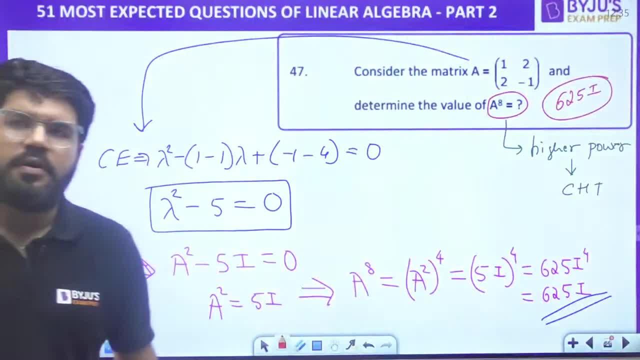 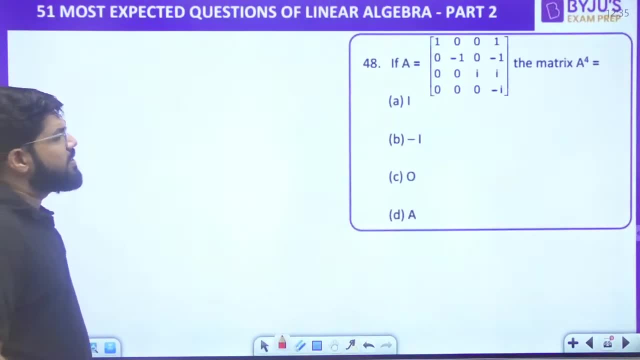 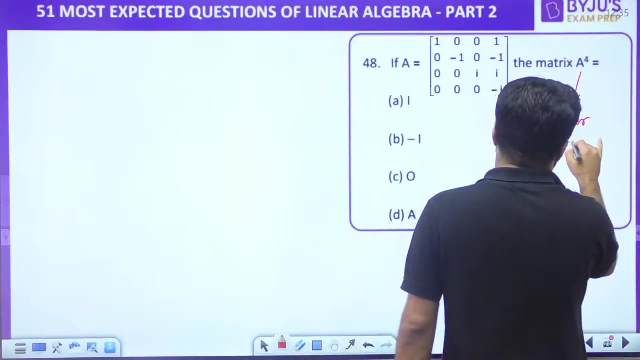 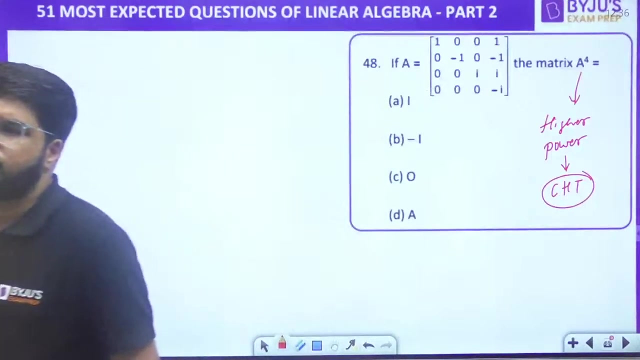 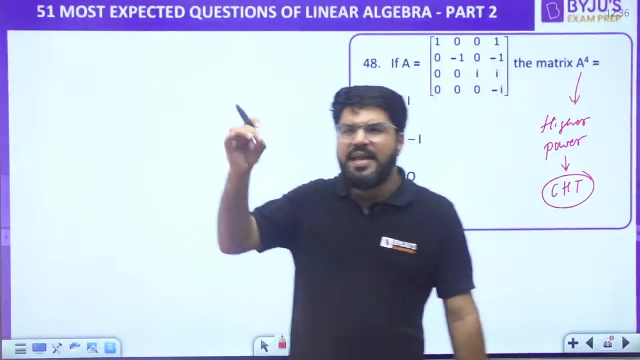 625 i, higher power, another one matrix and a power four. once again higher power. once again you see the higher power. so once again, think about the kylie hamilton. right, think about the kylie hamilton, but this is a four cross four. kylie hamilton needs the. 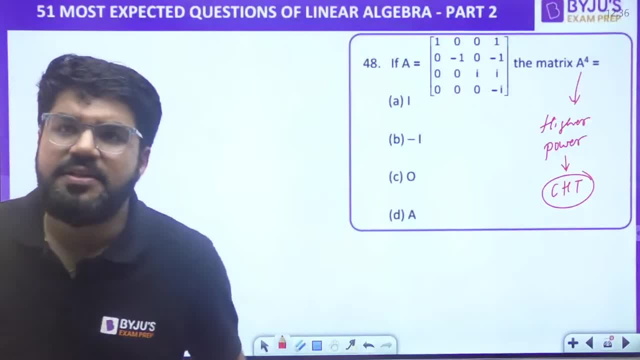 characteristic equation. every square matrix will satisfy the characteristic equation. every square matrix will satisfy the characteristic equation. this is a four cross four. what is the? this is a four cross four. what is the? this is a four cross four. what is the characteristic equation of four cross four? 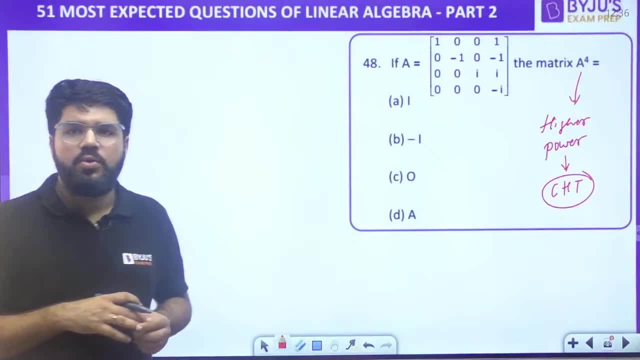 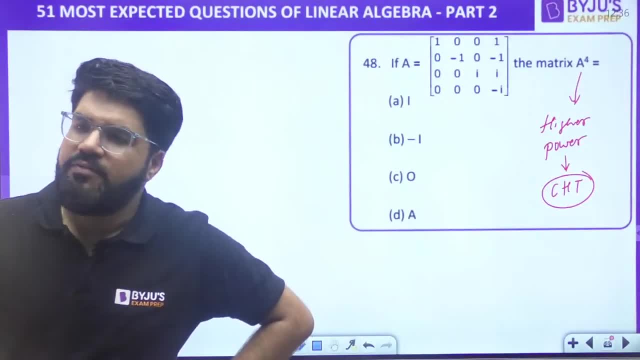 so what to do? characteristic equation of four cross four directly. i don't know i have given you cross four directly. i don't know i have given you cross four directly. i don't know i have given you two cross two. i've given you three cross three. 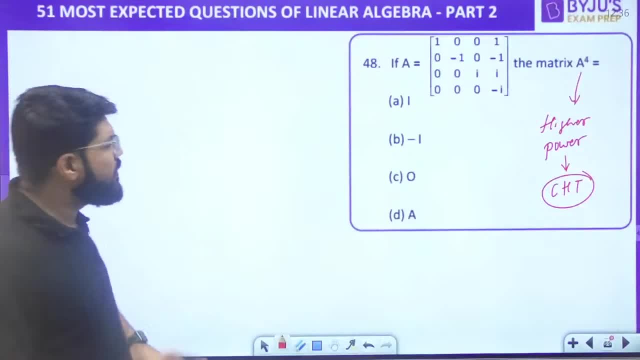 two cross two. i've given you three cross three, two cross two. i've given you three cross three, four cross four. will it be time taking here it? four cross four. will it be time taking here it? it will not be time taking because the type of matrix that is given to you observe this: this is 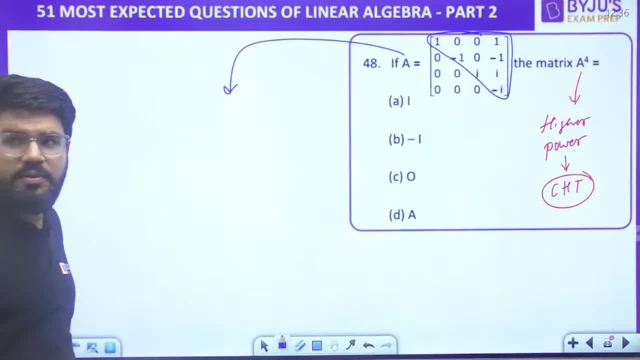 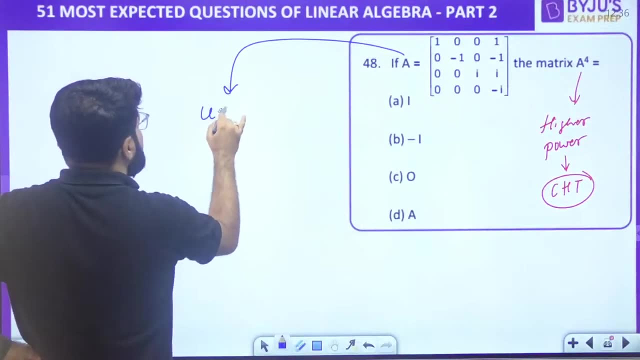 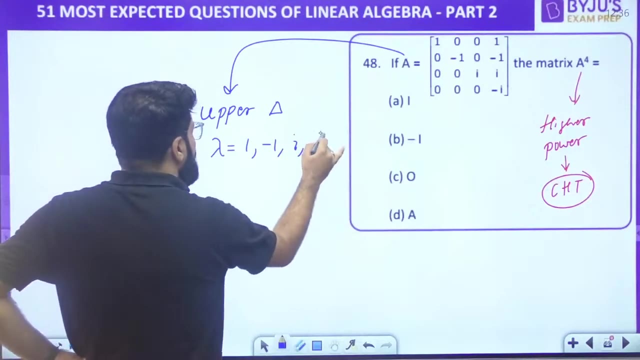 again upper triangular. that is what is going to make the question simple: a power 9, a power 8 into a akg right. so this is upper triangular right. if it is upper triangular, eigenvalues are equal to diagonal numbers. but i don't want the eigenvalues, i want the characteristic equation only. how can i? 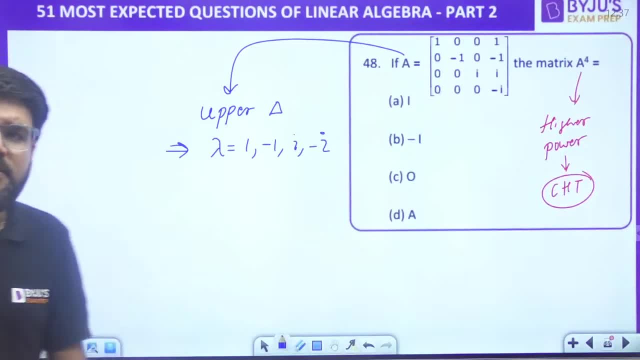 find the characteristic equation. eigenvalues are roots of characteristic equation. so what should be the characteristic equation? it should be lambda minus 1, then only you get lambda equal to 1, then lambda plus 1, then lambda minus i, then lambda plus i. from the knowledge of the roots i have got the. 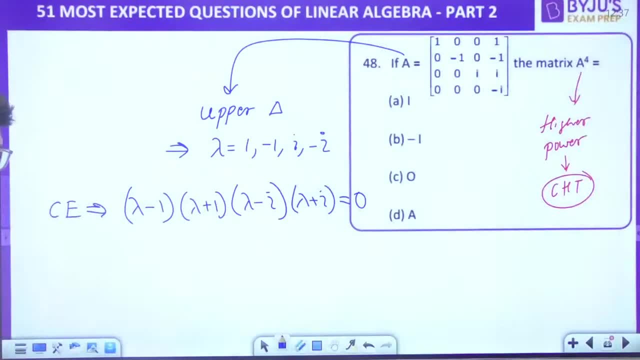 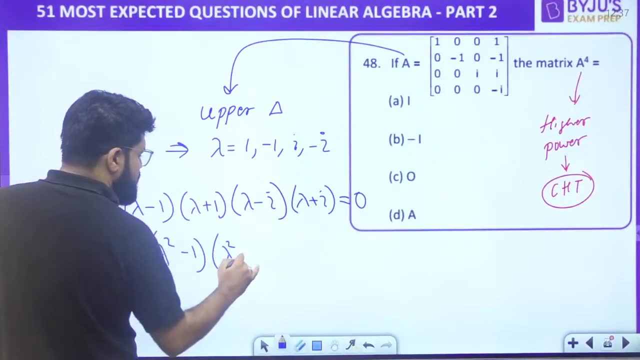 factors, multiply, you get the characteristic equation. that is how you make the problem simple. so lambda minus 1, lambda plus 1 is lambda square minus 1. lambda square minus i square minus i square will be plus 1 and this is 0. again, a minus b, a plus b. so lambda power, 4 minus 1, equal to 0. this is what is your characteristic. 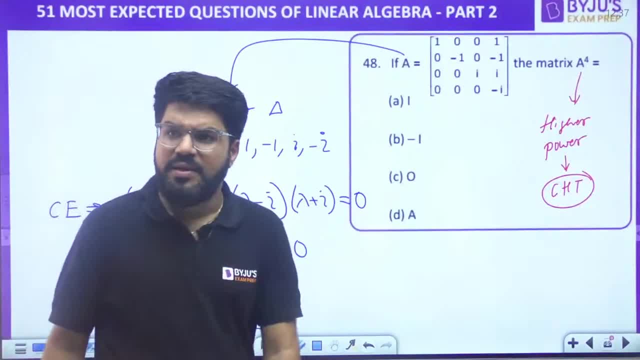 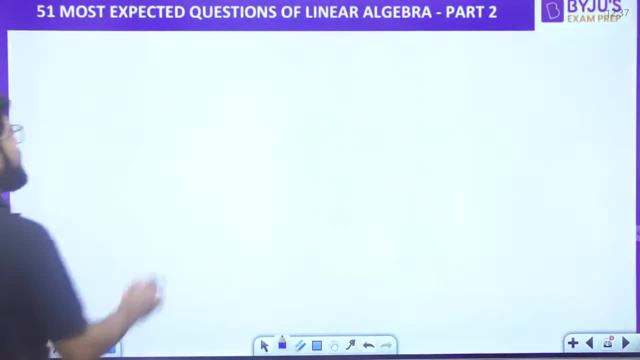 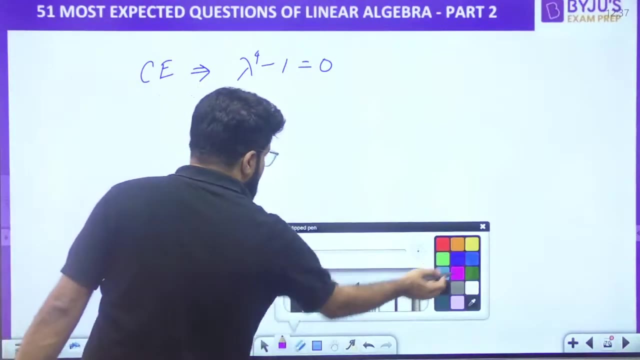 equation final. this is what is your characteristic equation final. don't worry, we'll plan full marathon of apti maths. everything will plan, don't worry. okay, so what is the characteristic equation? lambda power 4 minus 1 is 0. now it is the turn to apply the kylie hamilton theorem. kylie hamilton theorem. 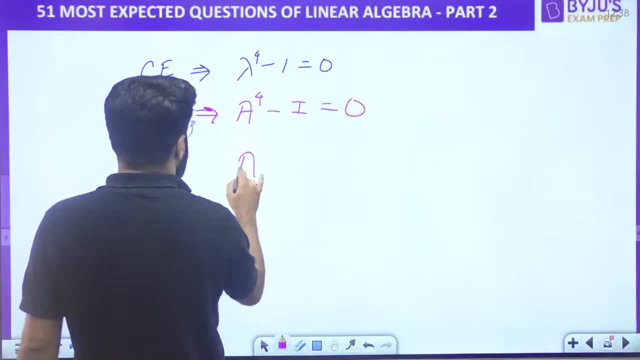 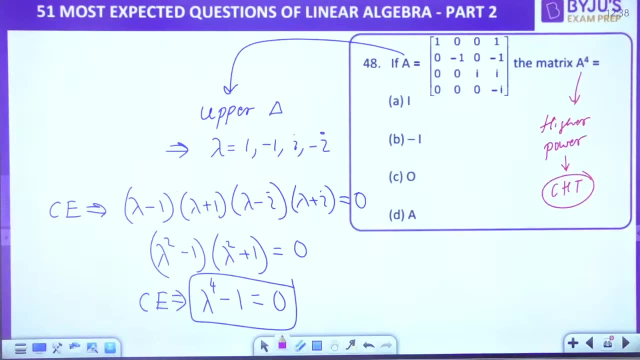 a power 4 minus 1, 1, 0. so what should be the? a power 4 is equal to identity. what should be the? a power 4 is identity. question is asking a power 4 only. the answer is option number a. finished, very simple, finished. 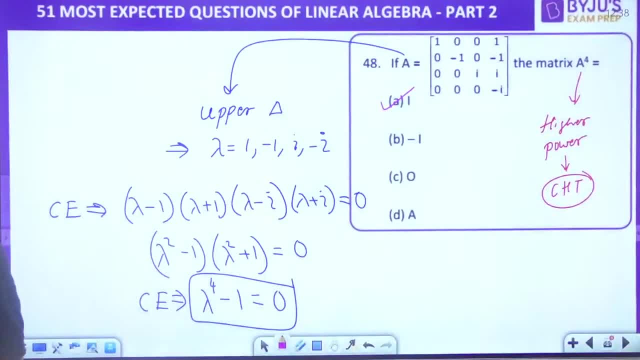 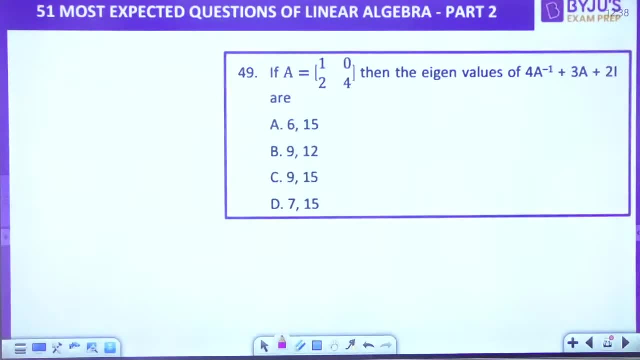 and simple, katham. this is finished and very simple. next question for you, number 49: if a is 1, 0, 2, 4, what are the eigenvalues? are a? this is not on kylie hamilton, actually here it is wrong. this is lower. 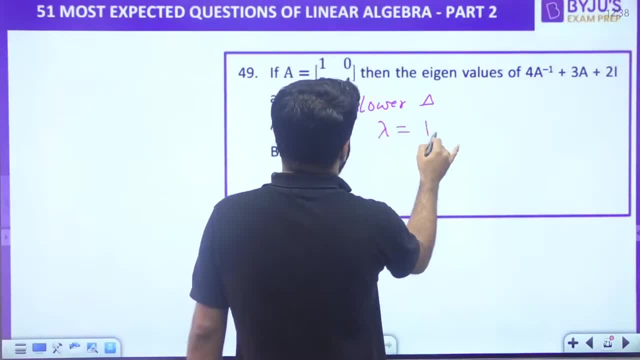 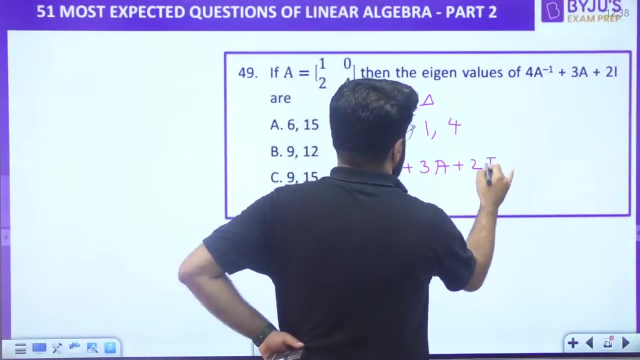 triangular. this is lower triangular. so what are the eigenvalues 1 and 4? whether it is upper or lower triangular, any triangular matrix eigenvalues are diagonal numbers. so what should be the eigenvalues for simple case 4a inverse plus 3a plus 2i? what should be the eigenvalues 4 into lambda inverse? 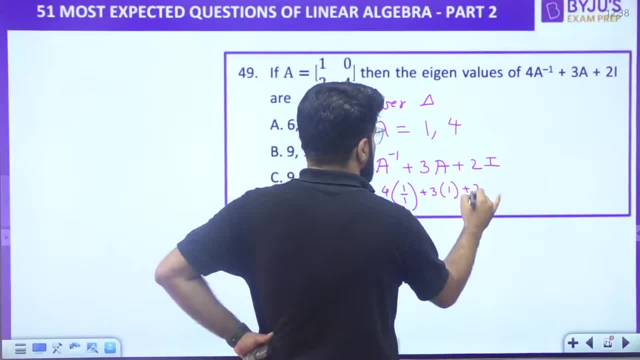 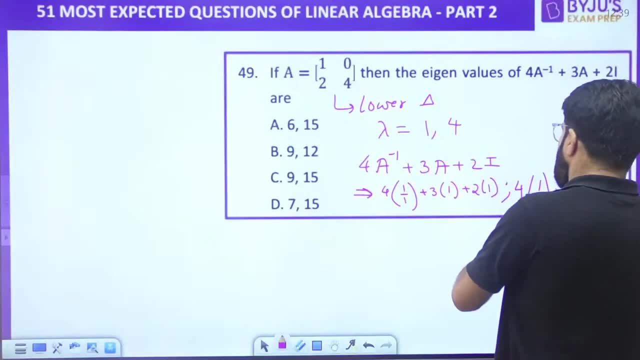 that is 4 into 1 by 1 plus 3 into lambda plus 2 into 1. and second, valakia hoga 4 into lambda inverse, that is, 1 by 4 plus 3 into 4 plus 2i, and i will be replaced by 1, so this is equal to 4 plus 3. 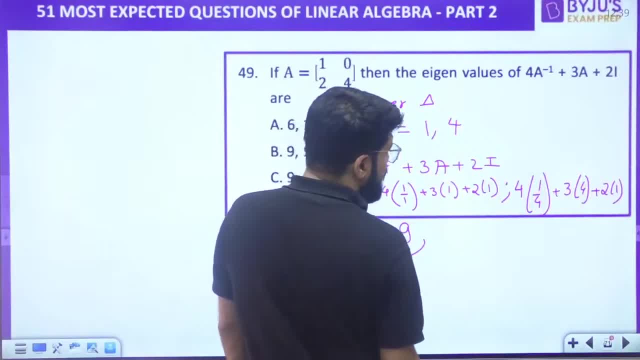 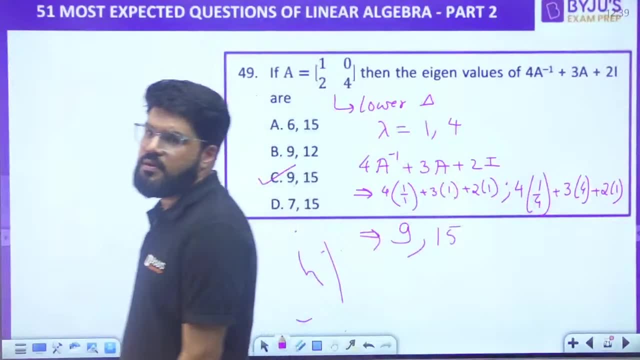 plus 2 is 9 and then 4 by 4, 1, 1 plus 12, 13 plus 2, 15, 9 and 15. is your answer? option number c: yes, simple guru, this is simple. option number c: 9 and 15. 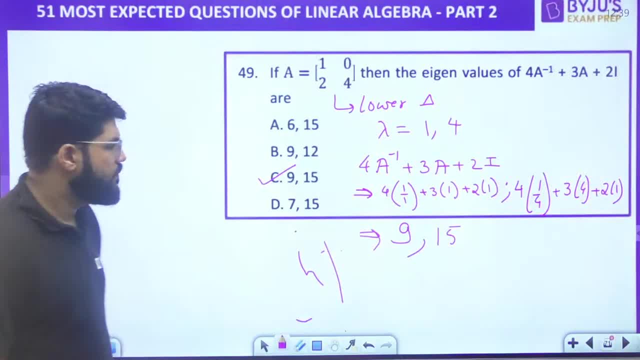 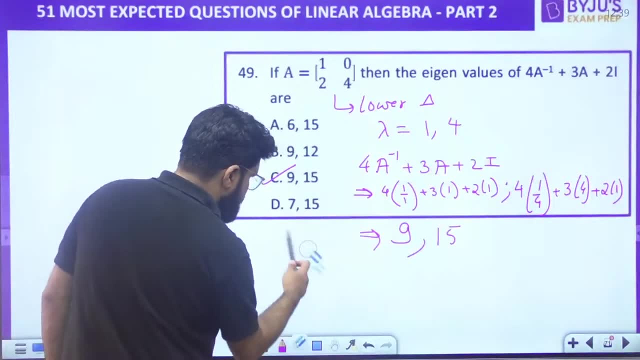 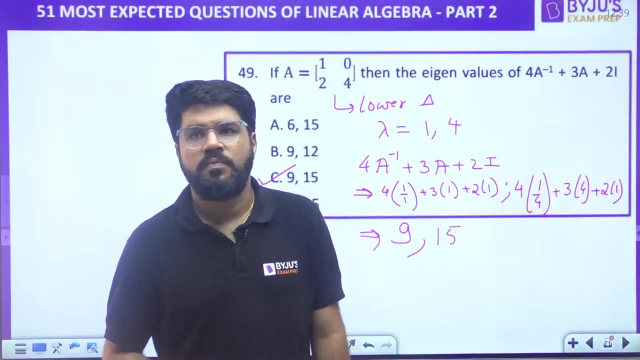 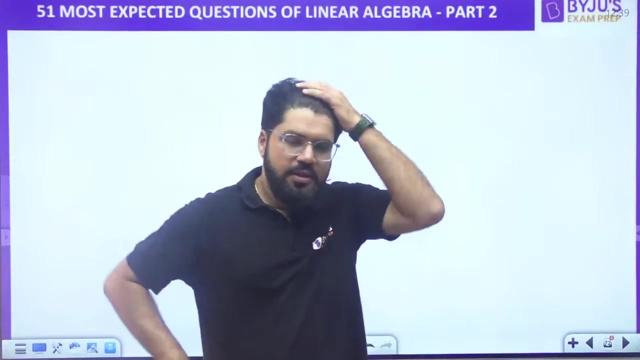 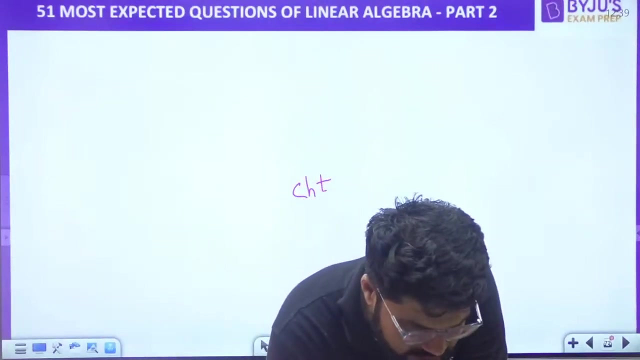 9 and 15. before i show you the next question, the password for today's pdf, like yesterday, i will share you the today's pdf in the telegram, which telegram i am going to share. let me once again share you the link of the telegram. let me just share you the link of the telegram and, if you have enjoyed, 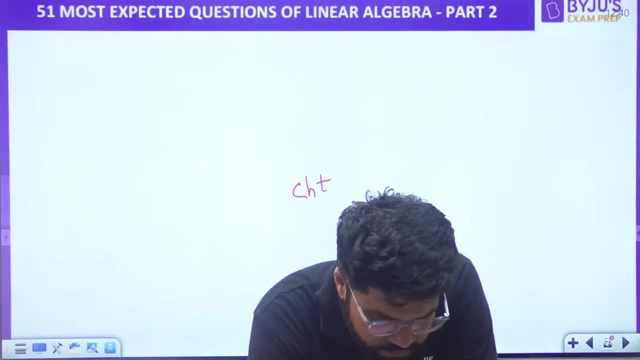 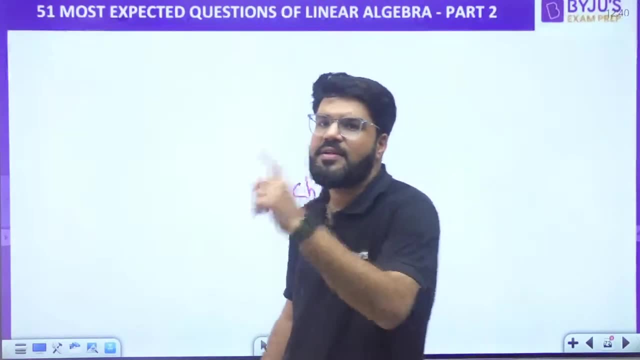 the session till now. please subscribe to my channel and i will see you in the next video. there are a few more questions, just wait for it. but if you have enjoyed the session till now, do not forget to like the session. let us increase the number of likes. this is the link of the telegram. password is cht. 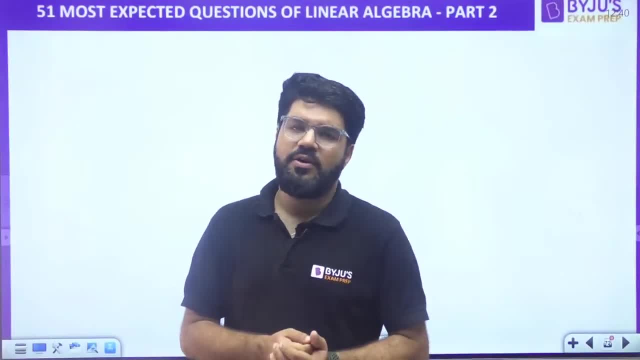 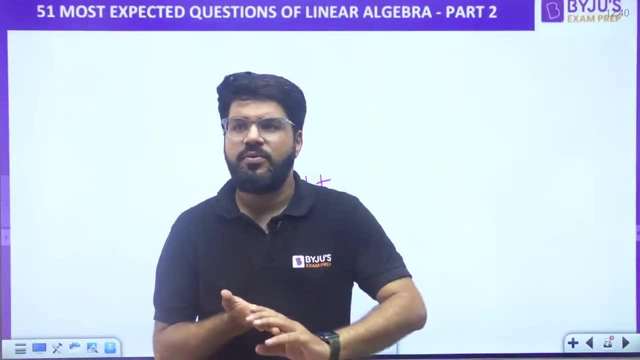 in short, kylie hamilton is what we discussed right now. so password is everything in small cht. okay, the pdf will be in the telegram group, the link i have shared with you. right for that only we need to have, okay. so this was the question number 49. 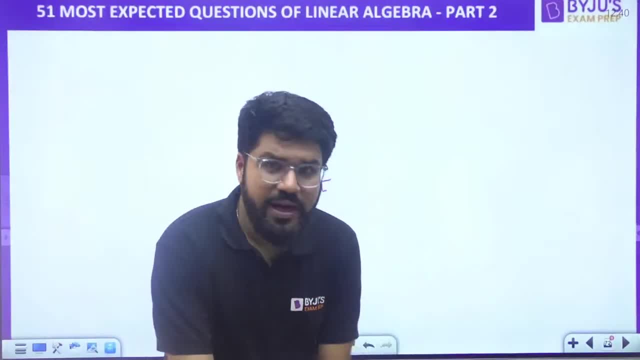 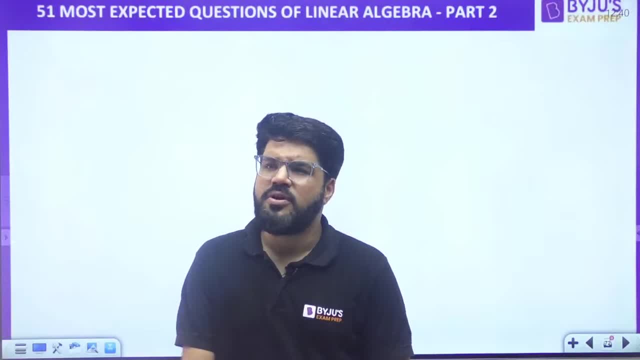 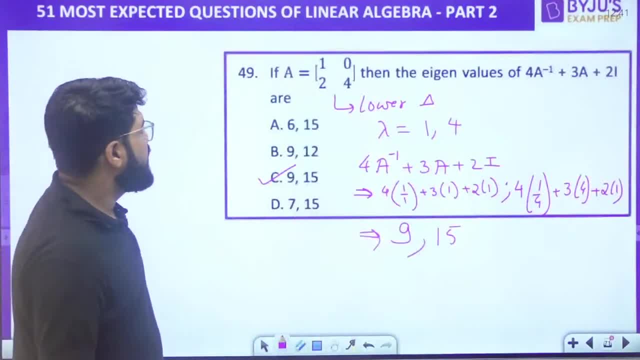 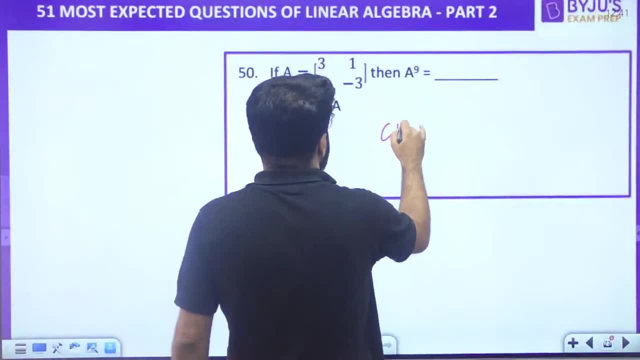 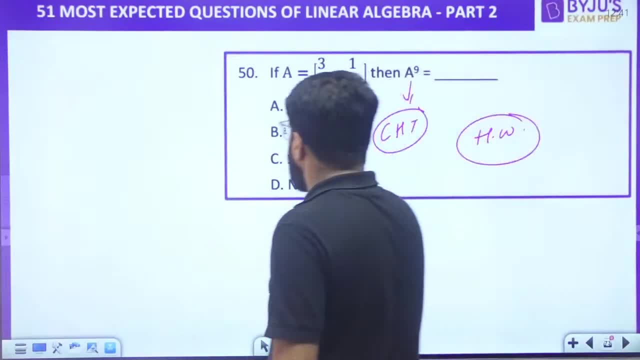 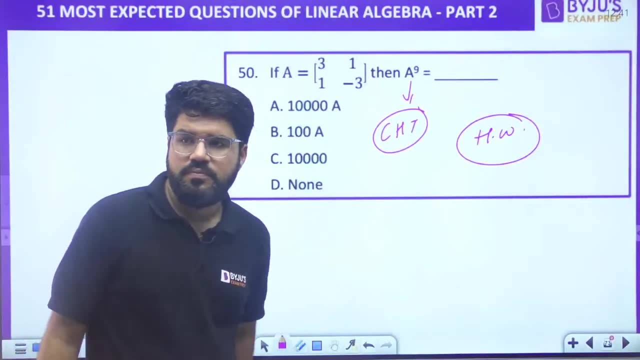 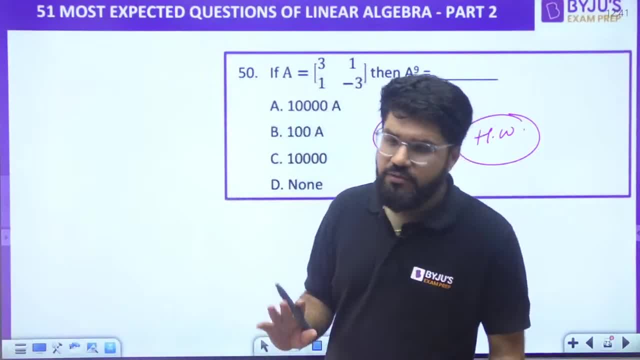 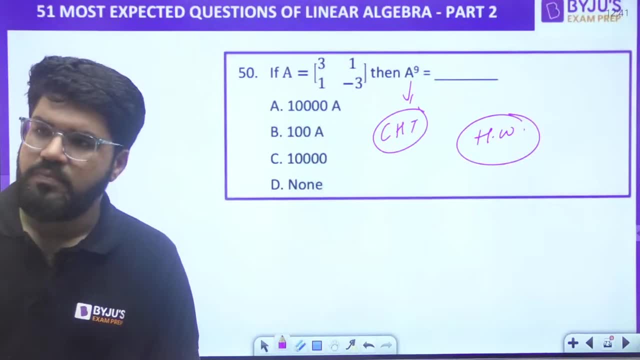 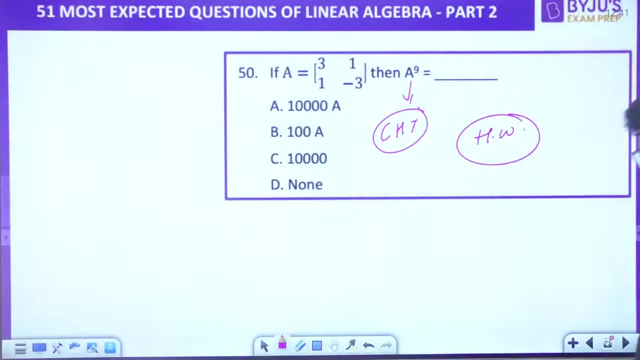 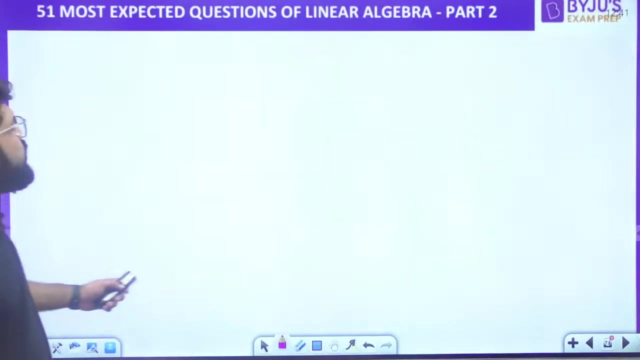 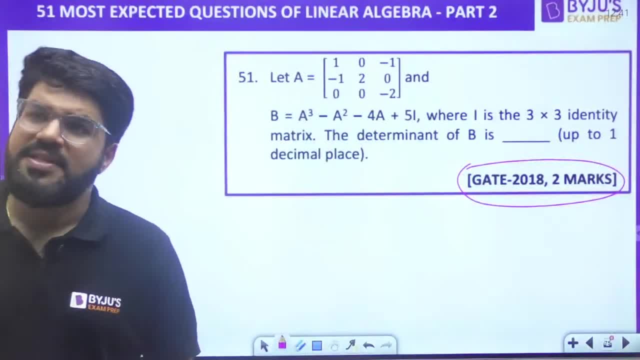 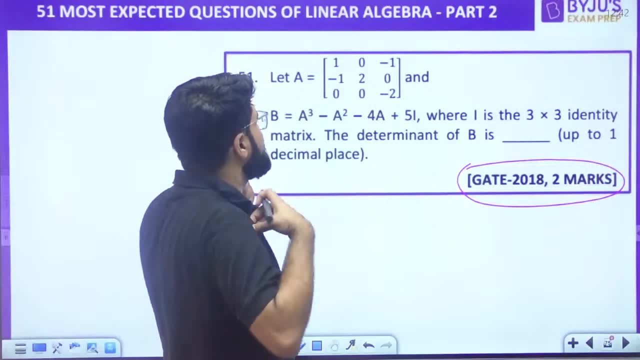 gate question. it's again a decent good question I want to discuss, and then we will go back to the AMGM concept. also, right, let A is equal to 1, 0 minus 1 minus 2, 0, 0, 0 minus 2 and B. 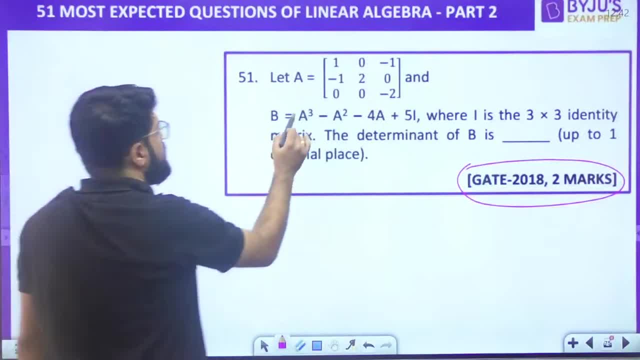 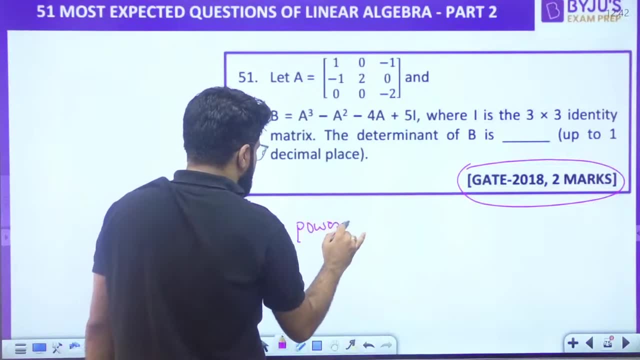 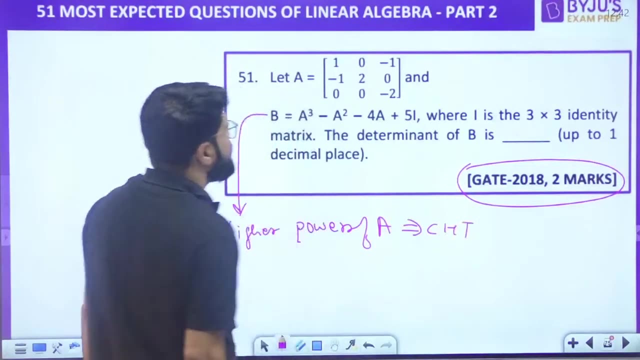 is given to you, where I is, the identity matrix. what is the determinant of B? Now, B is involving higher powers of A. B is a matrix that is involving higher powers of A right. so I will think about the Cayley Hamilton theorem. I will think about the Cayley Hamilton theorem. 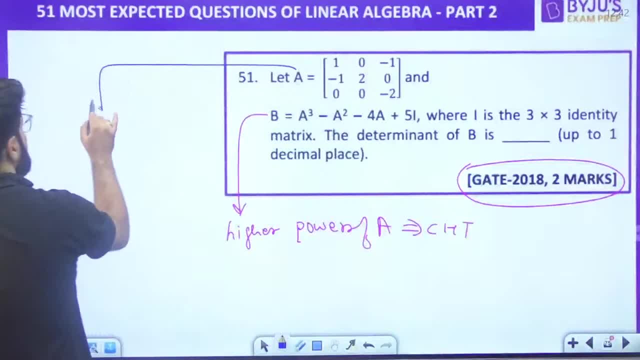 okay, For Cayley Hamilton theorem I need the characteristic equation. so what is beta 1, beta 2, beta 3, beta 1 is known as trace is known as trace. 1 plus 2 plus minus 2, that is 1, beta 2 is. 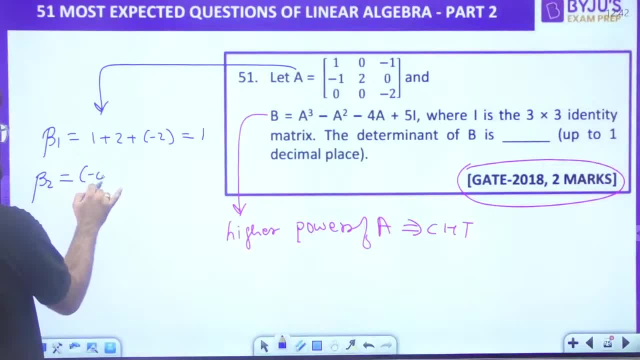 sum of the minor. so let me calculate: first one is minus 4 minus 0, next minus 2 minus 0, and third minor will be 2 minus 0, sum of the minus of diagonal numbers I have explained you in the beginning of the class. 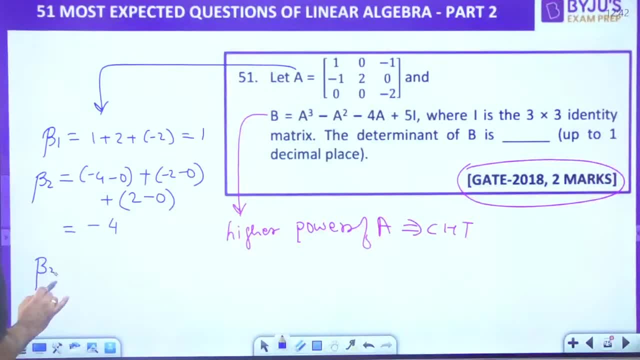 Let me stop the session. minus 2 plus 2: cancel. beta 2 is minus 4, what about the beta 3,? beta 3 is the determinant of the matrix. what should be the determinant? this is 1 into minus 4. 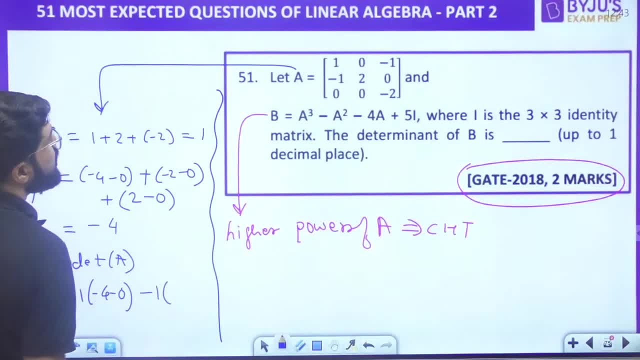 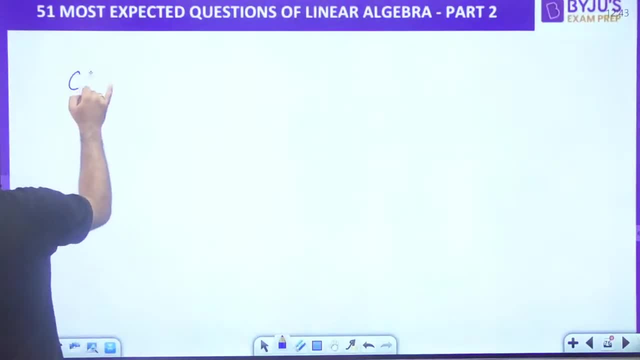 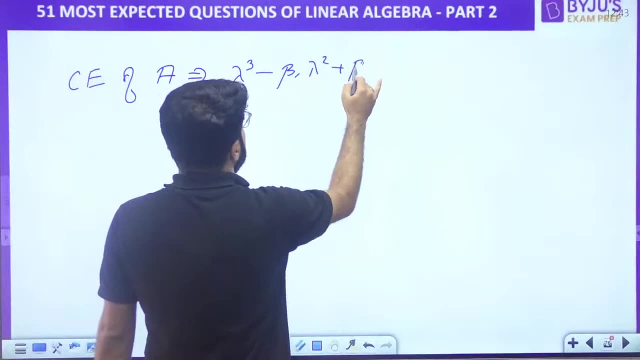 minus 0 and directly I have minus 1 into 0, okay. so determinant is minus 4, okay. So what is the characteristic equation for the matrix? A? Lambda cube minus beta 2.. Okay, That is beta 1 lambda square plus beta 2. lambda minus beta 3 is equal to 0, so lambda cube. 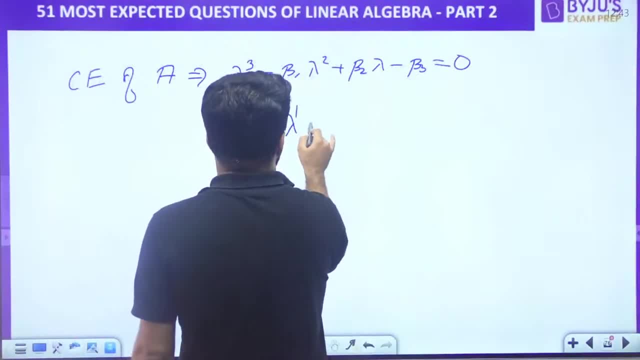 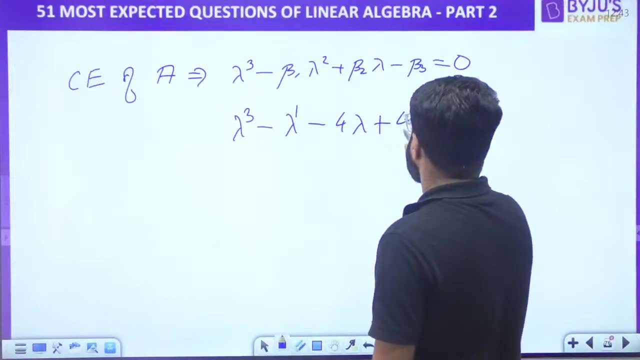 minus beta 1 square, that is, beta 1 is 1, so minus lambda square plus beta 2, beta 2 is minus 4, so this is minus 4 lambda minus beta 3, so minus minus here, plus 4 equal to 0.. 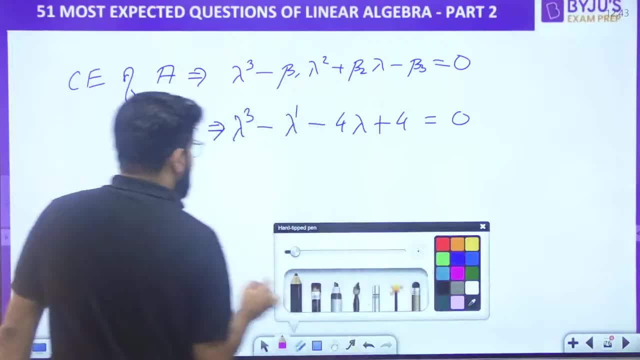 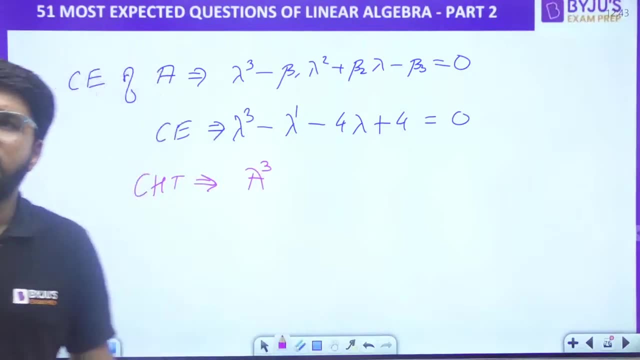 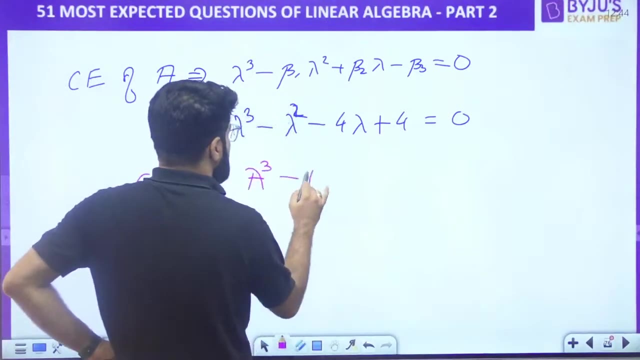 This is the characteristic equation of the matrix A and after taking the characteristic equation, I will apply the Cayley Hamilton theorem. Cayley Hamilton theorem says that every square matrix will satisfy. It is characteristic equation to put down lambda equal to A. This is A cube minus A square, minus 4A plus 4I. with the matrix it should be, I it cannot. 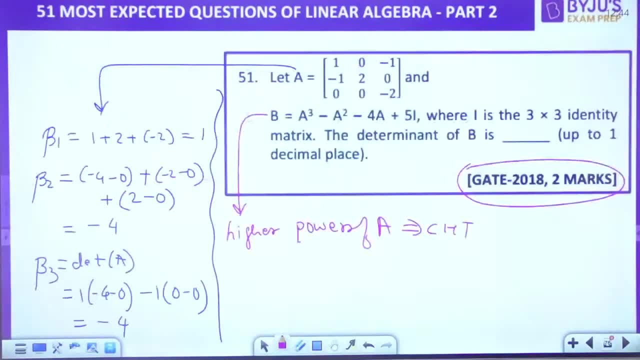 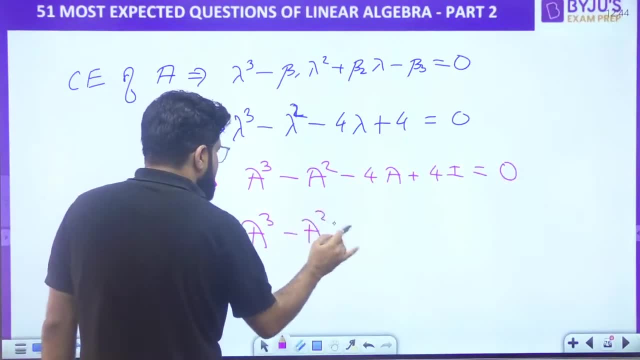 be a number. this should be 0,. right, this should be 0.. Now, what is the matrix B? it is similar to this: What is the matrix B given to you? A cube minus A square minus 4A plus 5I. 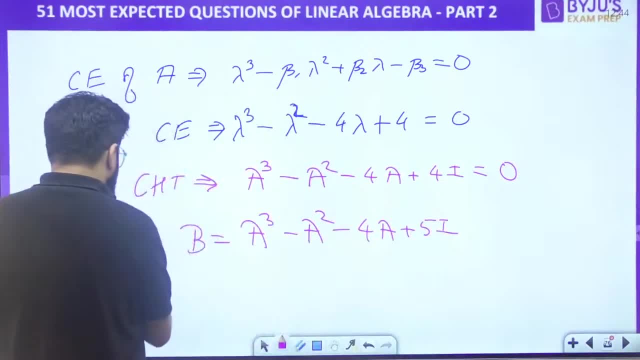 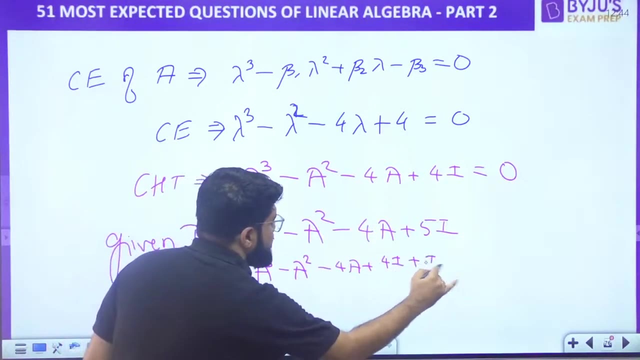 Okay, Okay, This is the matrix B given to you. This is the given matrix whose determinant is required. Now, only thing is- it is pretty much similar- this: you have to do A cube minus A square minus 4A plus 4I plus I. right, and up to this, much of part answer is 0 because of the Cayley. 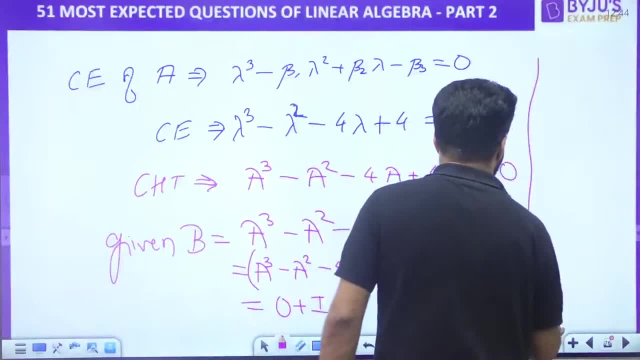 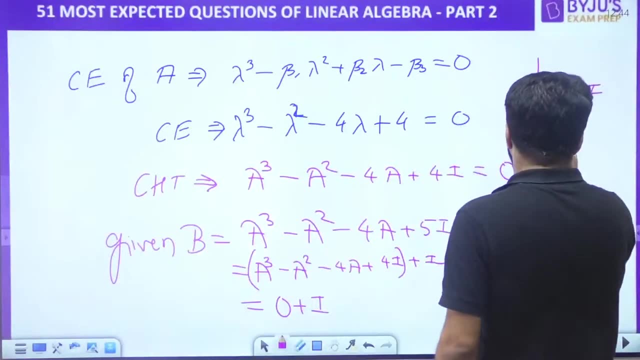 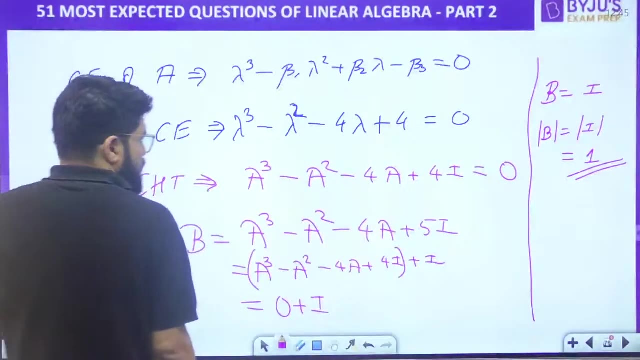 Hamilton theorem. So what is the B matrix? The B matrix itself is identity matrix. question finished. The B matrix is identity matrix. So what is the determinant of B Will be determinant of identity and determinant of any identity matrix is always one. 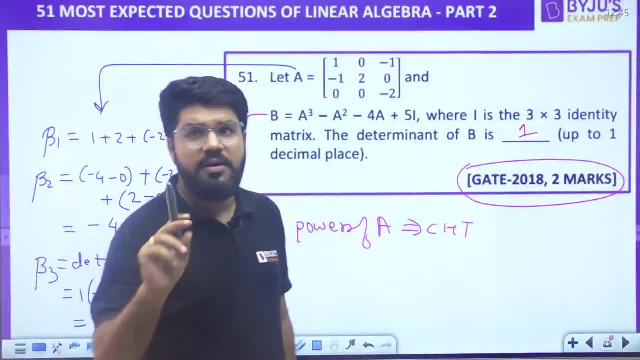 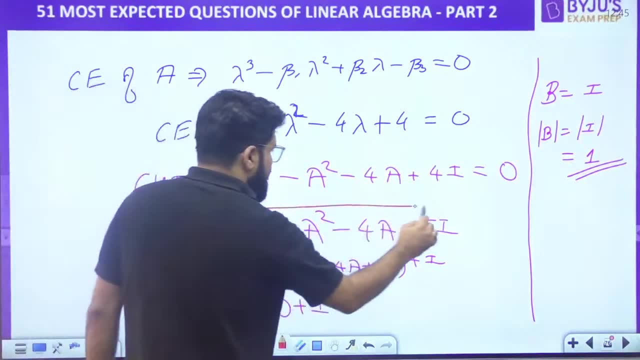 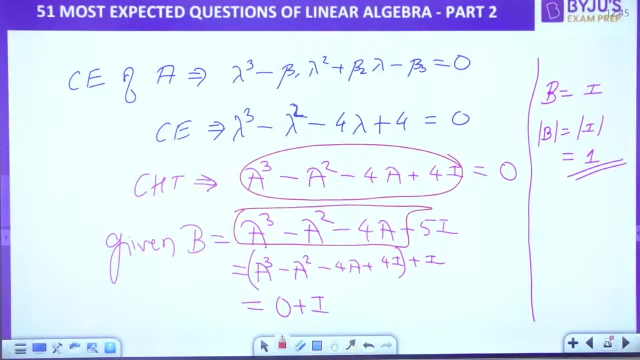 Okay, So one gate, two marker question level. also I have shown you from the Cayley Hamilton Simple conceptual question. Answer is one. The B matrix is given. okay, Up to this part is common. 5I was broken as 4I plus I and then it up to 4I it is just the 0 because of Cayley Hamilton result. 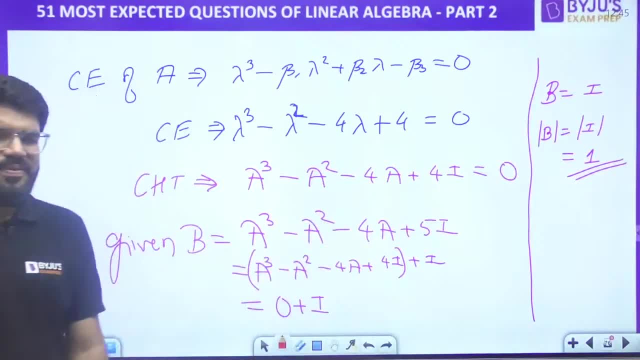 9B matrix is given and 5I was broken as 4I plus I and then it up to 4I. it is just a zero because of Cayley Hamilton result. okay, so B is just equal to I, so determinant of B is one determinant of. 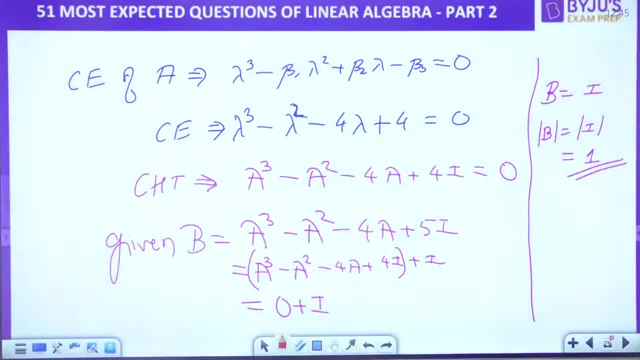 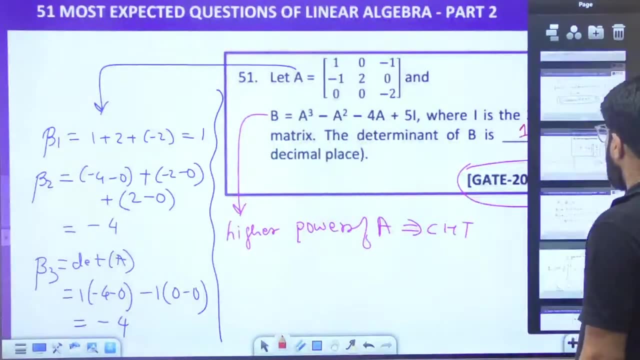 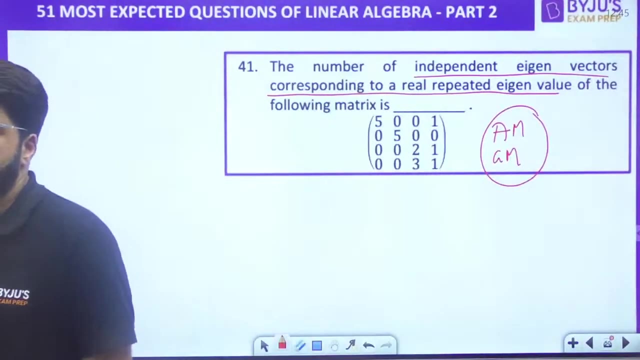 identity matrix is always one. okay, so this was the 51st question. but there is one question I told you. I'll explain in the last: Abhi pahle, property based kiya. now one more new concept. I have to add question number 41. I've shared, you know, money in the chat only once again it is there. 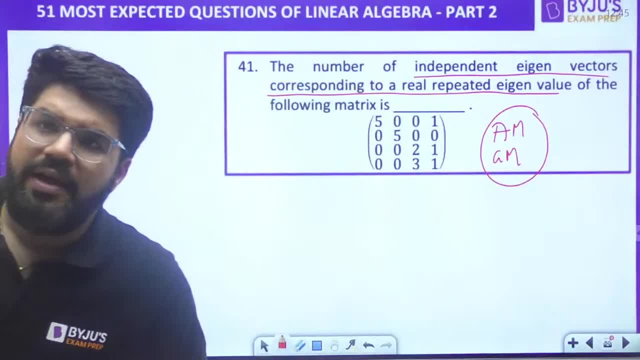 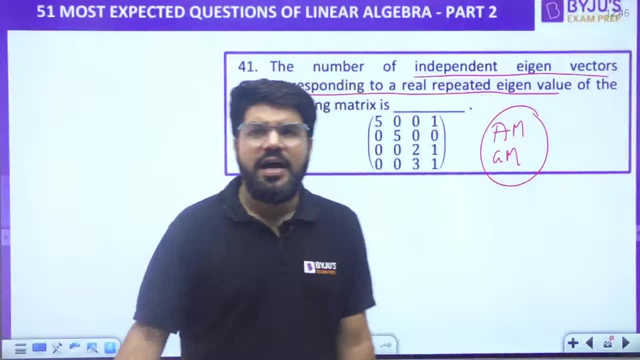 just pasted once again. please have a look now, everybody, now, what is the number of independent eigenvector corresponding to a real eigenvalue, corresponding to a specific eigenvalue? well, what is the eigenvalue of this matter? is gonna call up a deca. it's a 4 cross 4, and that too is it lower. 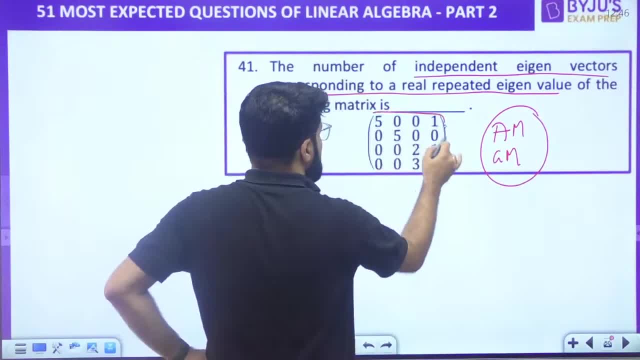 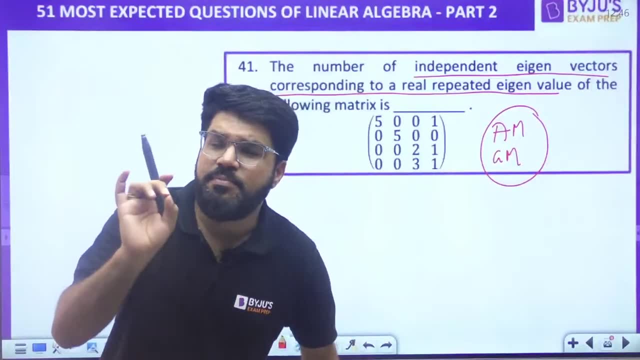 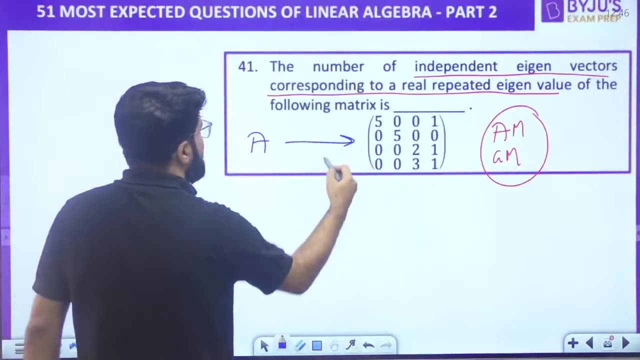 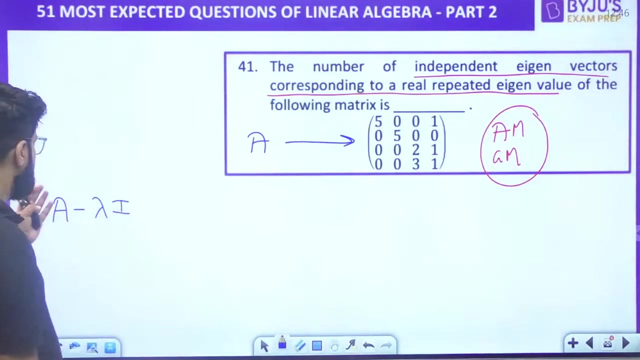 triangular? no, is it upper triangular? no, it is neither upper not over lower triangular. so you have to find the characteristic equation. by the basic method, modulus of a minus lambda i equals to 0. right, let's say this is the matrix a. what is going to be a minus lambda i? 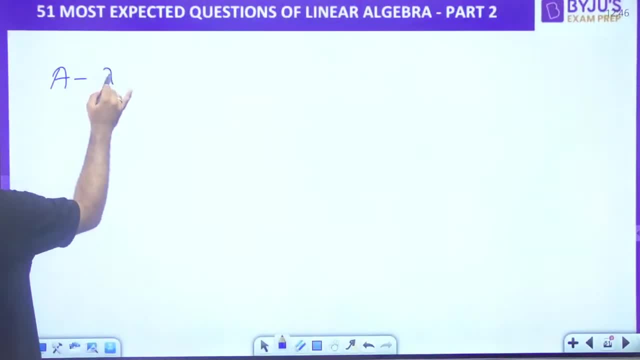 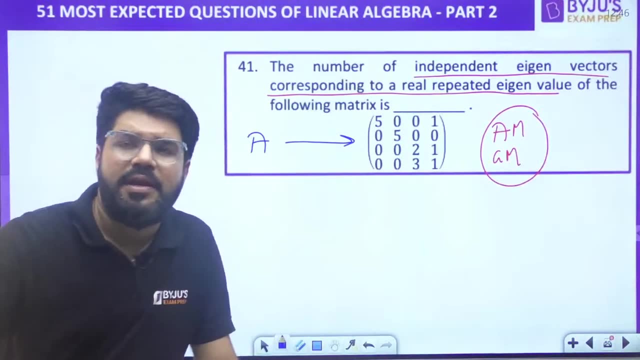 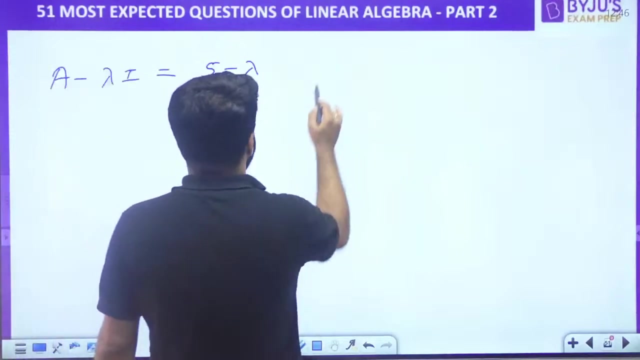 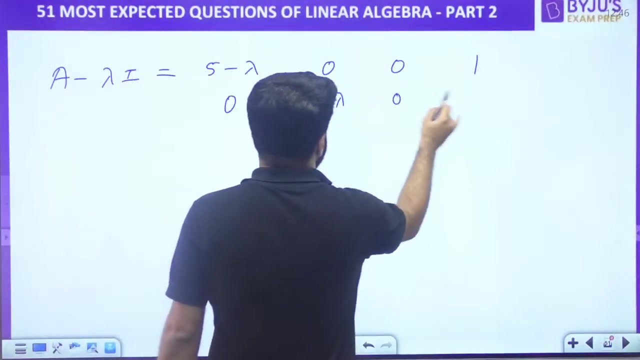 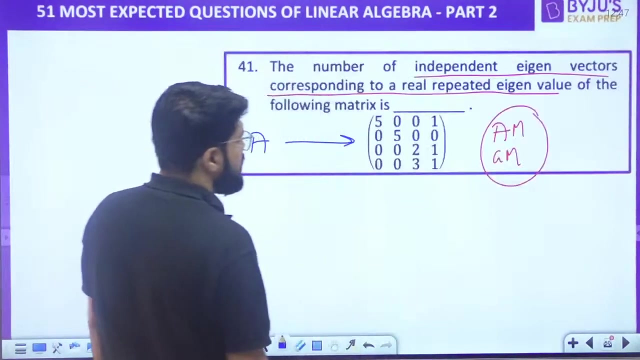 yeah, later then I'll explain you what is am and gm. what is a minus lambda? i minus lambda, i matlab lambda will be subtracted from every diagonal number, so 5 minus lambda, rest will be same: 0, 0, 1. X is 0, 5 minus lambda, 0, 0. last is 0, 0, 2 minus lambda and 1 and 0, 0, 3, 1 minus. 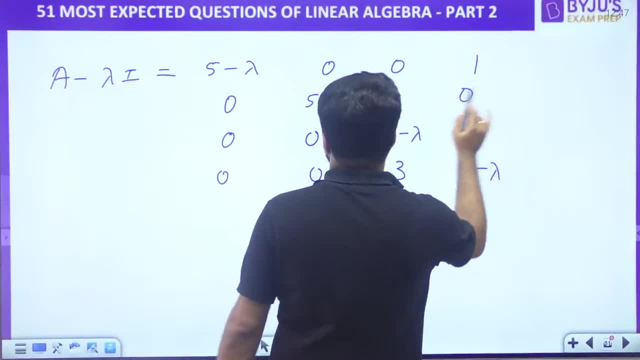 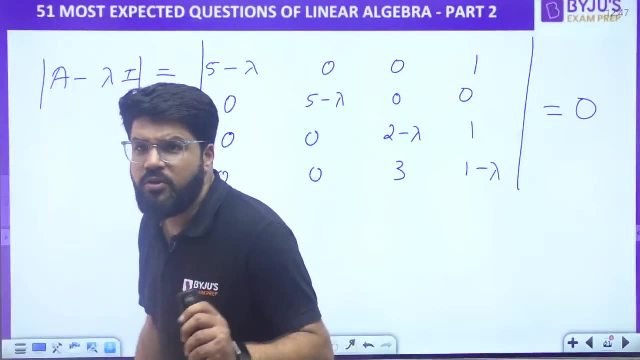 lambda: 0, 0, 3, 1 minus lambda. right, I want the modulus of a minus lambda. I should be equal to 0, because it is a 4 cross 4. I have not given you any direct characteristic equation for 4 cross 4, so what is that? I'm using it over the. 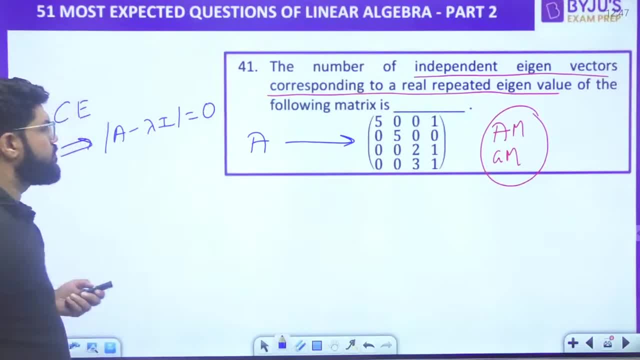 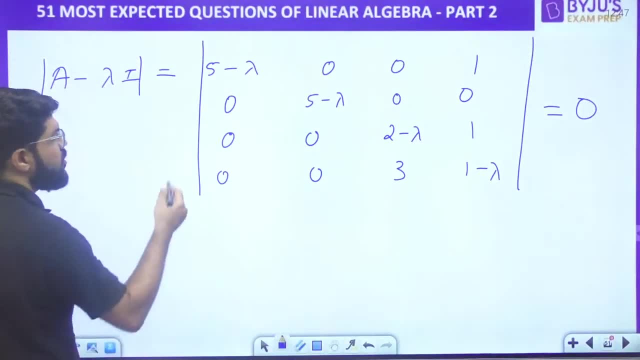 using modulus of a minus lambda equal to zero. i'll explain you the question then. first let us complete the eigenvalue process. okay, first let us complete the eigenvalue process. now determinant: expand about the first column, because most of the numbers are zero here. okay, so i get five minus. 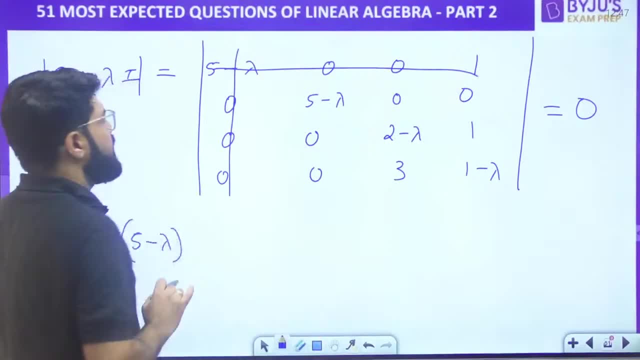 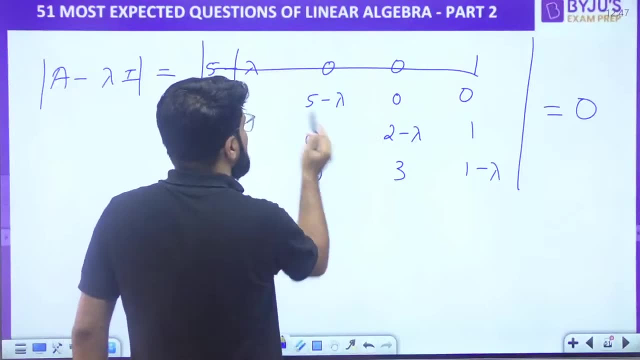 lambda. right, so this row and column is deleted. then then expand. then we are left with a, then we are only left with a three cross three in this three cross three. also now expand about either row. expand about this row. you get five minus lambda. this is again gone. rest two are zero, only this. 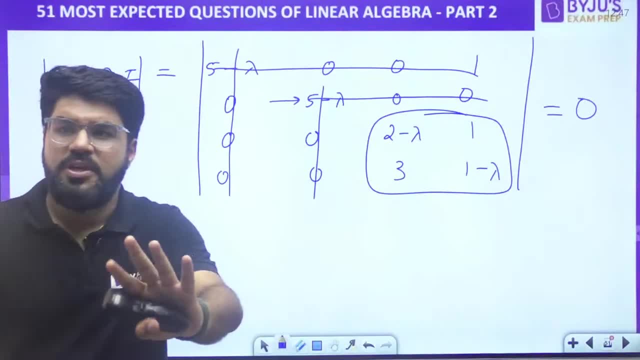 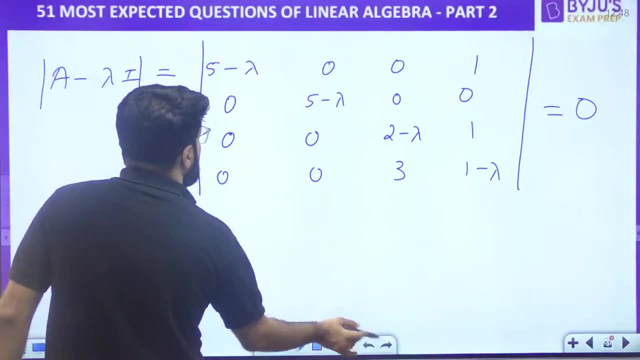 minor will be left. so it is a simple determinant calculation. don't worry, four cross four is not like so lengthy. they have given them numbers will be easy, only right. so applying this logic: five minus lambda, again five minus lambda, and then i have got this particular minor. 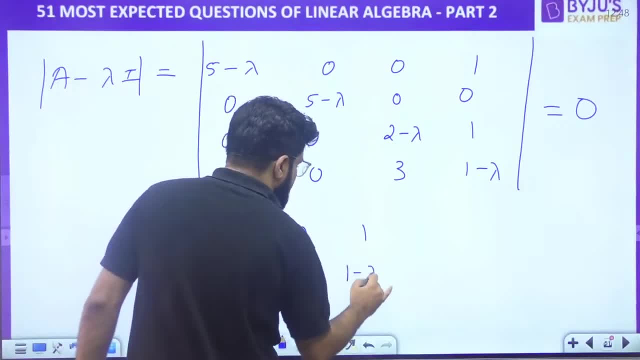 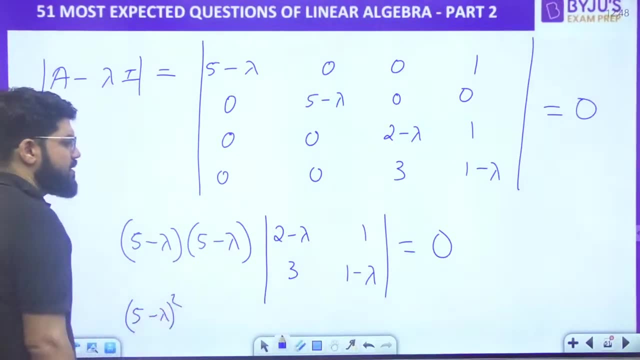 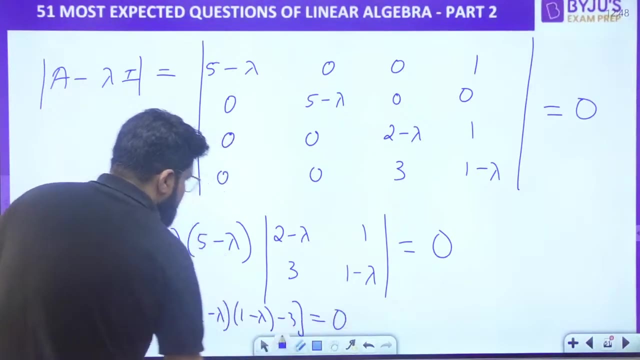 that is two minus lambda, one, three, one minus lambda, you whole equal to 0, right? so i have 5 minus lambda, whole square into 2 minus lambda, 1 minus lambda minus 3, whole equal to 0.. this will be 5 minus lambda, whole square, multiplied by 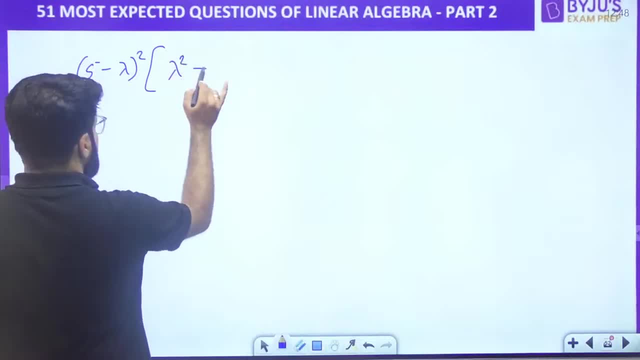 it's lambda minus 1, lambda minus 2, so this will look like lambda square minus 3. lambda plus 2. plus 2 minus 3 will be minus 1, net equal to 0.. so what is going to be? lambda? 5 minus lambda. 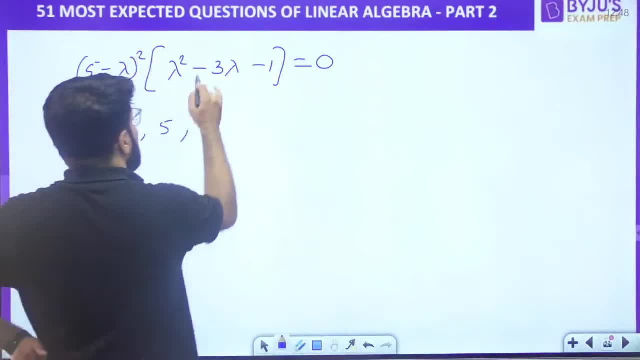 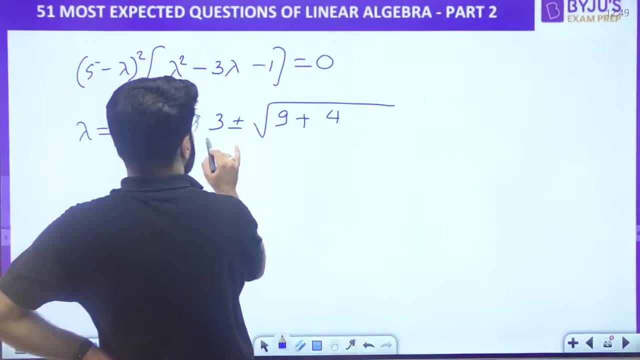 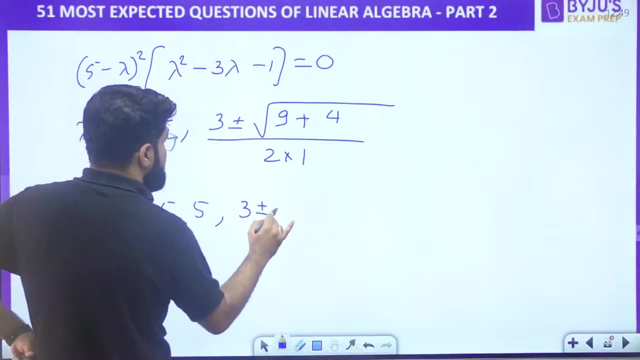 is zero, the lambda is 5 and 5 because it is square, so repeated that right and then from the quadratic i get 3 plus minus root over 3. square, that is 9 minus 4 ac. the minus 4 ac becomes plus 4 divided by 2 into 1. so lambda is equal to 5, 5, 3 plus minus under root of 13. 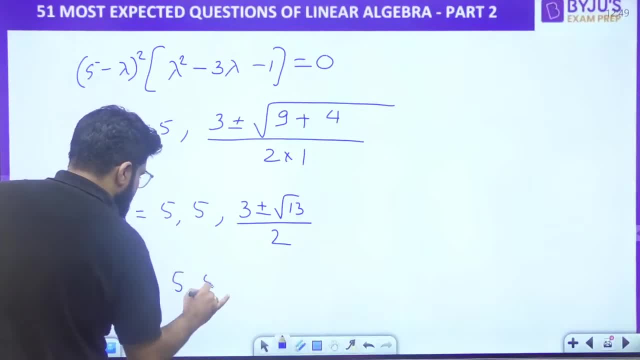 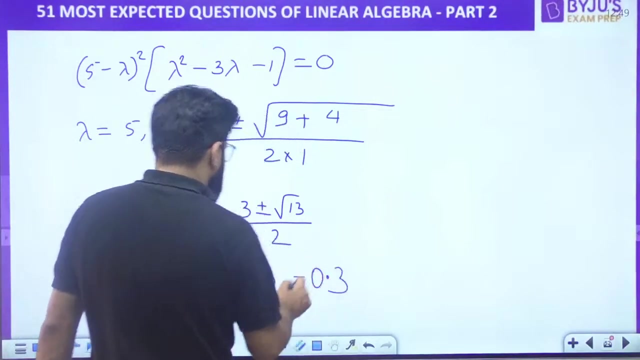 divided by 2, lambda is equal to 5: 5. let me me give you these values. right? let me just write down these values for you: 3.3, approximately. I am writing 3.3 and next will be minus 0.3,. this minus 0.3, okay. 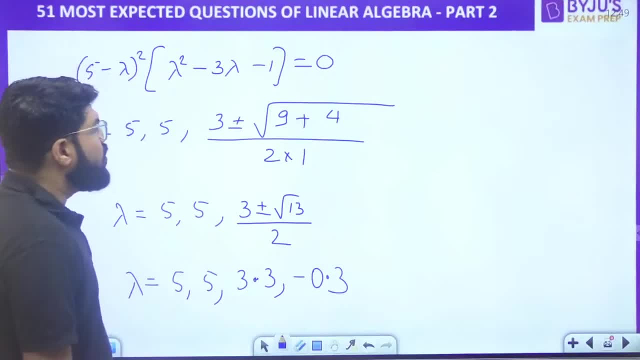 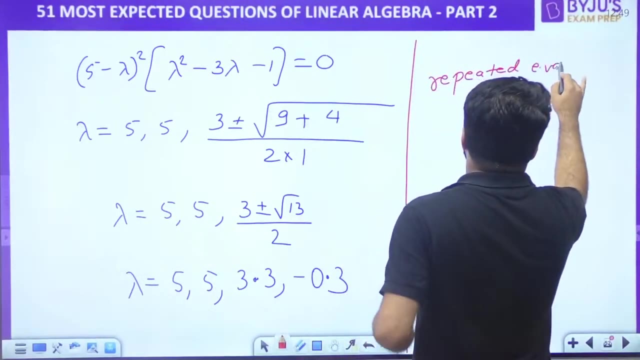 Okay, now eigen number of independent eigenvectors corresponding to a real repeated eigenvalue. what is that repeated eigenvalue? 5 is the repeated eigenvalue. There are 4,. what is that repeated eigenvalue? All are real, but what is that repeated eigenvalue? 5.. How many? 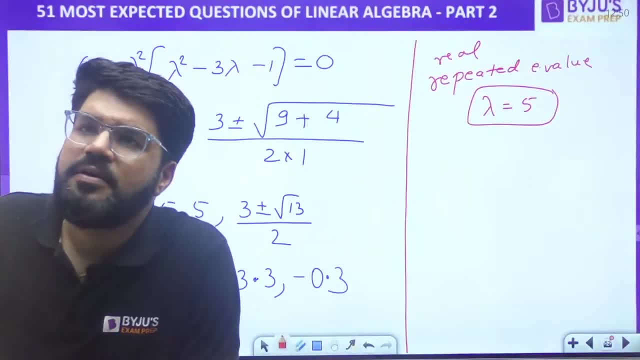 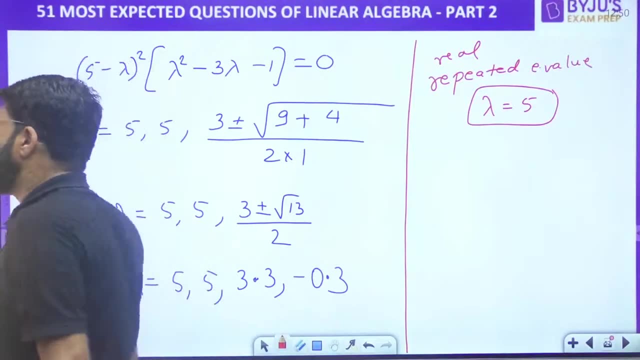 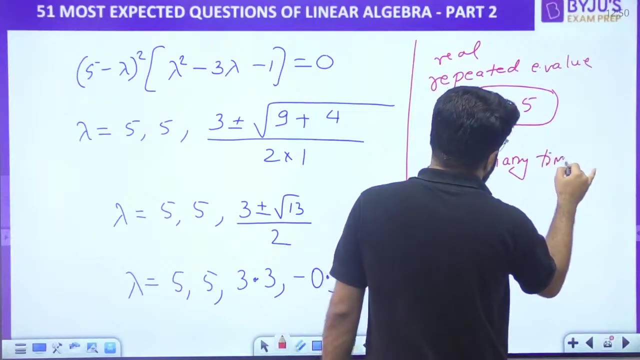 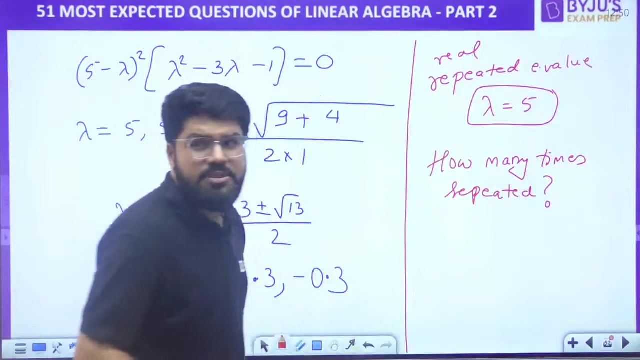 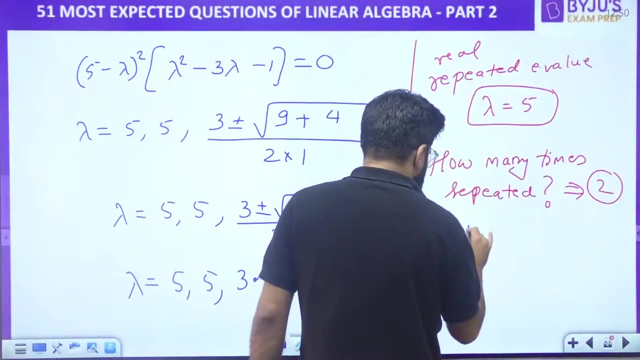 times it is repeated. How many times it is repeated Everybody? how many times it is repeated? 2 times. That is known as. that is known as its AM, that is known as its AM algebraic multiplicity. How many times repeated? It is repeated 2 times. right, I write down its AM equal to: 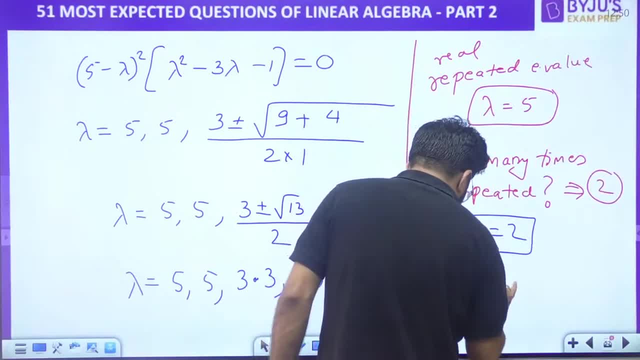 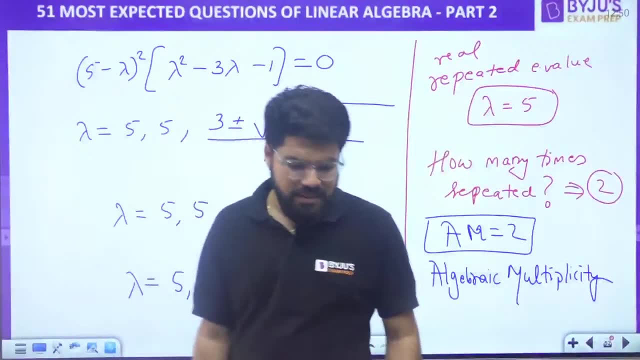 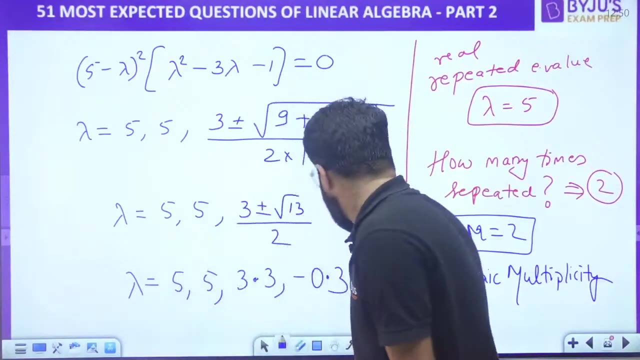 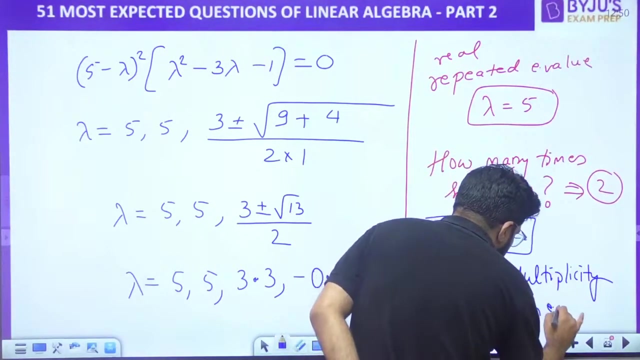 2, AM, known as. So what is the meaning of algebraic multiplicity? Just note down one more concept here: The number of times an eigenvalue is repeated. GM is also mentioned, Ravi, just wait. okay, How many times? 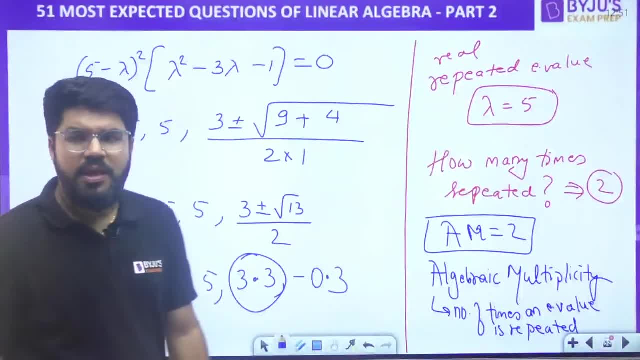 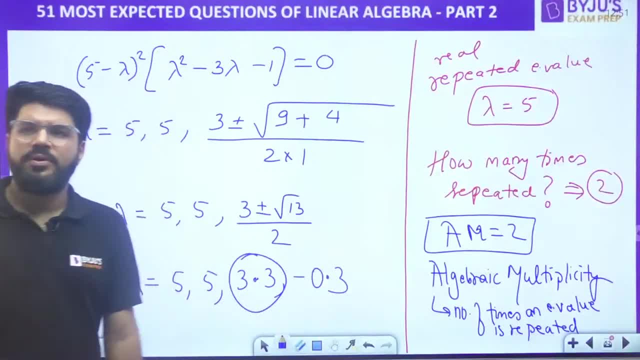 has repeated only once. so am is one. similarly, minus 0.3 am is equal to one. okay, so that is what is the first concept. first one more thing. see, these are not very, very frequent question, but yeah, this is what they can touch, maybe next time. so we should be aware about the concepts am. 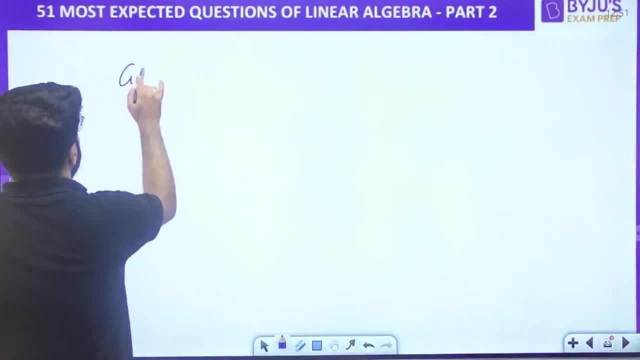 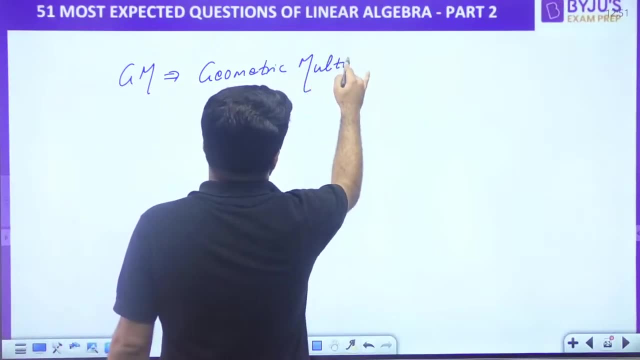 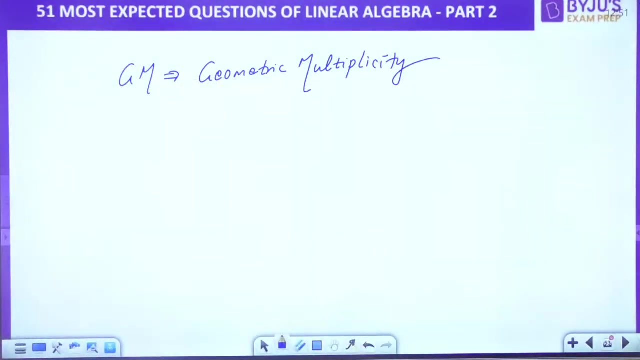 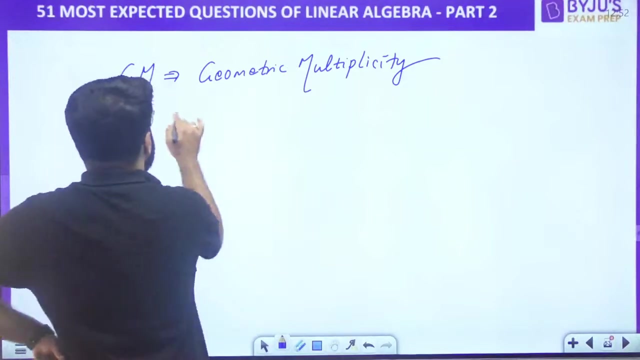 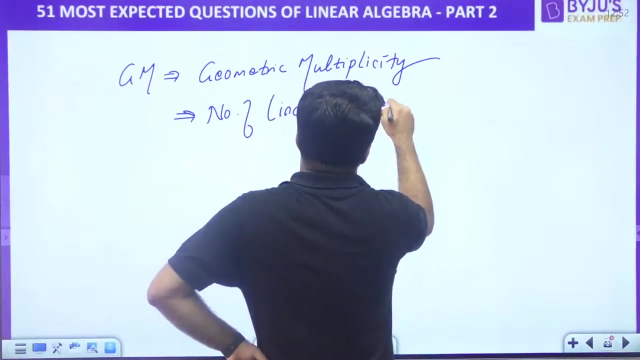 and gm. now, gm, gm dir is known as geometric multiplicity. gm dir is known as geometric multiplicity, geometric multiplicity, geometric multiplicity. gm dir is known as the geometric multiplicity, geometric multiplicity. what is the meaning of geometric multiplicity? it is the number of linearly independent eigenvectors. 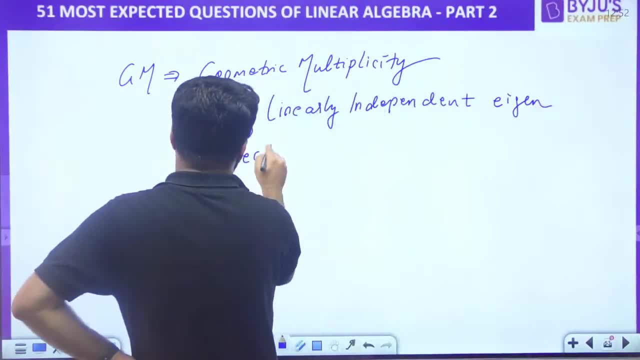 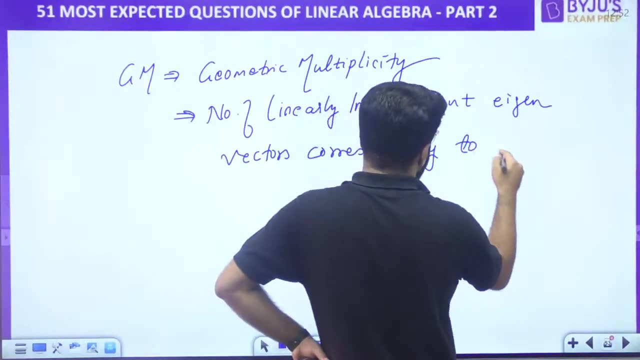 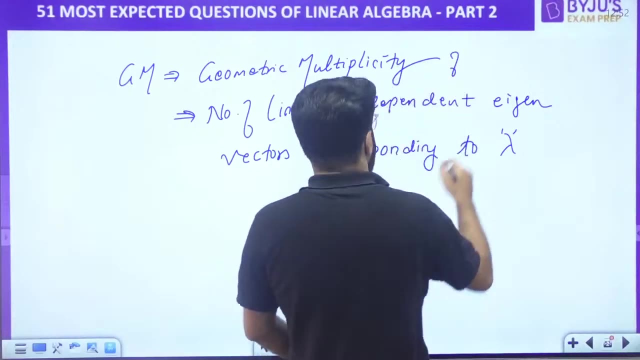 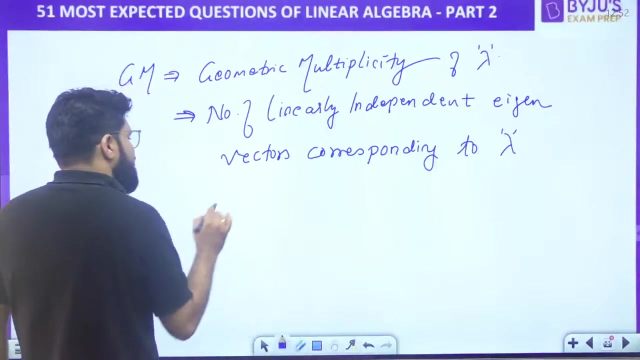 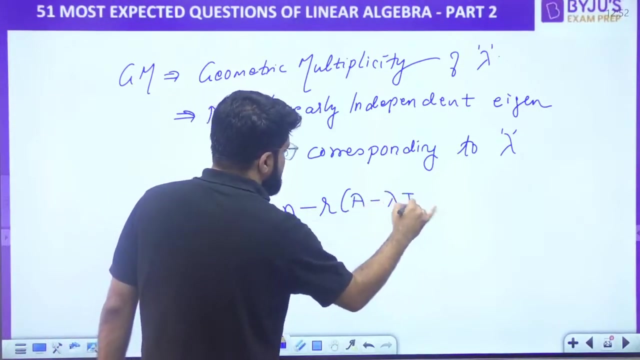 number of linearly independent eigenvectors corresponding to. corresponding to lambda. this is the geometric multiplicity of lambda, of any eigenvalue lambda, the number of linearly independent eigenvectors corresponding to it. and how do you find this? it is simply given by the formula n minus rank of a minus lambda i. 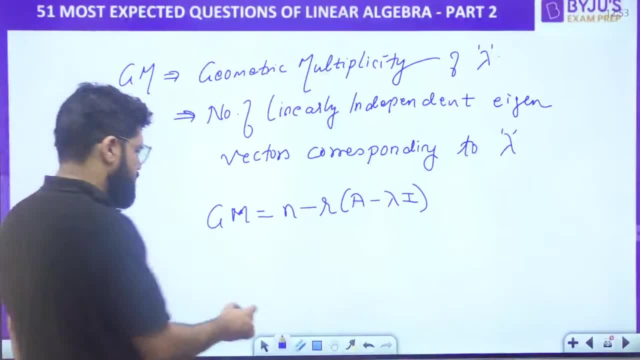 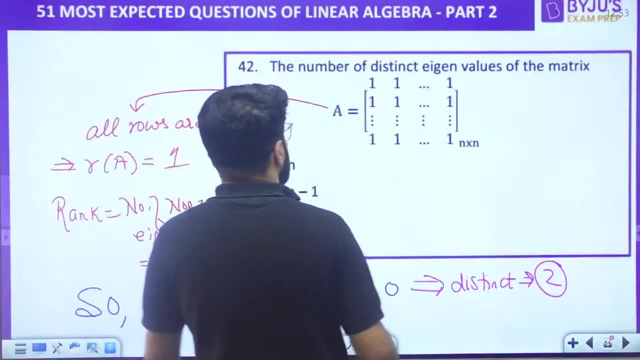 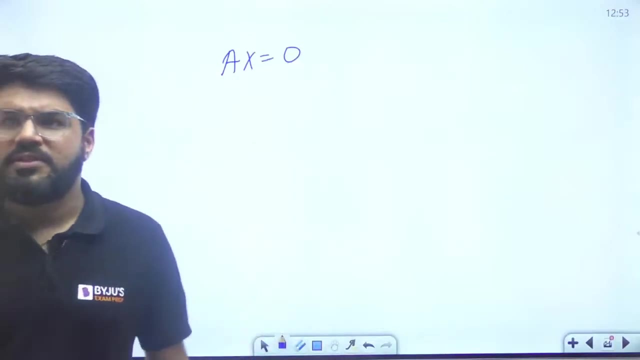 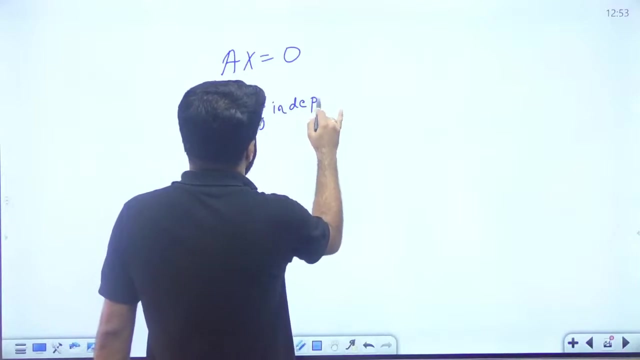 also by the formula for the dud me to use. it is by yesterday's concept of homogeneous system of equation. right at this point, ourho, we are knowing that is the solution today. Конечно, cisco 아니야. i crow n a, what else? we have learned today too. at yesterday we are learning ax equal to zero. and if it has non-trivial solution? if it has non-trivial solution, how many number of independent solutions does it? das塞 cowboy says this couple of 독, zero, n. and if it has nontriverial solution, how many number of independent solutons does it have? lets say, a number not of und Issua. What are the other two solutions? 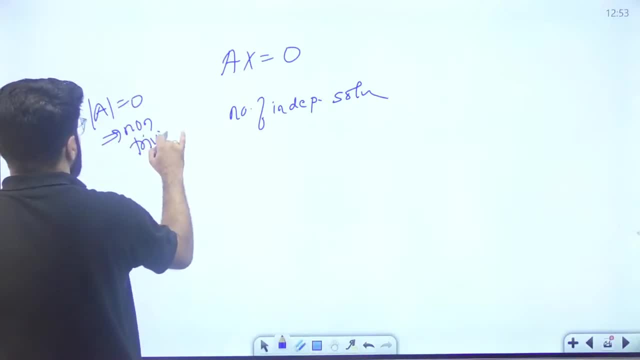 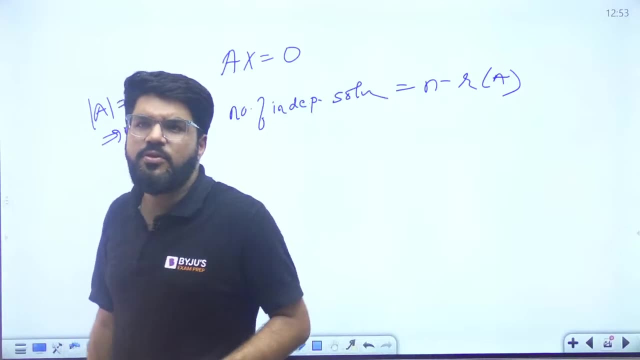 to zero means non-trivial. here also we have figured out non-trivial solution. only right number of independent solution was given by n minus rank of a. correct now here. what is the equation you are working right here. what is the equation you are working? you are working on a x. 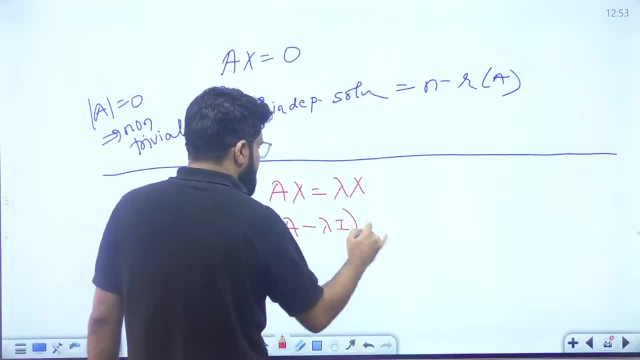 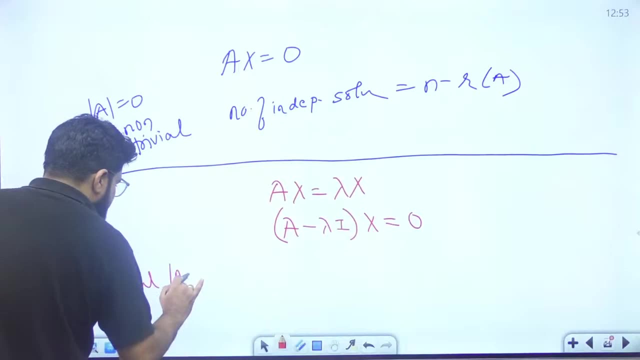 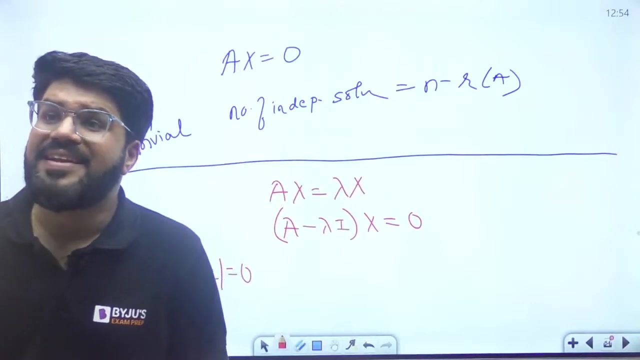 equal to lambda x for the eigenvalue, or a minus lambda i into x equal to zero for non-trivial solution determinant of a minus lambda equal to zero. from here what we got. from here what we got, we got the characteristic equation to find the eigenvalues. right then, number of independent. 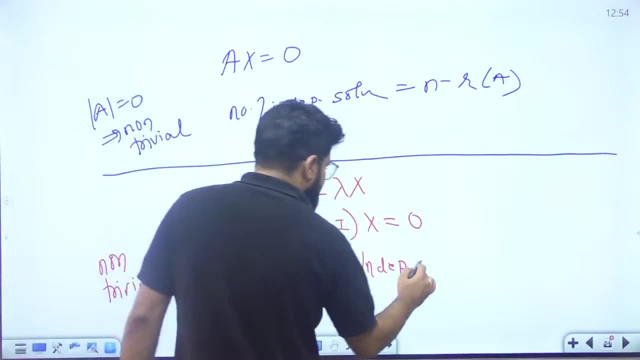 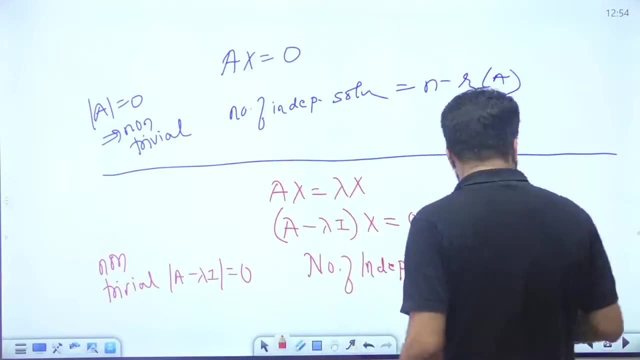 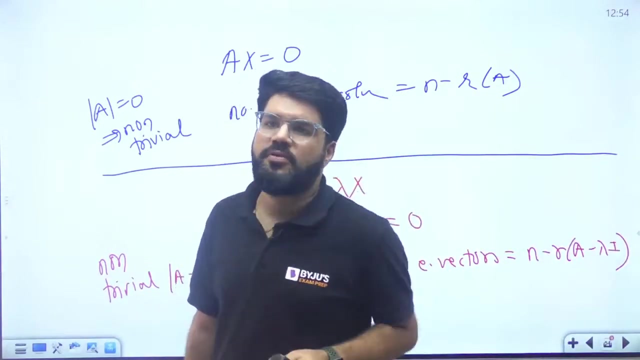 solution. so what is the solution of this equation x? what is x eigenvector? so number of independent eigenvectors should be n minus rank. rank of which matrix? the matrix here is a minus lambda. i got this is how the gm is calculated by the yesterday's concept of homogeneous system of. 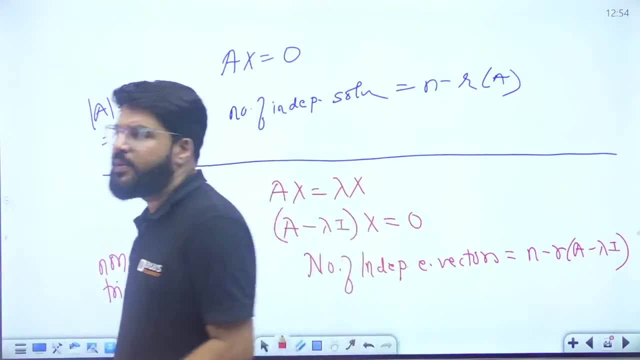 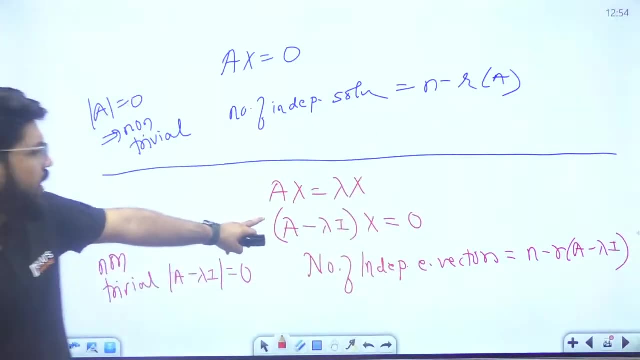 equation: number of independent solutions of the homogeneous system of equation. here the solution is x. x is the eigenvector. so number of independent eigenvectors is n minus rank: rank of what: a minus lambda i, a minus lambda i. so let us come. let us come quickly calculate this. so we are working on. 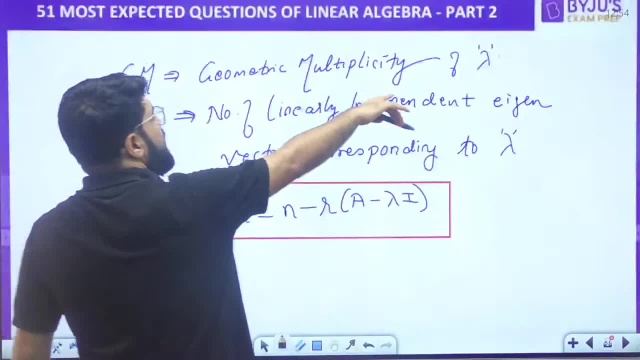 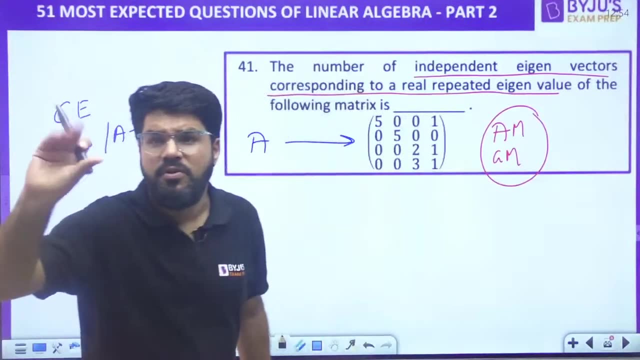 what we are working on, what is said here, calculate the number of independent eigenvectors corresponding to real repeated eigenvalue. so they are asking for which eigenvalue? for the eigenvalue of five? they are asking for the eigenvalue of five repeated, while a five a repeated. 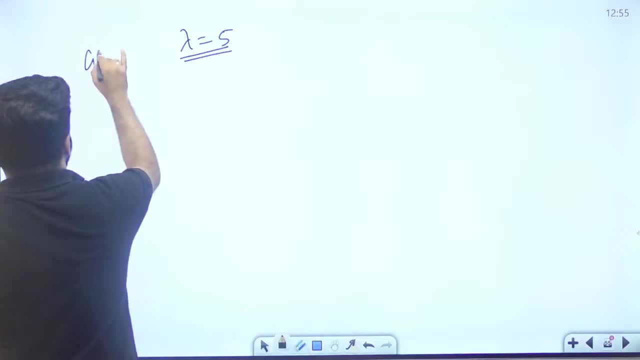 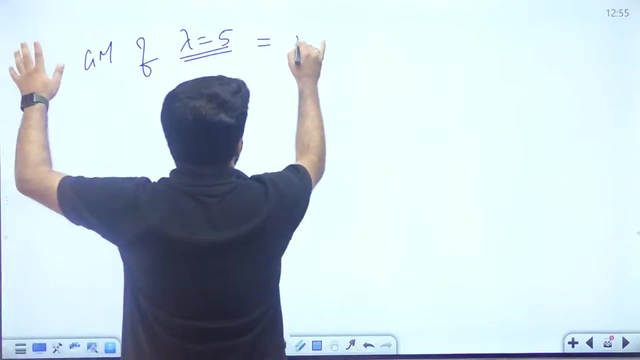 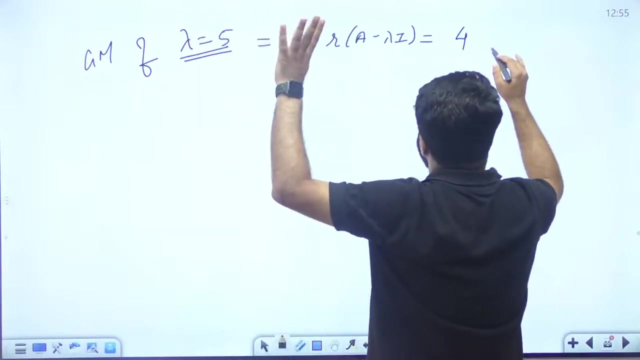 while a five a right. so lambda is equal to five and i want to calculate the geometric mean of that and it should be given by the formula. okay, it should be given by the formula n minus rank of a minus lambda i, that is n. n is four here. size of the matrix is four here minus the rank. 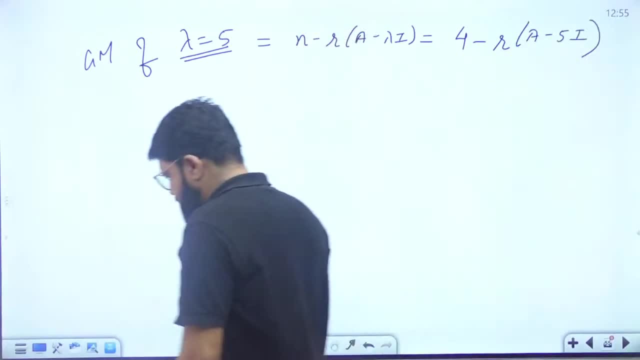 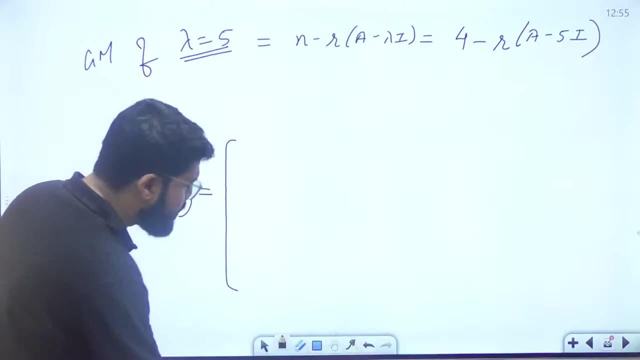 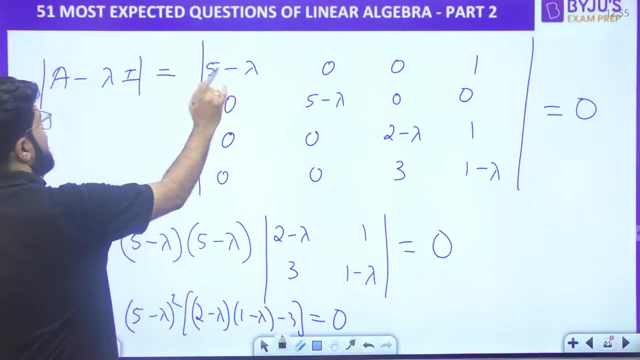 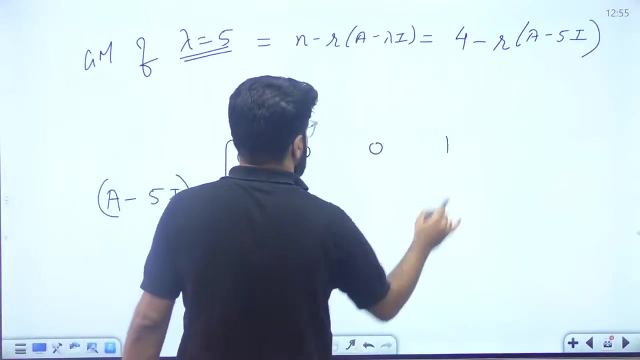 of a minus five i. okay, what is a minus five i? what is the matrix? a minus five i. you will have to see this was a minus lambda, so we will keep five instead of lambda. so a minus five i. this is zero, zero, zero. one. next row again: place lambda equal to one. so zero, zero, zero, zero. 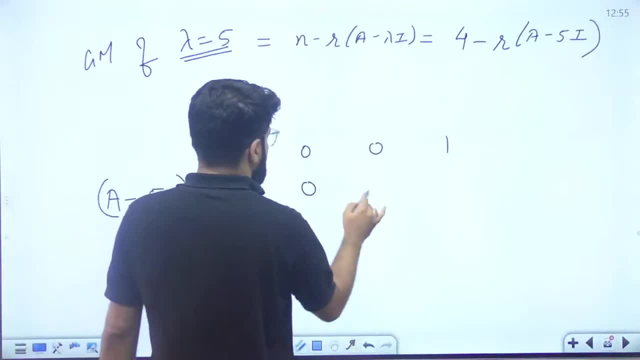 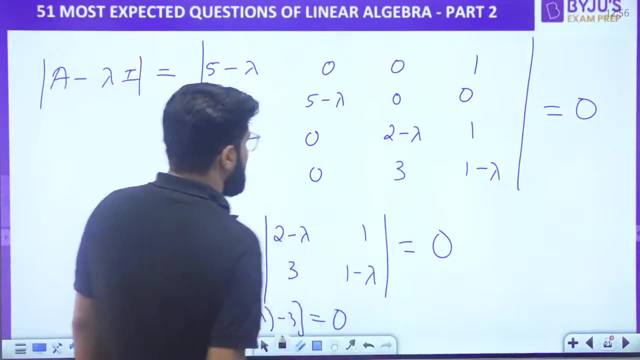 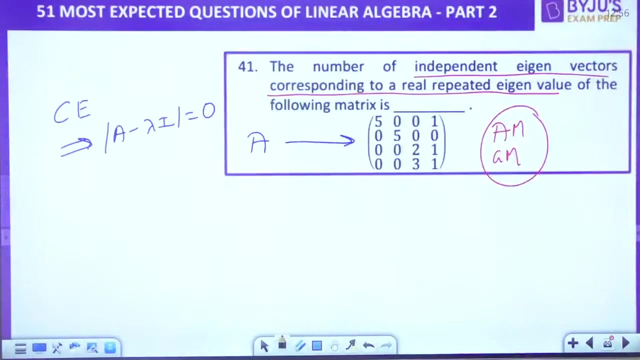 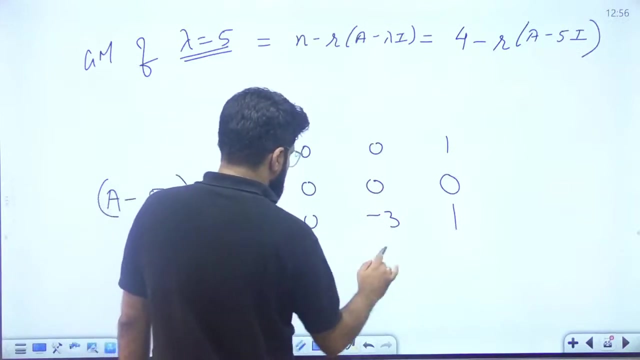 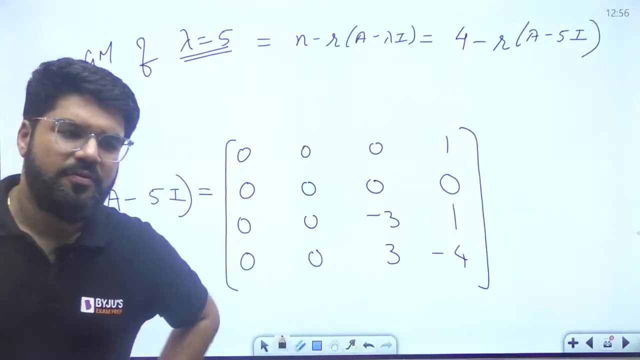 again, place lambda equal to five. so you have zero, zero minus three and one. last row, last row: zero zero three and minus four. what is the rank of this matrix now? what is the rank of this particular matrix? tell me what is the rank of this particular matrix. 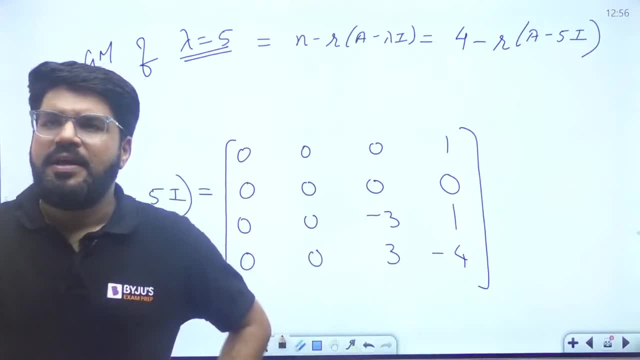 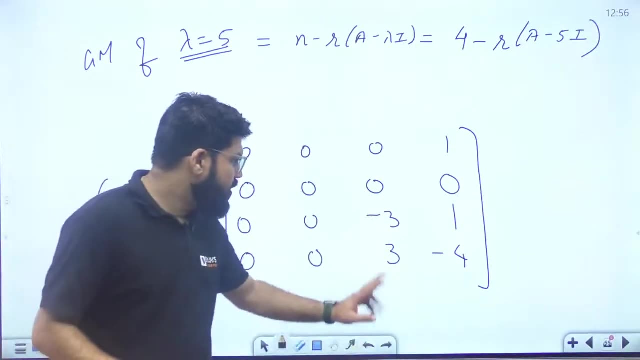 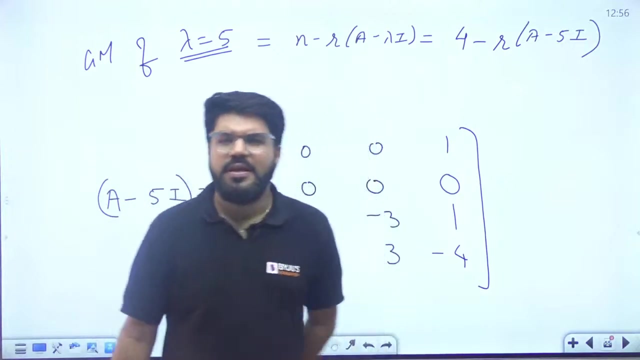 can the rank be three. logic say no. echelon form nothing. one of the row is zero, so determinant is zero. rank cannot be full, rank cannot be four. for the rank to 3. now understand like this. now the understand like this: for the rank: equal to 3. for the rank. 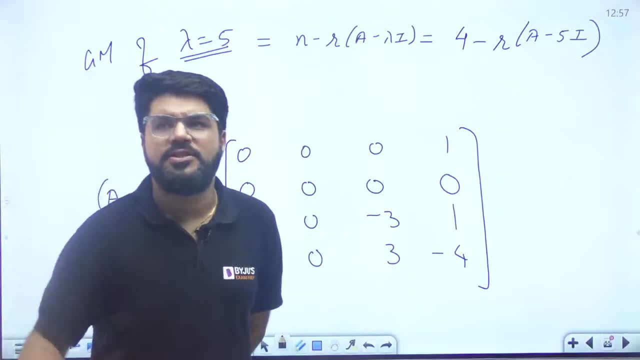 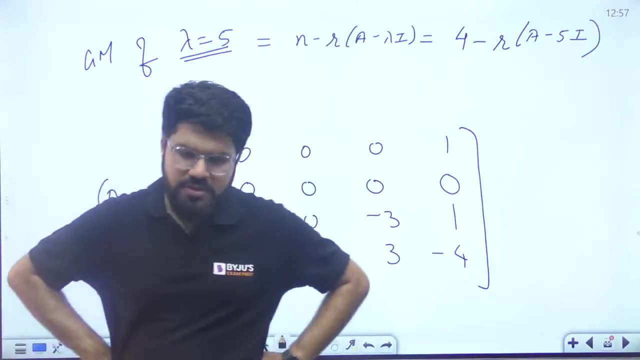 equal to 3. you should have 1, 1, 3 cross 3 minor, which is non-zero. you should have 1, 3 cross 3 minor, which is non-zero. you should have 1, 3 cross 3 minor, which is non-zero. listen to this logically. 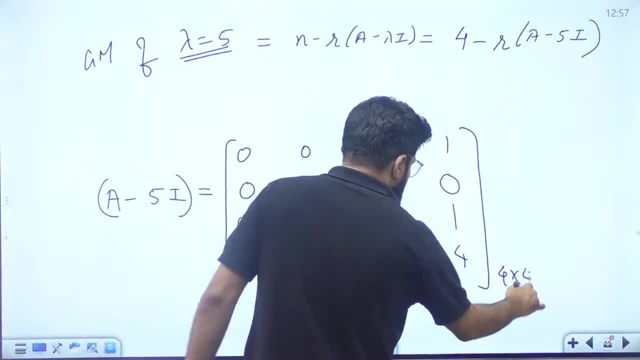 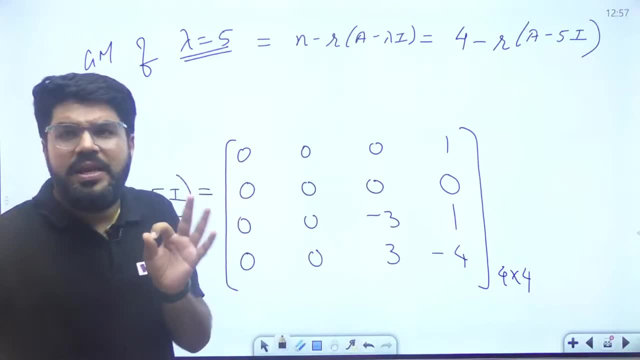 orally. you have a 4 cross 4 matrix, right? how do you make a 3 cross 3 minor? by deleting any one row and any one column. listen to this carefully: by deleting any one row and any one column, correct. so you delete any one column only. now there are two columns, which is entirely zero. 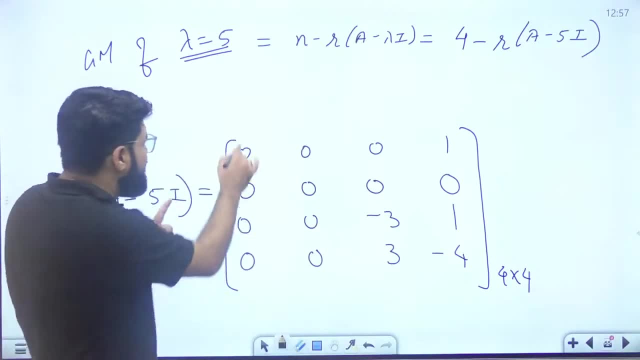 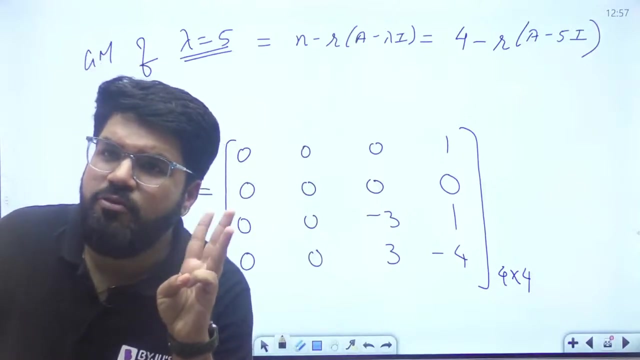 to calculate 3 cross 3 minor, you delete any one column. either you delete this or this, or this or this. but because you delete only one column, there is guaranteed that there is guaranteed that there will be one full, zero column left. whatever 3 cross 3 minor you calculate, there is going to be one full. 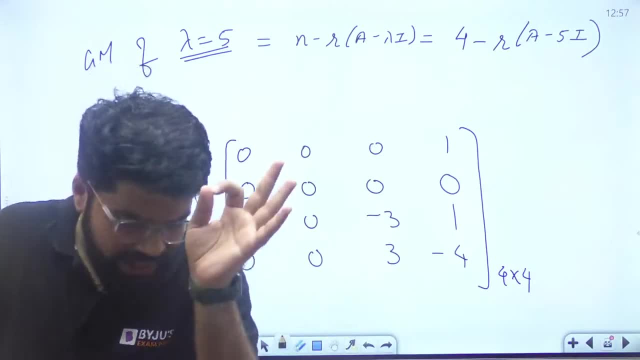 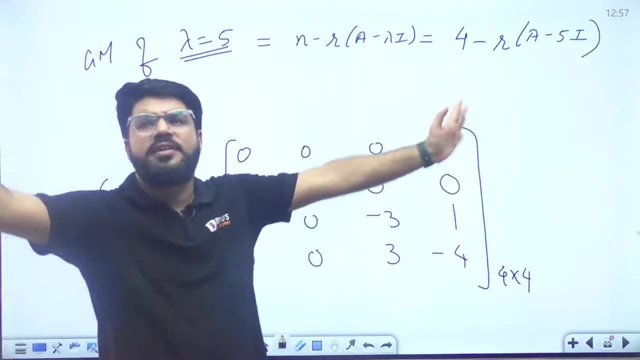 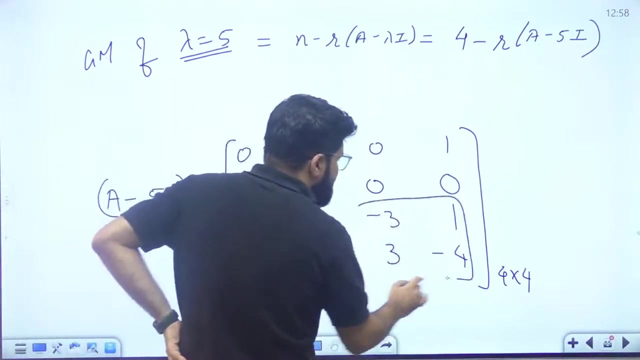 zero column left. and if an entire column of a minor? yeah, if the entire column of a determinant is zero, the determinant value is also zero, the determinant value is also zero. so all 3 cross 3 minors will be zero. all 3 cross 3 minors will be zero. rank 2: 2- is it the rank 2? check this. 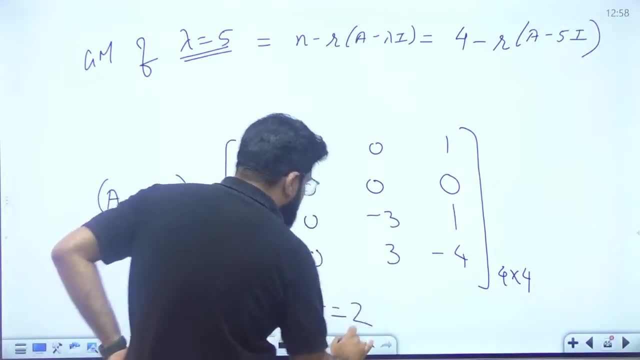 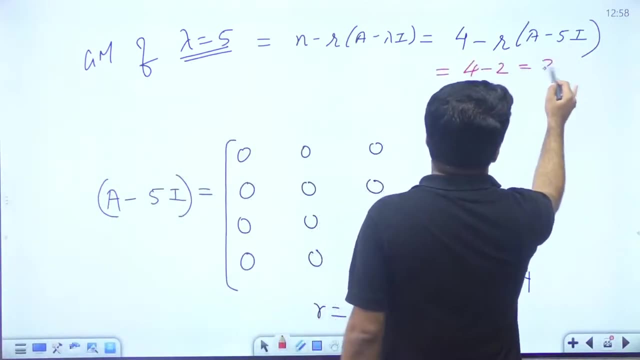 12 minus 3. this is also non-zero, so rank is equal to 2 orally. i have explained you. if you have followed yesterday's class, we can solve this orally. rank is equal to 2. the answer is 4 minus 2 and that is equal to 2. it is a very easy way to solve this problem. so if you have followed, 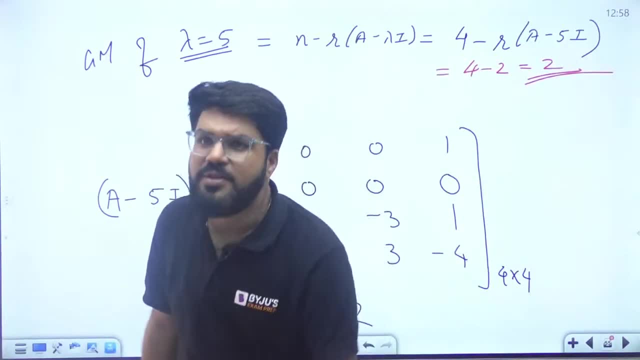 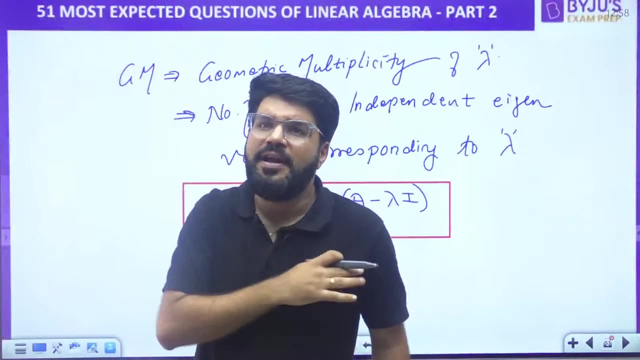 the concept of gm- not very frequent in the gate but i have still covered that concept. also am and gm. am is the number of times an eigenvalue is repeated and gm is the number of linearly independent eigenvectors corresponding to eigenvalue. this is gm. this part is am and 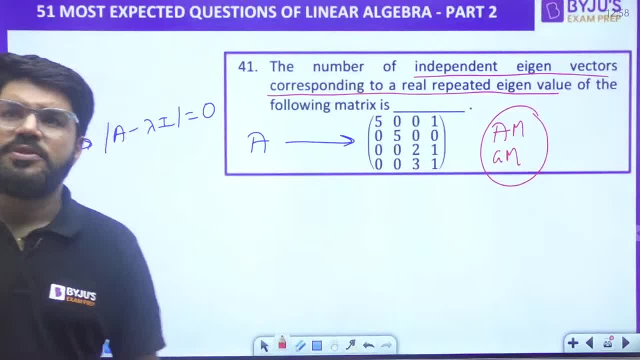 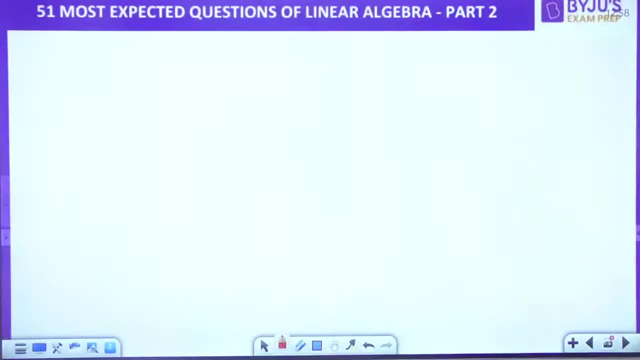 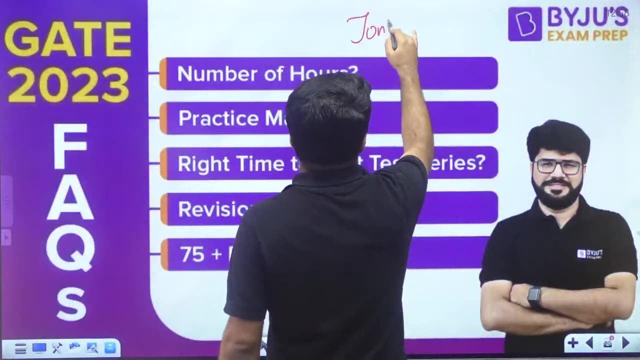 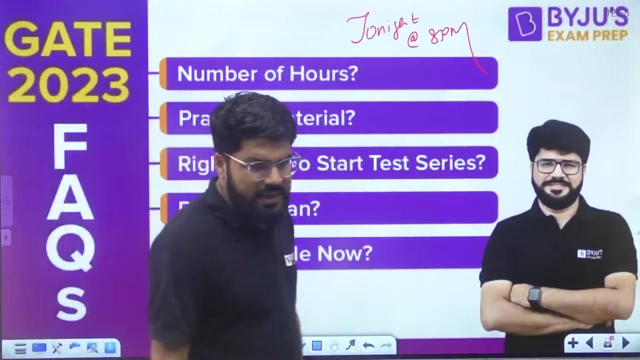 this question is sorted. this was the only question left. 41 rest- we have done rest, we are all done. kylie hamilton also discussed. okay, now guys, now guys. let us connect once again tonight at 8 pm. let us connect once again tonight at the 8 pm. let me see how many of you are enthusiastic for the tonight session. 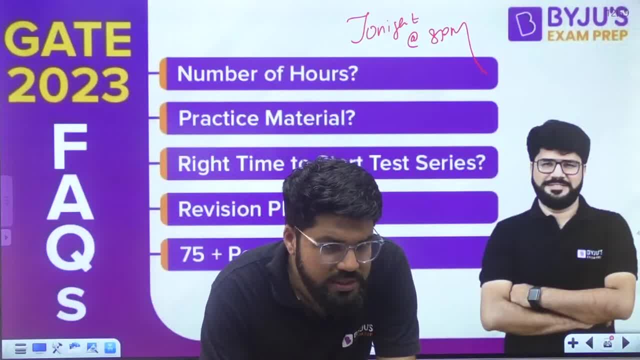 gate 23, all your end moment doubts when to study number of hours. what is the solid revision plan now? because without that solid revision plan you will not be able to perform that good. all of these things. yes, this is the link for the tonight's youtube session. i have shared it with you. 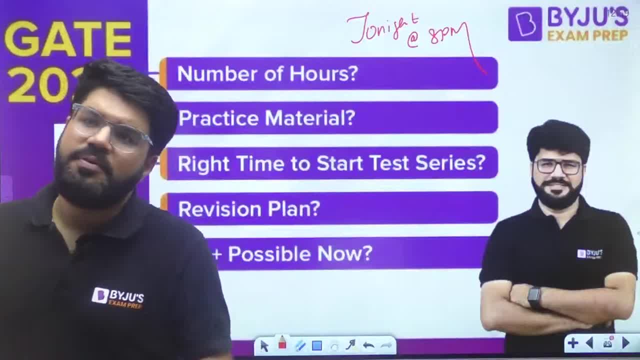 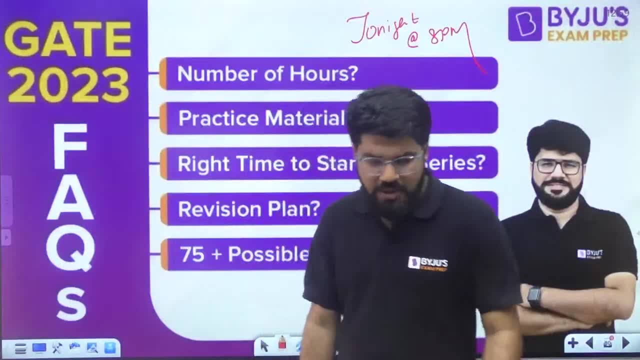 do open the link, set the reminder to join it up on the perfect time and do not forget to like that session immediately, spread the session, share the evening session also, because for any gate 23 aspirant that is also important. the last questions we have in between алҳҳели.